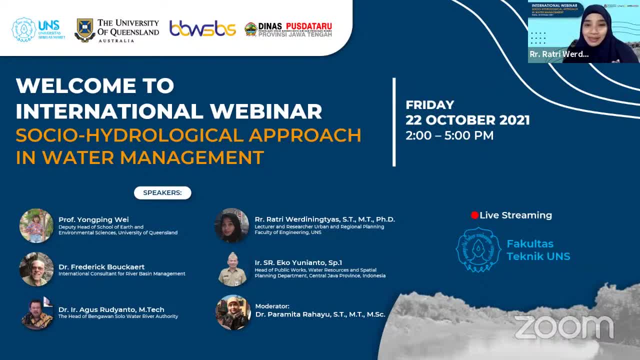 All right, see you guys soon. Yeah, probably I mute myself. Welcome, Okay, Salaam-alaikum, Muhammad. Yeah, good afternoon, good evening everyone. Will you start to AsunastGI graphic? Okay, uh, uh, uh, very soon, uh, uh, what is it? wait okay. 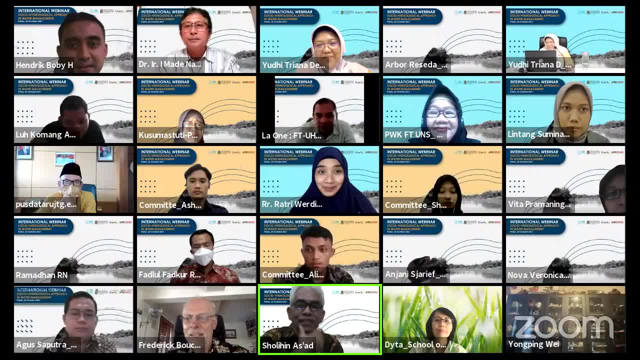 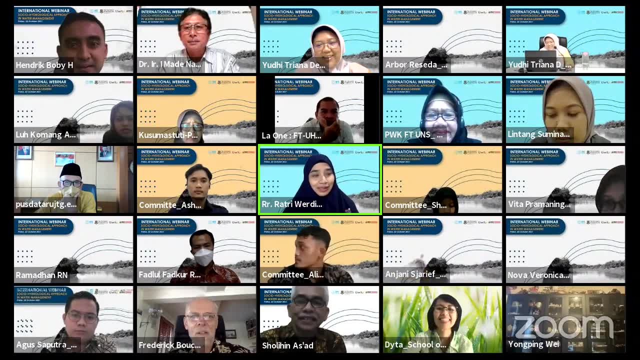 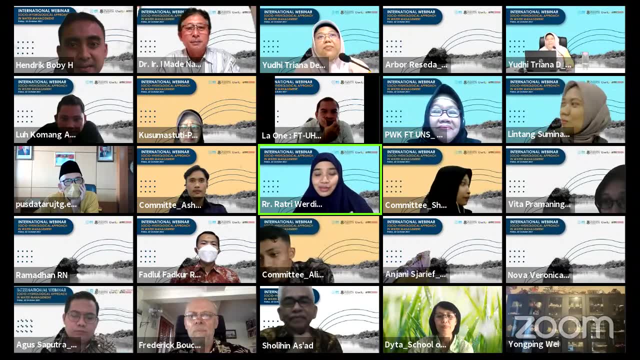 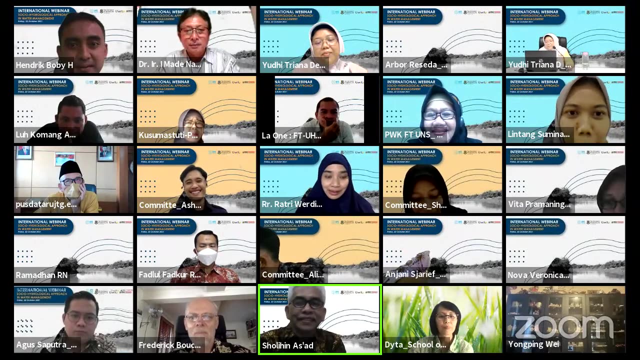 so, congratulations, we have a lot of participants today. yeah, we, we need to close uh last night because it's uh hit until 385 and uh, yeah, we try to remember the participants uh, if they cannot join uh, so we can uh to uh youtube, okay, okay, and this is surprising because in very short time we can arrange this. 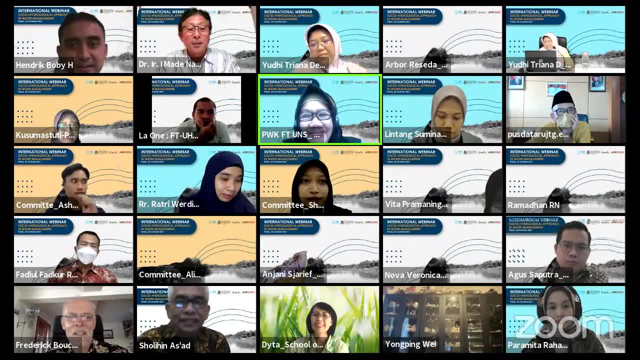 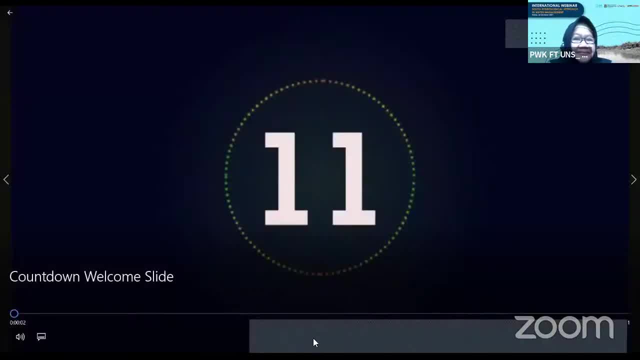 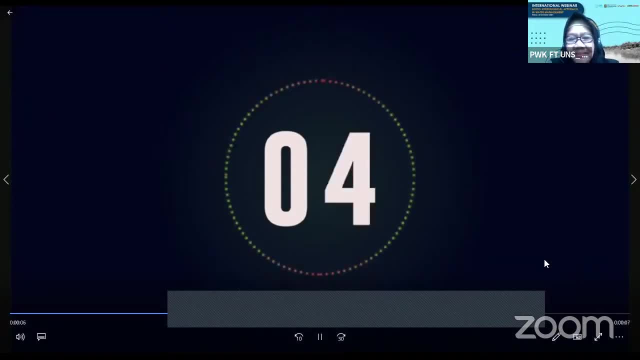 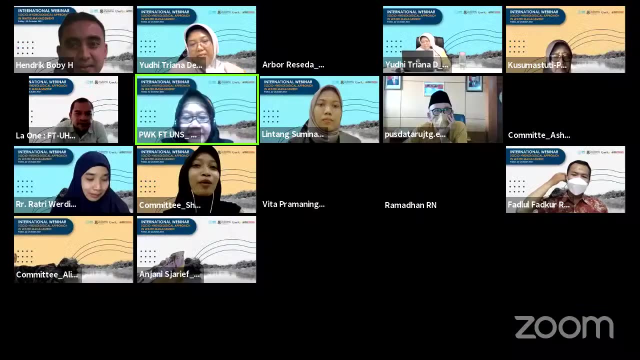 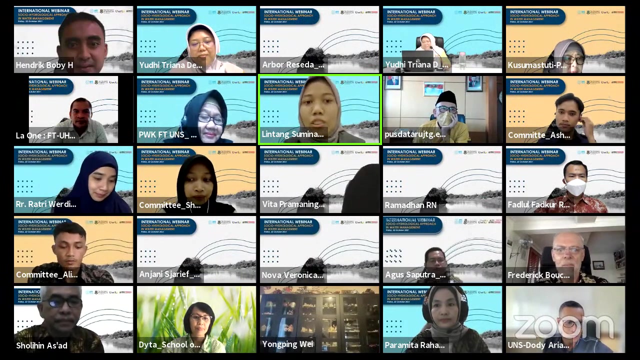 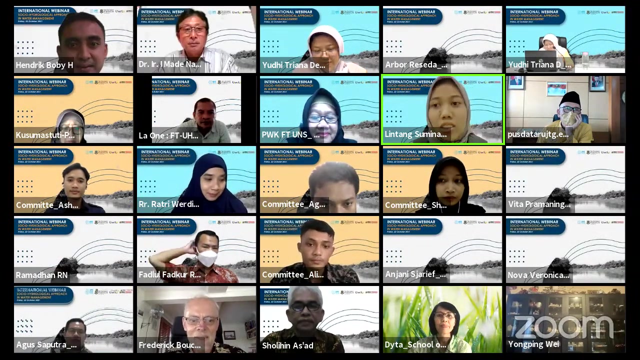 this event and lots of participants has been registered. so good afternoon, ladies and gentlemen. warm greetings from surakarta, indonesia. i hope you are all doing well in the midst of this challenging situation. my name is lindang seminar and it is my pleasure to welcome you all to this. 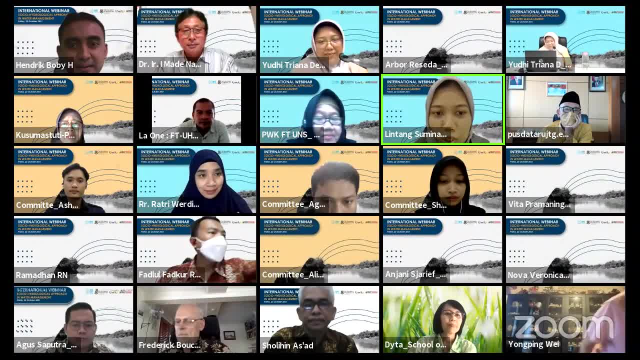 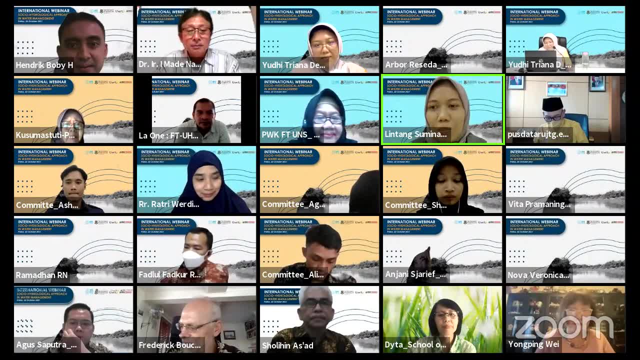 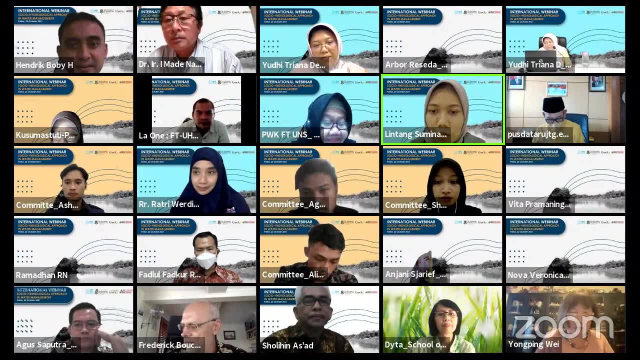 international webinar: socio-hydrological approach in water management, hosted by urban and regional planning program faculty of engineering universitas surakarta, indonesia. i would like to thank you for joining us on this zoom meeting platform. you can also access this webinar from facultas technique uns youtube channel. 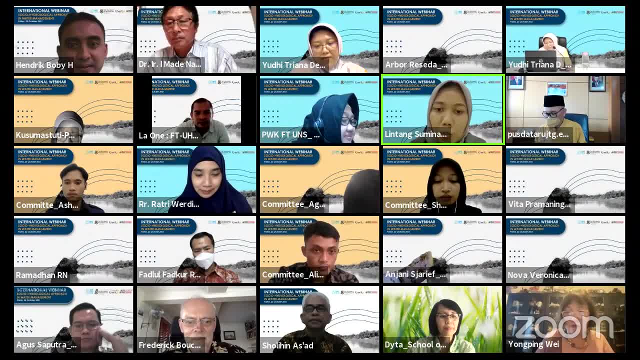 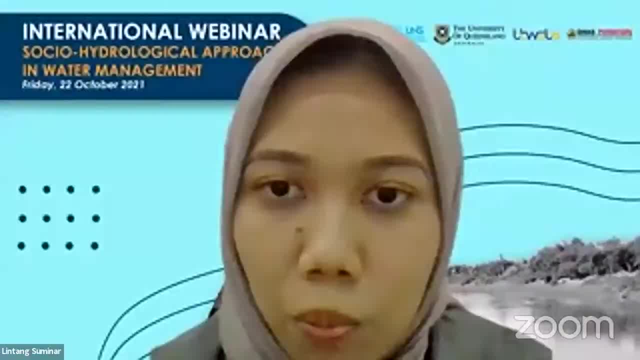 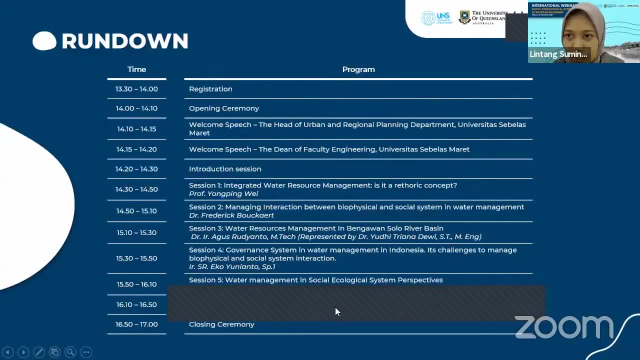 ladies and gentlemen, before we start i'd like to read the program agenda and the set of rules of today's webinar. so here is the program agenda, starting with the opening and then after this, we are going to have the welcoming speech from the head of urban and regional planning department and also from the team of the faculty. 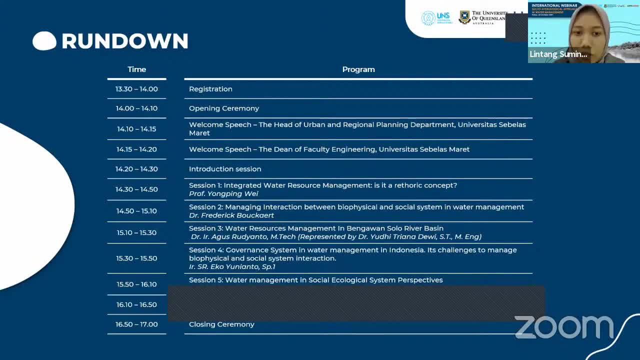 of engineering universitas, the blast matter, and after that we're going to have the presentation session from our speakers today, and this session will be moderated by the moderator. we have five sessions. the first session will be delivered by professor yong ping wei from the university of queensland, australia. good afternoon, or maybe it's already evening there. good evening. 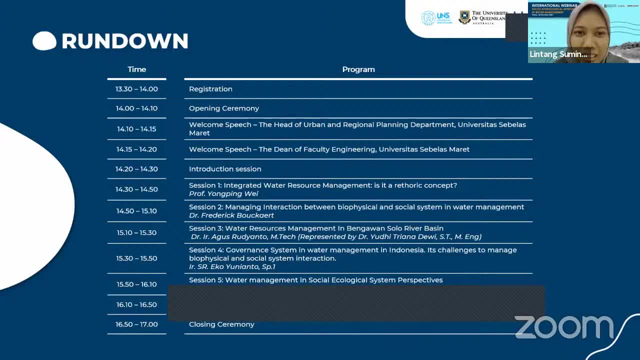 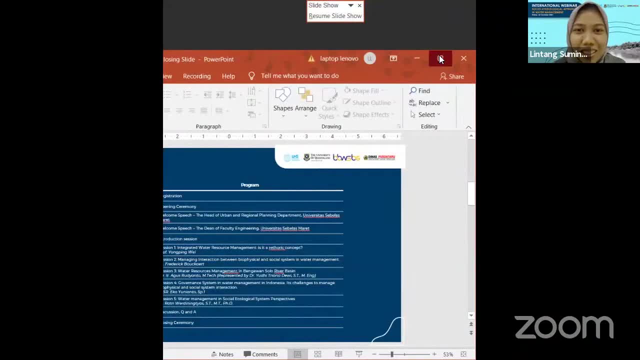 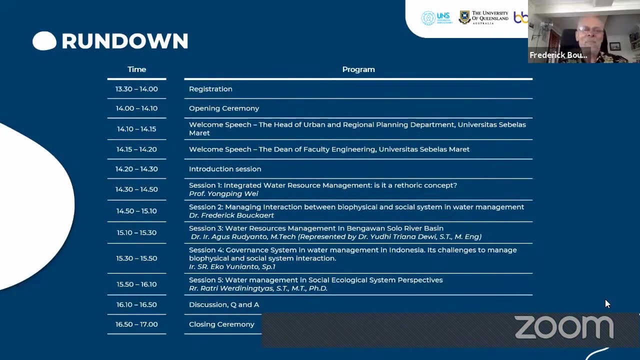 professor yong ping wei, and the second session will be delivered by dr frederic. good afternoon or good evening, dr frederick. thank you, um, it's still late afternoon here. thank you, okay, the third station will be uh delivered by uh bbws bengawan solo. that today will. 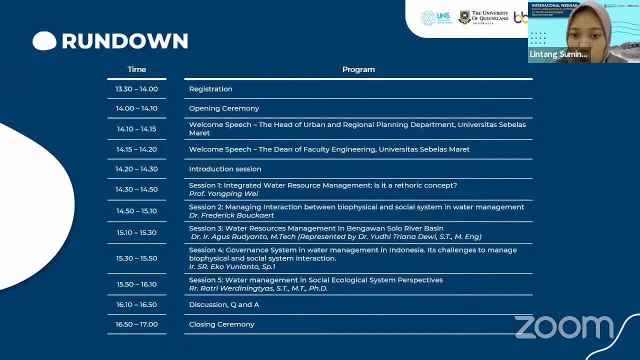 be represented by uh, ibu dr yudi triana dewi. good afternoon. selamat siang, ibu, and the fourth session will be delivered by uh, the head of public works, water resources and special planning department, central java province, indonesia, bapak insinyur eko yunianto sp. satu. selamat siang, good afternoon. 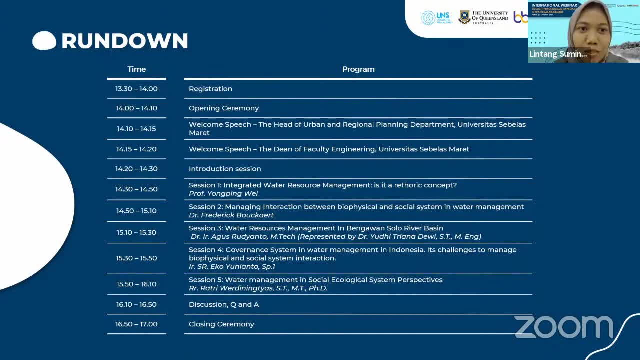 and the first session or the last session will be delivered by the head of public works, water resources and special planning department, central java province, indonesia. uh, this session will be delivered by the head of public works, water resources and special planning department, central java province, indonesia, and the last session will be delivered by the head of public works, water resources and special planning. 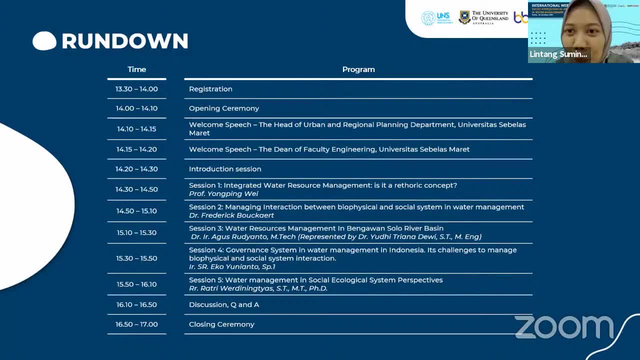 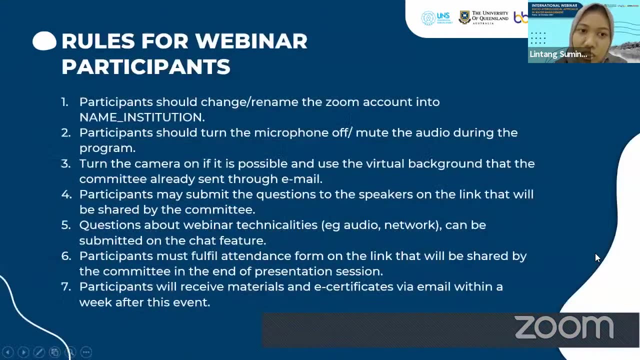 department, central java province, indonesia. you know, the first session will be delivered by ibu ratri werdenih, phd lecturer, and also the researcher from urban and regional planning department, uh, faculty of engineering, uns. selamat siang, sayang, bu ratri, selamat siang. 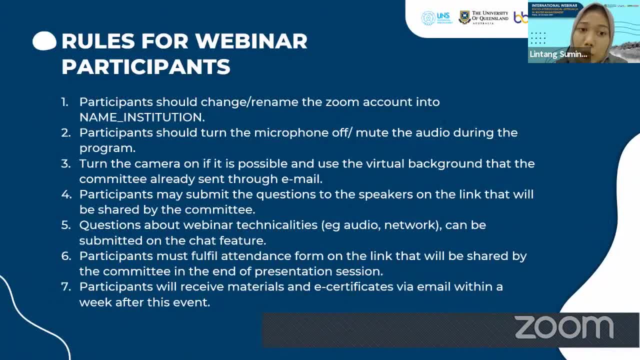 everyone and uh, ladies and gentlemen, i would also like to inform you the rules in this webinar, so please pay attention to this following instructions: The participants should change or rename the Zoom account into name underscore the institution or the affiliation. The participants should turn the microphone off or mute the audio during the program. 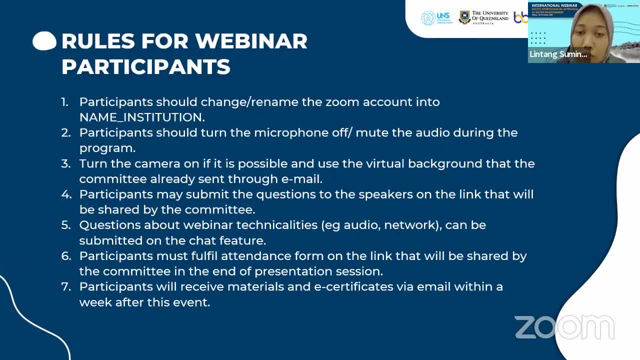 The participants are also expected to turn the camera on if it is possible and use the virtual background that the committee already sent through the emails. The participants may submit the questions to the speakers on the link that will be shared by the committee later, And the questions about the webinar technicalities, like the audio or network, can be submitted on the chat feature on this Zoom meeting platform. 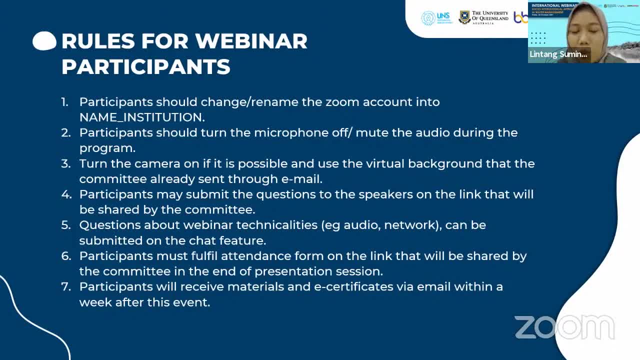 The participants must fulfill attendance form on the link that will be shared by the committee in the end of the presentation session And participants will receive the materials and e-certificates. The participants will receive the materials and e-certificates via email within a week after this event, only if participants completely fill the attendance form. 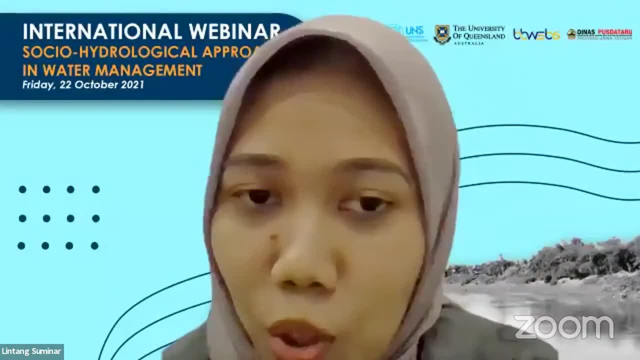 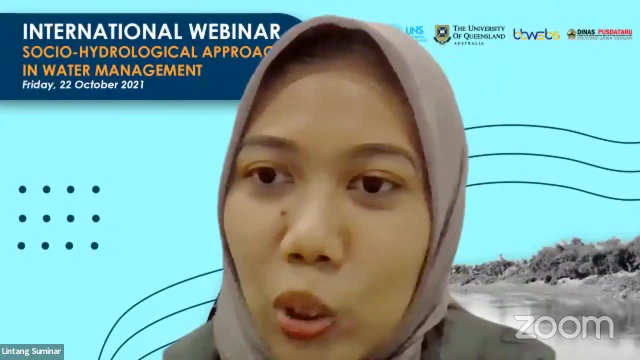 So next I would like to welcome Professor Winnie Astuti, who is already here at the head of Urban and Regional Planning Program to deliver the opening speech. So please, Bu Winnie. Thank you very much, Bu Winnie. Thank you for your time. 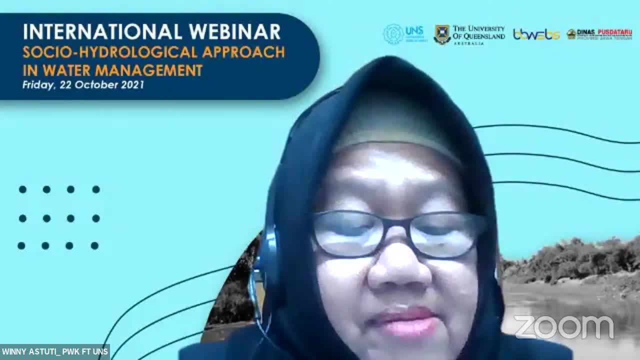 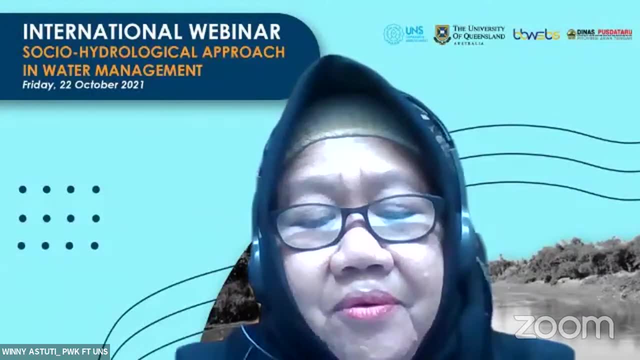 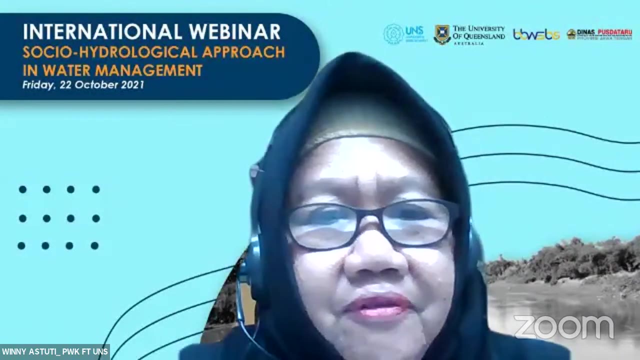 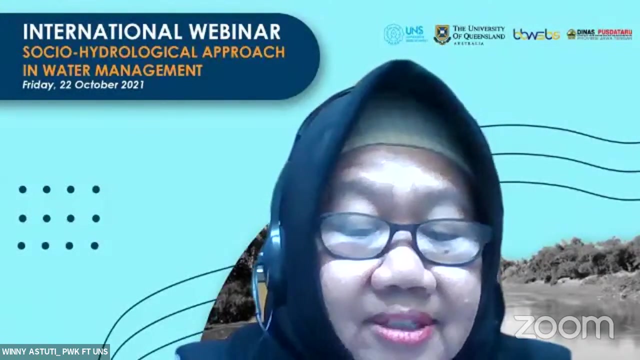 Good afternoon everybody. Assalamu alaikum, My excellency the Dean of the Faculty of Engineering, Universitas Bas Marat for the Faculty of Art and also the Dean of the Faculty of Science. I'd like to thank, of course, all the keynote speakers of this webinar, Professor Yongping Wei. 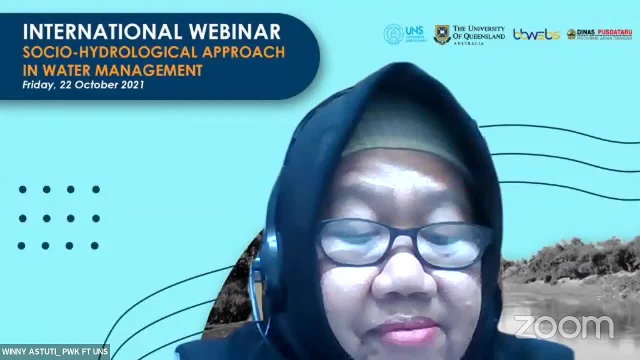 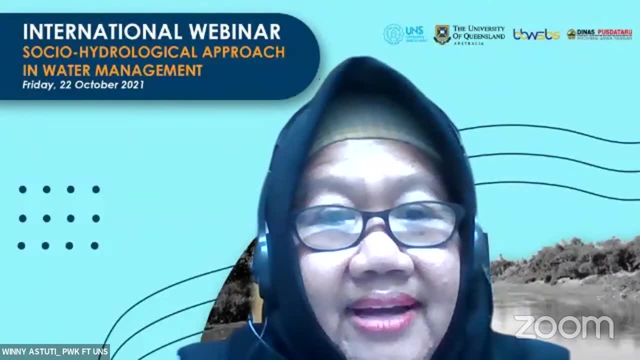 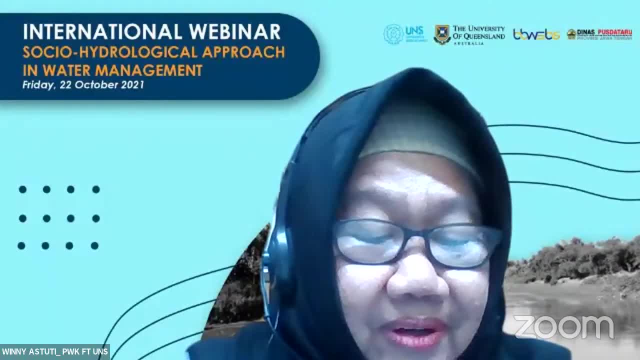 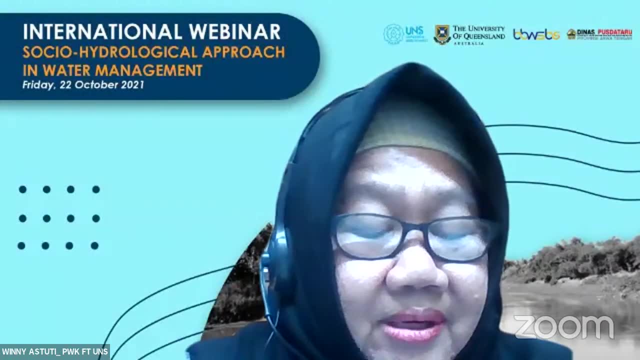 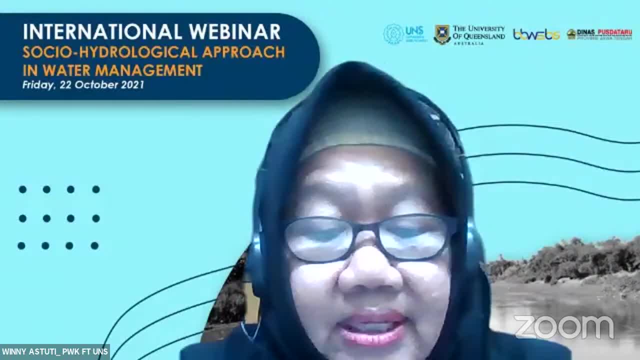 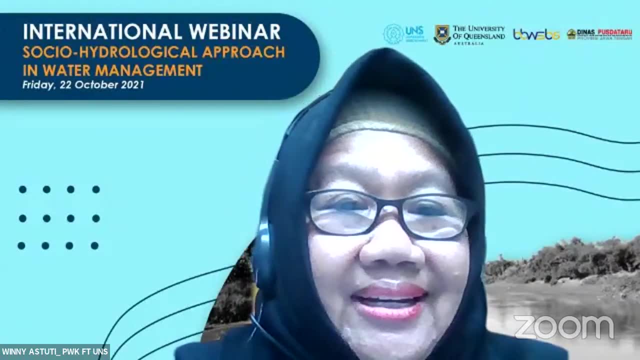 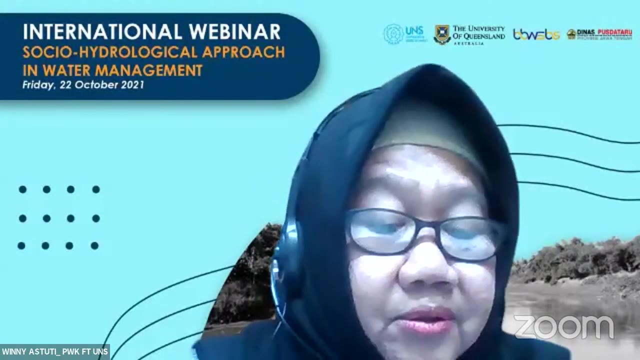 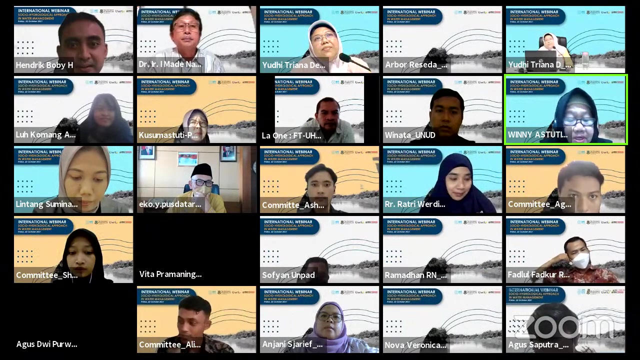 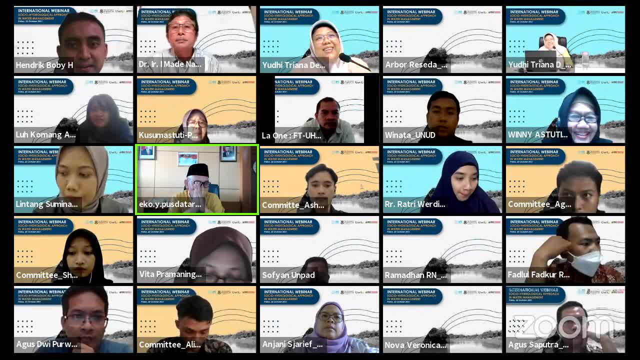 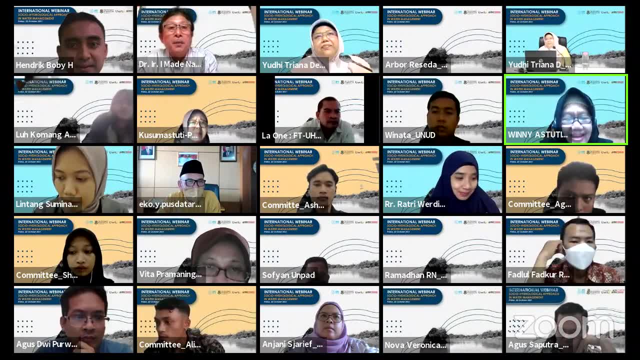 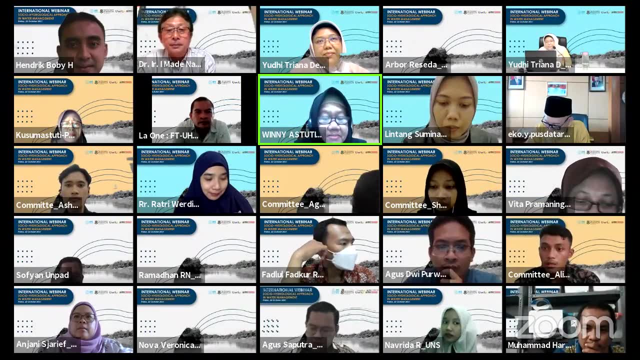 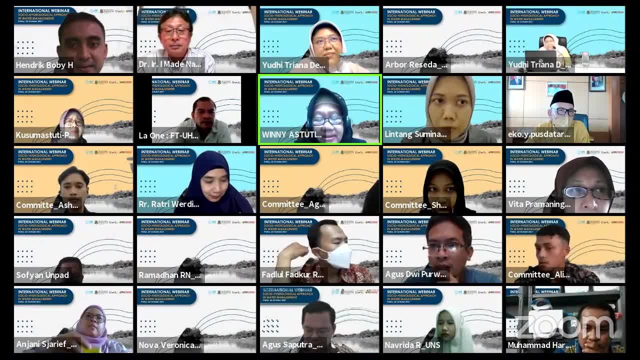 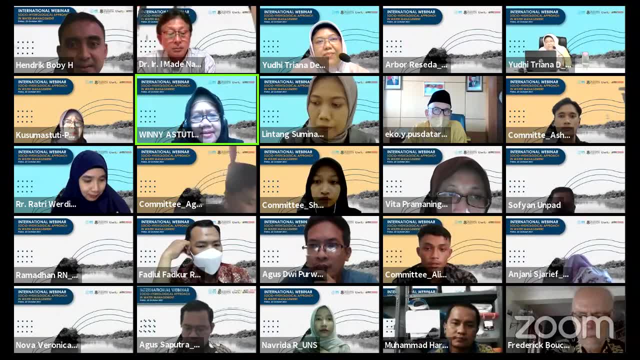 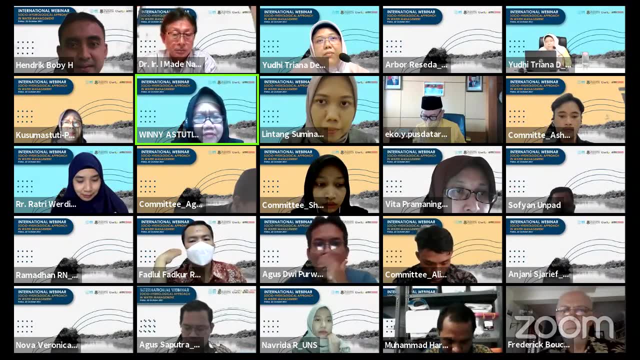 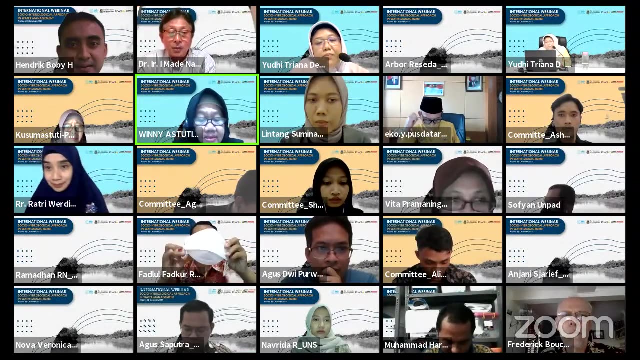 international webinar has been happening very well today and the second one, of course. i would like to express my great appreciations to all the keynote speakers. we would like to deliver the interesting and inspiring presentation in the topic of socio approach in water management, also for the team of the faculty. 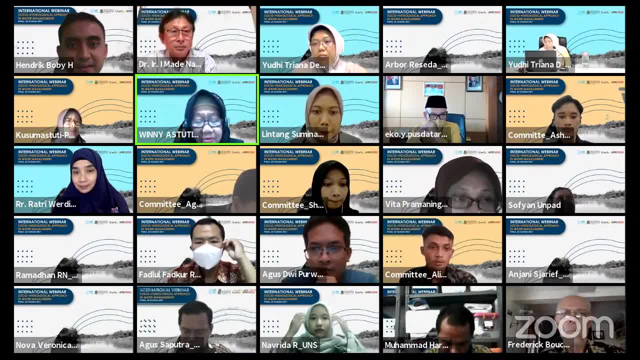 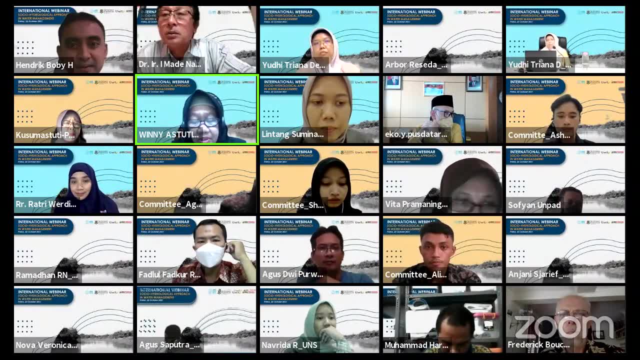 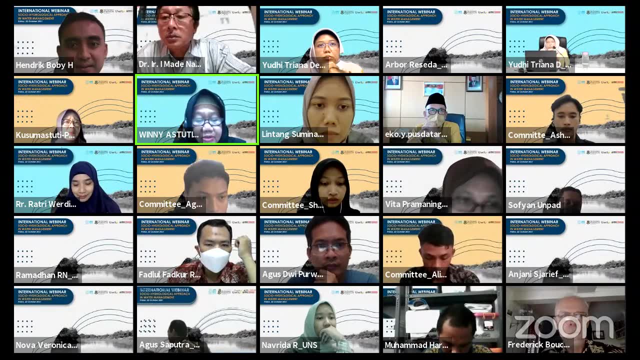 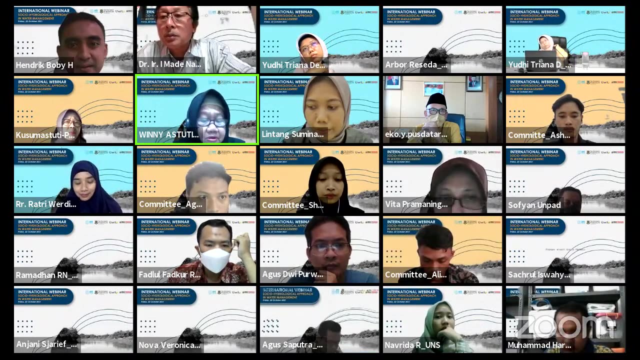 and all the audience. thank you for coming webinar. actually, the topic of socio-hydrological approach in water management is right now is very actual and also challenging, as the access to clean water is so potential becoming the basic issue of the sustainable development course. many, many people. 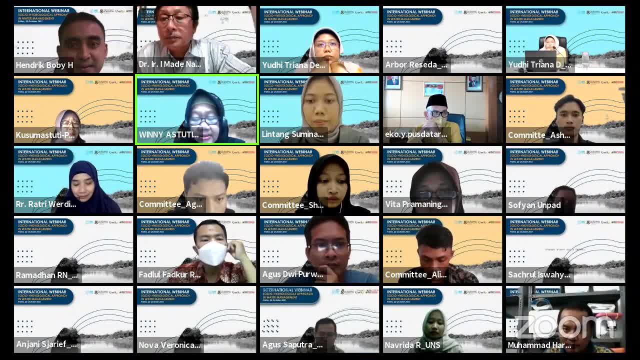 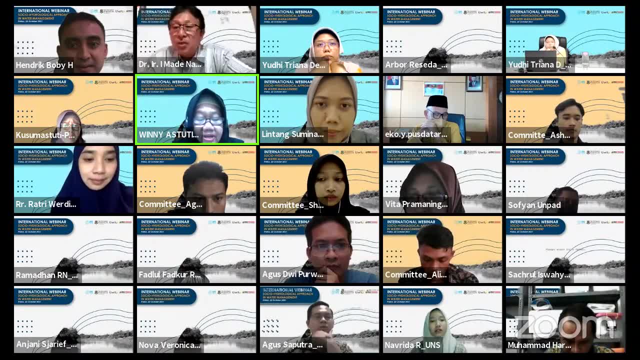 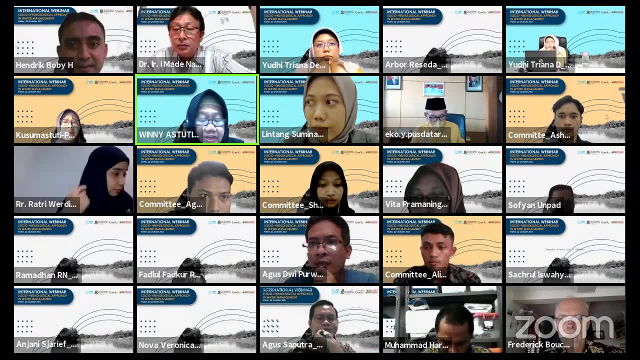 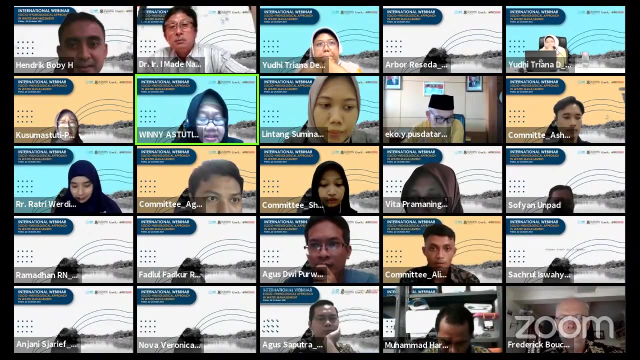 has been competing to get the water supply, so there are a lot of exploitation of groundwater and also lots of mafia has been the big issues and many more issues which trigger the conflict of the rest. so therefore, the open and regional planning program engineering faculty ons broadly present. 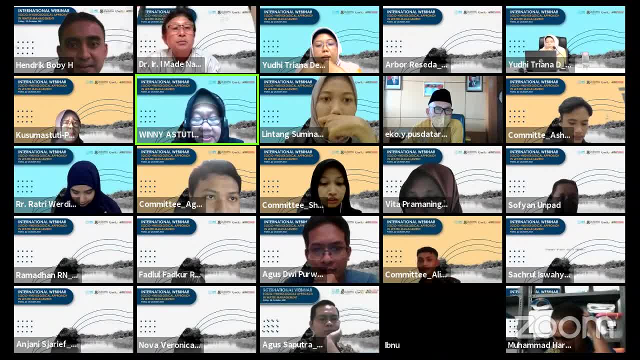 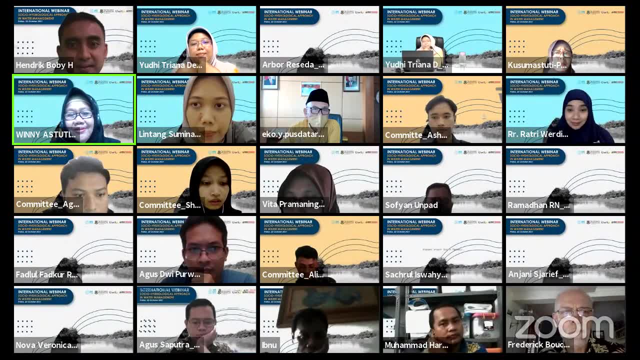 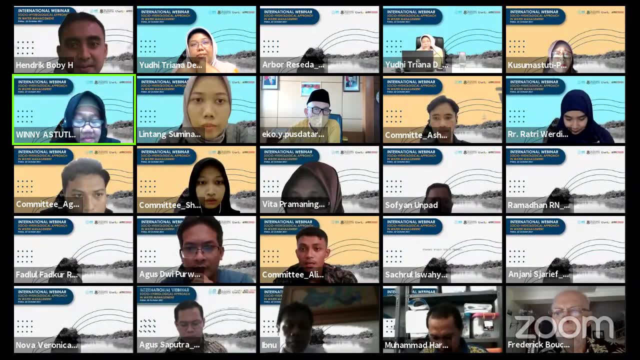 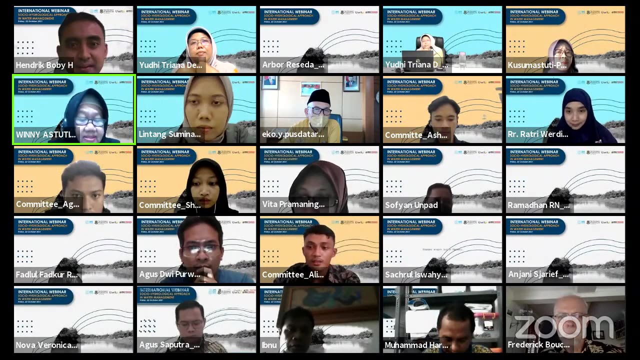 this webinar as we have some experts in water management- uh, here it is who: dr ratri, work in the gps, and also dr paramitra, uh paramita rahayu. they are the very expert in, and their water management. so we cannot hopefully the webinar and enrich knowledge about the social historical approach. 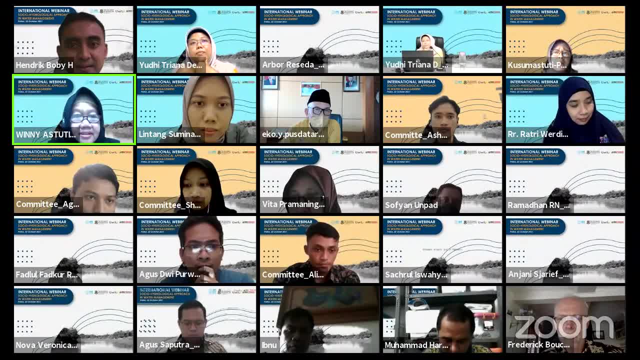 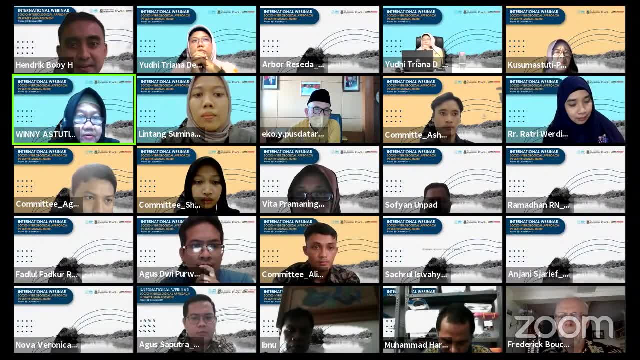 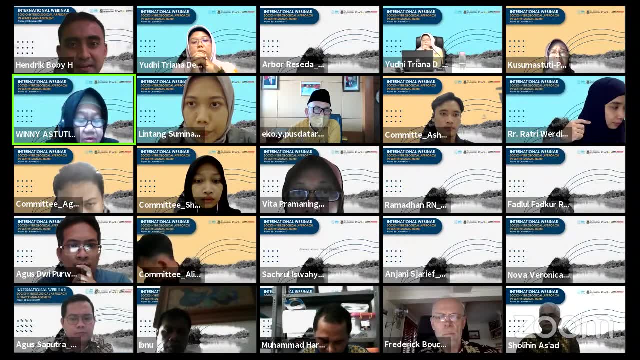 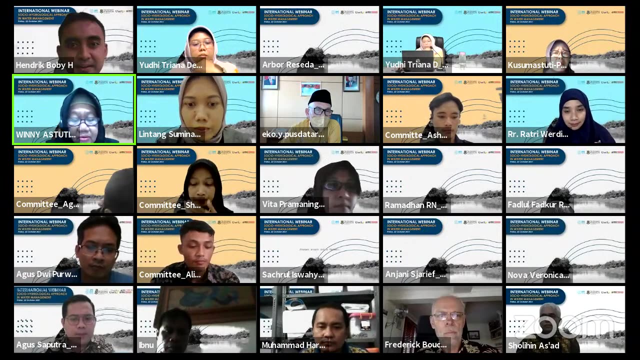 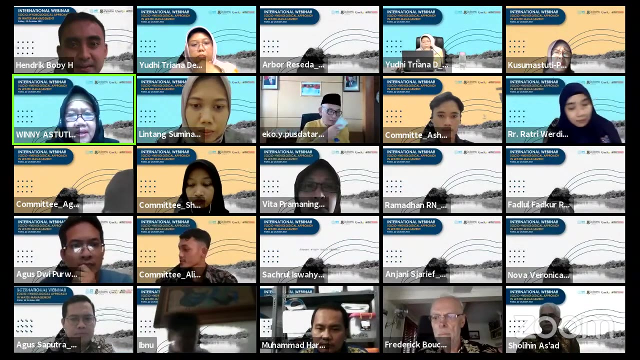 and also we can explore a approach and managing the interaction between physical and social system in water management, and also we can discuss the prospect and the test balance in socio-heterological approach to be implemented in Indonesian water management. so also, uh the big thanks to for the collaboration of all parties which is uh involved in this webinar. 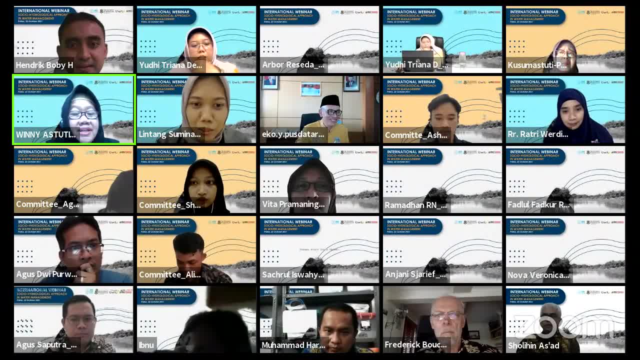 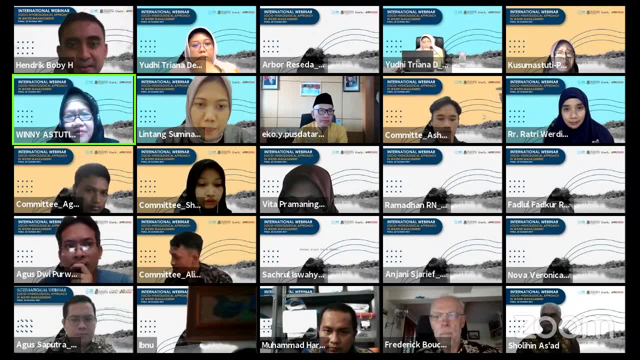 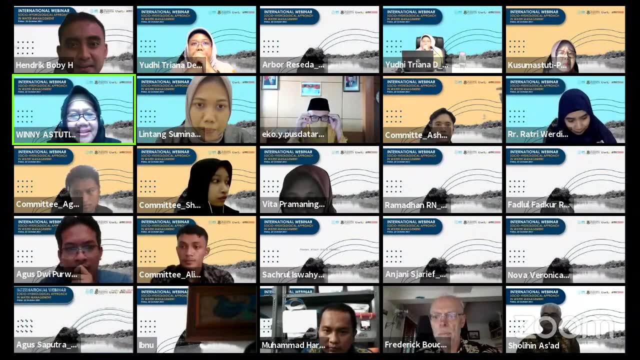 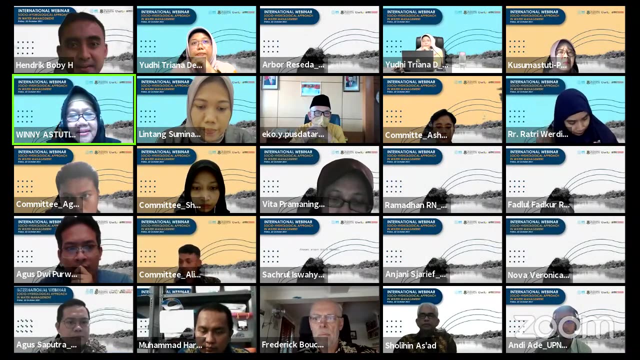 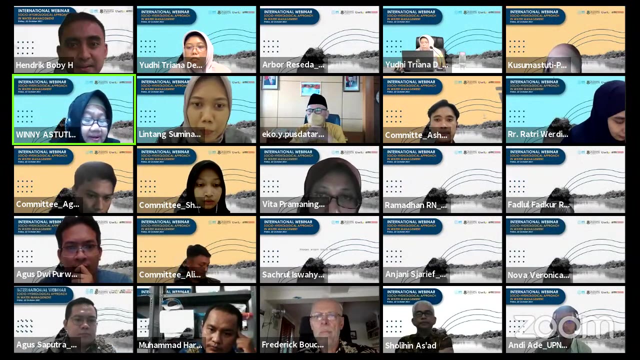 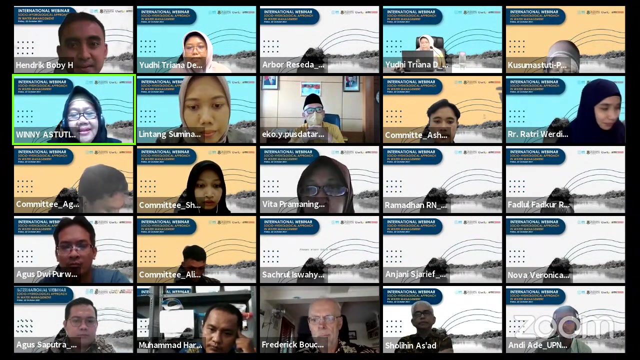 thank you very much for this collaboration. hopefully this will be another challenging collaboration in the future uh for the development of uh open energy planning program. things that's all uh enjoy to follow and be active in this interesting webinar until the end of uh this season. thank you very much. 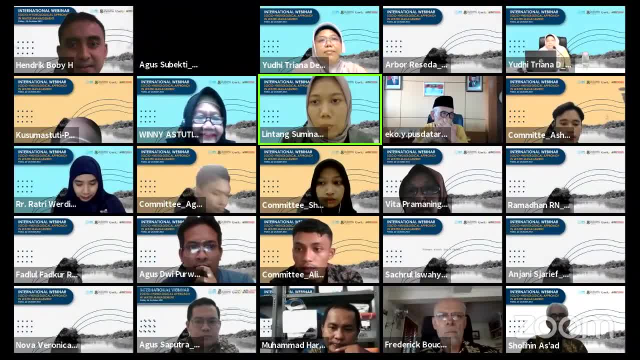 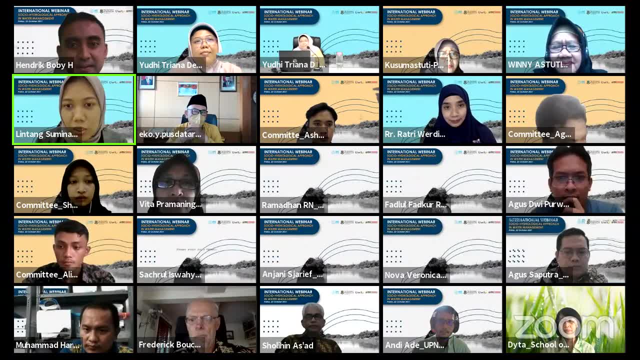 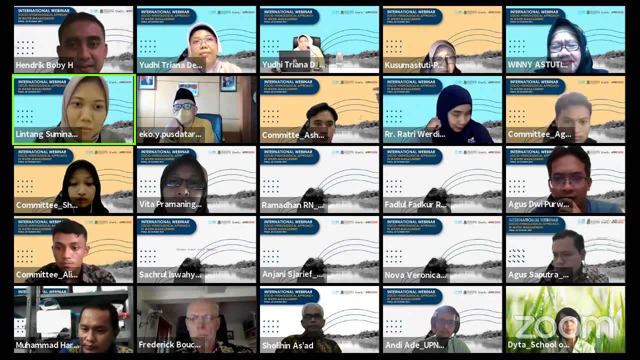 thank you very much, professor winnie astuti, for the opening remarks and, to kick off today's agenda, i would like to welcome the dean of faculty of engineering universitas, dr solihin asset, to deliver this speech and formally open this webinar program. so, uh, dr solihina said, the time is yours, okay, uh? 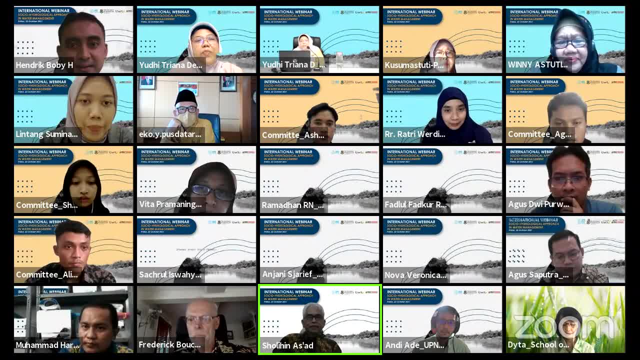 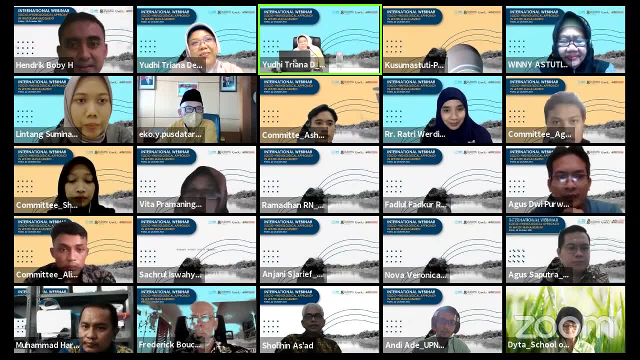 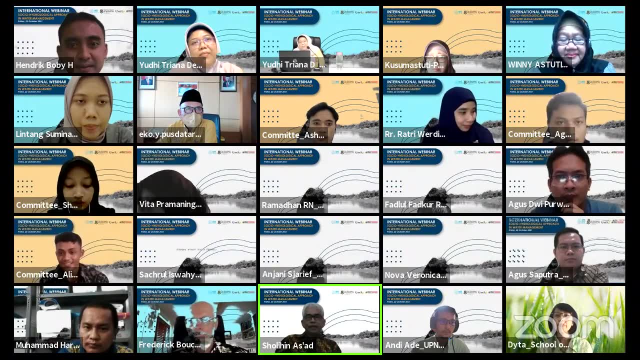 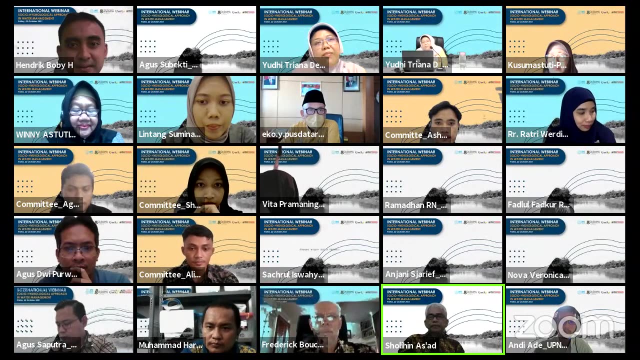 terima kasih. thank you very much. assalamu alaikum, good afternoon everyone. distinguished speakers: professor yong pin way from princeton university, australia. dr fredrick bob her from the uh uh from australia also. uh. dr agus rudianto uh. it will be represented by dr judy. 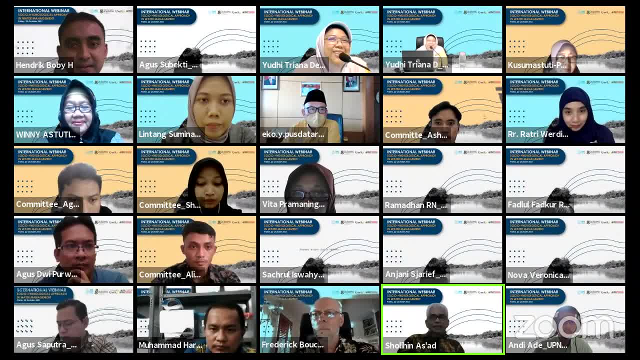 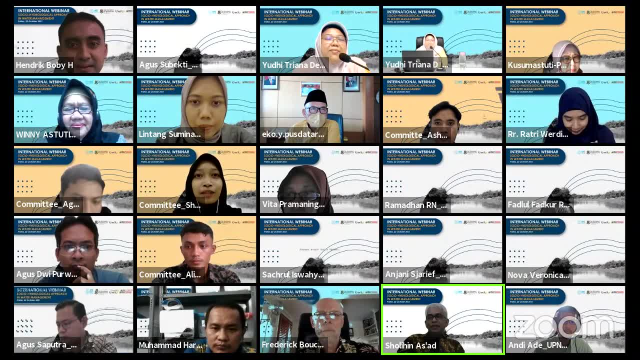 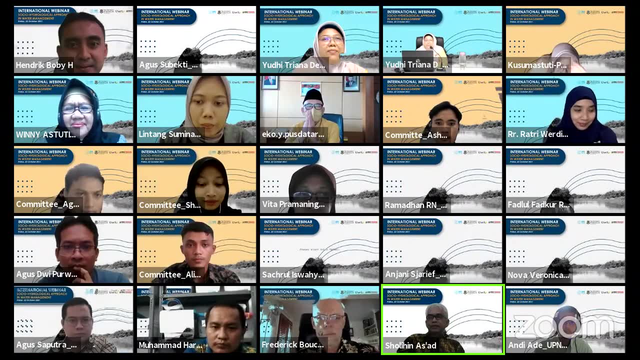 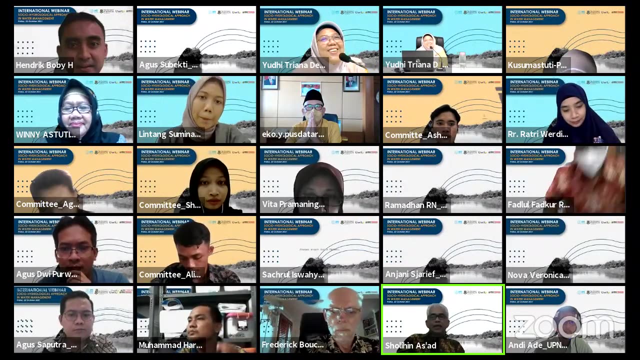 triana dewi uh so um dr atri wedding in ts mekalich from news um iku yung yanto uh uh from the uh usdataru yuh Dinas Pekerjaan Umum Sudantaru, Provinsi Jawa Tengah, Indonesia. 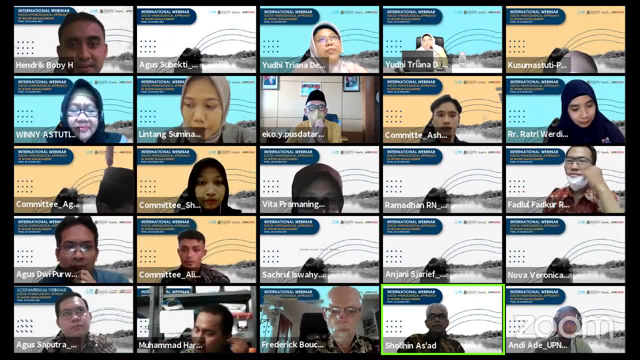 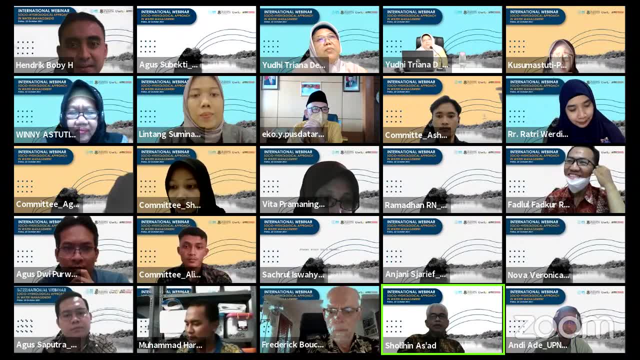 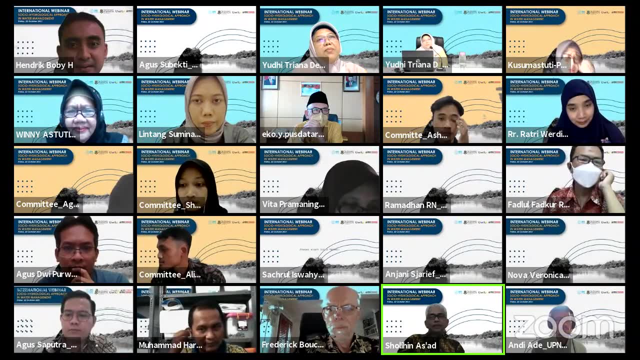 The head of the program of Urban and Regional Planning, Ibu Prof Winnie Astuti, and also the professor, the lecturer, the students and all participants in our webinar this afternoon. My name is Solihin Asad, the Dean of Faculty of Engineering Universitas Sebelas Maret, Indonesia. 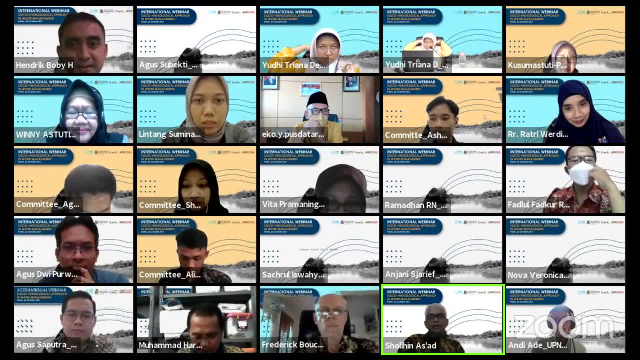 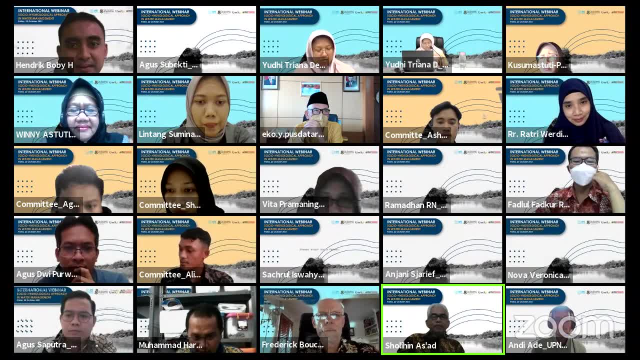 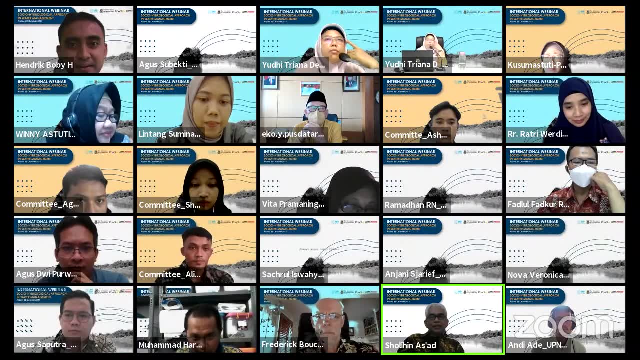 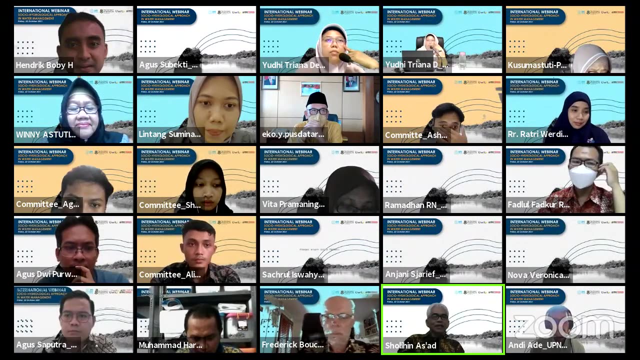 I am so delighted to welcome you all to this excellent webinar- international webinar with the theme of the socio-hydrological approach in water management. Thank you for joining. This is also a new terminology for me. Yesterday I met Dr Rathri. What is socio-hydrological? 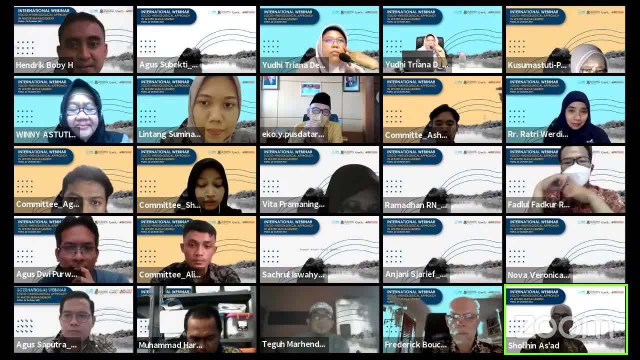 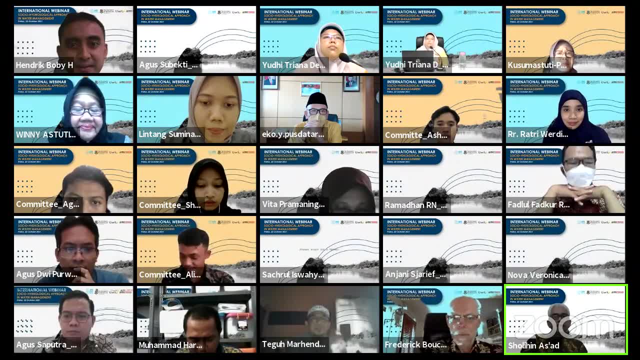 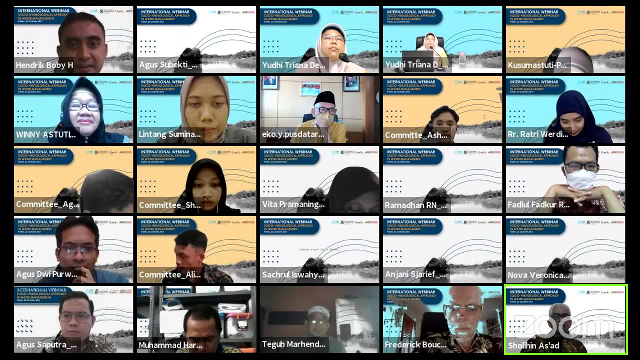 So she said, OK, tomorrow you will understand What is socio-hydrological. Ladies and gentlemen, water is not solely a technical matter, but it can be seen in various perspectives. It can be technical, economics, human, social, cultural politics and many more. 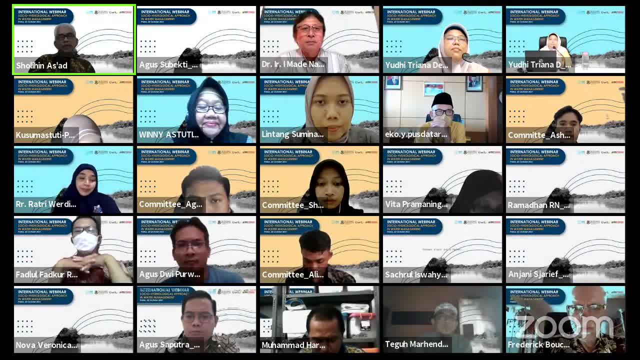 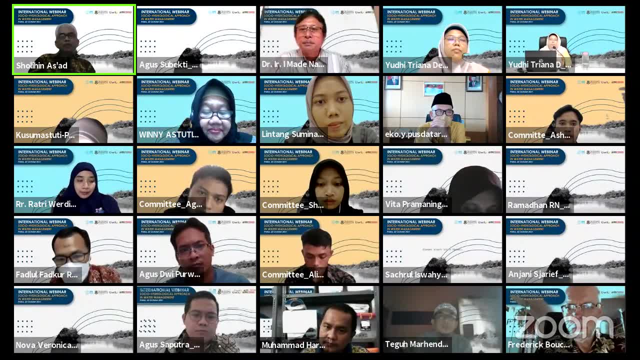 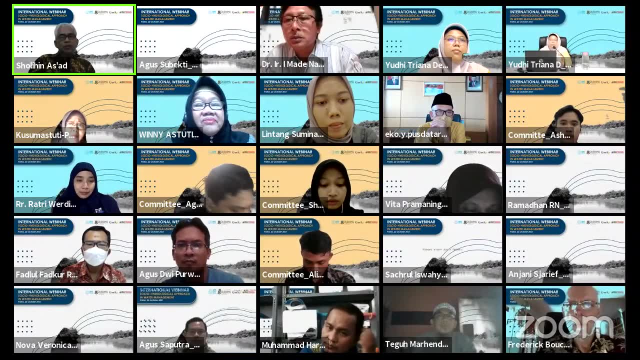 So, as we know, water is our basic needs as a human being, Water is a basic need for all of us in our planet. No one can live without water. So it's our task and our obligation to manage and to preserve the water for our living. 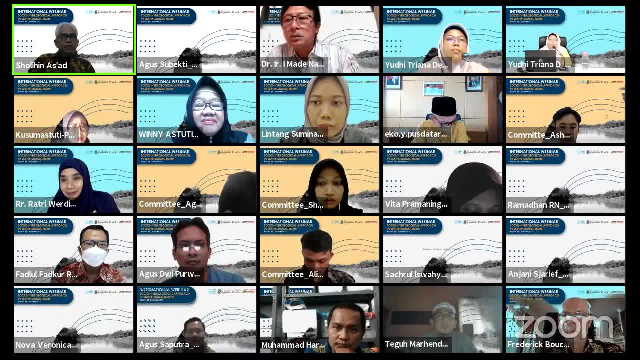 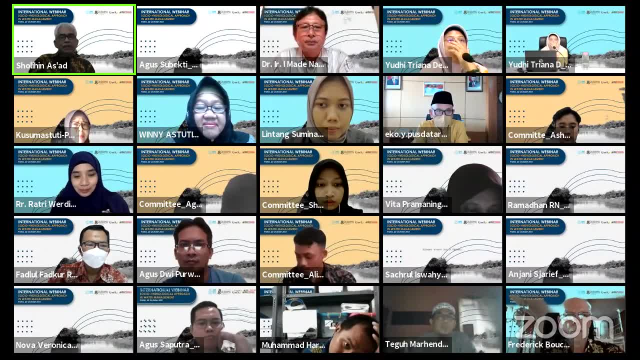 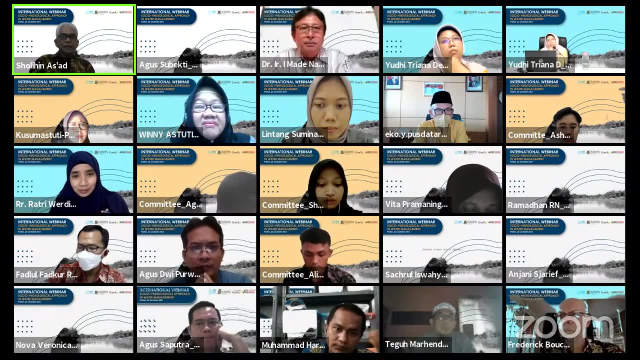 for our planet, for our community, for our family and for ourselves. Ladies and gentlemen, for our sustainable living, there are no other choices that we have to understand the character of the water surround us, understand our environment, understand the character of human beings. 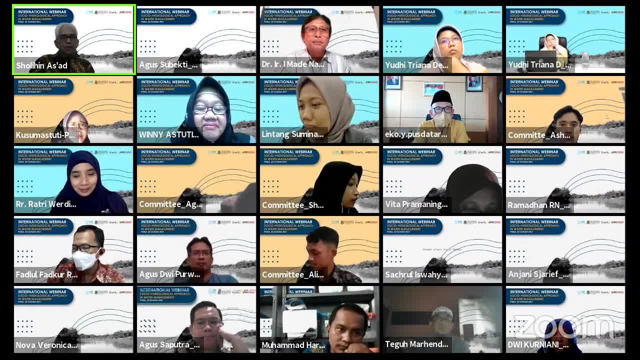 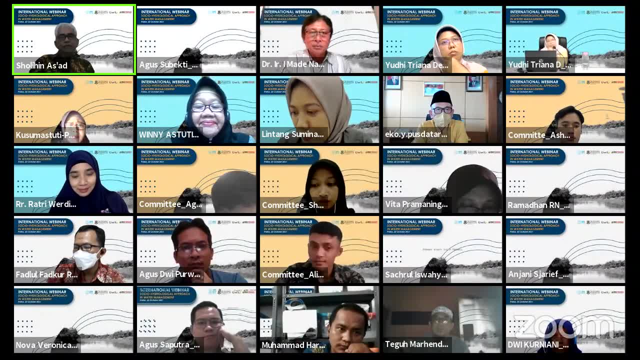 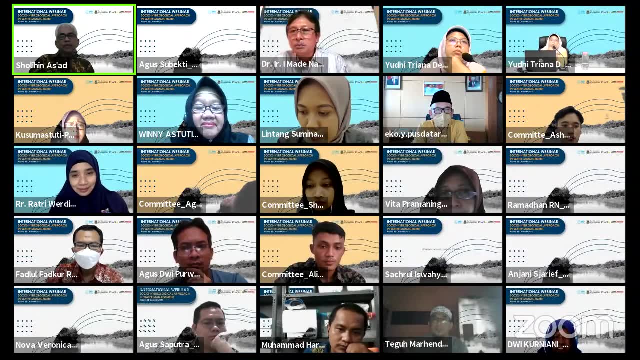 or the community who consumes the water. Here in Java Island, for example, located where our campus, Universitas Bras Maret is located, it's about in one island of Java- there's about 140, even 150 million people are living. 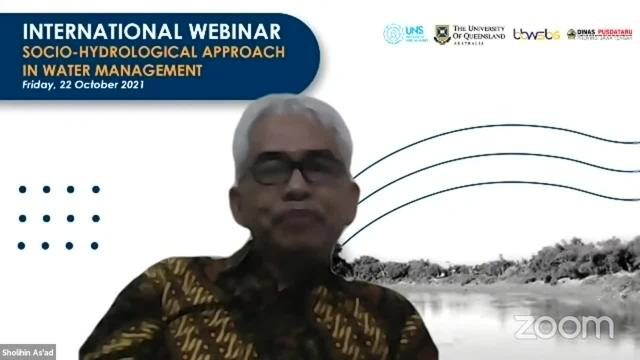 And just not far from our campus, our campus in Universitas Bras Maret, there is the Bengawan-Solo River. It's a very long river. in Java Island It's a very important river with 600 kilometers long And, as long as I know, at least about 20 or 40 million people have a close connection. 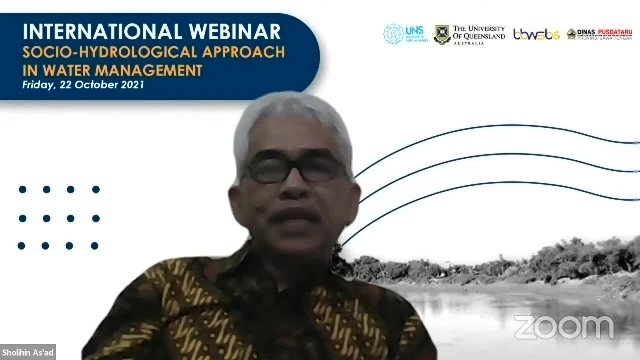 with this river, Or I would say they depend on this river. That's why we have to manage well this river, the Bengawan-Solo. Bengawan-Solo is one of our big assets And we have to manage it, not to mention other rivers. 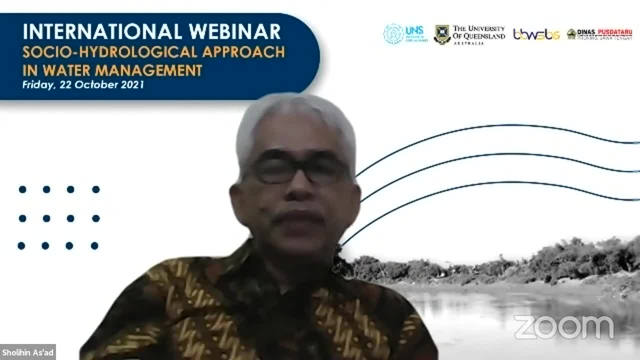 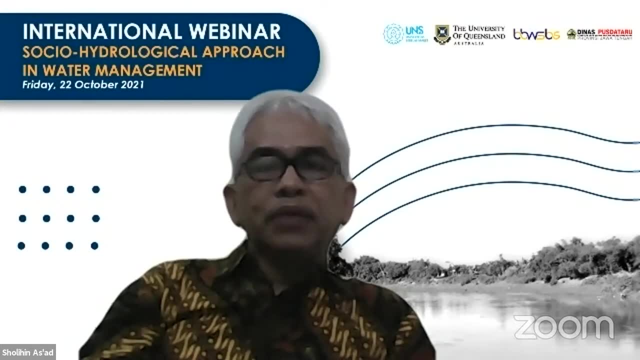 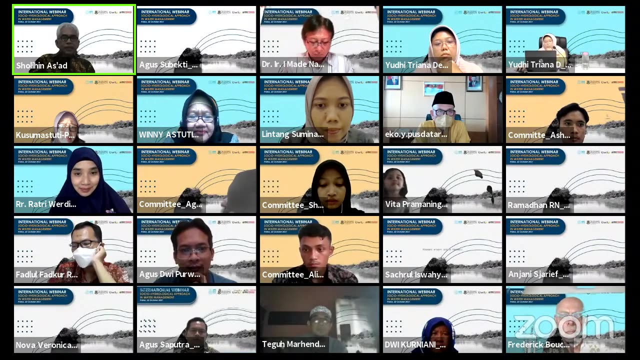 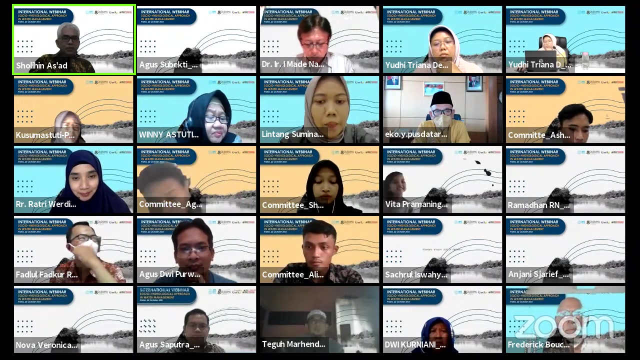 like some rivers in West Java, for example. So we have to preserve our water, Our water resources and our water assets. Ladies and gentlemen, as I mentioned that we have to manage our water resources, the water distribution also, water allocation, water supply. 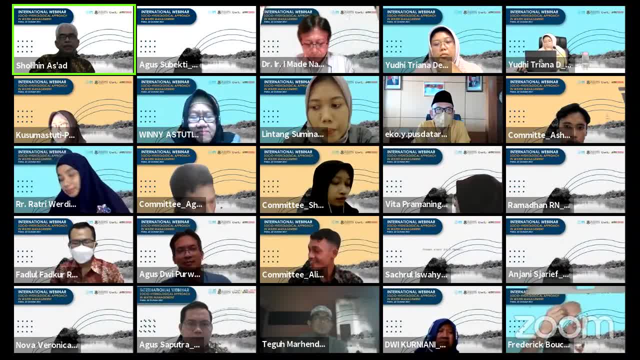 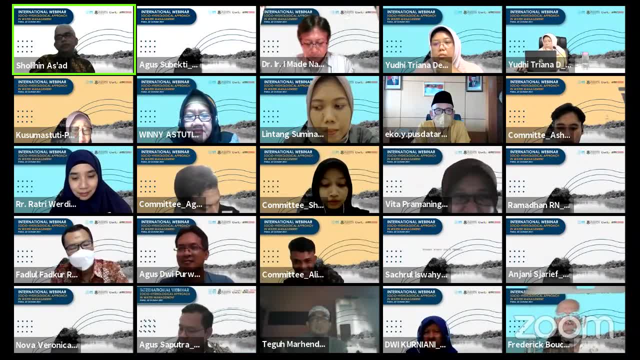 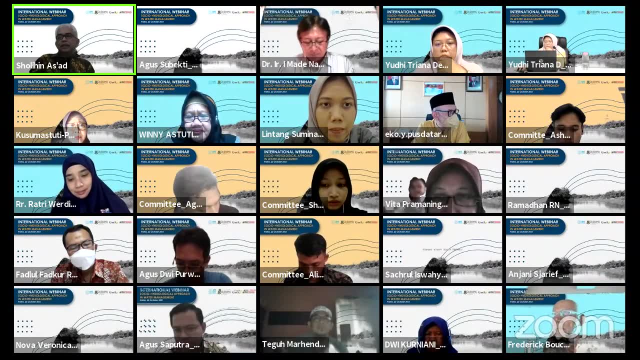 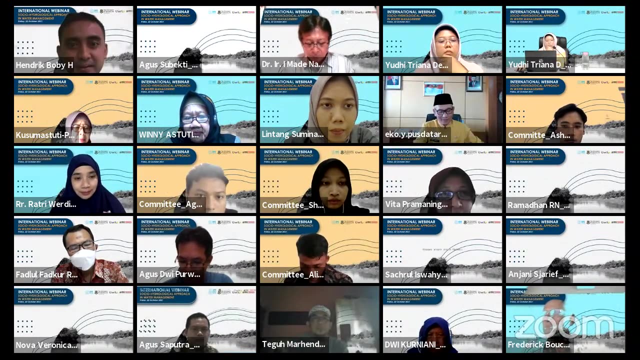 And this must be organized well, must be organized wisely, precisely, scientifically, Otherwise it will be a catastrophe for us. Ladies and gentlemen, therefore, this international business is very important. The discussion among us, the stakeholders from different backgrounds, as we're doing now, is very important. 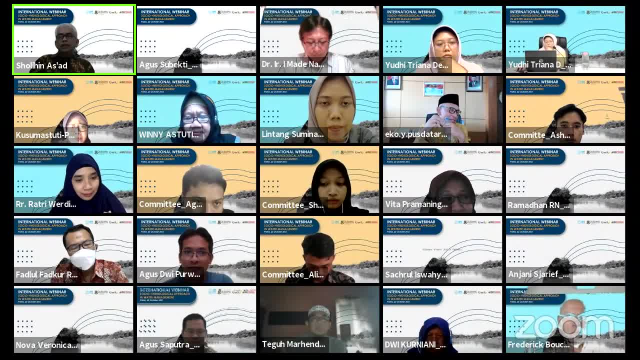 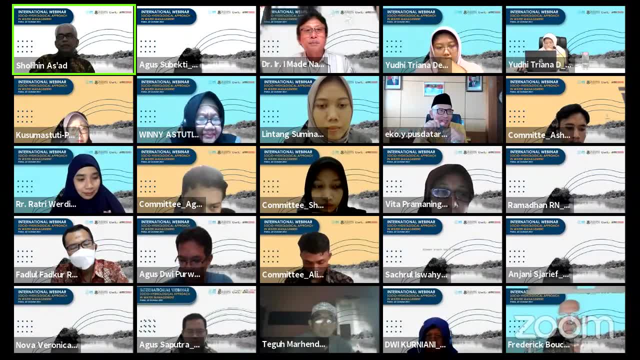 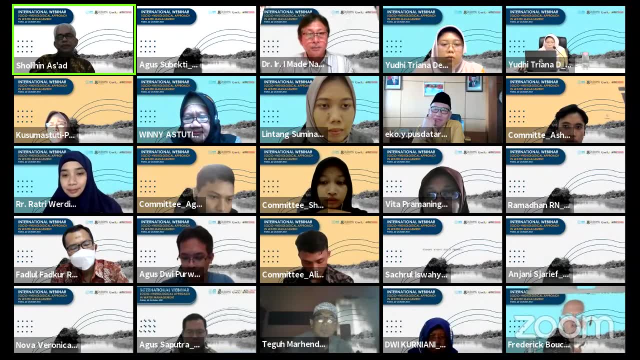 Coordination among us- the stakeholder, the regulator, the users- is very critical so that we may govern and manage our water effectively. Therefore, ladies and gentlemen, for our webinar today, I would like to extend my sincere gratitude to all the speakers. 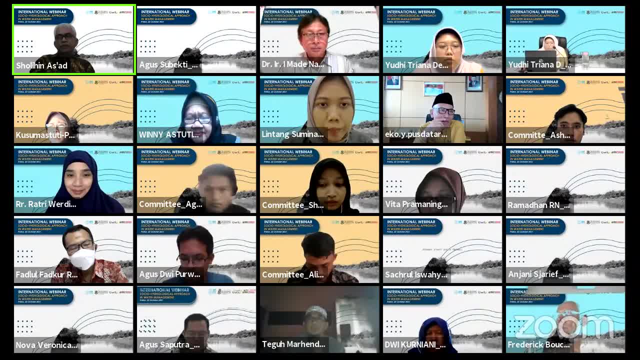 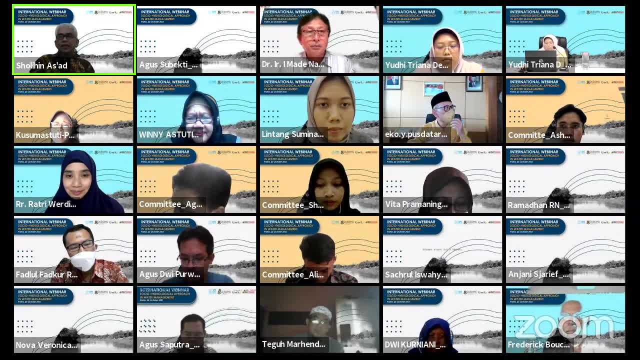 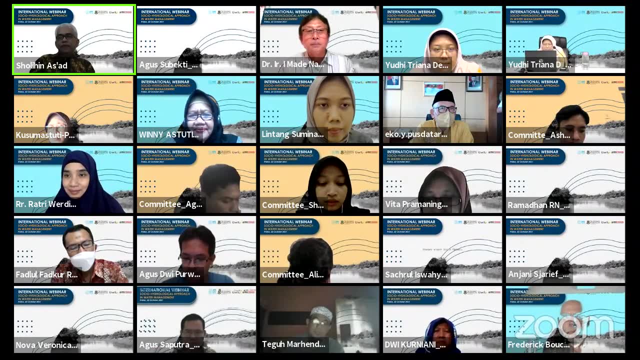 Thank you very much for Dr Professor Yong Ping Wei, far away from Australia. She is deputy of head of School of Earth and Environment Environmental Science University of Queensland, Australia. The second is Dr Frederick Bokhair. He is an international consultant for river basin management. 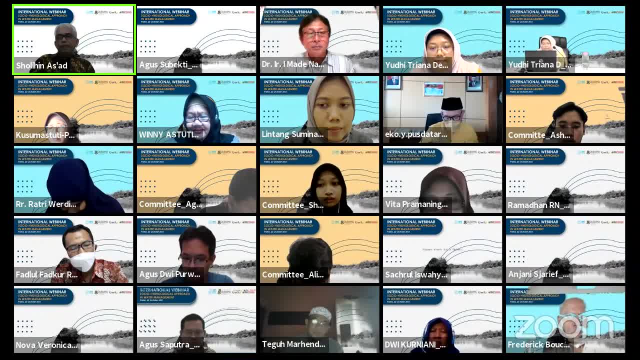 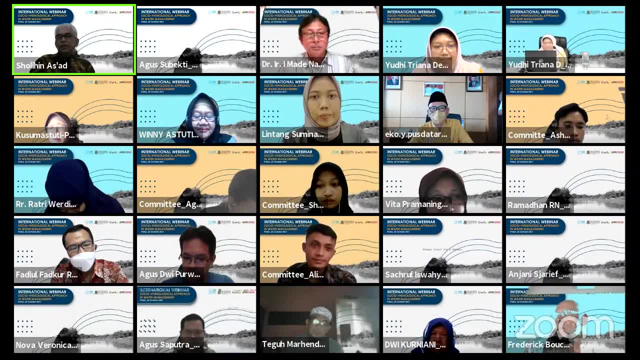 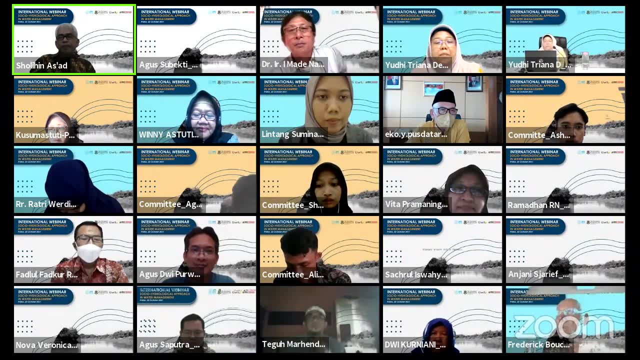 And the third, Bapak Dr Ingenieur Agus Rudianto. Right now he is represented by Dr Yudi Triana Dewi. Agus is the head of the Wangan Solo River, the authority in Indonesia. And the fourth, Bapak Eko Yunianto. 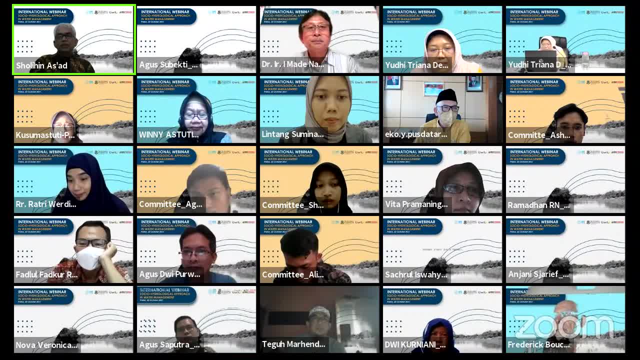 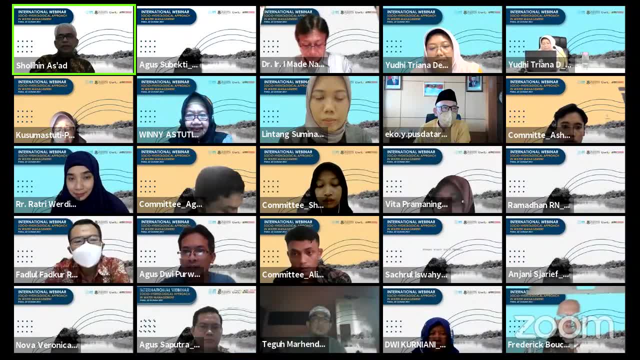 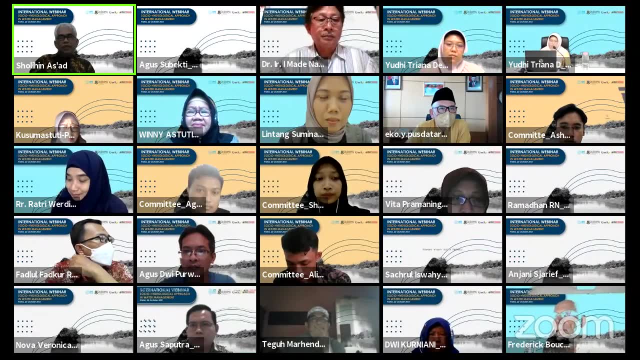 head of Public Works, Water Resources and Spatial Planning Department, Dinas Pusdataru Provincial Centre in Indonesia, Ibu Dr Ratri Witaningsi. she is a lecturer and researcher in urban and regional planning in Klas 11 Maret Indonesia. 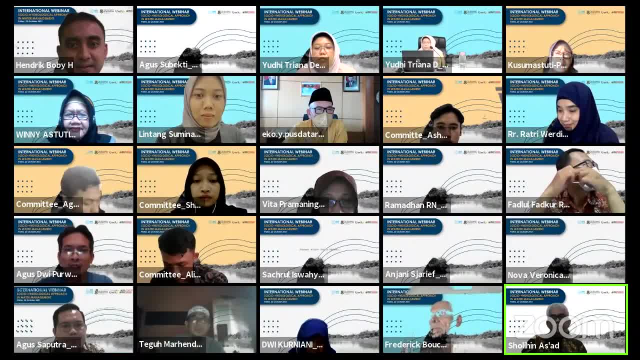 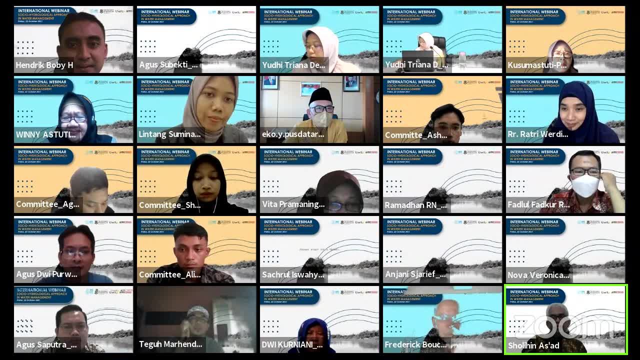 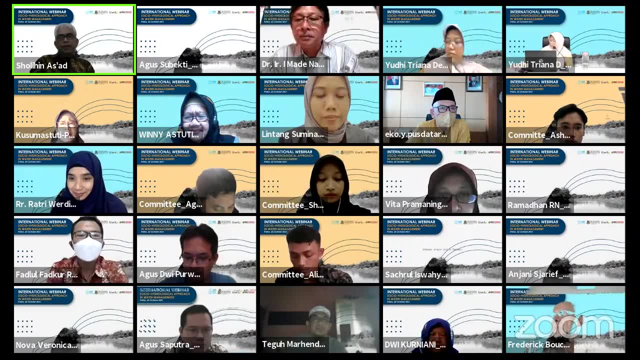 And also for our moderator. thank you very much, Ibu Dr Paramita Rahayu and all the committees led by Ibu Lintang Suminar. Thank you for your work hard for making this international webinar possible. Ladies and gentlemen, 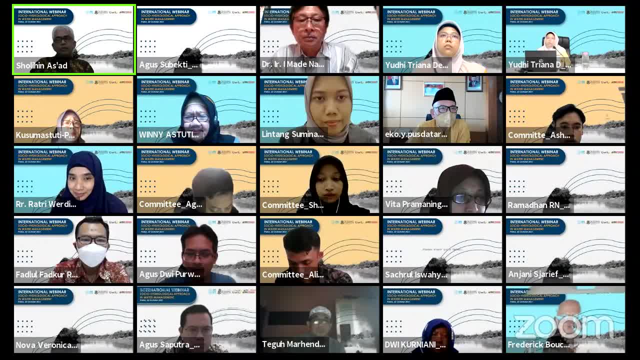 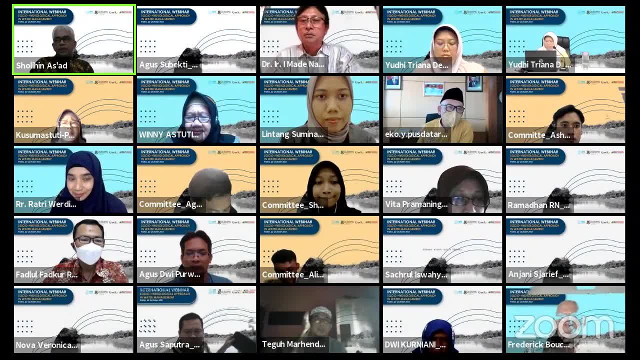 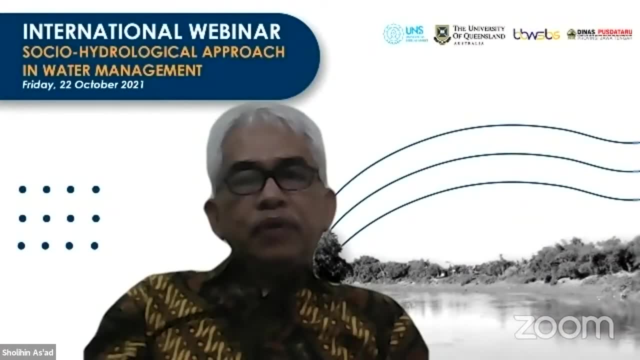 from this webinar, we expect so many excellent and genuine ideas, and even provocative ideas, And also they can be from a speaker and also from participants. We are looking forward to having you in our next works, for our collaboration to preserve our water and to have a good management of our water. 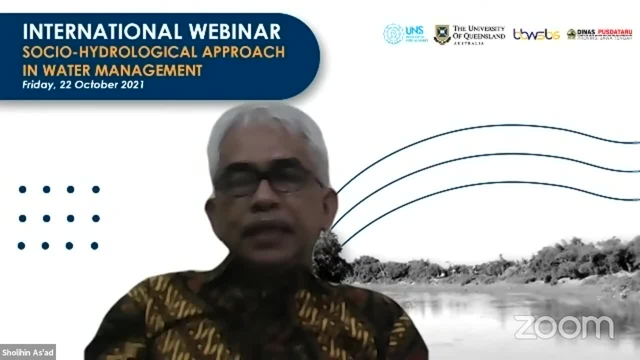 Last but not least, with saying Bismillahirrahmanirrahim, I declare that this international webinar is officially open. I thank you very much for joining and I hope you have a great webinar, and I wish you experience and excellence and a fruitful discussion. 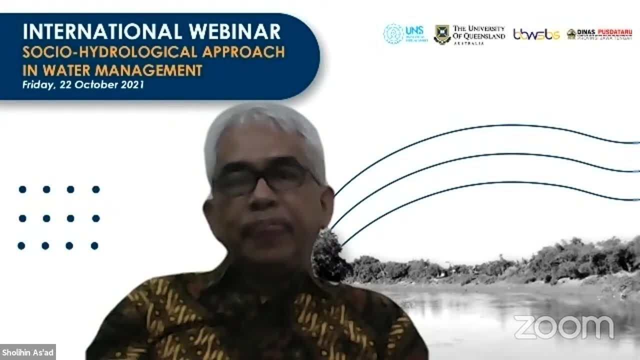 Thank you very much. Terima kasih, Assalamualaikum. warahmatullahi wabarakatuh, Waalaikumsalam, warahmatullahi wabarakatuh. Waalaikumsalam, warahmatullahi wabarakatuh. 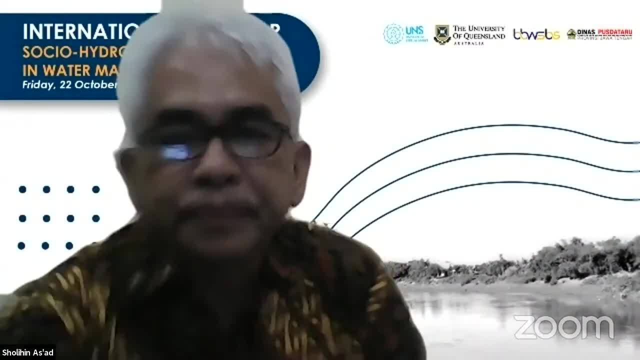 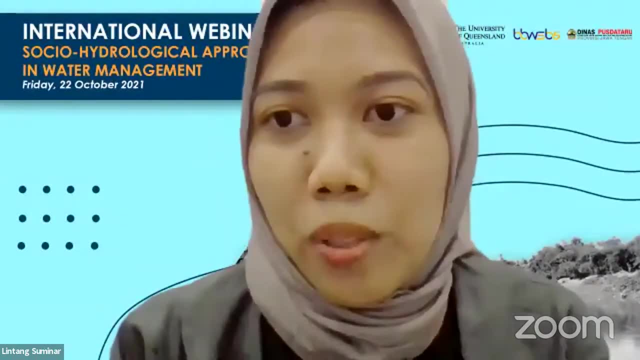 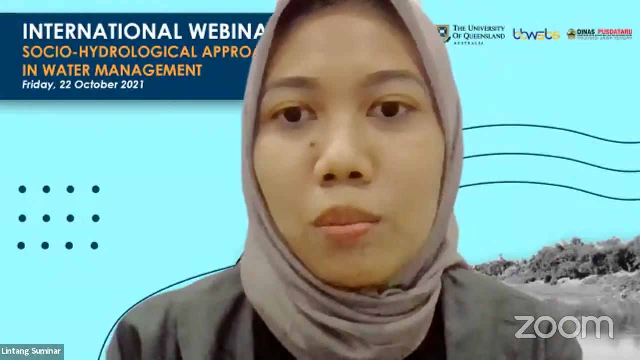 Over to you, Ibu Lintang. Thank you very much, Dr Soleh Nasaf, for the opening speech and also opening this webinar. Ladies and gentlemen, the next agenda is the most weighted, that is, the presentation session from the five amazing speakers. 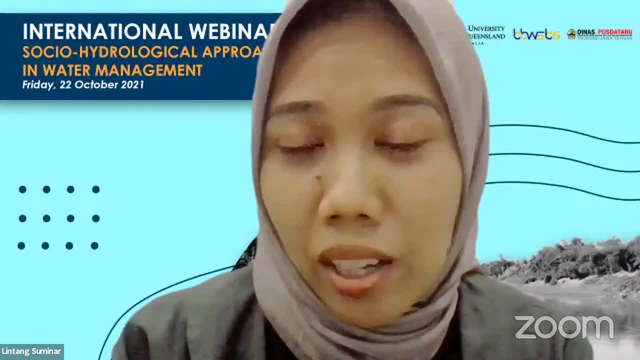 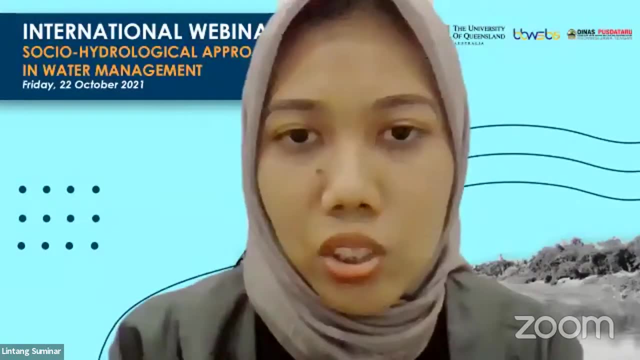 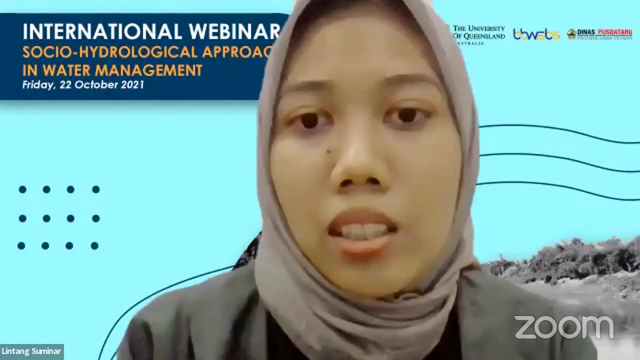 This session will be moderated by Dr Paramita Rahayu, who are an associate professor and the head of Regional Planning Laboratory in Urban and Regional Planning Program Faculty of Engineering Universitas Sebelas Maret. Dr Paramita completed her undergraduate degree from Institut Teknologi Bandung. 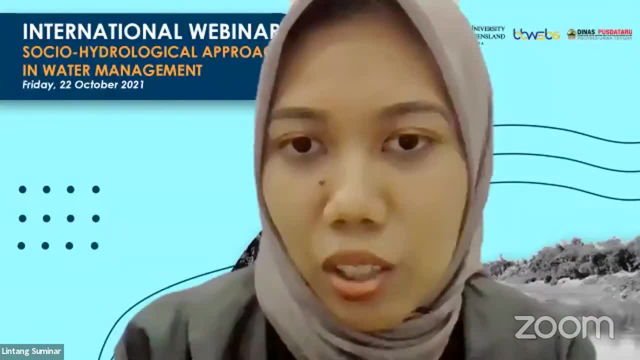 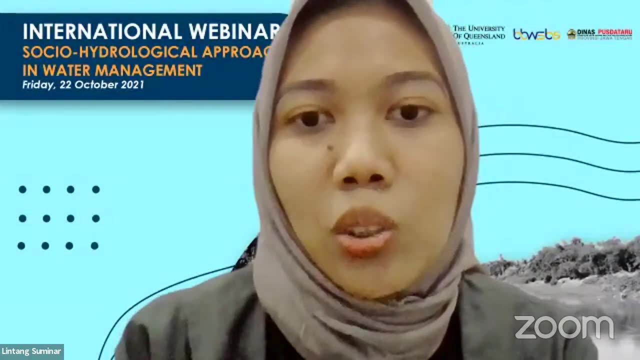 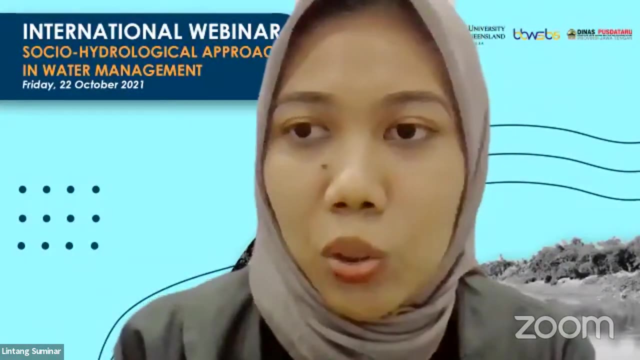 the master degree from the same university and also from the University of Groningen and the doctoral degree from the University of Groningen in 2016.. She is also active in publishing and conducting research, by which her focus are mainly on urban development, governance and also urbanization. 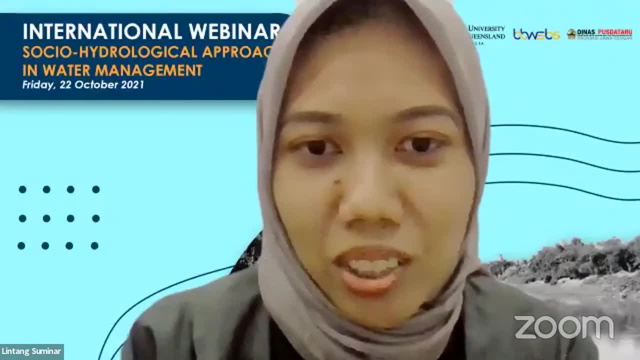 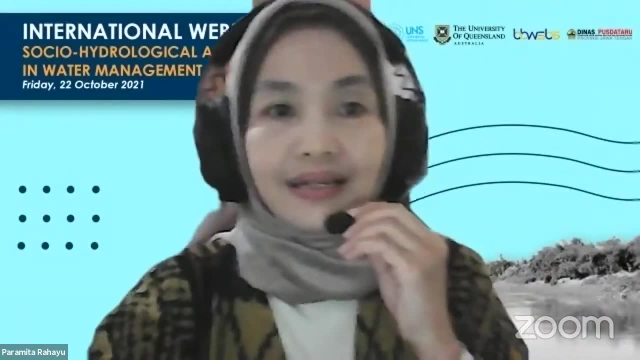 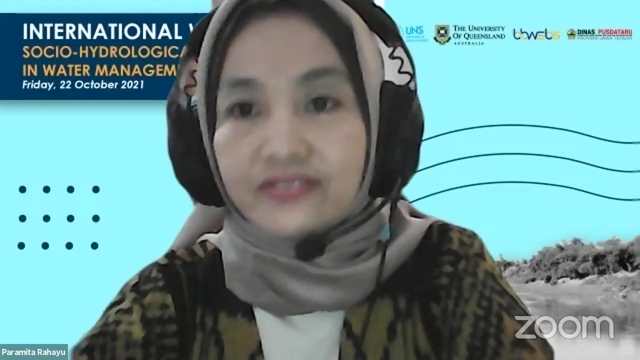 So, Dr Paramita, the time is yours to moderate this session. Thank you very much, Ibu Lintang. I feel privileged to extend my warm welcome to all our audience and also our five distinguished speakers, Professor Yongping Wei, Dr Frederick Bowkert. 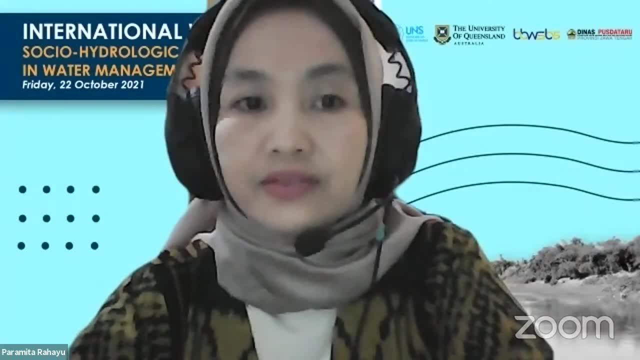 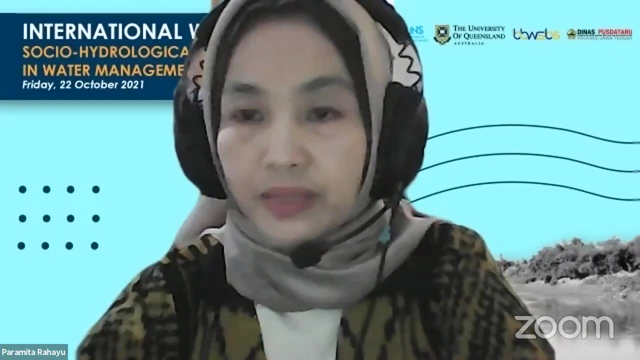 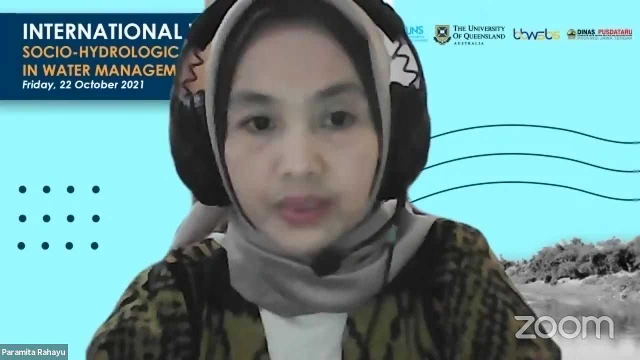 Insenior Eko Yunianto, Dr Yudi Triana Dewi and also Dr Rathri Werdinintas. Thank you for attending today's webinar Socio-Hydrological Approach in Water Management, And our first distinguished speaker is Professor Yongping Wei. 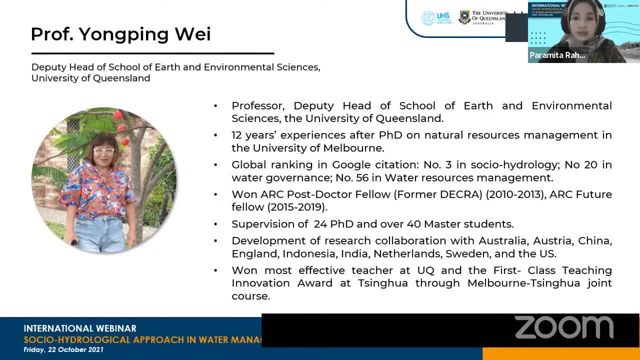 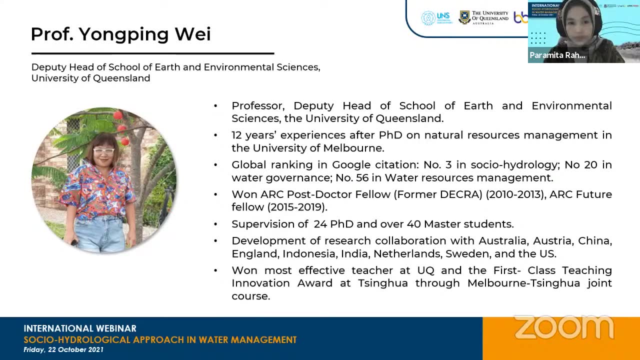 She is currently head of deputy of School of Earth and Environment the University of Queensland. She has 12 years experiences after PhD on natural resources management in the University of Melbourne. For global ranking in Google Citation, she is the third in socio-hydrology. 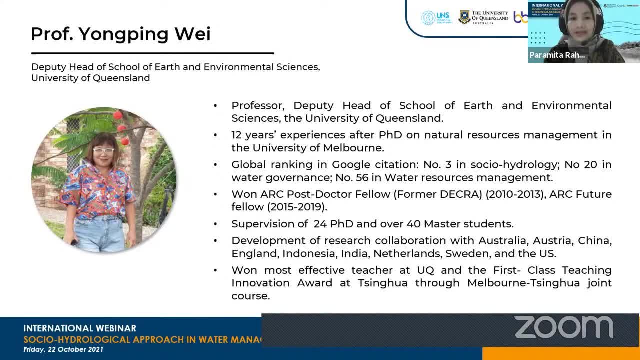 the second in water governance and the 56th in water resources management. So she also won ARC, both doctor fellow, ARC future fellow, and she supervises 24 PhD and over 40 master students. She develops research collaboration with Austria, China. 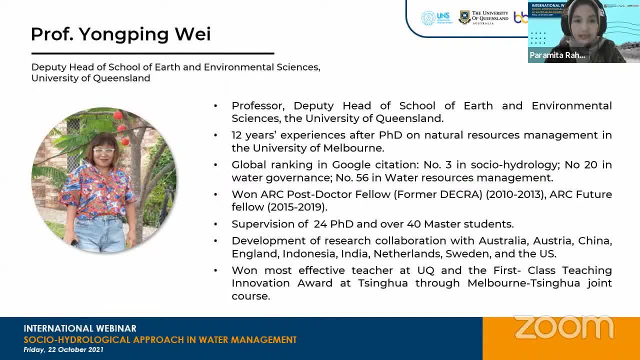 United Kingdom, Indonesia, India, the Netherlands, Sweden and also the United States. Prof Yongping Wei also won most effective teacher at University of Queensland and the first class teaching innovation award at SINGHUA through Melbourne SINGHUA joint course. 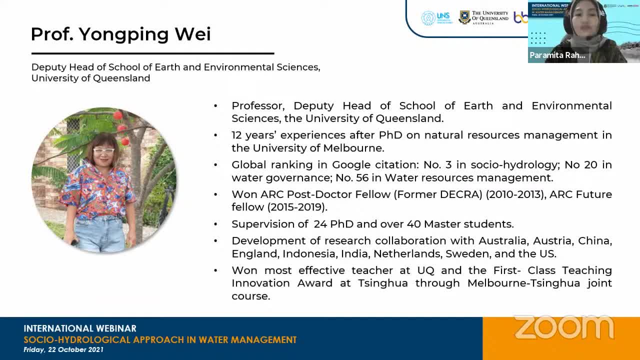 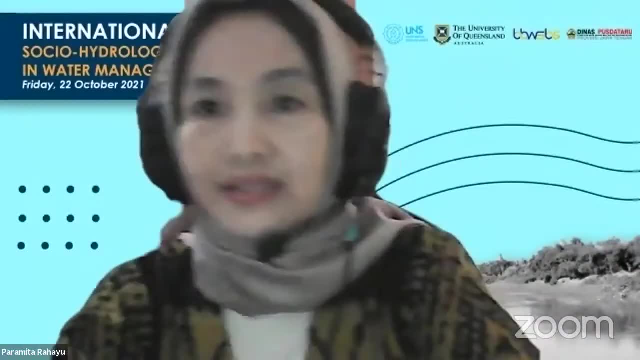 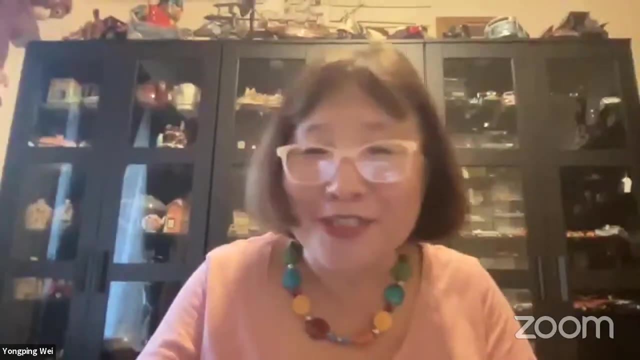 That's an amazing curriculum feature And, without further ado, please welcome Prof Yongping Wei. She will share her expertise in social hydrological approach in water management. Welcome, Prof Yongping Wei, The time is yours. Okay, thank you very much. 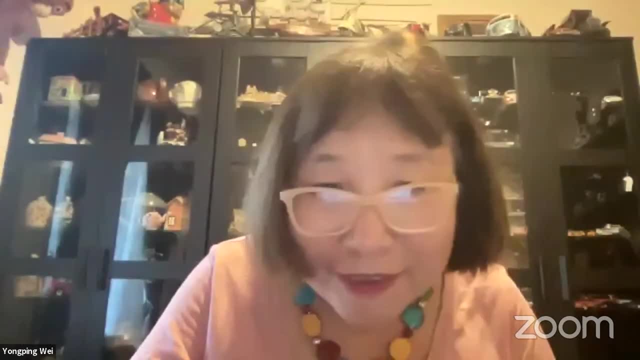 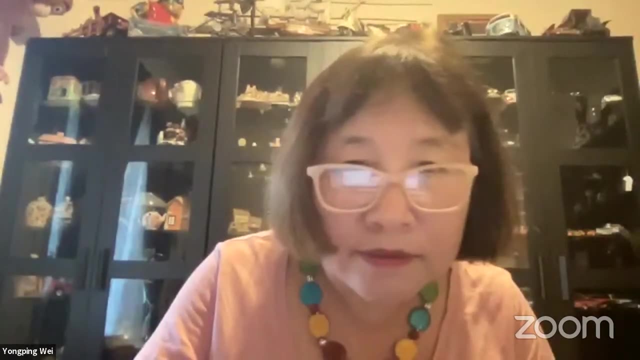 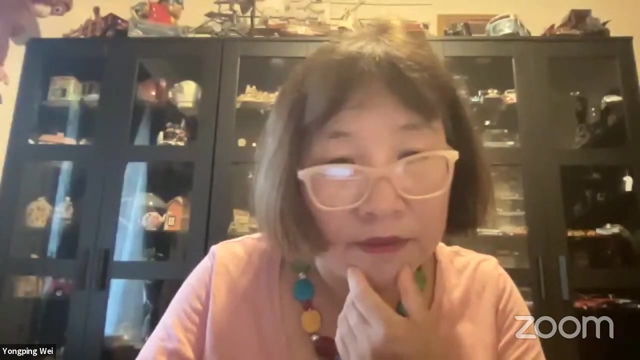 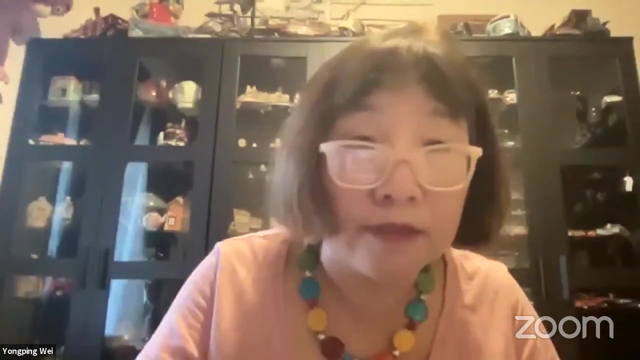 Let me find my slides first, then we can talk. Where's my slides? Sorry, Sorry, I couldn't find my slides. Sorry, I found my slides at the desk at the top, but I couldn't find it there, Sorry. 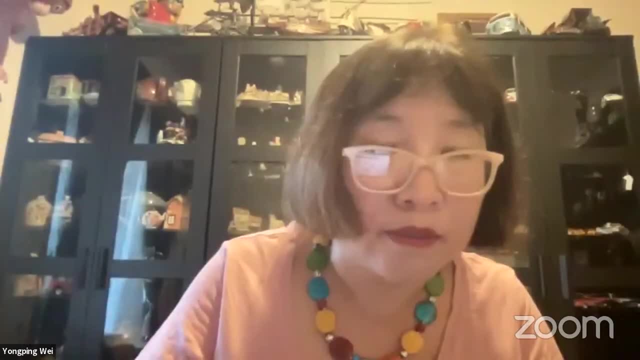 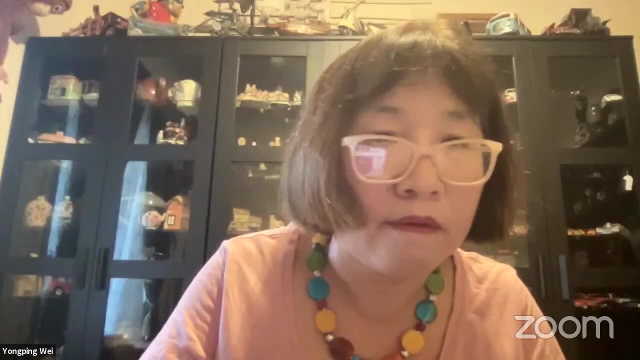 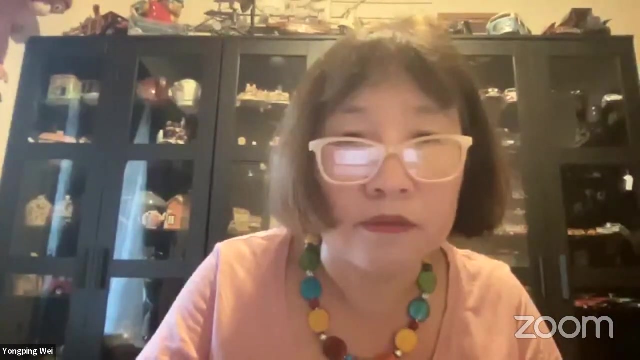 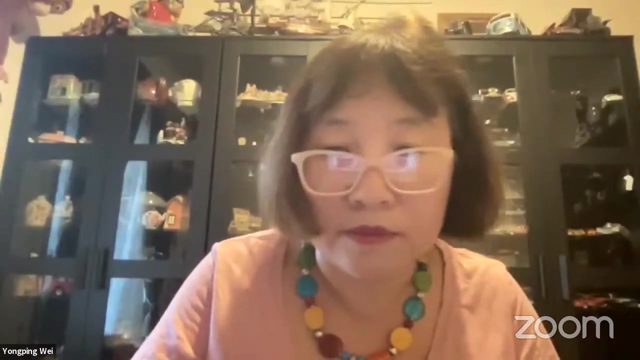 Okay, I'll try to find it. Where are they Here? they are Well great. Thank you so much, Prof Yongping Wei, and thank you so much, Dr Seng. Thank you, So what is the most effective? Michigan? 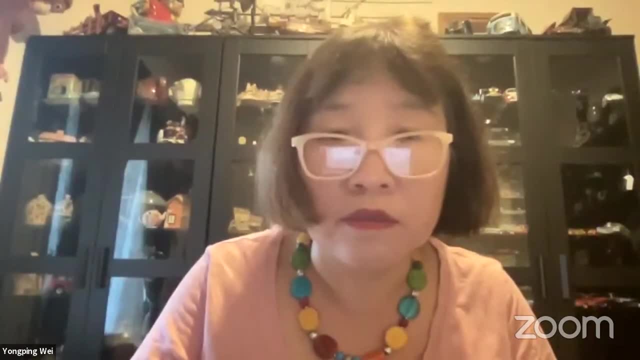 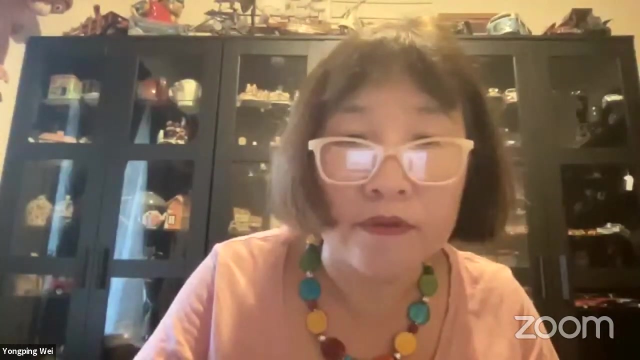 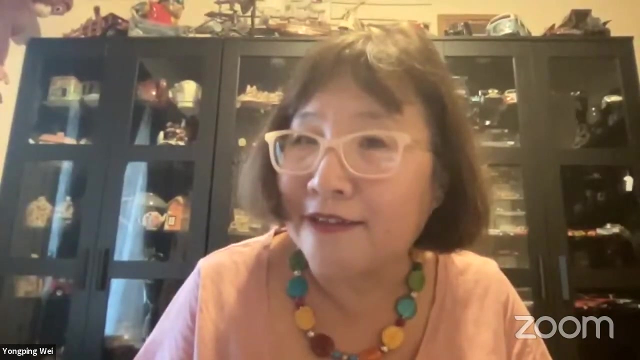 Dr Seng's research. Dr Seng is a professor of chemistry at the University of Queensland. She specializes in biochemistry and digital science. Sorry, I just changed my computer today. Farid, can you talk first, then I talk second, then I fix my computer. 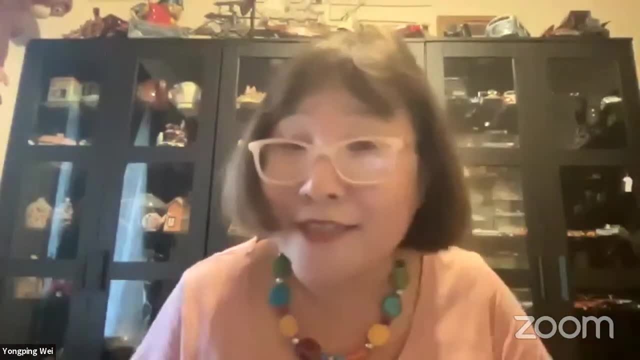 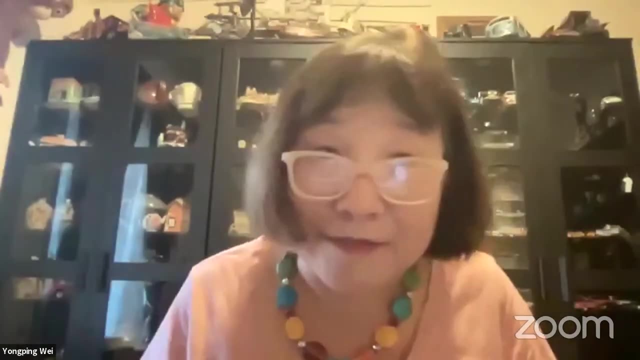 Because I changed my computer today. computer is dead, sorry for that. So can I? Farid can talk first, is that okay? Yes, I think. yeah, I was really sorry, because I don't know. I saw my slides in my, that's in my screen. 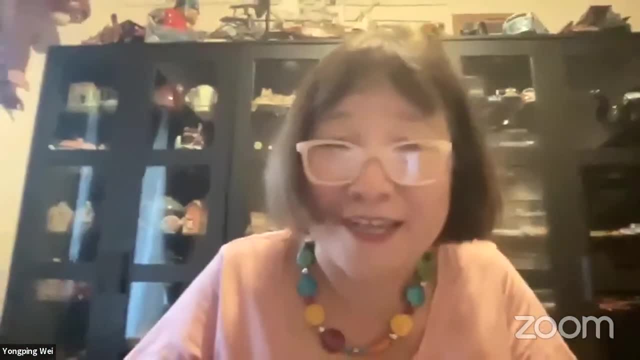 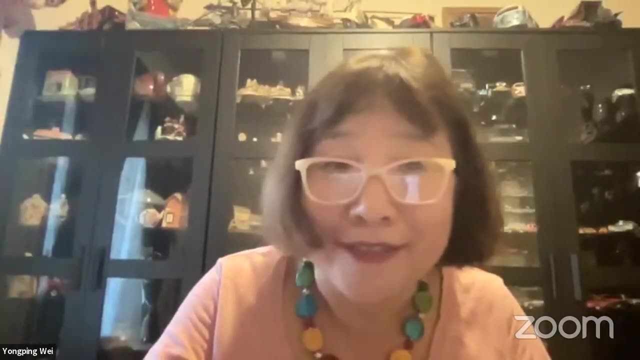 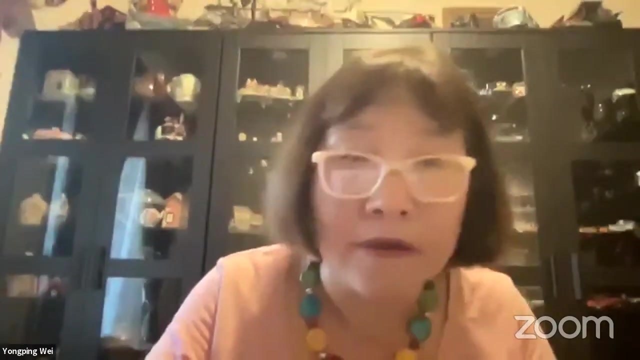 but I couldn't share with you guys. give me five minutes, I'll fix that, all right. yeah, Yes, it will be okay. I'm really sorry, Please take your time. Yeah, thank you. yeah, So, Paramita, would you like to introduce me first and then I'll start talking? 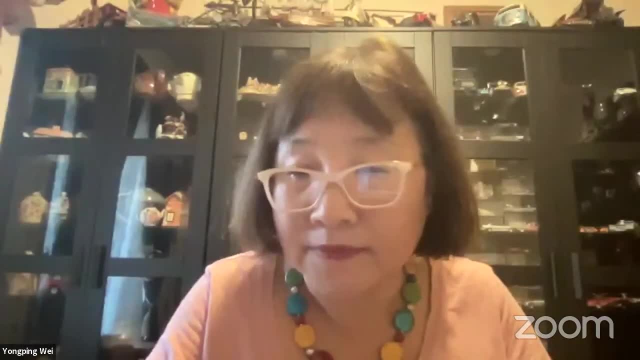 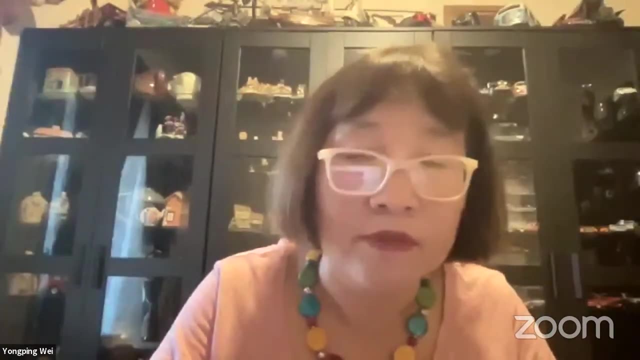 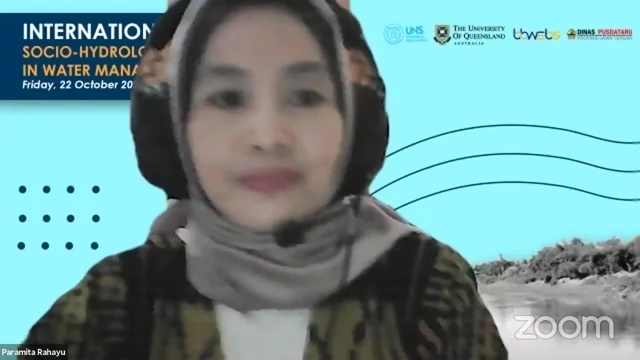 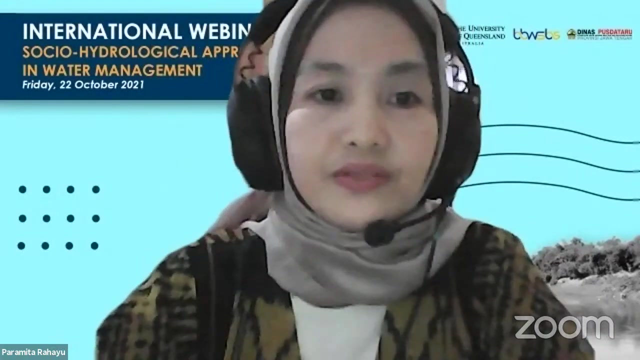 after that. Yes, sure, So we'll go to our second speaker for today because of the technical matters. Our second distinguished speaker is Dr Frederick Bowkert. He holds a PhD on integrating with our basins, governments and management. 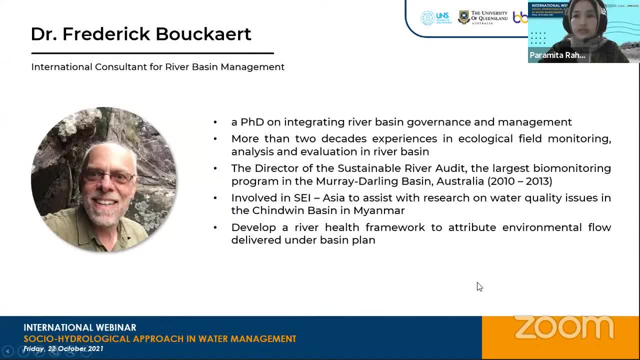 He has more than two decades of experience- sorry, has two decades of experience- in ecological field monitoring, analysis and evaluation information. He was the director of Sustainable River Audits, the largest bio-monitoring program in the Murray-Darling Basin, Australia, 2010, 2015.. 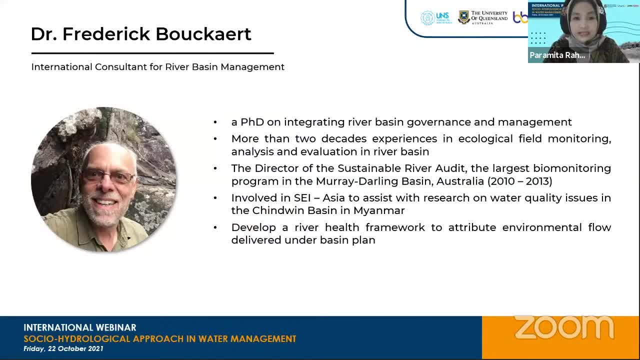 Dr Bowkert is involved in SER. He has been working with the National Fisheries Agency in Asia to assist with research on water quality issues in the Chinchewin Basin in Myanmar And he developed a river health framework to attribute environmental flow delivered. 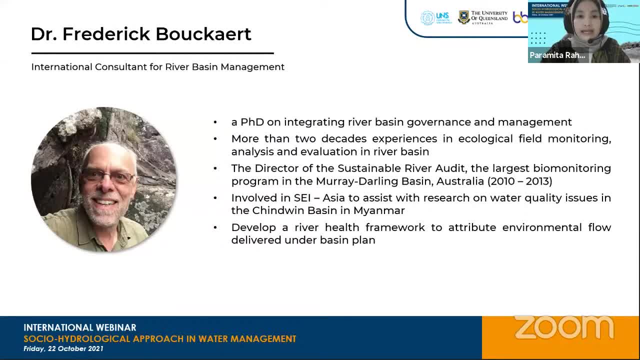 and delivered under basin plan, And Dr Frederick Bowkert will be investigating on managing interaction between biophysical and social systems in water management. Welcome, Dr Bowkert. Thank you, work at uh. please, you can start their presentation. thank you very much. i will first. 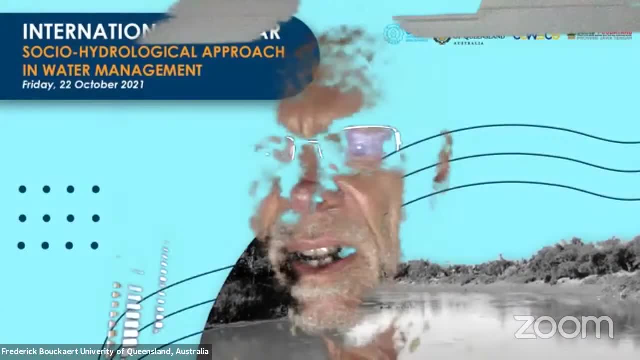 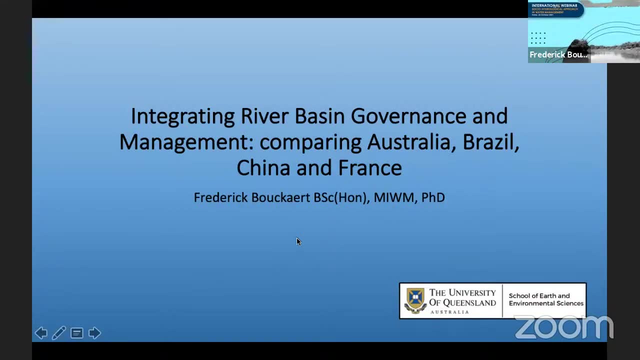 find the file to share my screen can. can you see my slides? yes, okay, so basically, um, thank you for inviting me to this conference. i'm very honored to be part of this and, uh, the research that i have done i i think can contribute something to the precious management of water governance. 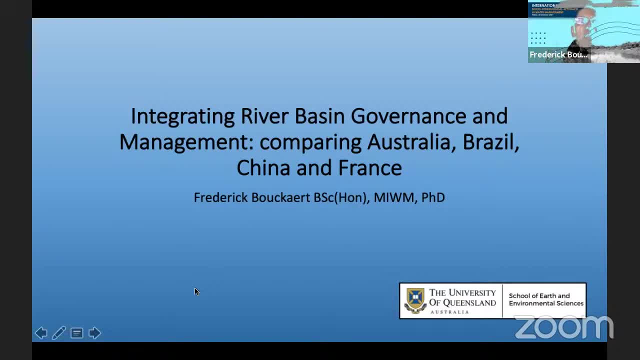 in indonesia as well. i will explain why in a minute. so basically, my research topic for my phd, which is what i'm talking about today, was around integrating river basin governance and management and comparing four river basins in australia, brazil, china and france. so why do we need to integrate river basin governance and management? 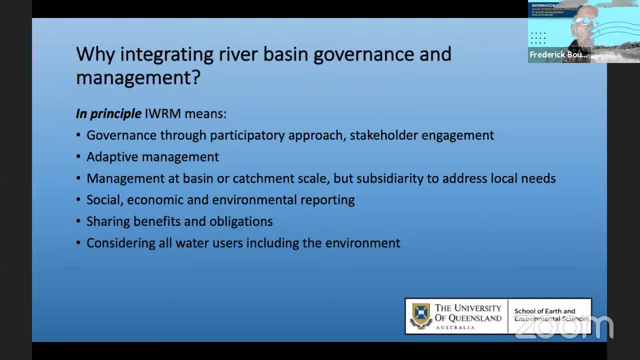 in principle. integrated water resource management means governance through participatory approach and stakeholder engagement. it means adopting adaptive management where you're learning by doing. it means management at the basin of catchment scale, but also subsidiarity to address the local needs of people. it means social, economic and environmental reporting. it means sharing the benefits and obligations of 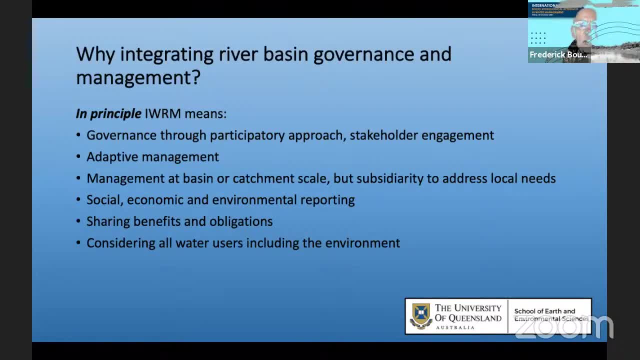 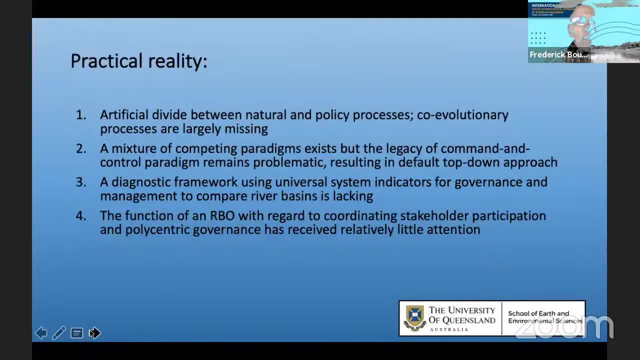 water use and also considering all water users, including the environment. however, the practical reality of integrated resource water management often doesn't work out like that always. there is still a very artificial divide between natural processes and policy processes and the core evolutionary processes, so the interaction between both is often missing. 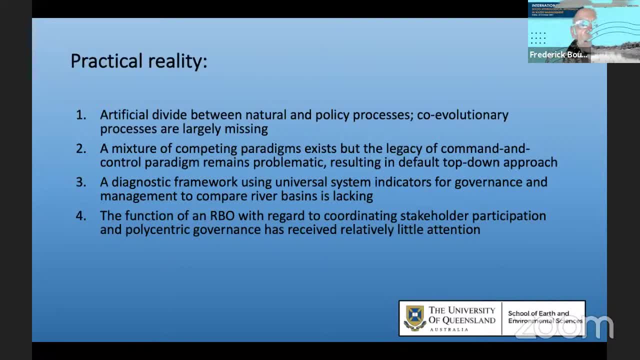 there is still a mix between natural processes and policy processes and the core evolutionary processes, and then there is a mixture of competing paradigms that exist, but overall in many basins there is a legacy of command and control paradigm which remains problematic. the reason is because that is evolved from a very strong hydrological approach. 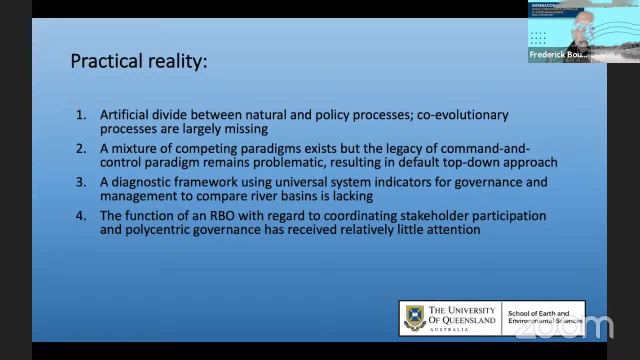 engineering approach and establishing infrastructure. this results in a very top-down approach and seems to ignore to some extent the system requirements and the local needs of water users. a diagnostic framework using universal system indicators for governance and management to compare river basins is also lacking at the moment, and the function of a river basin. 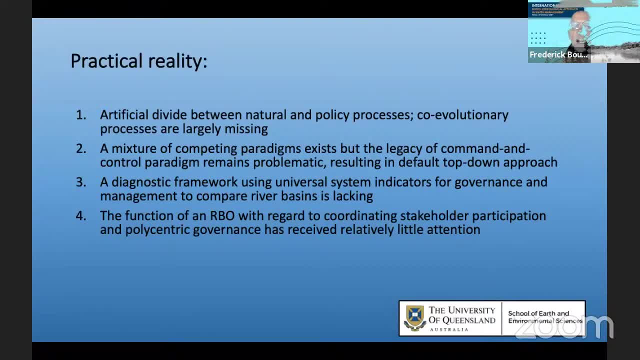 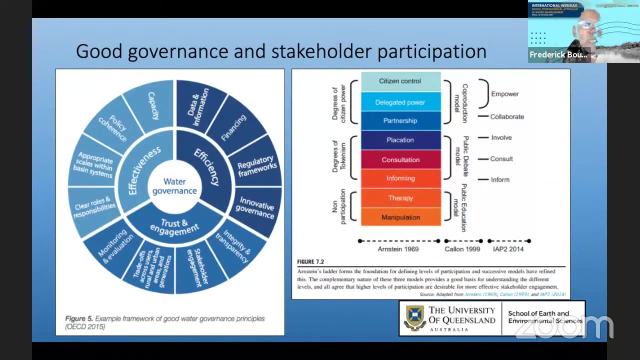 organization with regard to coordinating stakeholder participation and polycentric governance has also received quite little attention to date. so for good governance and stakeholder participation, some progress has been made recently, but there is still no universal agreement on what constitutes good governance and stakeholder participation. the oecd framework which basically was established 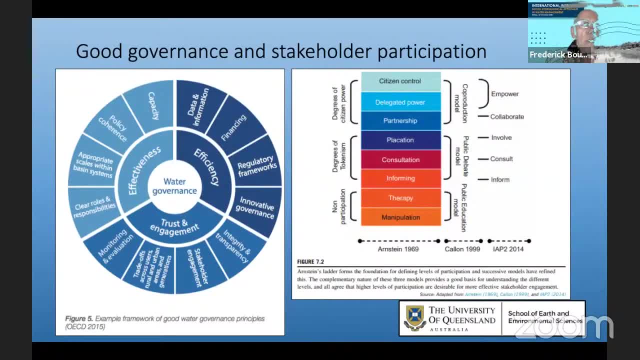 in 2015 is adopted more and more, and they have three major components, and they are effectiveness, efficiency and trust and engagement. for each of those, they have, uh, four different types of indicators that they want to use to assess good governance. on the other hand, stakeholder participation has been investigated as a ladder going from the 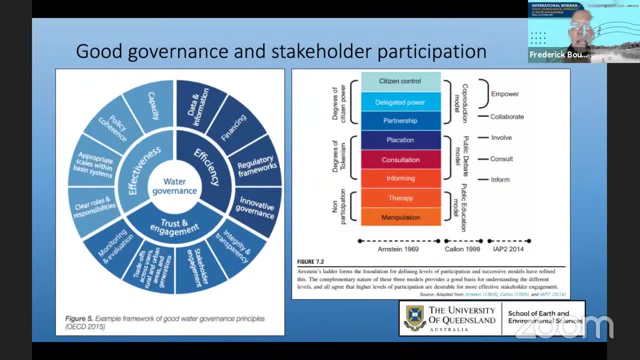 bottom rung, which is manipulation, to therapy, and gradually higher to informing, consultation, placation, partnership, delegated power and citizen control. control, so that the lower ranks of the ranks of the ladder really do not constitute participation at all. the middle ones are more like tokenism and the top ones are really degrees of citizen power. 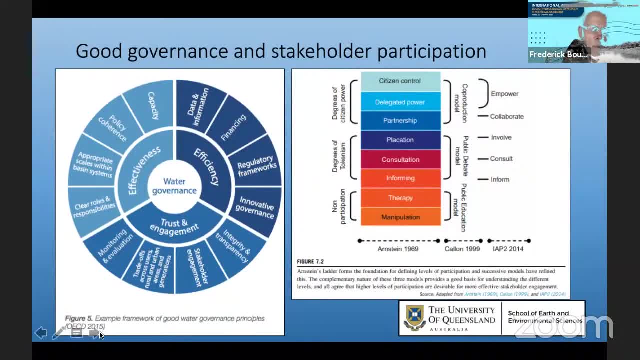 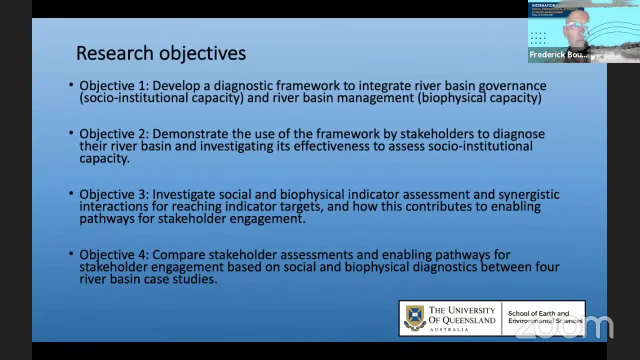 where people get really engaged with, with decision makers. so my research objectives were basically, firstly, to develop a diagnostic framework to integrate river basin governance, which is the social institutional capacity of a river basin, and river basin management, which is the biophysical capacity. the second objective, then, was to demonstrate the use of the framework. 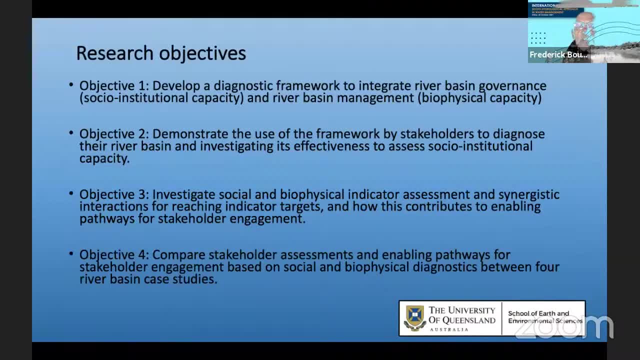 by stakeholders to diagnose their river basin and investigating its effectiveness, to assess social institutional capacity. why social institutional capacity? because, as i mentioned, there is still no universal agreement on what works best as indicators in that domain, whereas in the biophysical domain there is much greater agreement about what. what are the right indicators to use? in the third objective, then, 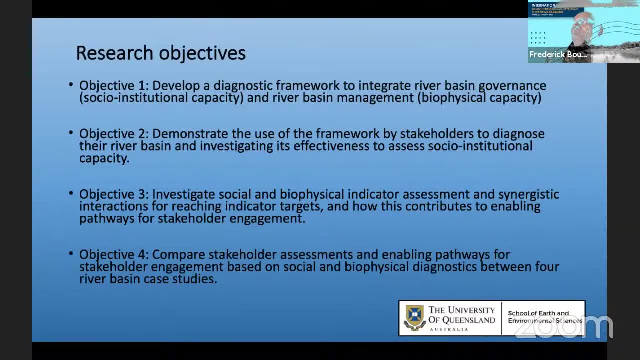 i want to investigate social and biophysical indicator assessment and the interactions between those indicators, also for reaching targets, and also how this contributes to enabling pathways for stakeholder engagement in reaching the target indicators. and finally, i want to compare the stakeholder assessments and enabling pathways for stakeholder engagement between the four river basins that. 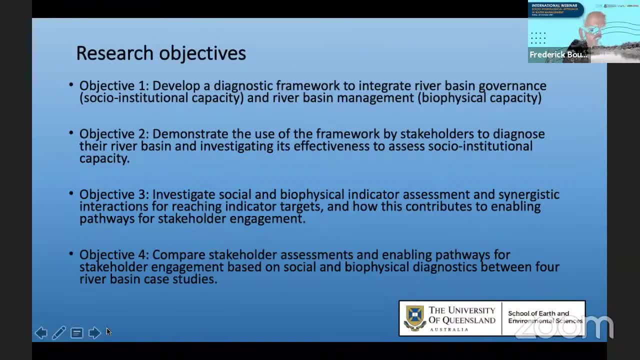 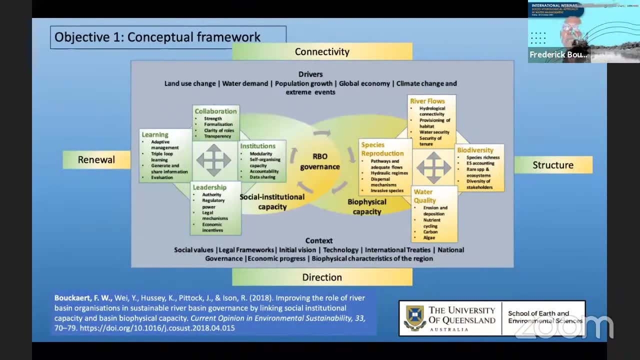 case studies that i have studied. so the first objective, then, is my conceptual framework that i constructed. it basically consists of two major domains- the social institutional capacity and the biophysical capacity, and for each of those there are four key indicators that correspond to four key functions. the first function to mention is connectivity. 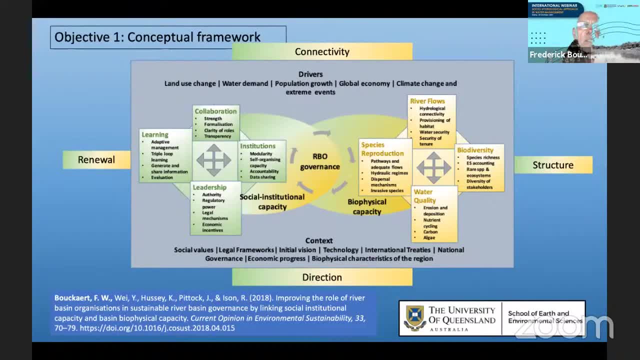 connectivity in a river system translates into collaboration between stakeholders in the social institutional domain, and under collaboration you find a whole range of attributes which can be also tailor-made for the specific characteristics of that river basin. in the biophysical domain, it translates into river flows. river flows are what connects all everything in the system. 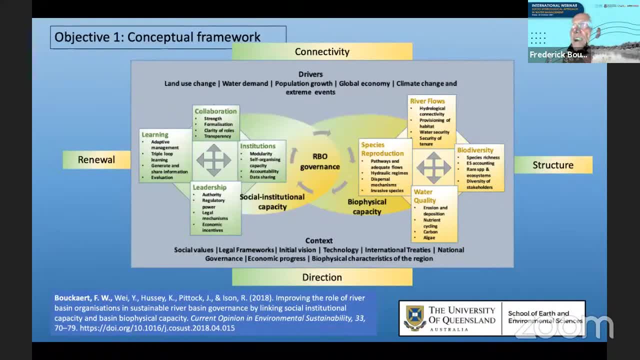 the second function is structure, and structure basically corresponds in the social institutional domain to institutions and they are the functions that are the individual structures and sometimes even the social institutions are the physical structures that are located in the community, within the community, and there is also the social institution data. that is an important part of this process. a lot of this is an interactive 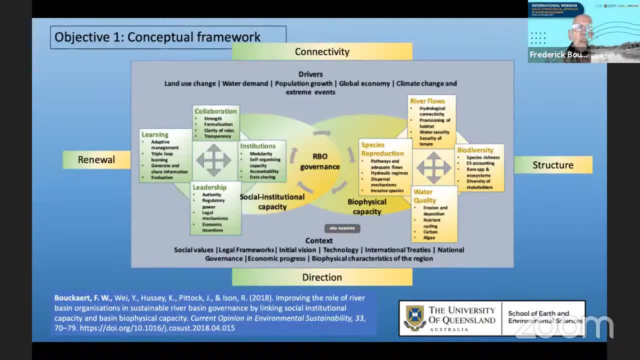 too extreme. All the rules, regulations, organisations and institutions that humans have devised to basically manage and govern the river systems are part of this. In the biophysical realm, this constitutes the biodiversity and all the structural elements of an ecosystem, ecosystem services, and so on. 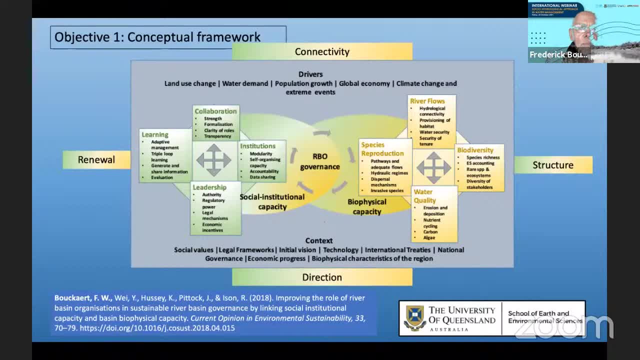 The third function is direction, and direction in the social institutional capacity translates into leadership, basically to aim for a particular sustainable development goal or a particular end point, whereas in the biophysical capacity this corresponds to water quality. That may not be immediately apparent, but water quality. 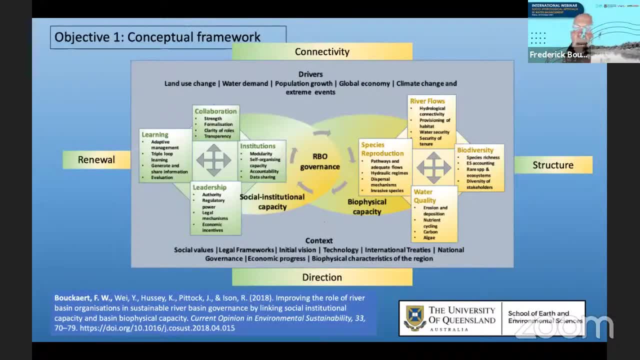 Is something that can change from very good quality to very bad quality in rivers and lakes, and also water quality is part of erosional and depositional processes which determine the channels of the rivers and basically, in that sense, determine the direction as well. And finally, the function of renewal translates into social, institutional capacity, into learning. 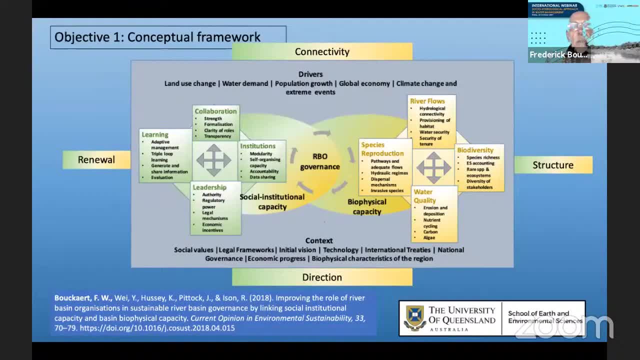 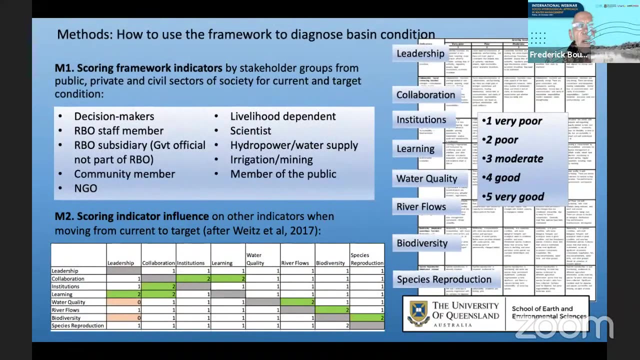 And In the biophysical domain, into species reproduction, basically so that the system can keep continuing over time. So how did I use that framework? I basically use the framework to let the stakeholders themselves diagnose the river basin condition. First of all, I categorise stakeholders in 10 different states. 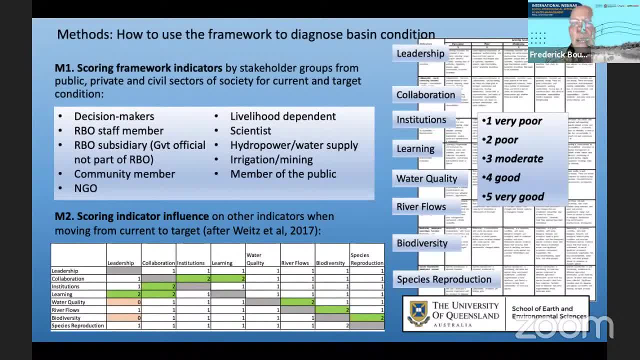 Stakeholder groups And then I asked them to basically Use each of those 10, each of those indicators and sorry, And asked them to rate it from very poor to very good, and I gave them a descriptive, descriptive rubric, which you see on the right of the slide. 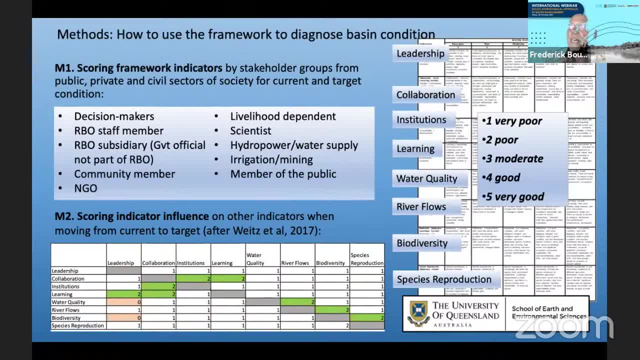 With explanations for each of the indicators, What it means When something is very poor or something is moderate or when something is very good. So I asked them to do a rating of the current condition And then I also asked them to do a rating of what is a reasonable target. 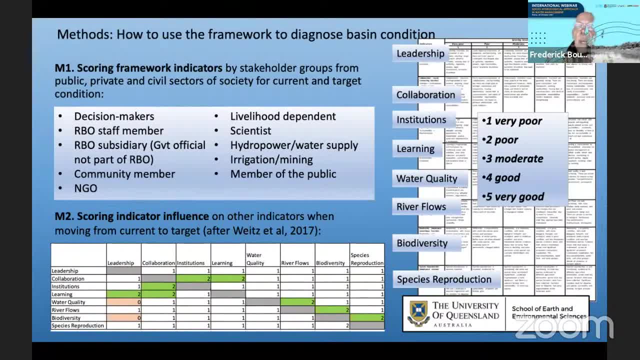 condition for the end of the basin plan, so that you can start seeing what the current condition is, what the target condition is and how far away each of those indicators are from target. I also asked them to look at how each of the indicators score in terms of influencing other indicators. 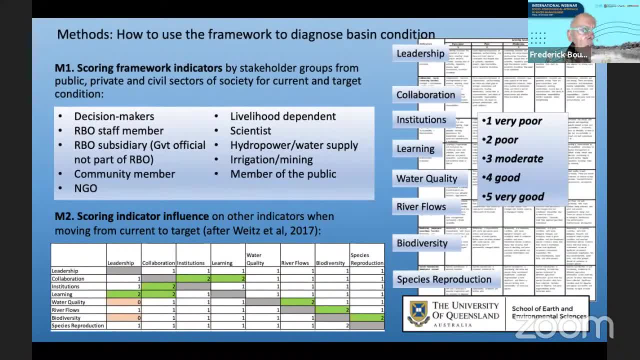 So if there is a progress going from current to target for, for example, for collaboration, if you see in the bottom part of the slide here what would be the influence of collaboration on institutions and on learning, And you can see here that that would be. 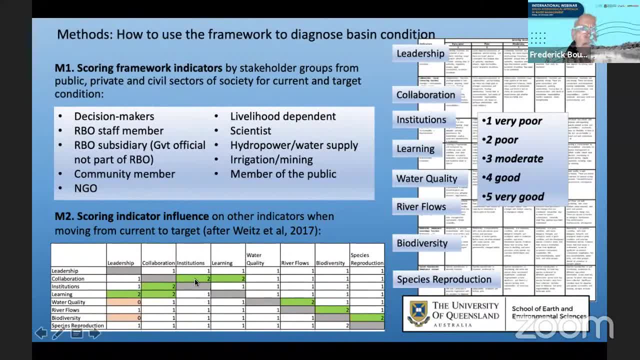 assigned a number two, which is actually very synergistic. The rating scale here goes from two, which is synergistic, One is actually a little bit less, zero is neutral, minus one is actually counteractive and minus two is stronger counteractive as well. 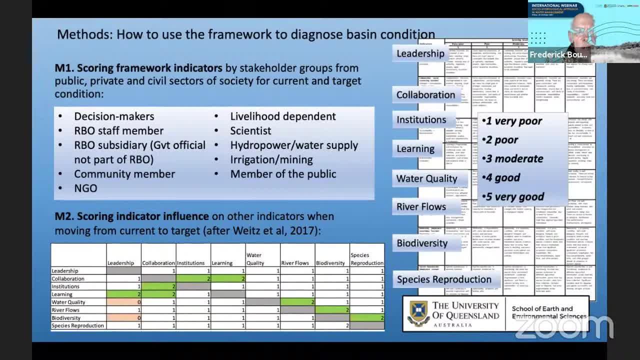 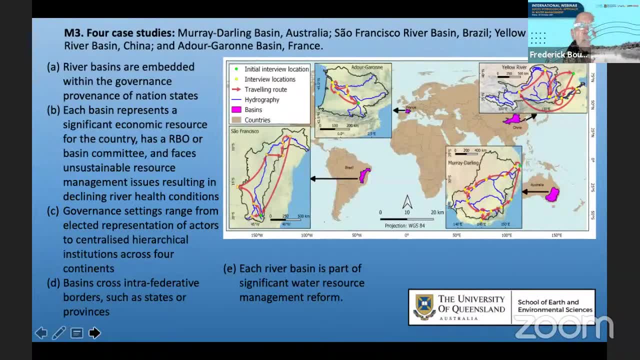 So that basically allows you to map out where the synergies are between the different indicators. So I basically looked at four case studies: the Murray-Darling Basin in Australia, the South Francisco River Basin in Brazil, the Yellow River Basin in China and the Adour-Garonne Basin in France- and each of those river basins are embedded. 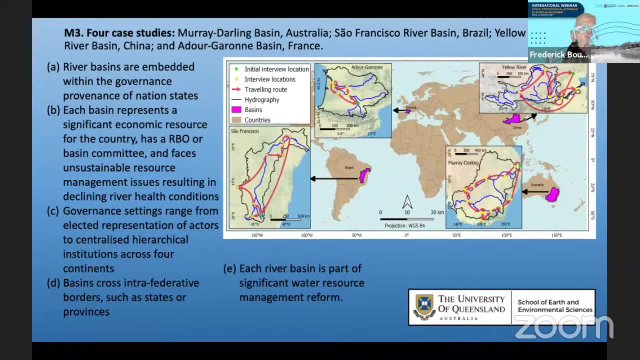 within the governance provenance of the nation states, meaning they are not international river basins. They represent a significant economic resource for the country, They have a river basin organisation or a basin committee and they face unsustainable resource management issues resulting in declining river health conditions. 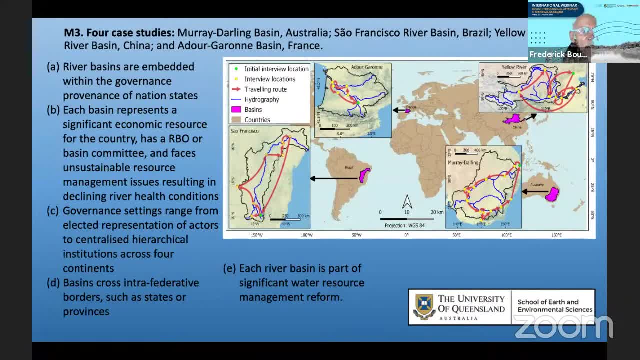 Their governance settings range from elected representation of actors to centralised hierarchical institutions across four continents. And also, what's important is that for each of the basins, there are state borders or provincial borders within the country that provide, you know, governance challenges. 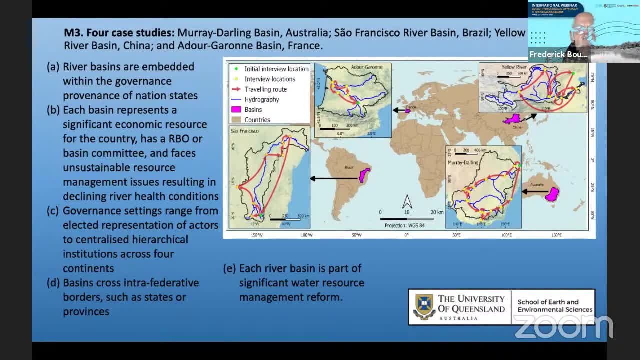 And also each of the river basins is part of significant water resource management reform. I travelled in each of those basins and interviewed between 20 and 30 stakeholders in each basin, from the upper, the middle and the lower parts of the basin, as indicated in the travel on the map of the slide. 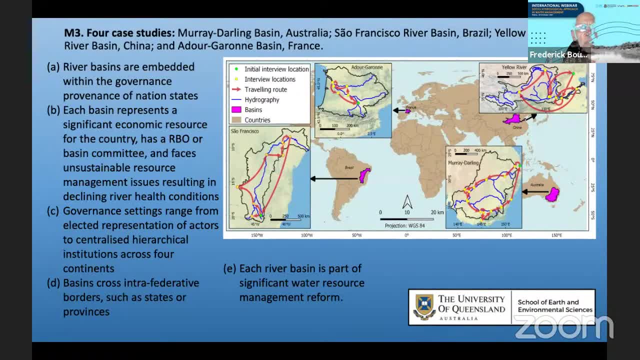 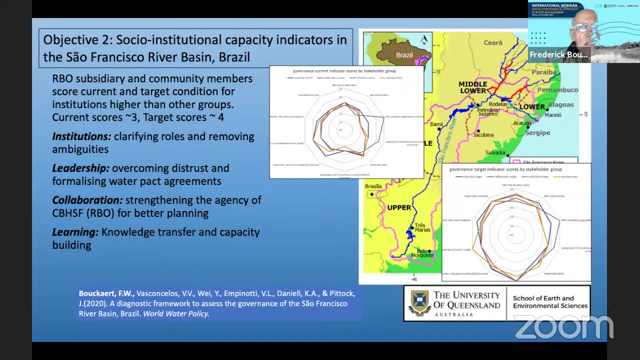 So the second objective then investigating the social institutional capacity indicators in the South Francisco River Basin. when I did this, I basically found that, for the indicator institutions, what was really important for the stakeholders was clarifying roles and removing ambiguities. The leadership was overcoming the distrust and forming 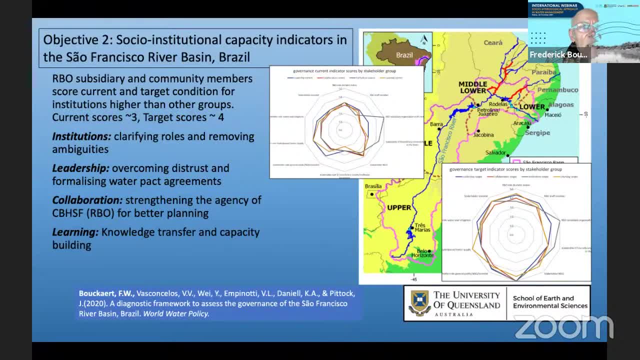 border pact agreements in collaboration, strengthening the agency of the river basin organisation for better planning and for learning, the knowledge transfer and capacity building. The diagrams you see here on top of the maps are basically the 10 stakeholder groups and for the RBO subsidiary, which are the government officials not part of the River Basin Committee. 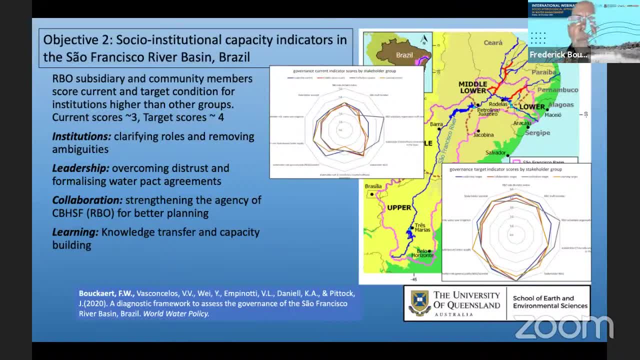 You can see that they basically have more institutions, much higher than any of the other indicators for current, And that's still the case also for target indicators as well. So this basically gives you a picture of the difference between how different stakeholder groups rate each of those diagnostics. 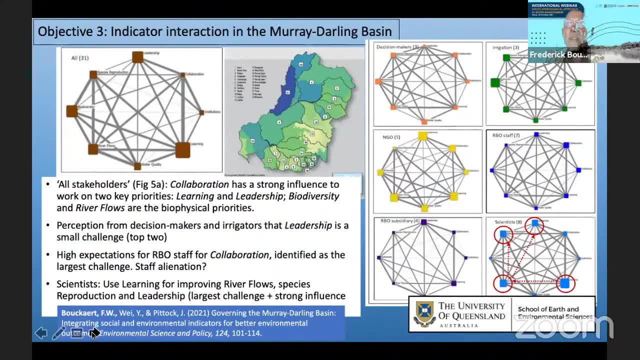 In the third objective, I looked at the indicator interaction between river basins, between indicators in the Murray-Darling Basin, And what you see here are the social network diagrams that are constructed And what they actually mean is for each of the nodes there are the indicators. 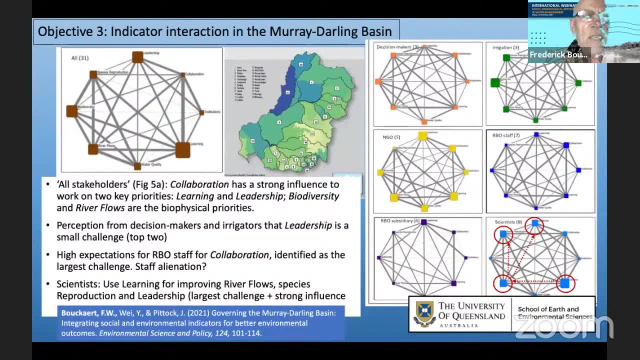 and the larger size of the nodes indicate that the difference between target and current is larger, which basically means that they are more difficult to reach Because they're starting from a poor current condition and have a longer way to travel. All the links between the indicators. 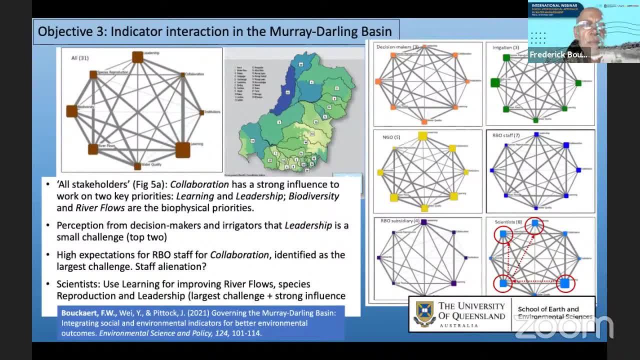 the thickness of the lines indicate the synergies between them. So the thicker the line, the stronger the synergistic connection between indicators. What you see on the upper left is a diagram for all of the stakeholders in the Murray-Darling Basin and you can see that. 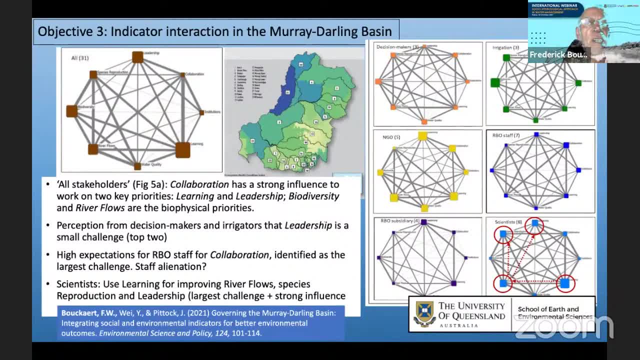 collaboration is a relatively small node. That means it's easy to achieve and it connects very strongly to learning and also to leadership, which are much more challenging indicators to achieve. So from this you can basically start devising enabling pathways for how you might strategize reaching your indicators. 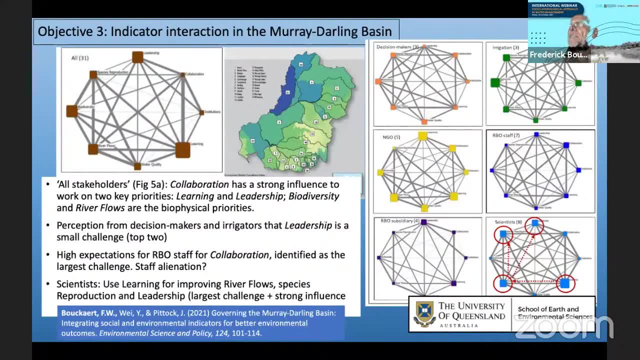 The other important thing to note is the difference between different groups. You can see, for example, decision makers on the top right- the orange diagram- and irrigators- the green diagram. The top node there is basically leadership, And you can see that these nodes are very small, meaning that for those two groups, 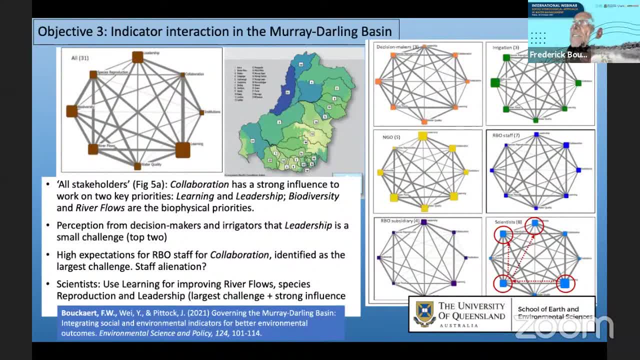 leadership is an easy target to reach, But if you go down and look at the other diagrams for NGOs, for example, the yellow one below it, leadership is much larger and is seen as a much larger challenge, And that's also even the case for government officials. 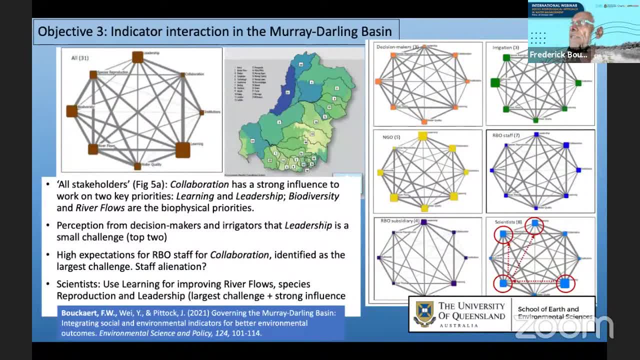 below it, and also for River Basin staff as well. Finally, the bottom diagram for scientists is an illustration of how you can use these diagrams to create enabling pathways. You might want to start from the most challenging indicator. In the case for scientists, that is basically learning. 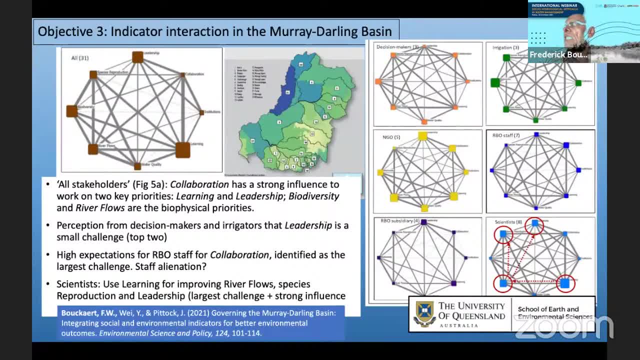 And then decreasing in size. look at the connection towards river flows, which is a little bit smaller in size, and then further to species reproduction, which is slightly smaller, but also in connection towards leadership, And you can see that using these diagrams, you can start prioritizing and focusing on what is important for each of those. 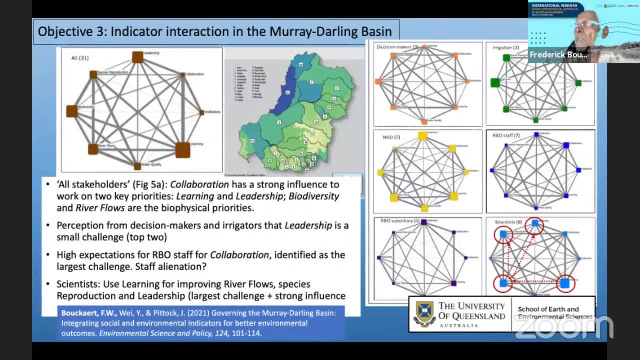 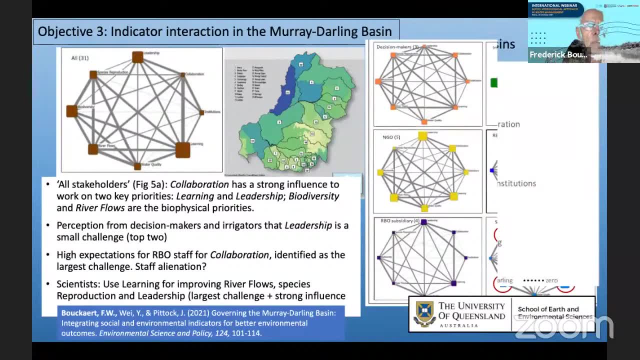 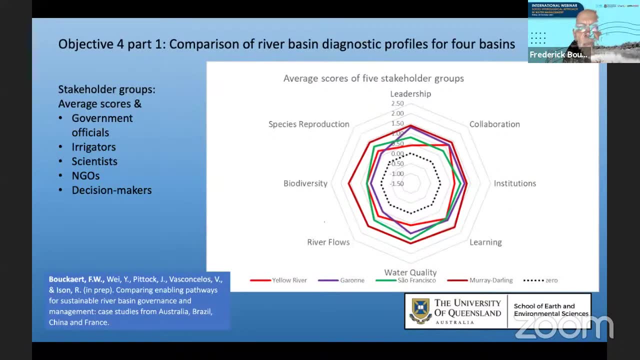 stakeholder groups to focus on in their role that they would play in a strategic plan for river basin management and governance. So the fourth objective then the comparison of river basin diagnostic profiles for the four river basins. What you see here is a diagram with the scores between targets and current. 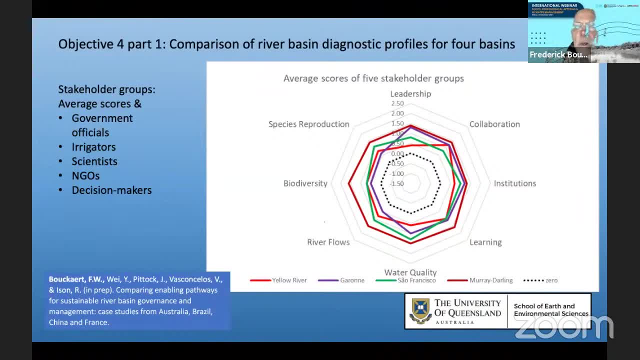 For each of the four river basins, for all the stakeholders collectively, And you can see here that for the Murray-Darling Basin the outside profile looks larger than the other ones. What that actually means is that, for all of the indicators, the Murray-Darling 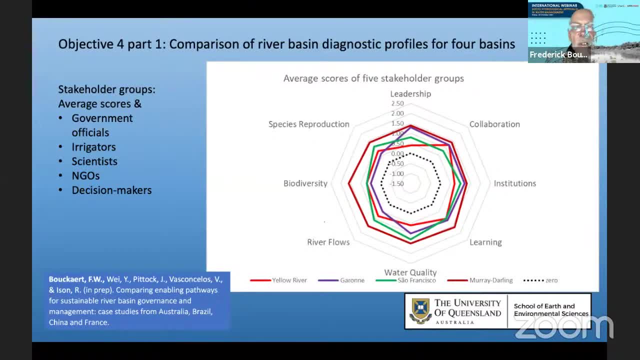 Basin has bigger challenges to reach the targets than for the other river basins. What you can also see, for example, is that for species reproduction, biodiversity and river flows, the scores for the other three river basins are relatively small compared to those of 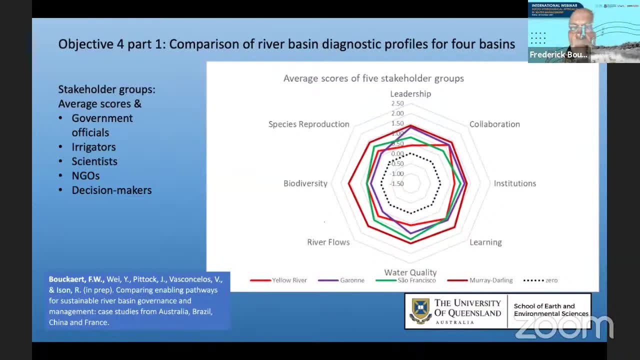 the social institutional indicators, such as collaboration and learning in particular. So this, basically collaboration, looks like a particular challenge for the Yellow River, which is the red profile, And so this basically allows you to distinguish between the different river basins. What are the bigger challenges in each of those basins? 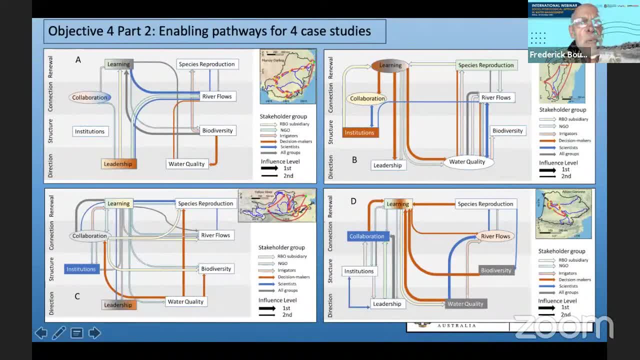 And then what I'm showing you here now is the enabling pathways for each of the river basins, And what this represents is the priorities that I was talking about, which are color coded for each of the stakeholder groups, and the thicker lines are basically the first priority. 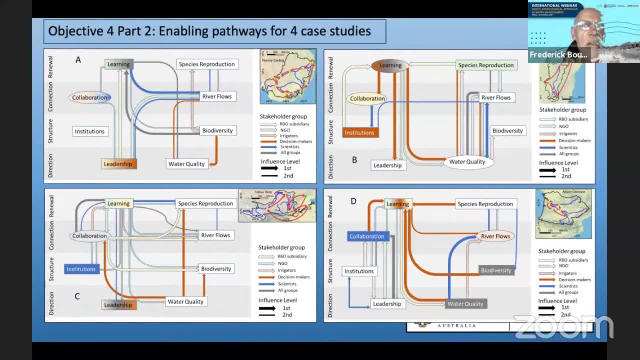 And the thinner lines are the second priorities And you can see where some of those lines for different stakeholders start to converge. In the Murray-Darling Basin, for example, a lot of the lines point towards river flows, which is where a lot of the objectives also focus on of the basin plan. 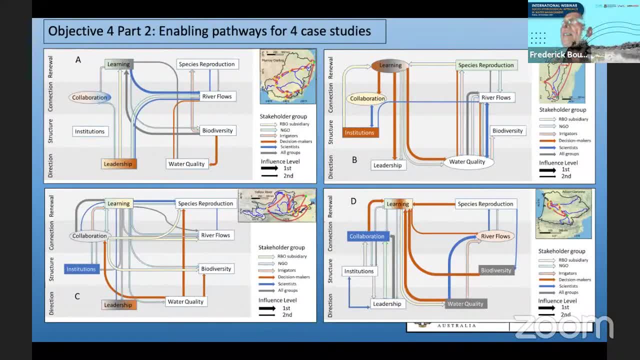 In the, the other one for the South Francisco River Basin. learning is a very important indicator, but that basically also flows towards water quality and river flows, where you can see that a lot of these arrows are coming together In the Yellow River. learning, leadership and collaboration are important indicators. 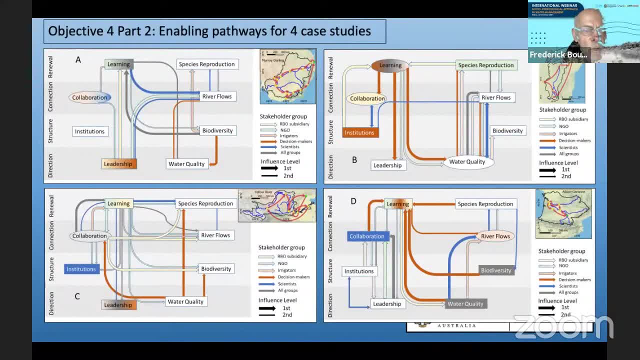 And they basically also point, of course, towards river flows, but also some of the other biophysical indicators, And in the Adour-Garonne Basin, leadership and learning and collaboration are really important indicators, in particular leadership, which is deficient in that river basin because of the consensus model. 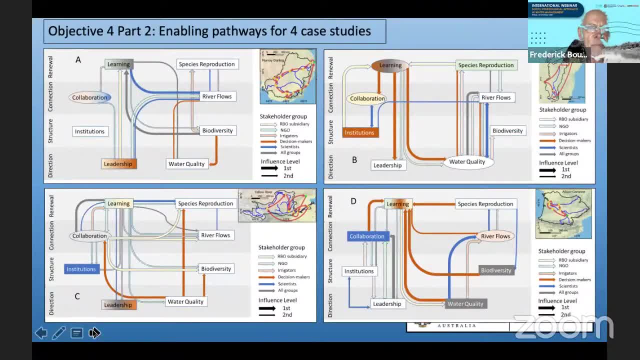 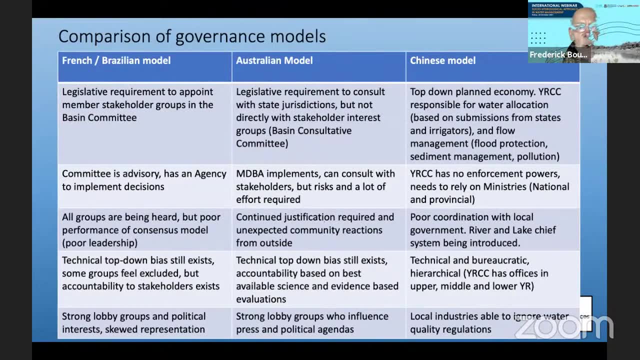 and the fact that they cannot agree very well in that river basin, which leads me to the comparison of government goals. Your time is about one minute more, Dr Bokart. OK, I'll try and speed it up a little bit. 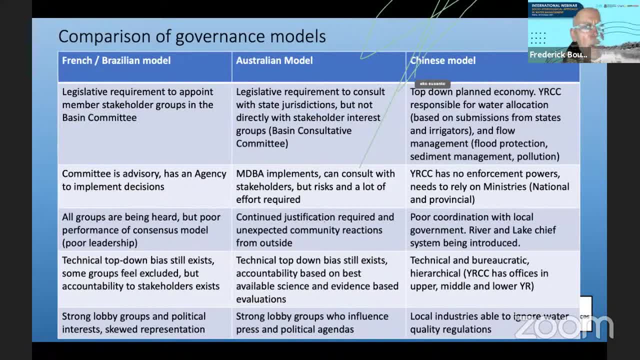 So in the French-Brazilian model they have the same governance model. There is basically a legislative requirement to appoint member stakeholder groups in the basin committee. The committee's advisory has an agency to implement decisions and all the groups are being heard. 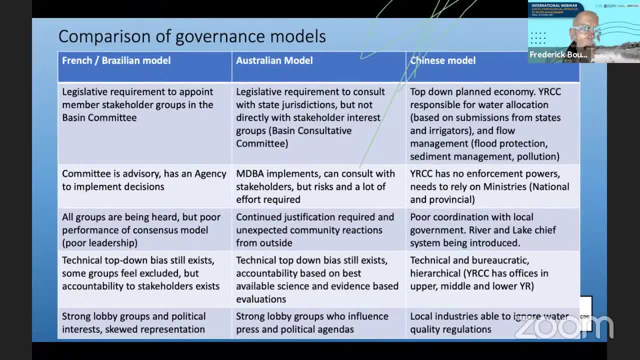 But it's a poor performance model because the consensus model means that there is poor leadership very often and therefore sometimes it's dominated by lobby groups. So in the Australian model there is no legislative requirement to consult with stakeholders, but with state jurisdictions instead, and they basically have to justify what they do based on evidence. 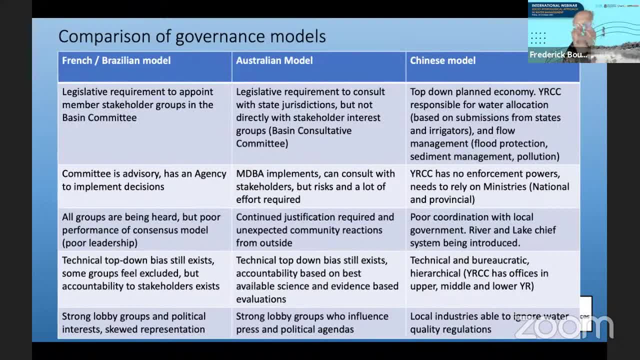 based on science, whereas in the Chinese model is very, very top down And basically the Yellow River Conservancy Commission is the one responsible for water allocation, but they have no enforcement powers and have to rely on the ministries, And there is a poor coordination with local government. 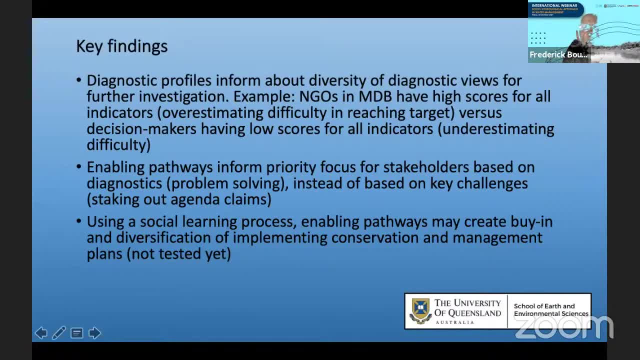 So the key findings of my research is that diagnostic profiles inform about the diversity of diagnostic views for further investigation. There are enabling pathways that stakeholders can base for diagnostics and using a social learning process might create buying and diversification of services. So the information is no longer an apparatus. 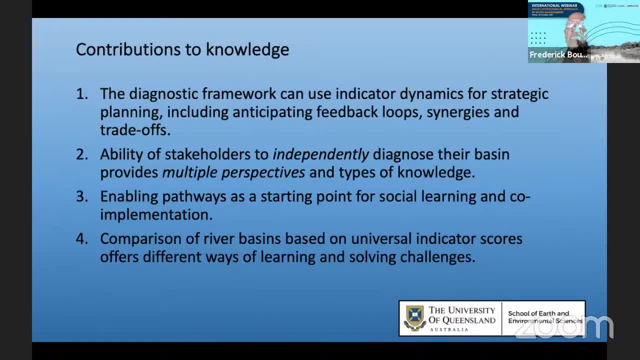 for implementing conservation management, but that still has to be tested. So my contributions to knowledge are basically that a diagnostic framework can use indicator dynamics for strategic planning, including anticipating feedback loops, synergies and trade offs. It allows the stakeholders to independently diagnose the basin and provide multiple perspectives. 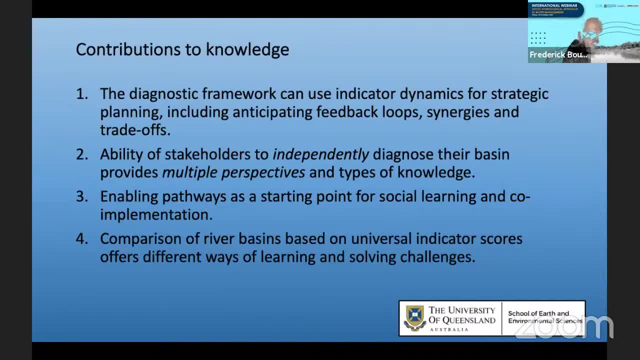 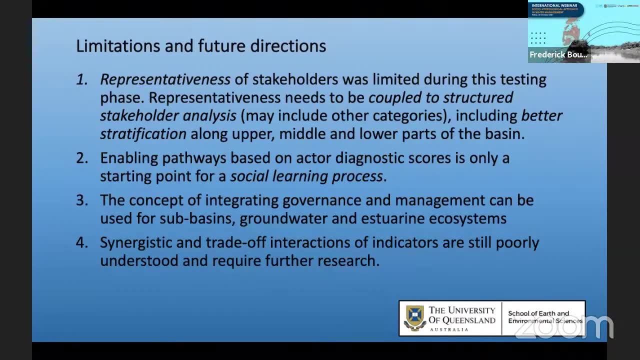 And it's a starting point for social learning. so, finally, the limitations and future directions: um, basically, um, there were some limitations in representatives of stakeholders. that needs to be expanded, i think. um, and, as i mentioned, it's a start of a social learning process. the concept can also be used in sub-basins, groundwater and 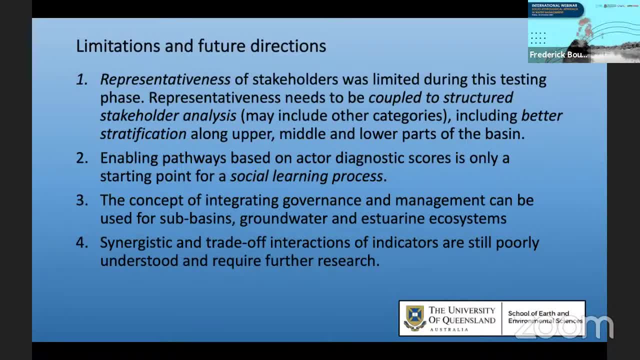 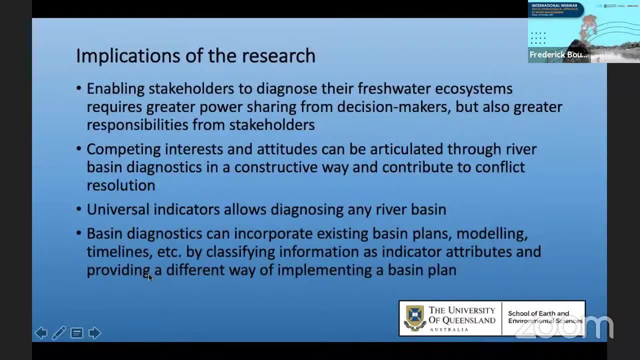 estuarine systems and synergistic and trade-off interactions still need to be investigated more, because that's poorly understood. so, basically, the implications then are that enabling stakeholders requires greater power sharing from the decision makers, but also greater responsibilities from stakeholders. competing interests and attitudes can be articulated through this diagnostic framework. 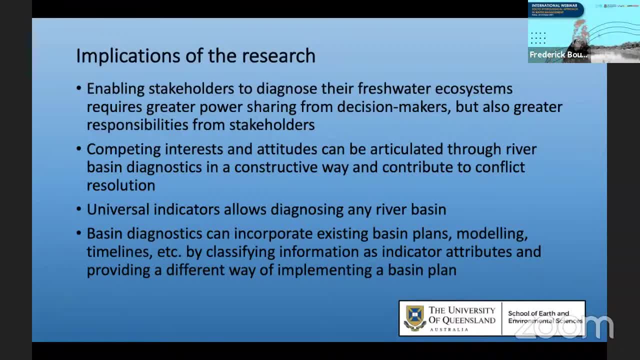 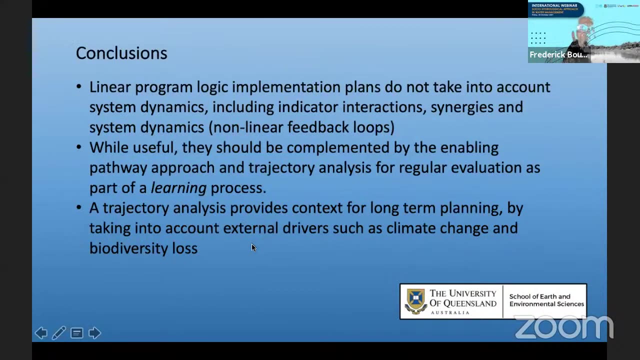 and these universal indicators allow diagnosing any river basin, also in indonesia, and uh, the basin diagnostics can incorporate existing basin plans and information, which is quite important. so in conclusion, then, um, the linear program logic that often uh is used in implementation plans doesn't take into account system dynamics. so, um, basically, this framework uh complements that. 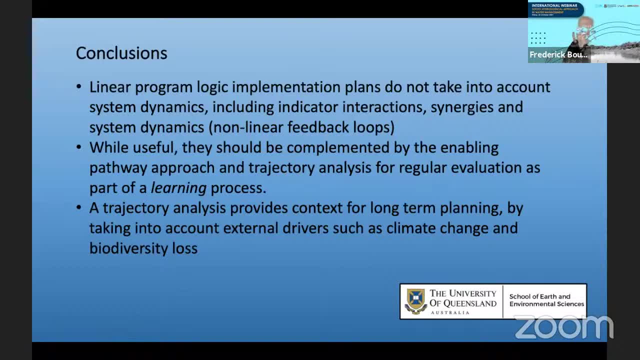 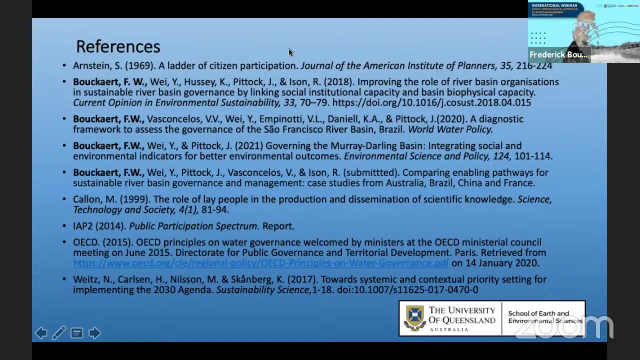 and um. so this should be um in the trajectory. so this is basically uh the major conclusion of it. so thank you very much for that. thank you very much, dr uh bookert, if if i may uh emphasize uh several uh important point. maybe i could not grasp it all, but i'm trying to just emphasize several important point. the: 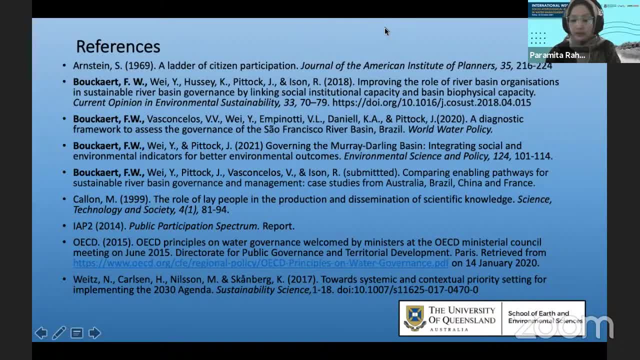 first is your framework is very, very interesting: uh used in social, social, institutional capacity, with biophysical capacity, with key for functions, connectivity, structure, direction and renewal. that you translate into eight indicators: collaborations, institutional domain, leadership, learning and water quality, uh and uh biodiversity, species reproductions and all those indicators. 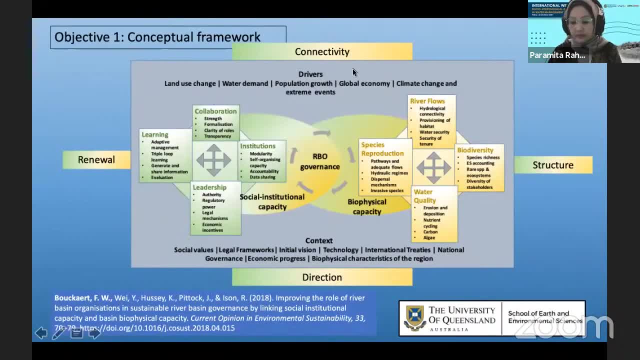 you apply to assess the uh conditions and vitae in coral water quality, uh allies working science and Bal фд and and uh, the kinds of governor's model that can be applied to manage that, the river basin management. but maybe we let the audience to maybe ask more to you in the Q&A sessions. 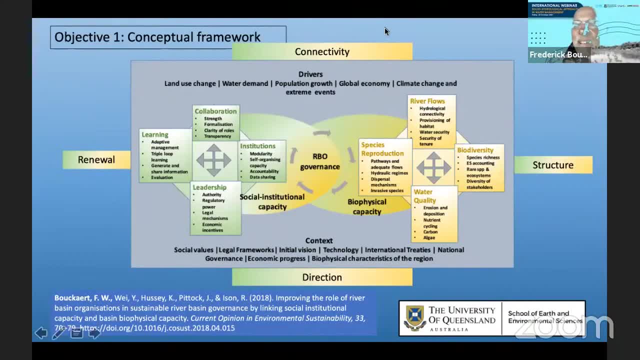 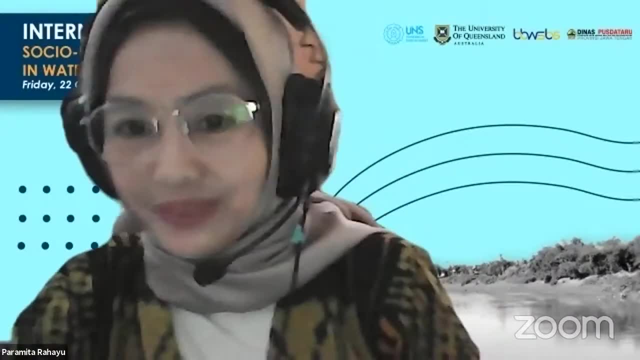 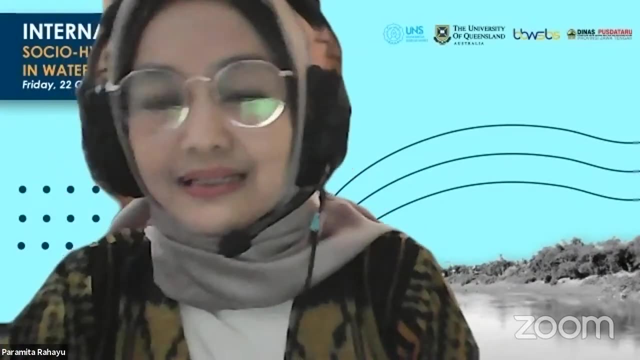 Thank you very much for a very interesting presentation. Thank you, And we are going back to our first speaker, Professor Yongping Wei. The time is yours now, I think. Thank you, Can you please share my slides? Yeah, then. 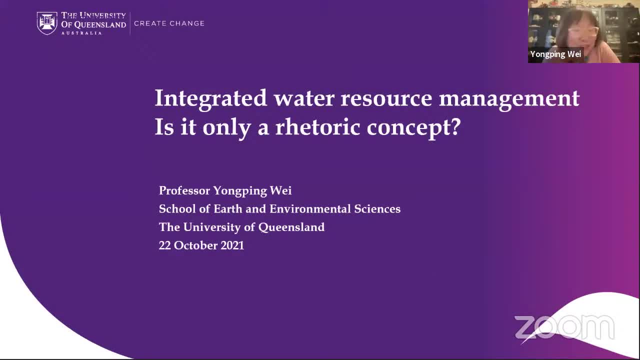 Yeah, put a slideshow. Thanks, Yeah, Thank you very much. Firstly, thank you very much all of your good effort for this webinar. I feel honored to attend this such a webinar, So being last 12 years, being always work at home to do my research. 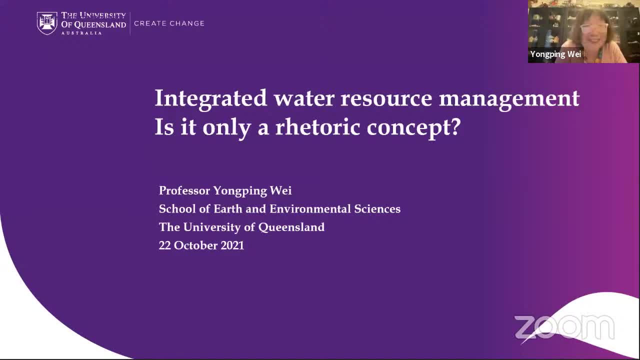 So I feel excited to talk, whatever I can talk today. Firstly, I'd like to reintroduce myself. So I started as an irrigation engineering, So engineer, for many years ago. After that I worked for government to do the water resource management. 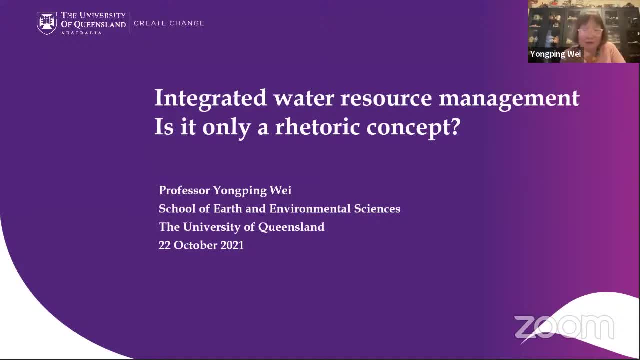 Then I came to Australia to do my research in the water resource management. So now I've got 12 years after my PhD. I have to work lots of collaboration, work through different development agencies, Like I work with AusAID, World Bank, Asian Development Bank, ACA- a variety of agencies. 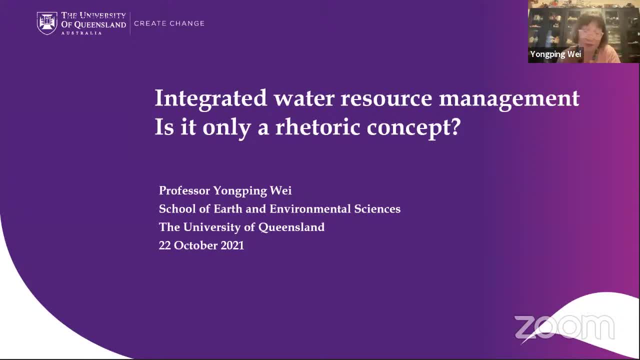 So my research is practice-driven research. So I like to take this opportunity. If we, after we share the experience, we develop more collaboration research to solve the river basin issues, That should be the end of destination of us. That's the nation of our today's webinar. 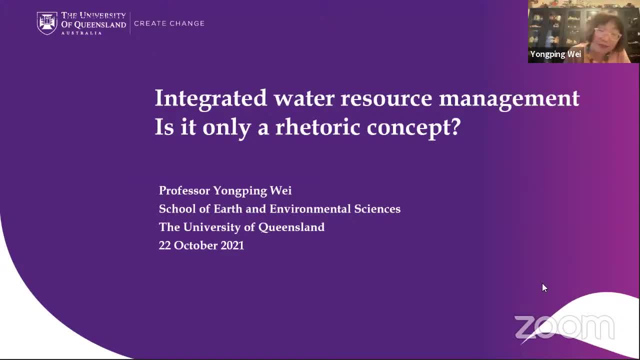 Five years ago I take this leadership in this school. I developed lots, lots of collaborations through different universities- probably over 20 universities, different countries Again, probably that's another opportunity We can work together to develop more research project. So I offer what I can do today. 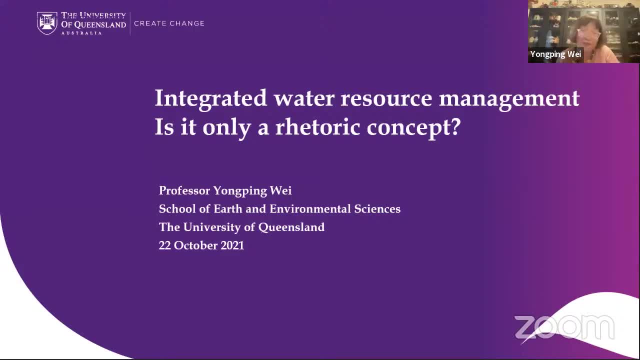 I'm looking forward to more collaboration, either through the water resource authorities or agencies or through your universities. Okay, so that's my feeling. now. I really feel really honoured to share my experience with you guys. I tell you, I have lots of experience working with different river basin authorities and different universities. 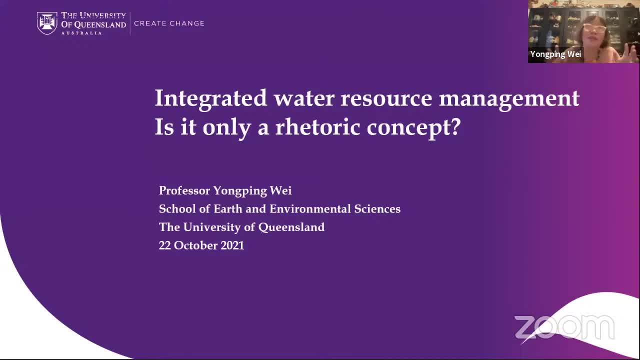 If you think we share some, we have some common interesting that's we work together. All right, Let me start my talk today. So my title is this title. It's Roger gave me this title, Sorry, it's called Integrated Water Resource Management. 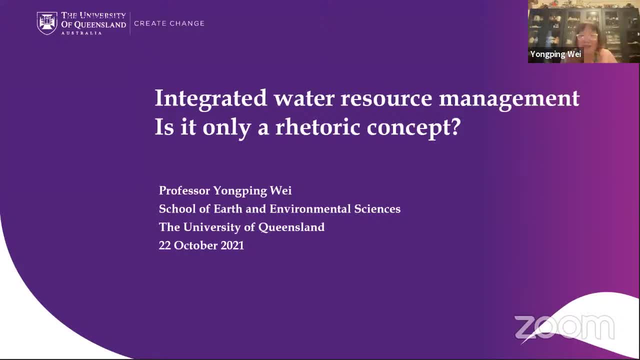 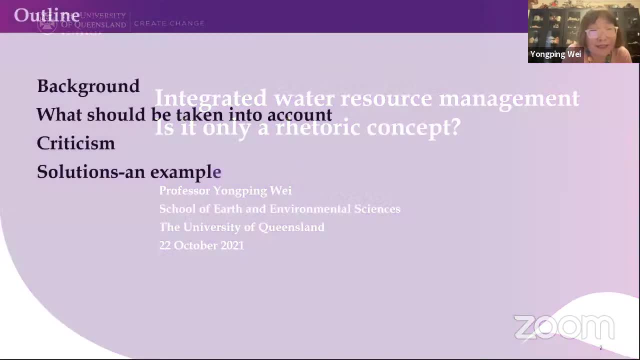 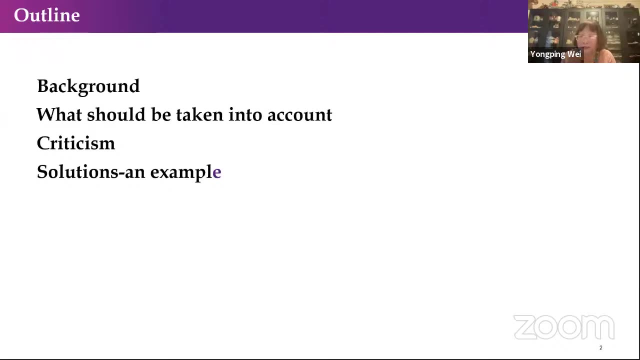 Is it only a concept? Nirvana concept? So next slide, please. So I'd like to talk a couple of things. One is: what's the background? Second one is what should be taken into account when you do integrated water resource management. 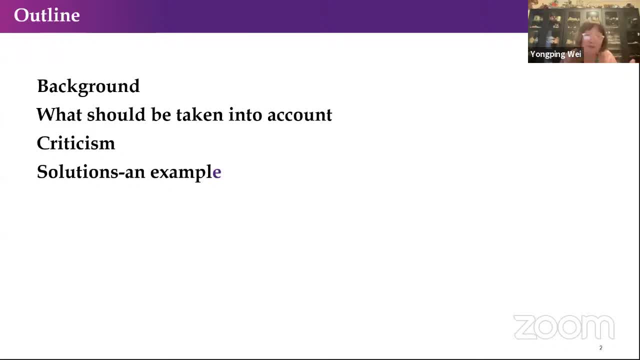 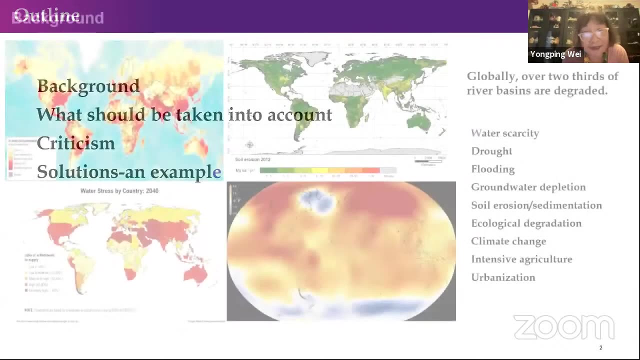 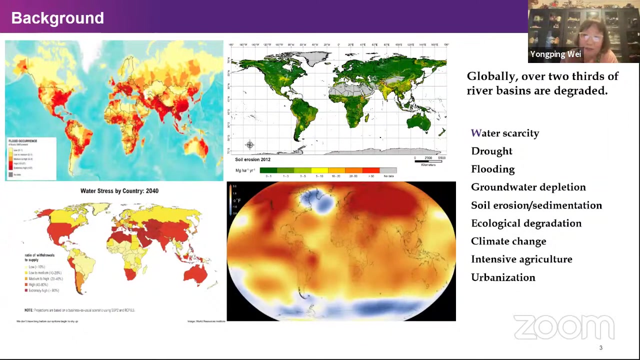 Then what's the current criticism? Lots of people don't like integrated water resource management. Why, Then? I'd like to share one of our recent research. What are solutions? Thanks, Next slide: Yes, I think, as everybody knows, we have global water challenges. 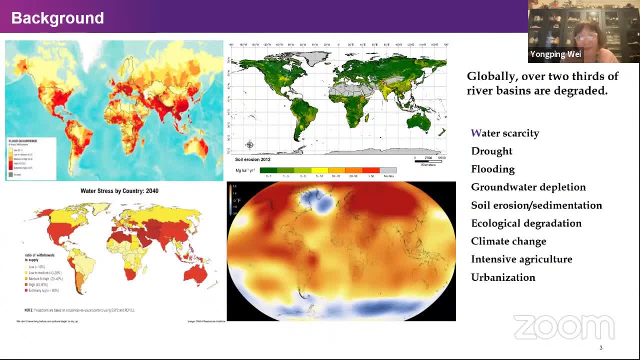 We have lots of water issues globally. It's like water scarcity, flooding, droughts, groundwater depletion, soil erosion, ecological degradation, climate change. So everything, Basically, two, Over two-thirds of river basin, Two-thirds of river basins, are degraded globally. 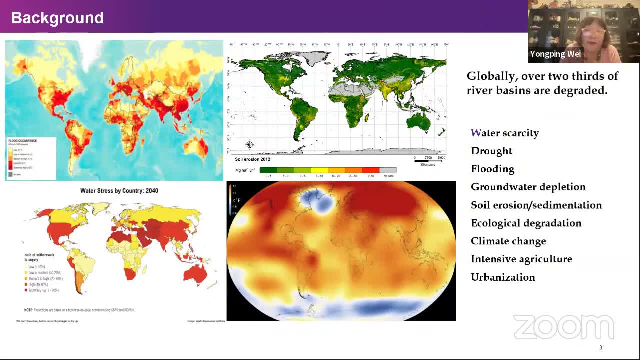 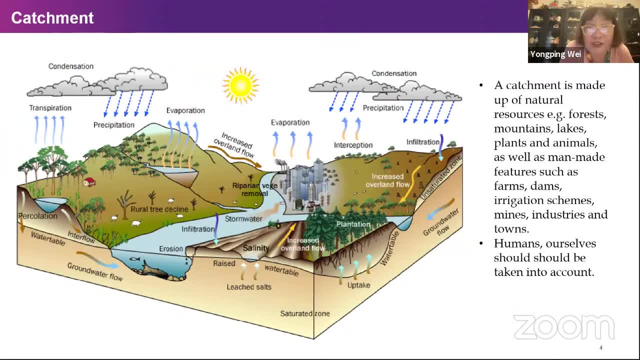 So that's a global challenge facing us. now Next slide, please. So catamount is a logical management unit to do water resource management. So, as the slides here show, catamount includes everything. It includes natural resources like first mountain lakes, plants, animals. 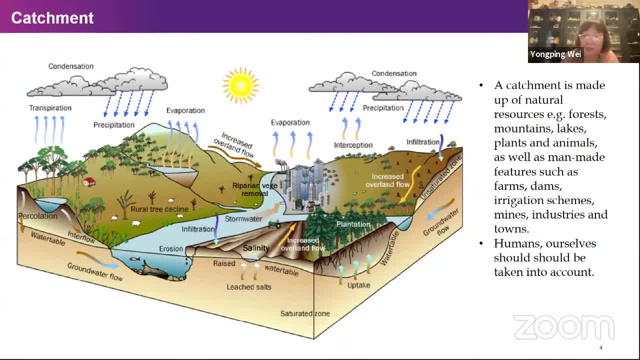 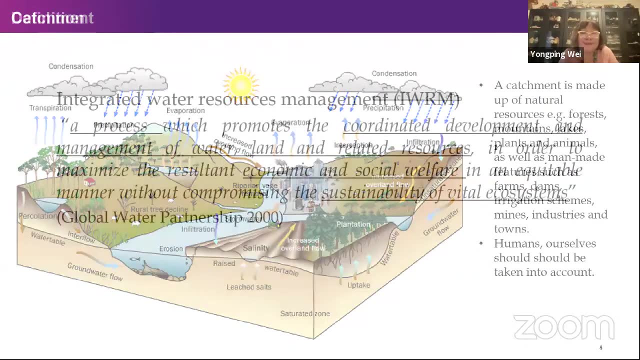 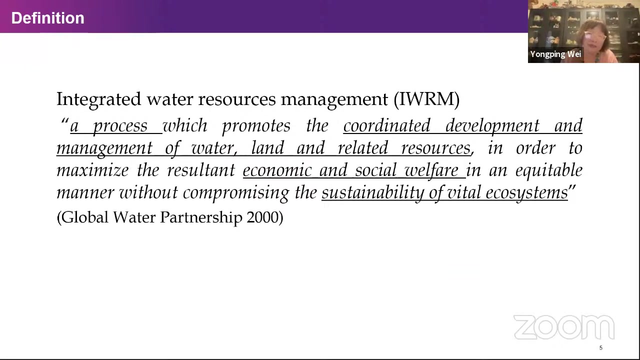 And as well as lots of man-made features such as farms, dams, irrigation schemes, industrial towns And don't forget, catamount, includes ourselves. Next slide, please, So to address this global water challenges to management of catamount, which have lots. 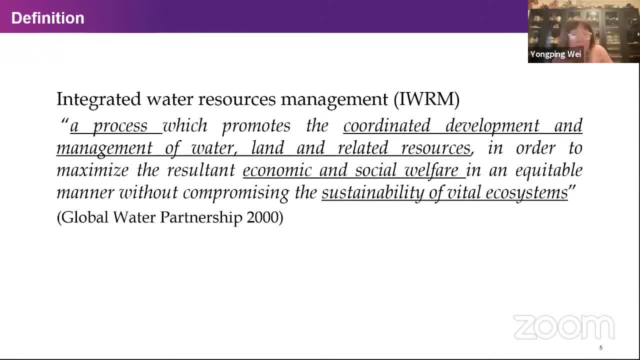 of different elements, So many, Probably 50 years ago, we integrated water resource management has been encouraged, proposed by lots of international organizations. The definition I give here is Which was be given global partnership in 2000.. It's 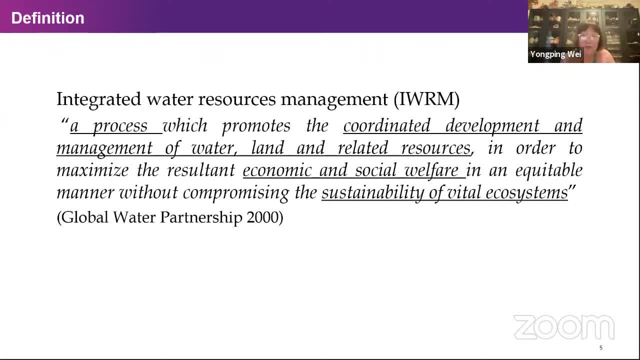 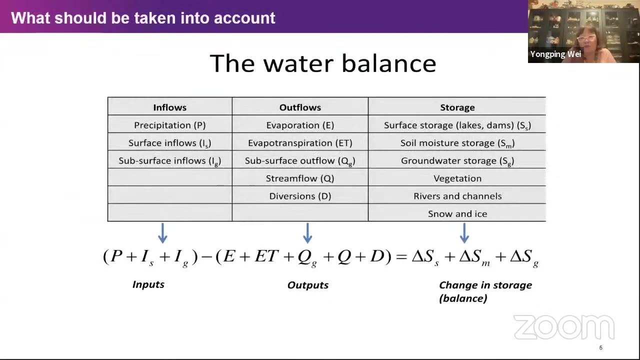 The definition here is a process which promotes the coordinated development and management of water, land and our resources to achieve social, economic welfare and environmental sustainability. So that's the key things for integrated water resource management. Next slide, please. So what should be taken into account when you do an integrated water resource management? 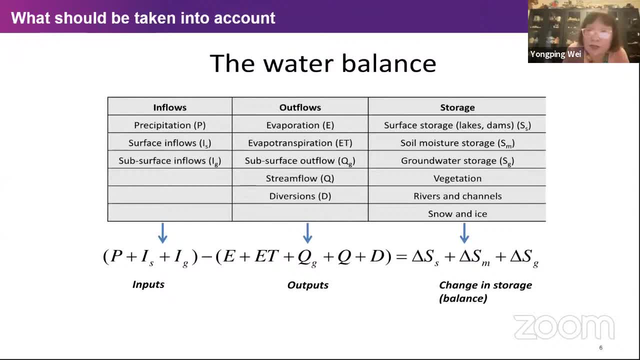 First thing is water balance. We have to know. We have to know where water come from and where water go, who use what, how much water has been used and how much water has been stored in the catamount in our lakes in. 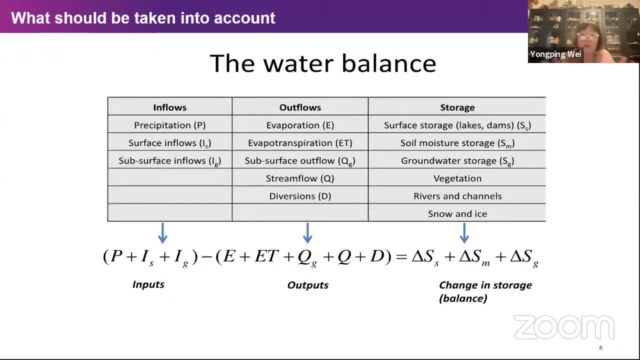 our soil in ground, in our groundwater, in rivers. So I wouldn't give too much. Introduce the equations. So first thing we have to think about when you do integrate water resource management is water balance: Where water come from, where water go. how much water has been stored in your catamount? 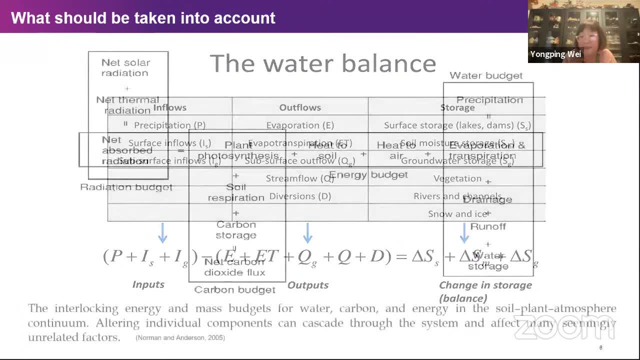 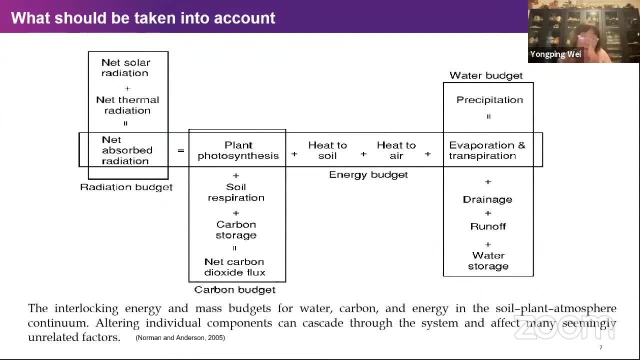 Next slide, please. So once we got a clearly understanding or clearly accounting about water resource, we have to think other resource too. In this slide, left side is water balance. That's what I introduced in previous slides. So water balance- it's connected or integrated with energy balance. 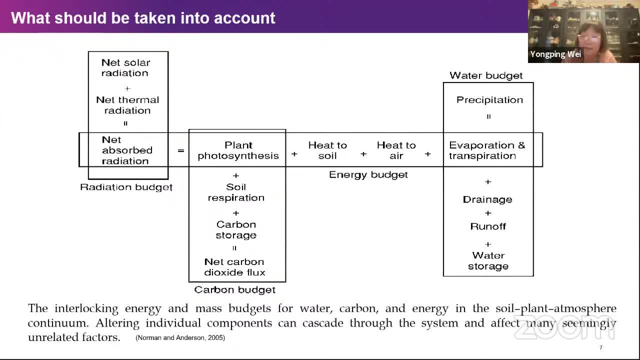 So that's energy balance. Then it's connected with the carbon budget too, Also with energy budget. So when you do the integrated water resource management, you can think about the nutrient balance, What to call it. So where nutrient come, where nutrients go, how that connect with water. 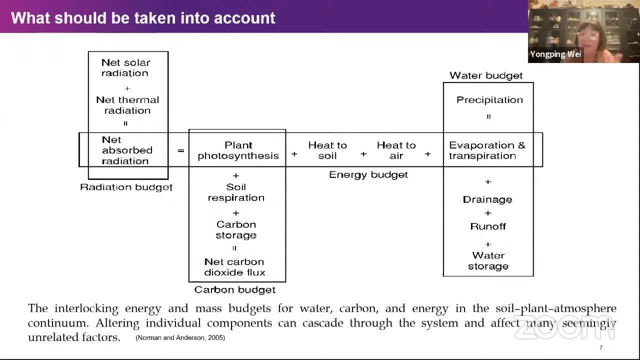 You also can think about the carbon budget. That's our hot topic now. It's climate change. So where carbon come from, where carbon go, how that connect with water. So when you do the integrated water resource management, you think of energy, budget, water. 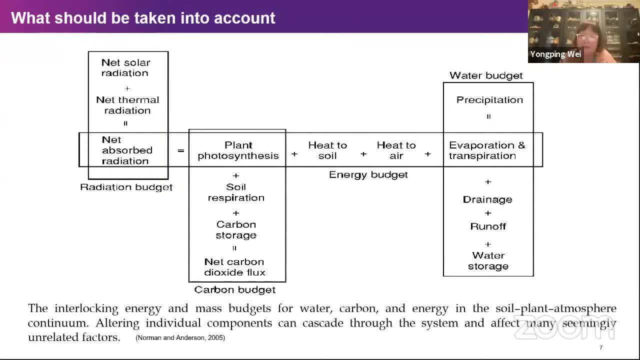 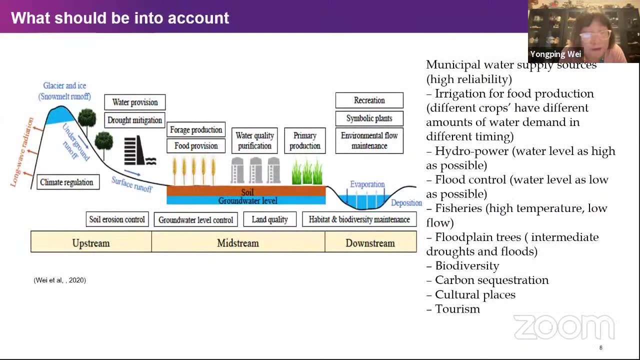 budget and carbon budget. That's all well connected. So that's why the challenge of integrated water resource management at the river basin- all well connected. Thank you, Next slide, please. So then, from the ecosystem perspective, that's the river basin fingers. 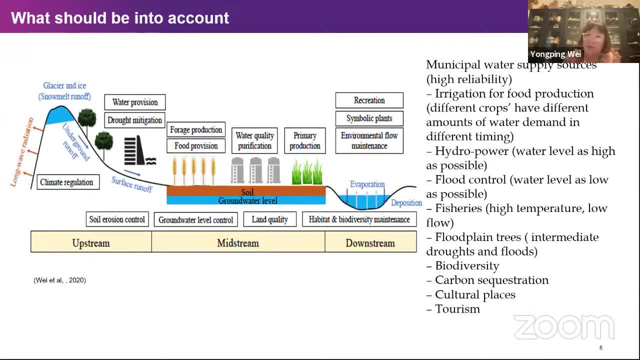 From upstream- middle stream and downstream- you have lots of ecosystem function to achieve through integrated water resource management. Normally, from upstreams we look at climate regulation and water supply. In the middle stream we try to look at water food production, water quality, water treatment. 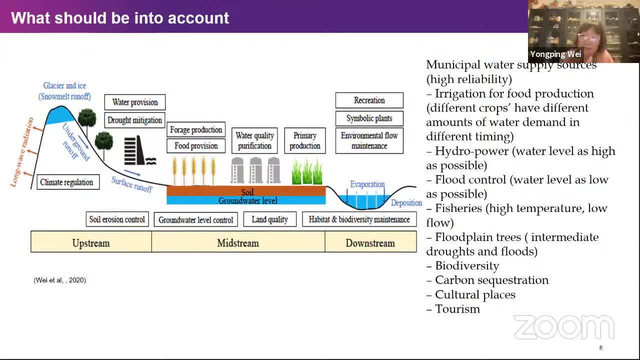 and other primary production In the downstream. we normally look at what's the environment flow and what's the other culture flows. So to management all these different ecosystem service, we need to have a very good ecosystem, Have a very good integrated water resource management plan and even dam operation plan. 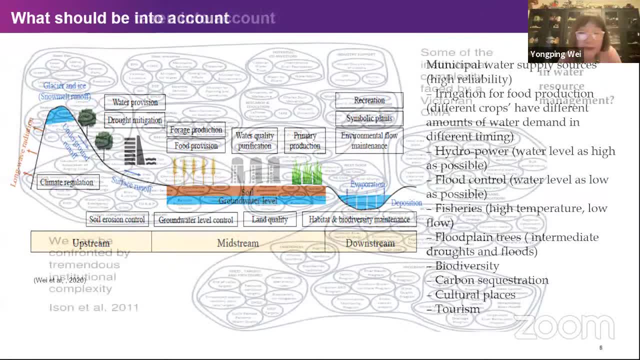 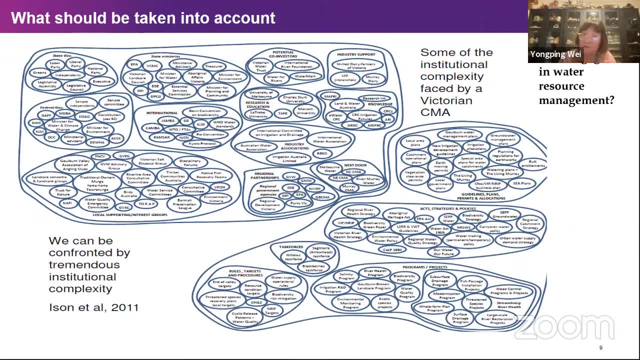 Next slide please. So what I talked before, what should be taken into account, that's from biophysical perspective. So that should be well understood or well studied. So lots of research already has been done how much, how we can do the water balance. 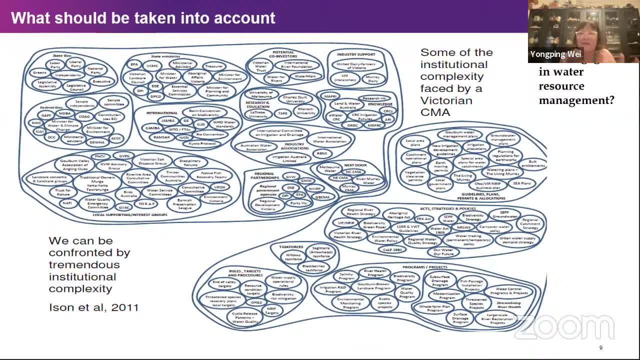 how we can integrate- think of water balance with carbon balance and energy balance, How we look at different ecosystem service. That should be well studied now. From these slides I tried to emphasize the other part of integrated water resource management, So how that could be integrated in. 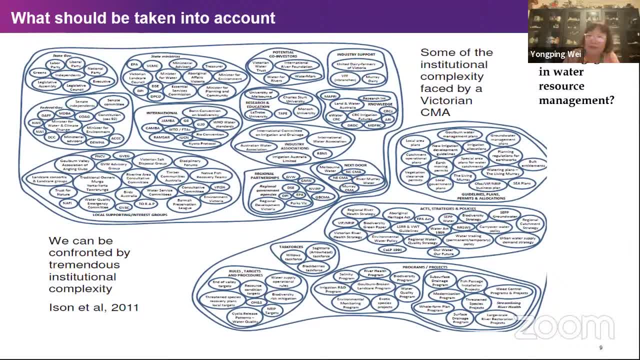 So, from social perspective, This slide here is who should be engaged in the water resource management. This is one of our collaboration project in the catchment in Victoria in Australia. In the small catchment we did lots of research, As so many groups, so many different engagement groups, has been, has been, has been engaged. 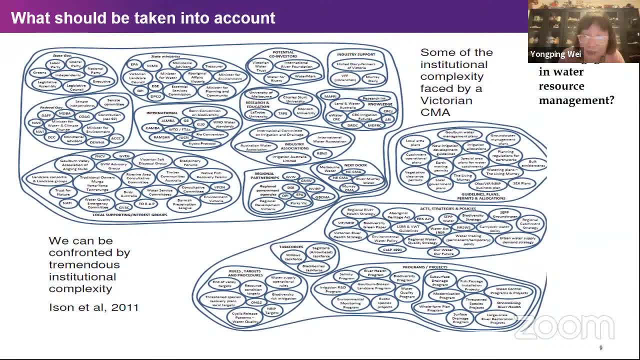 or make their influence in the catchment authorities catchment management. So I wouldn't give too much data, Too much details about this. You can clearly see so many different groups which has been included, involved in the water resource management. 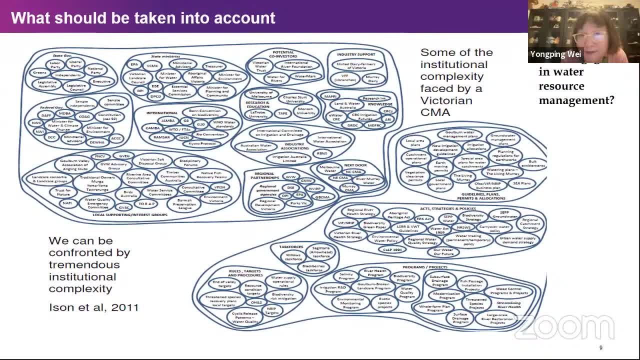 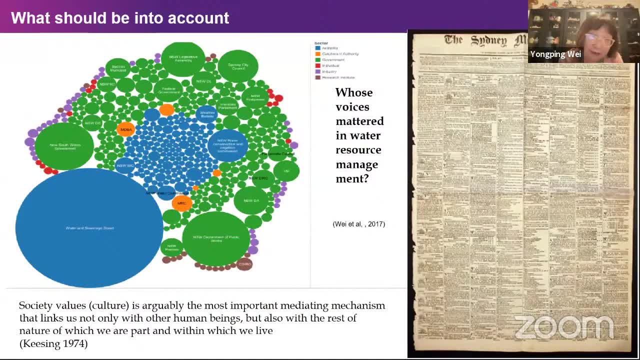 So next slide, please. That's one of our research Another PhD student did a couple of years ago, So whose voice mattered in water resource management? So that's one of our project we did So we look at this Sydney Morning Herald newspaper from 1943 to 2016.. 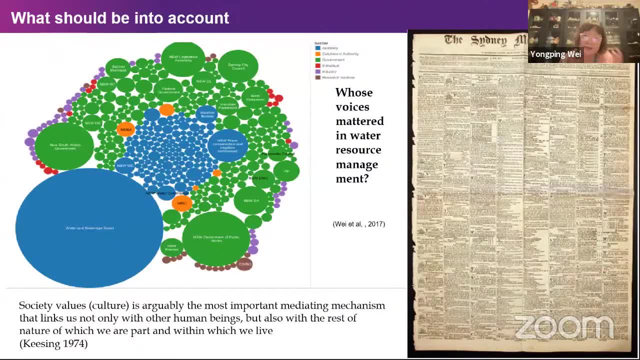 Whose voice has mattered has influenced the integrated water resource management in Australia. You can see, the blue one is government department, The green one is authorities. Even in Australia, The research of the stateholder's voice? nearly nothing, You know. that surprised me. 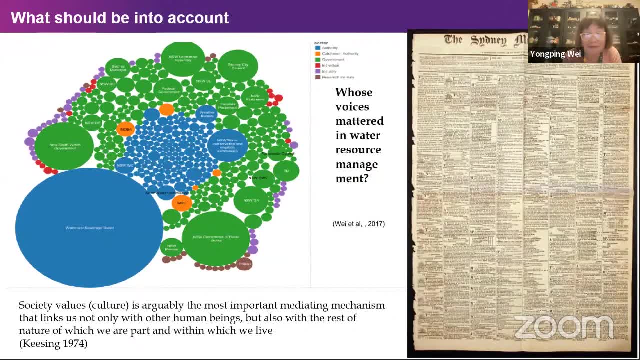 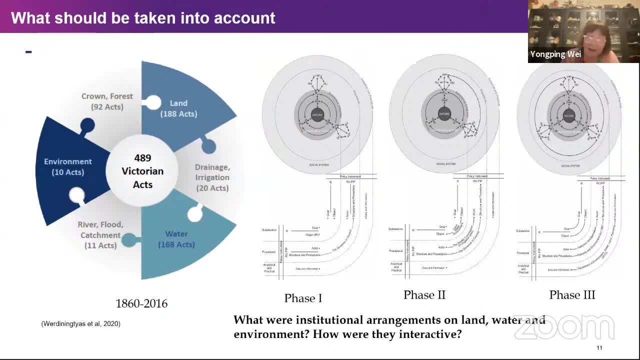 Anyway. so that's Next slide, please. So another very important social factor is the institutional arrangement, The law, regulation and other informal organizations of governance. That's work which has been done by rights, Actually fantastic work. Through her four years PhD she invested all Victoria Act 489, Victoria Act on land and water and environment to understand in different phases which kind of act has been involved in the integrated water resource management. 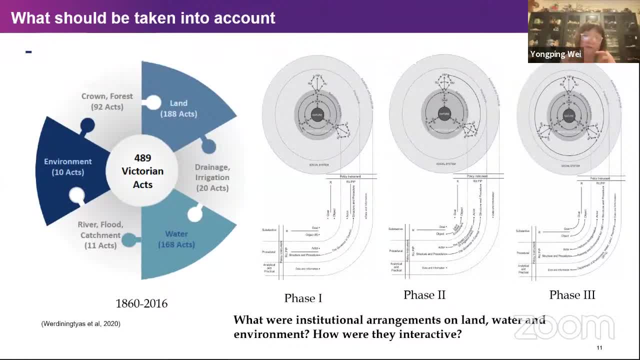 How were they interactive? So it's fantastic work, I think actually. well, We'll talk this later. So I'm proud of her research. Through four years research, she has fantastic findings in this area. Next slide, please. 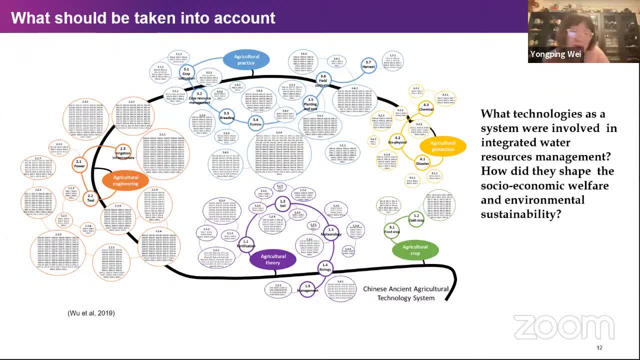 So technology is another very important part for the integrated water resource management. So because technology can shape both the social, economic and the economic And environmental sustainability, That's one of my PhD student did. That's a Chinese case. She look at over the last 8,000 years which kind of technology, how they work together as a system to influence the integrated water resource management. 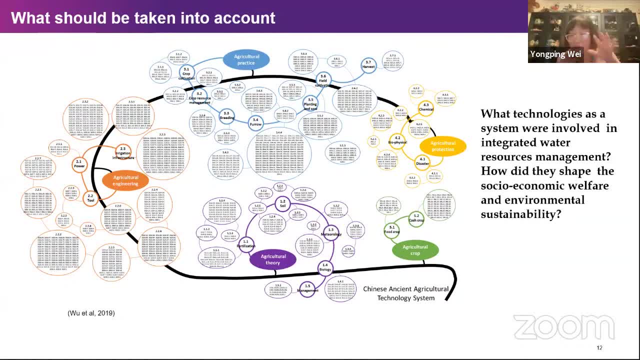 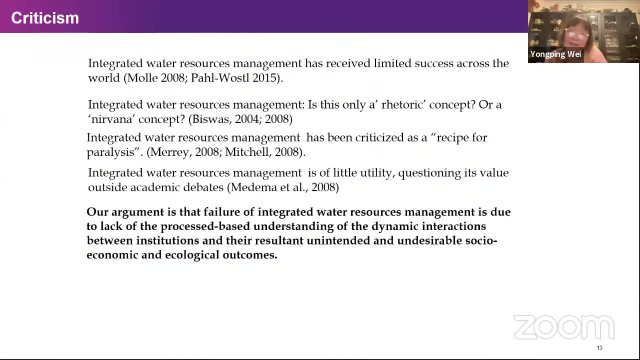 I wouldn't give you too much details, Just show you that's quite important for integrated water resource management. Next slide, please. management, Next slide, please. So look, so many things we have to take into account when you do integrate water resource management, from biophysical science, from laws and from. 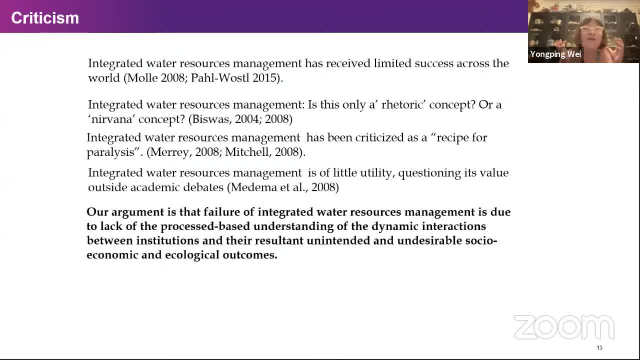 social science We have this, this stuff, how these factors can be integrated together. So so far we haven't had a good approach. So that's where lots of criticism come from. I just copied just a side couple of conclusions: Basically integrated water resource management. 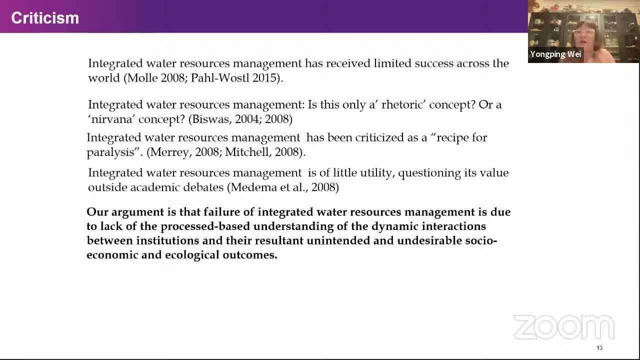 have received limited success across the world. So people start to doubt: should that's only a concept or academic interest? Everything wouldn't have any real application or real influence in the catchment management or integrated water resource management. So I put our argument. here is: our argument is: 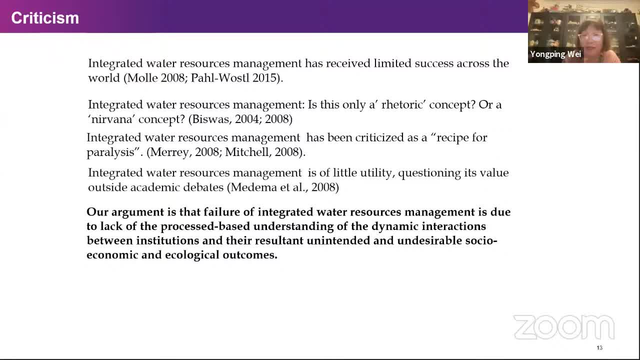 the failing of integrated water resource management is due to lack of the process-based understanding of the dynamic interaction between different subsystems. So that's it, Thank you. Next slide please. Next slide please. Our argument: we don't have the process-based. 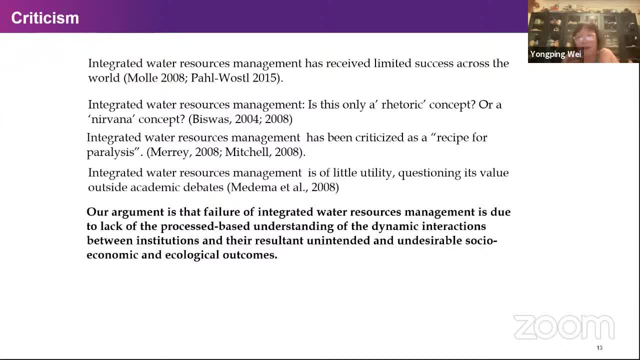 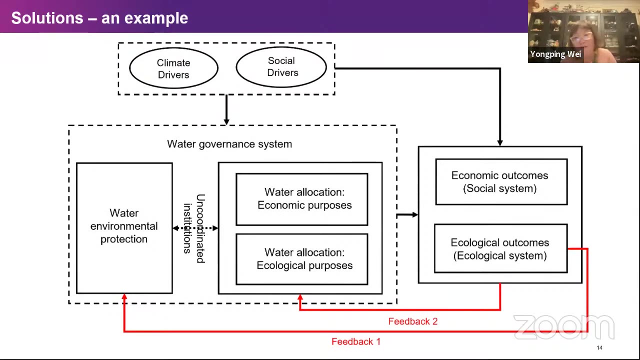 understanding, In other words. so lots of social factors has not been quantified, Cannot be integrated with the biophysical process, mostly, so we couldn't have the process-based understanding. Next slides: please, Okay, I just use one of our recent ads. Next slide: 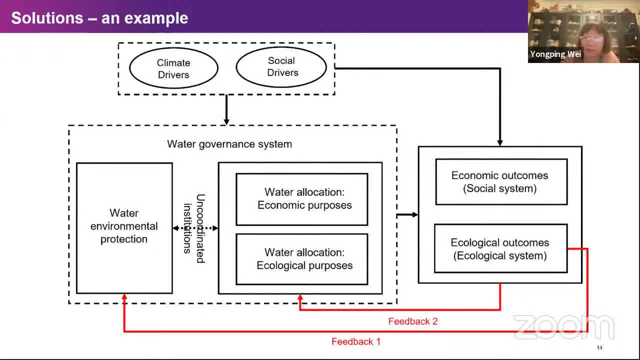 please. Next slide. Okay, I just used one of our recent ads. Next slide, please, Okay. project to to demonstrate how we can do this process based on standing. that's the master works. paulina just finished, uh, research it. she trying to understand, you know, in the 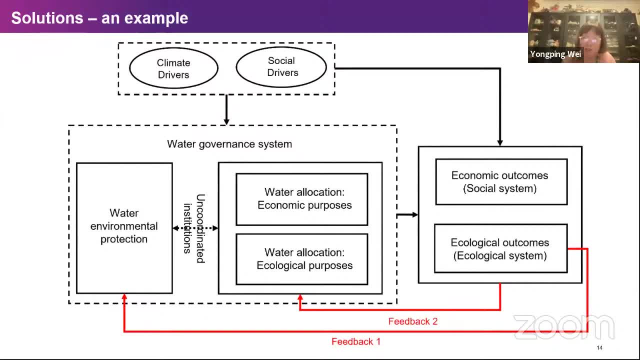 integrated catchment management. we have the major two function once what? environment protection, which means it's the other ones, water resource management. this normally is the management, the management, different authorities, like in australia, china, so water resource allocation is meant by minister of water resources. so what quality and what environment has been managed by? 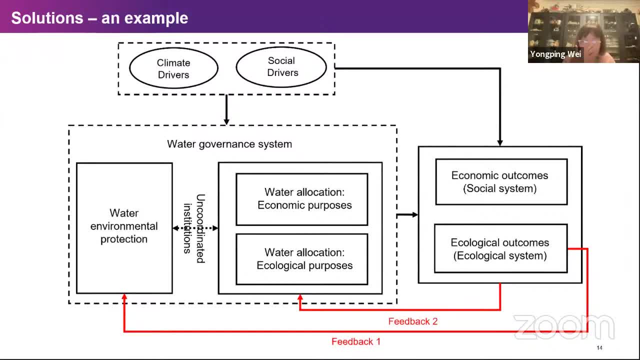 environmental protection, minister of environmental protection. so that's they have a very weak coordination. so so what resource, what resource management aim to to achieve economic outcomes and ecological outcomes? what environment protection achieved to the better ecological outcomes? so that's hardly connected. each other, coordinate each other. it's not only australia, china, it's global issues. so we're trying to understand if we build. 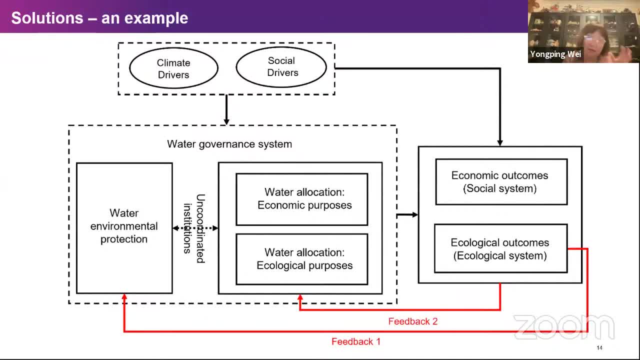 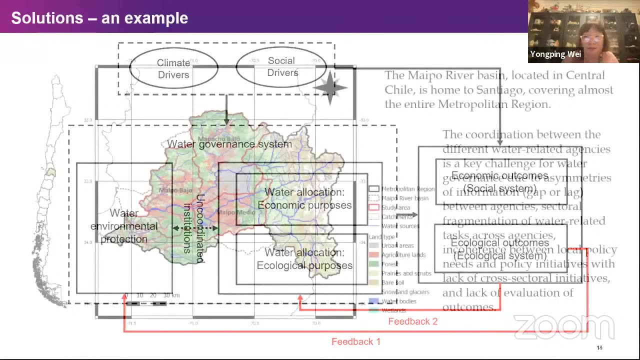 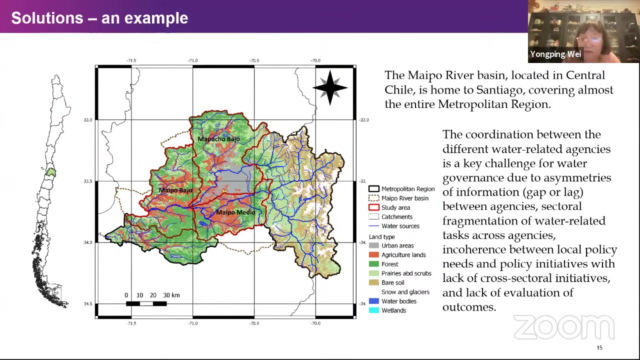 these relationships between the outcomes and the management authorities. so to uncover these issues. so if what involved protection management and what resources matter, if they separately or weekly coordinated management, what would happen? so that's a conceptual model here. next slide, please, thank you. so paulina is as examples, that's maple river is in the central chile as an example to investigate these issues. 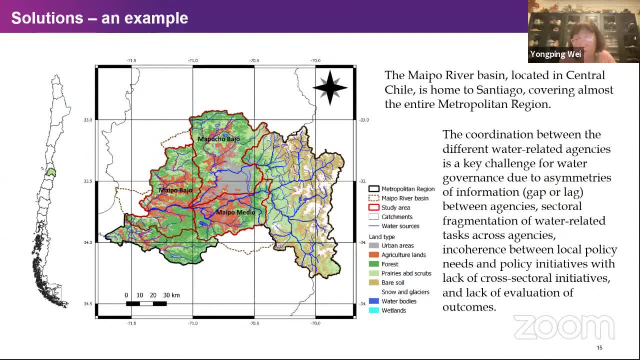 so maple river is one of the hot pot, hot topic in integrated water resource management globally. they have a lot of global agencies work there. so the major, major issues is they have a fragmentation of water related agencies and their water resource management and water quality management never be coordinated together. next slides, please. 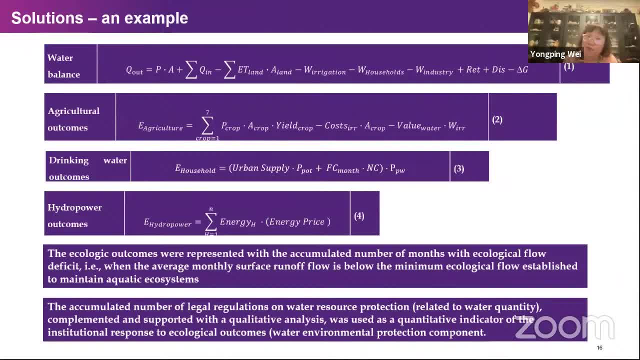 what we did here is, like i said we do, we build the water balance model, so where water come from, who is used and how much water has been used by different uses. that's we build the first water balance model. i think that's a that's a fundamental step to do integrated water resource management now. 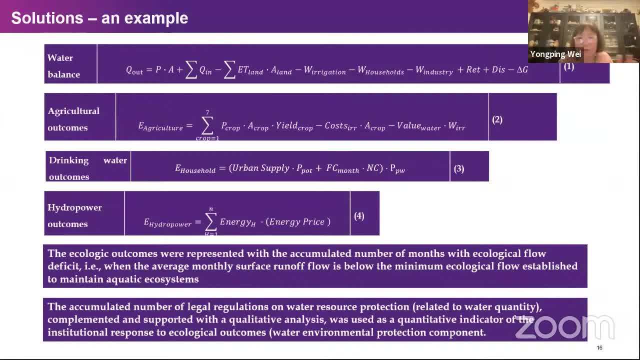 we build some economic model. what's agriculture outcome model? so how much water has been used by agriculture and what's their uh benefit? when then we suddenly we did the drinking water model and hydropower model later we have ecological outcome model. so if this much water has been used, how that has been. 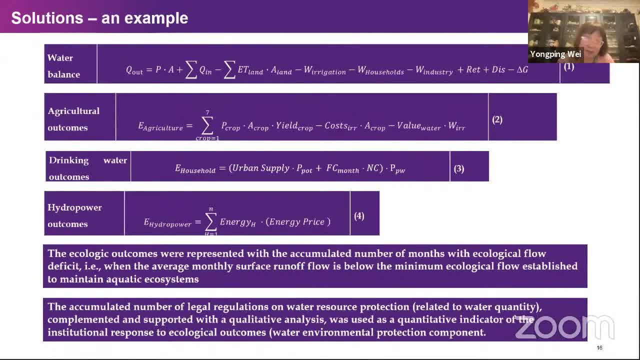 affected by factor. affected the ecological outcomes. here we just use the accumulated numbers of mass as the ecological representative indicators. then the last part is we look at the last 50 years of the water and how much the water has been used and how much the environmental regulation is. 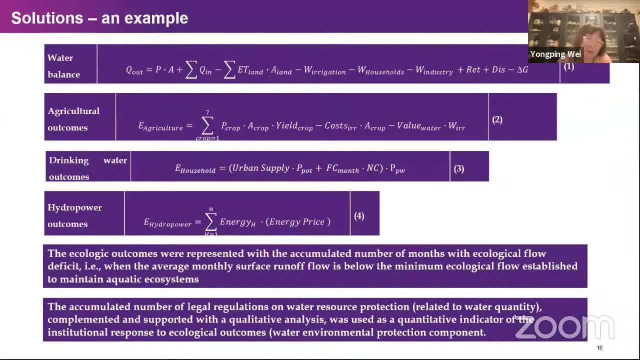 affected by that. so we need to look at the last 50 years of the water and how much environmental regulation has been made and what's the influence, influences and what's the themes about that. now we quantify, quantify this legal regulation, then later we try to integrate this with the our 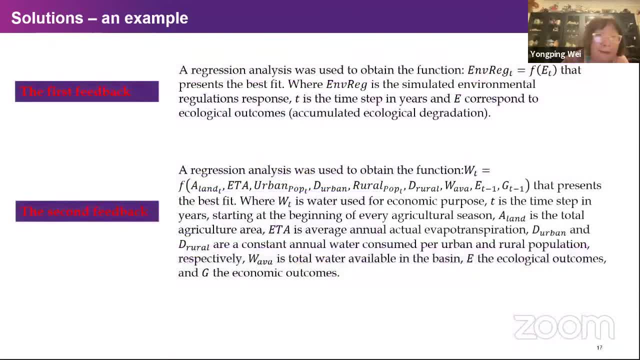 biophysical models. so next slide, please. So then we have two hypothesis of this first feedback and the second feedback that I try to understand. if these two agents didn't work together, what would be the outcomes? So I have the two equations. The first equation I try to understand: what's the relationship between environmental regulation and environmental ecological outcomes? 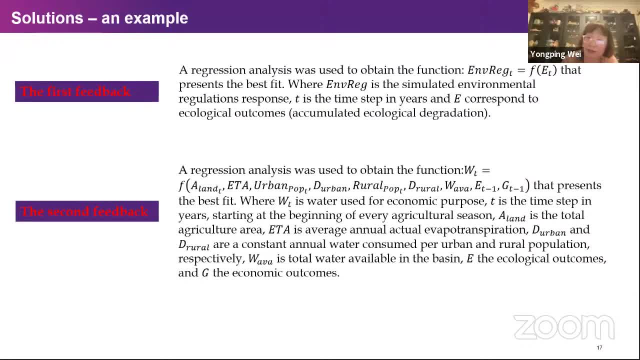 Second equations are trying to understand what's the water resource allocation, What variables should be taken into account when doing water resource allocation? So we look at the land area, look at the population, look at the population, look at how much water has been used, what's available? 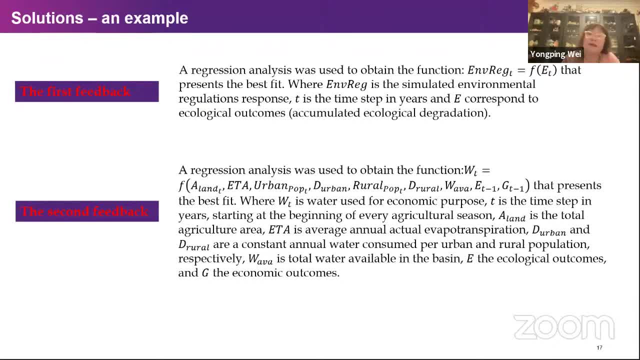 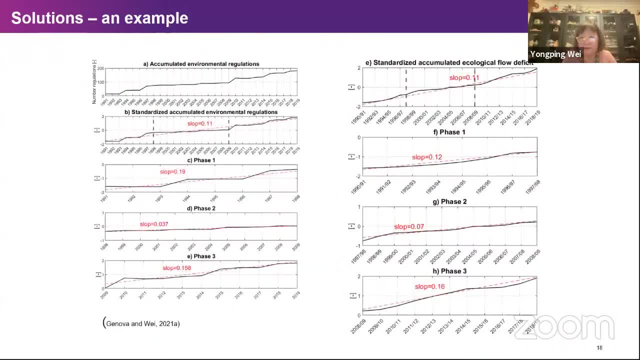 So what's the ecological outcomes and what's the economic outcomes? Next slide, please. So through this project we have lots and lots of results. Here I just show one part of the results. So left side, that's the environment regulation results, how environment regulation has been. 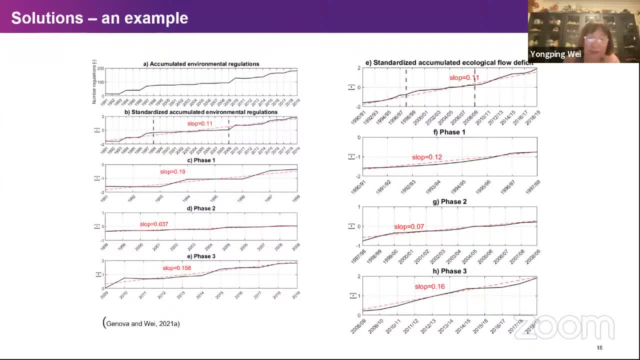 involved in the last 50 or 30 years On the right side is how ecological outcomes, environment flow, has been involved in the last 30 years. So if you have left side fingers, right side fingers, can build the equations between the equations between response of professor. you have one minute. 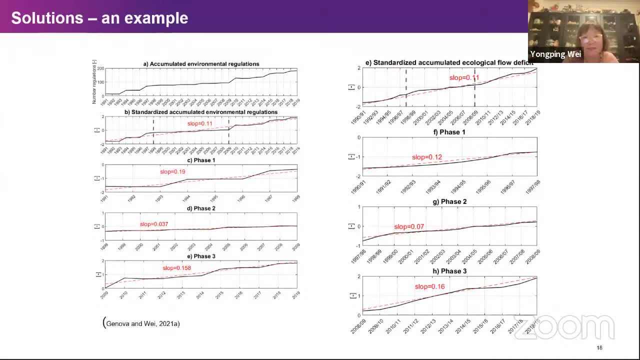 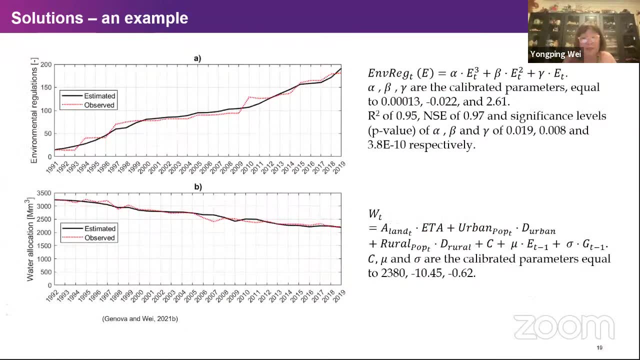 okay, i finished it one minute. yeah, okay, thank you. so next slide, please. yeah, so that we build these two equations. these equations to tell how environment regulation to response to the ecological outcomes. second curves is how water resource allocation responds to to the economic outcomes and ecological outcomes and other populations here. 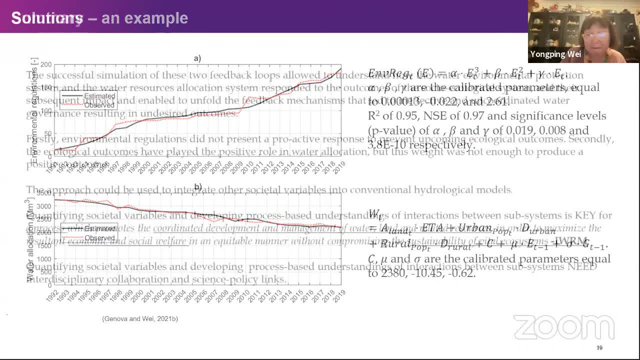 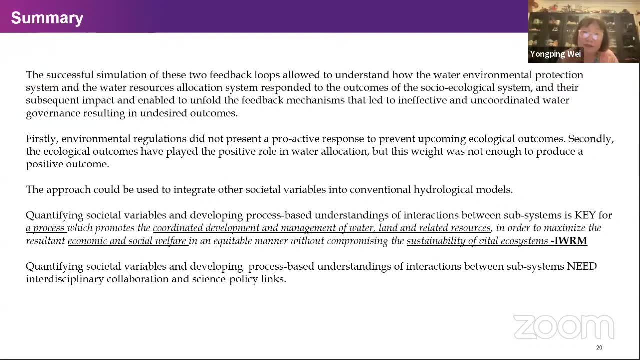 next slide, please. so with this successful simulation of these feed banks, that's very important to feed when it allows our to understanding how what environment protection and water resource allocation responded to the outcomes of the social acre, social ecological systems, to that's to enable us to unfold the feedback mechanics that's led to if 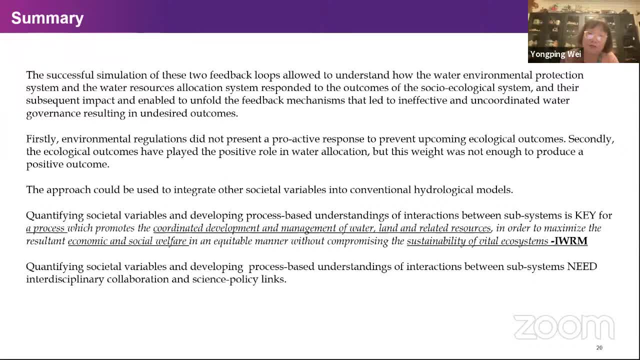 ineffective and uncoordinated water governance, resulting in the undesired outcomes. so this this can in this case is environment regulation didn't print present a proactive response to to the to ecological outcomes. so in the water resource allocation didn't have enough f size to the ecological outcome. so this pro, this project, this approach could be used to. 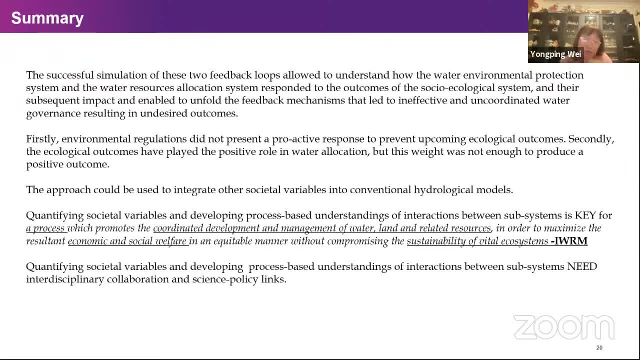 integrate other social verbs into traditional hydraulic models. so quantum, آBBII, social society variables and developing process based understanding of interaction between different systems is key for integrated water resource management, because all integrated water resource management is process based actions. if we have a process based outstanding, we could this: 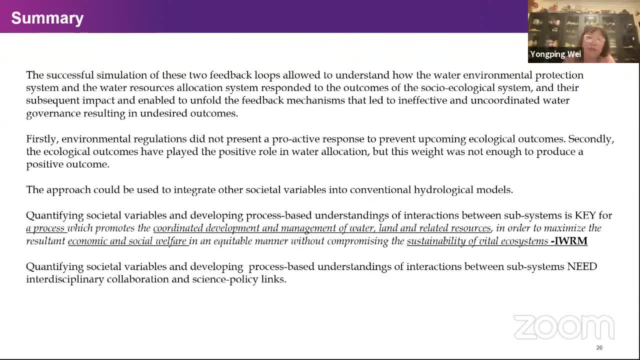 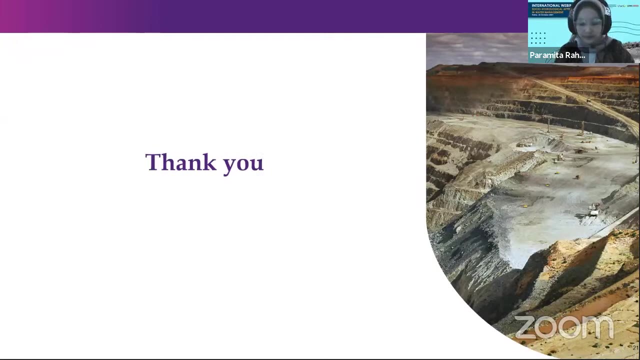 support is process based actions, so quantifying social society variables and developing process space outstanding need interdisciplinary collaboration and the size policy links. thank you. thank you very much, professor yongping way. if i may try to like conclude several important points your presentation is about: uh, is what the resources? 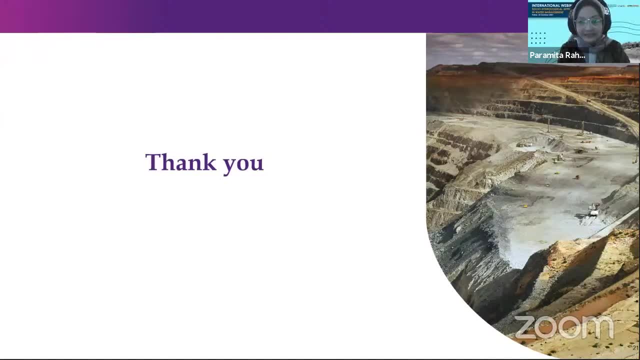 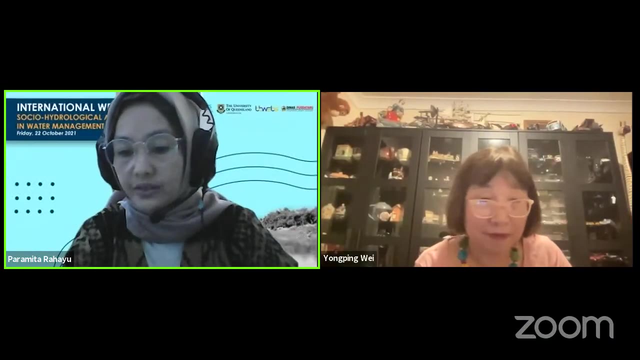 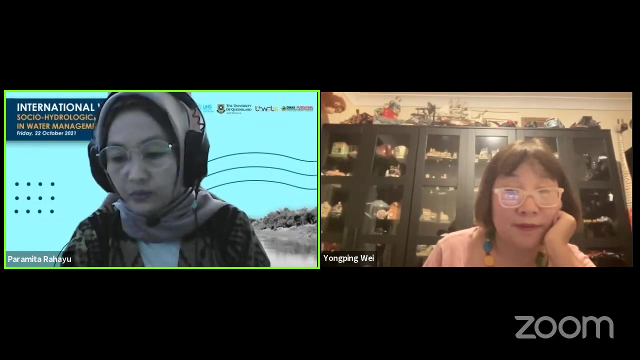 management possible or is? is it a rhetoric? so you point out that water resources management is a concept that combine social values, institutional arrangement related to regulations on land, water environments and also the role of technology as a system that influence integrated water resources management. but there are many criticisms about this concept and you 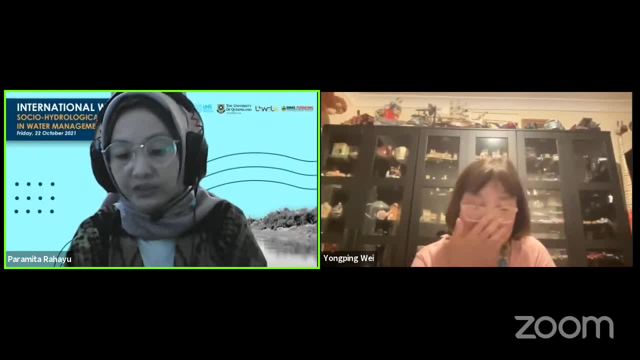 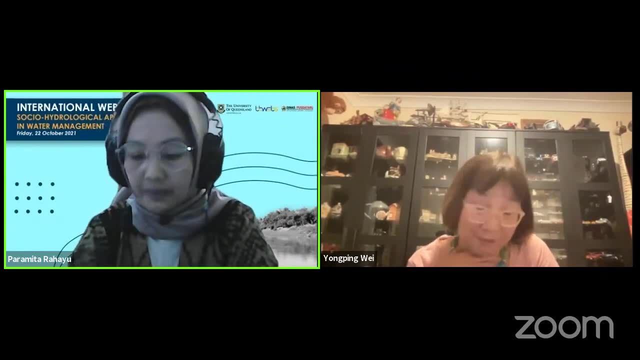 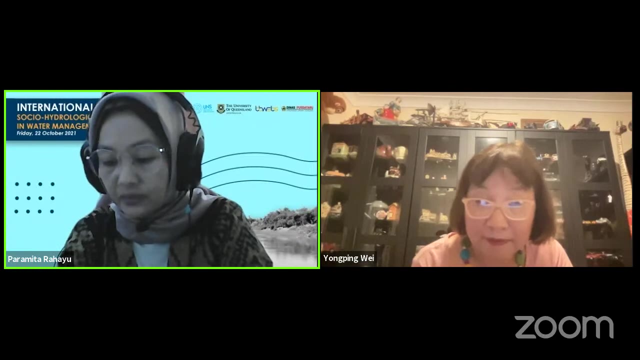 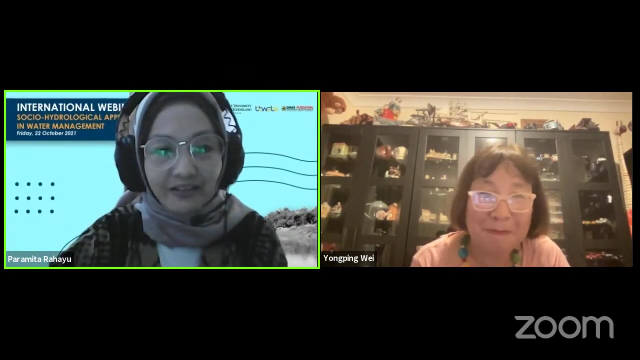 provide, suggest solutions to this criticism of water resources management by using the combinations of water resource management and water quality management in a system of water allocations for economic outcomes and water allocations for ecological outcomes. yeah, thank you very much. this is very interesting and elaborated, the presentations. uh, and now we will go. 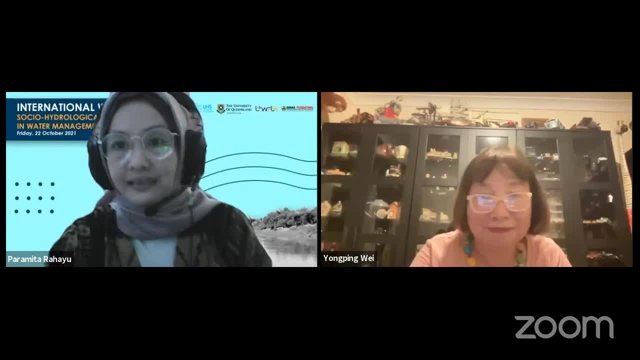 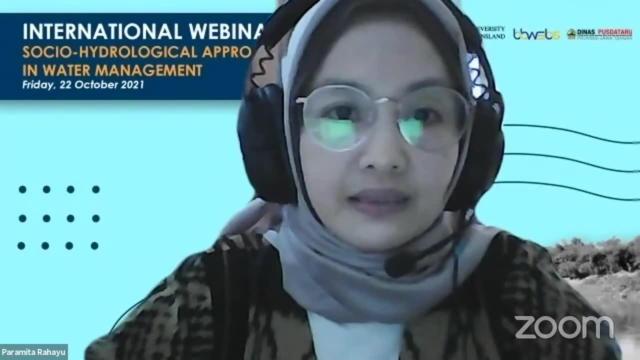 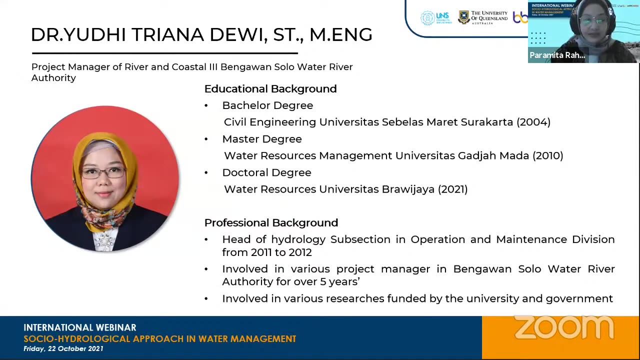 uh third speaker. i think uh, our third speaker will be uh dr uh yudi triana dewey uh. she has bachelor degree from musical engineering, master degree in water resources management, mada, and doctoral degree in water resources research at university of korea, and she is currently the project manager of river and. 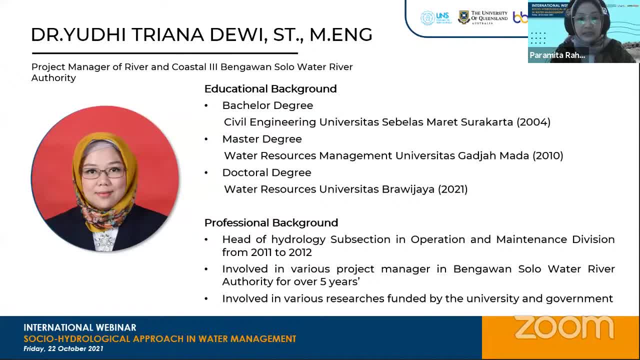 coastal bakawan solo river authority and she involves in various project manager in bakawan, so also involved in research, many research funded by the university and the government. and i would like to welcome uh our speaker, dr yudi diana dewey, that she will talk about the river basin. 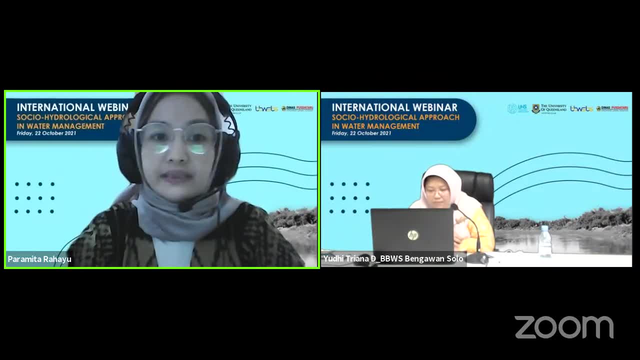 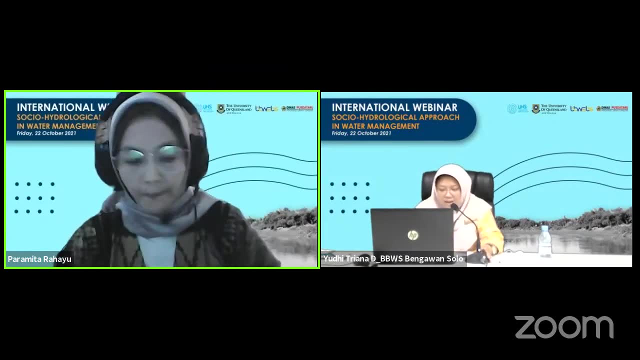 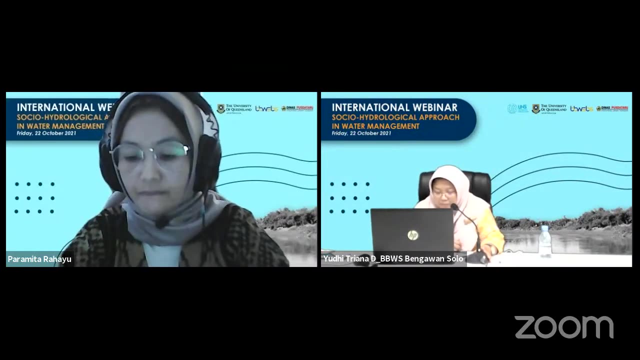 Management Challenge to Manage Biophysical and Social System Interactions with Case Study Bengawan-Sololifor. Please, Ms Yudi. Assalamu'alaikum, warahmatullahi wabarakatuh, Ladies and gentlemen, Your Excellency, Prof Solihin Asad. 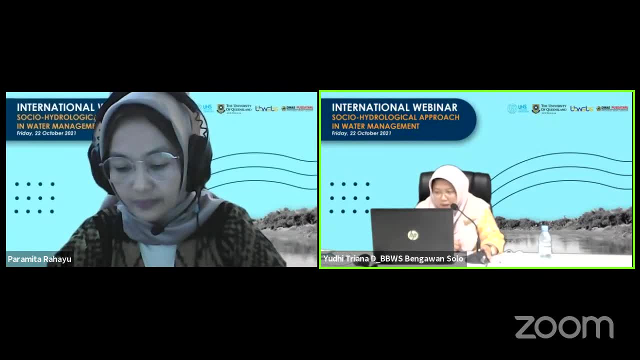 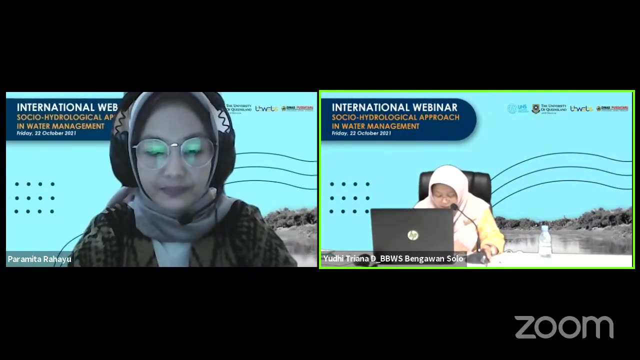 Ibu, Prof Rwini Astuti, and distinguished speakers Prof Yongping Wei, Dr Frederick Bogert and Bapak Eko Yunianto, and also Ibu Ratriwerdi Nintias, PhD. This afternoon I'm representing my head of PBWS, Bengawan Solo. 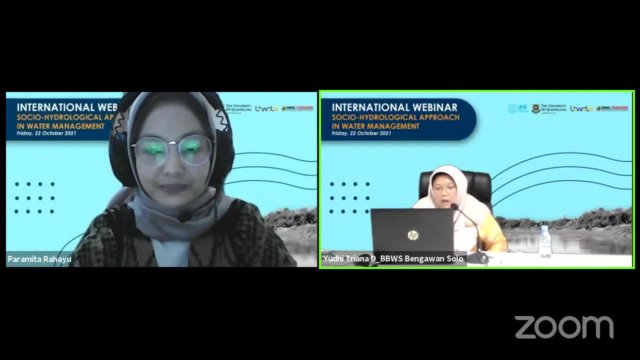 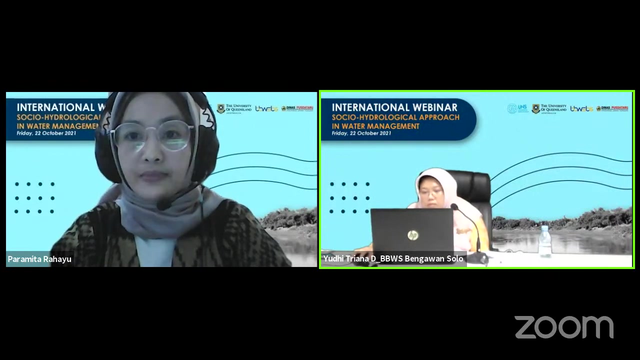 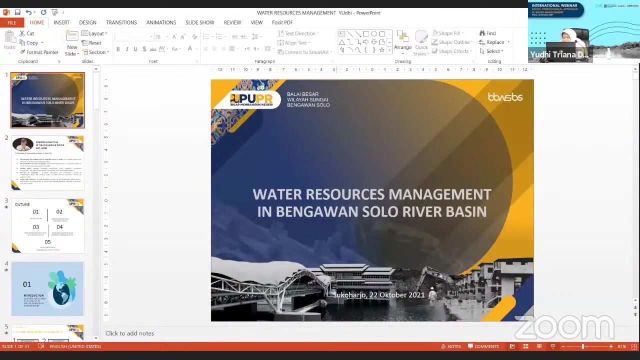 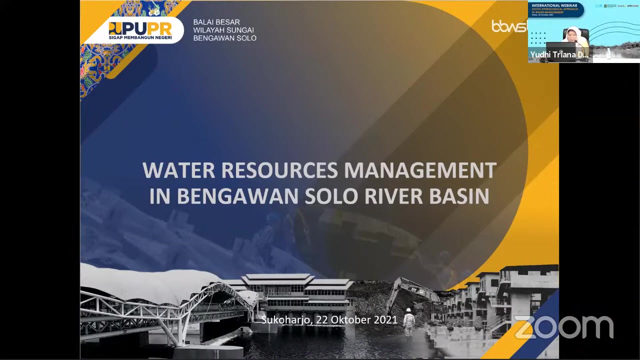 Bapak Dr Agus. He is not available now because he is in Jakarta for some agenda And, excuse me, I can share my screen. please Di overhe atash Jakarta. Now we gonna start the Denise and Fatheraitud together awareness. 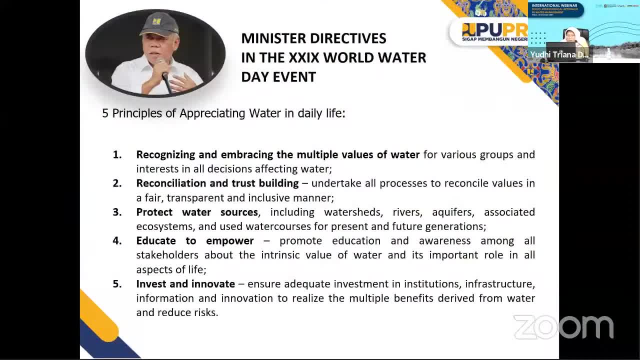 gathering ceremony. Before I start my presentation today, maybe I want to remind us our Minister of Public Works, Bapak Basuki Hadi Mulyono, 5 principles in appreciating water in daily life. First is First is recognizing and embracing the multiple values of water. 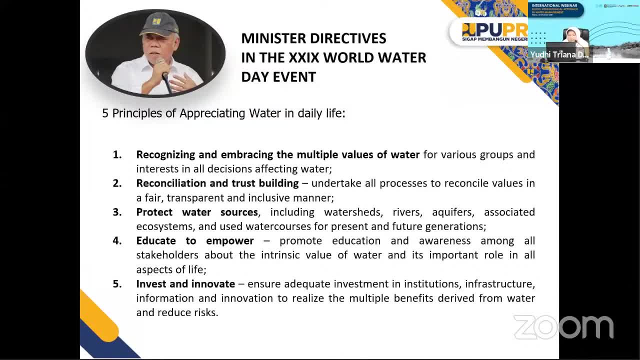 Second is reconciliation and trust building. Third is protect water resources. And fourth is educate to empower. And five is invest and innovate. These five principles, hopefully, can be implemented in our river basin in Bengawan Solo. Okay, today I divide my presentation into four parts. 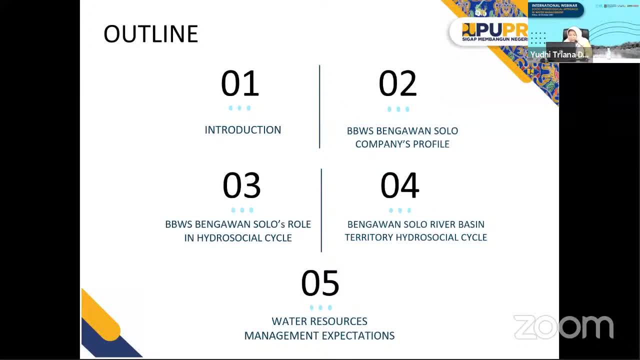 Introduction, Bengawan Solo company's profile and BBWS: Bengawan Solo's role in hydrosocial cycle And Bengawan Solo river basin territory hydrosocial cycle. And the last is water resources management expectation. Okay, introduction. 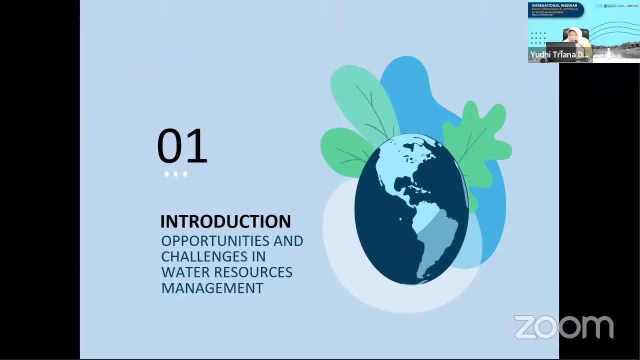 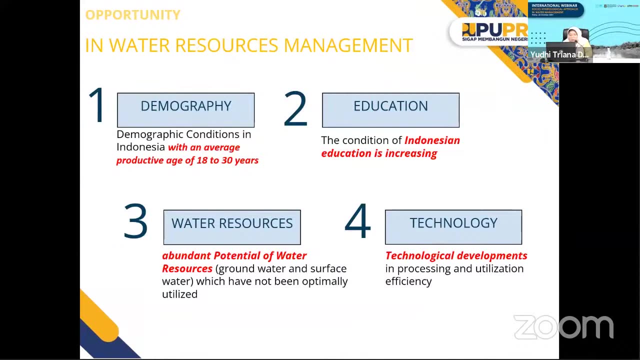 Opportunities and challenges. What are the challenges in water resources management? Actually, we have opportunities in Indonesia right now. Our demographic condition in Indonesia, with an average productive age of 18 to 8 years, And the education- The education is increasing And the water resources. 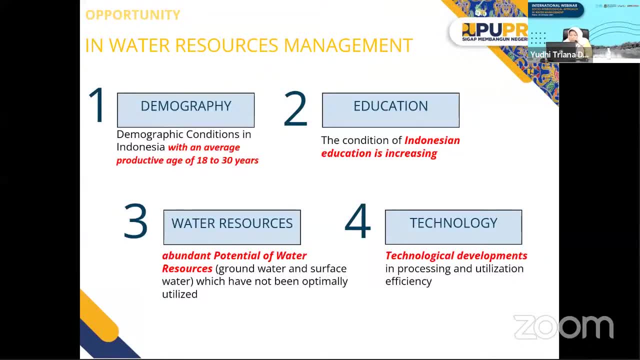 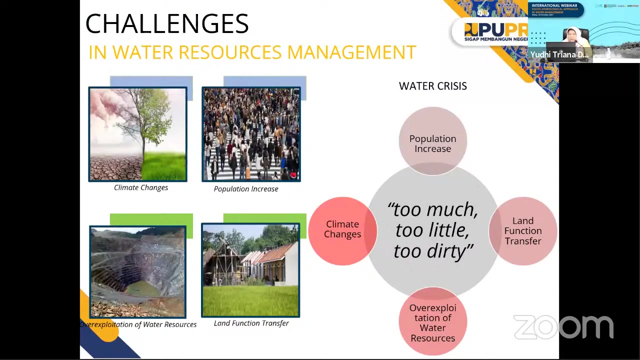 There are abundant potential of water resources On water and surface water which have not been optimally utilized. And the fourth is technology: Technological developments in processing and utilization efficiency And our challenge. Actually, there are four parts Or four challenges. First is population increase. 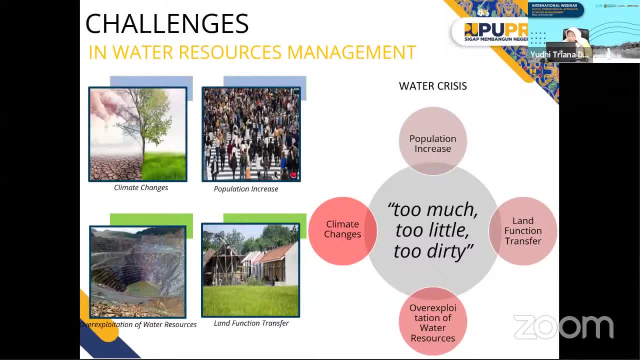 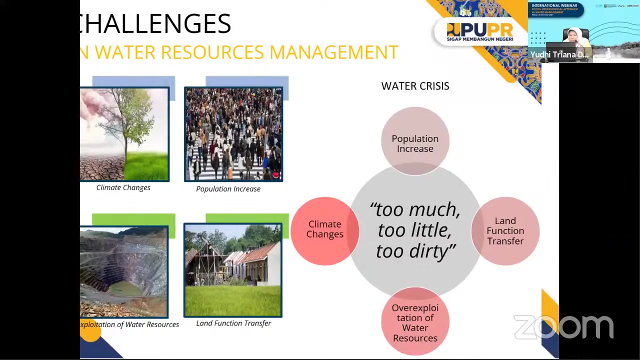 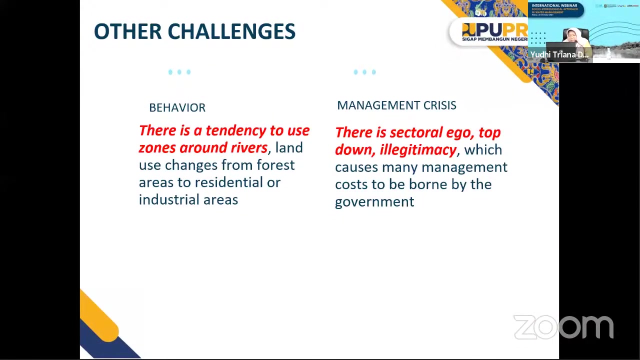 And land function transfer. and the third is over exploitation of water resources. and the third is climate change. These four components causing three. two: first is too much water, second is too little water and the third is too dirty water. Unfortunately, there are still two problems. First is behavior. There is a tendency to use 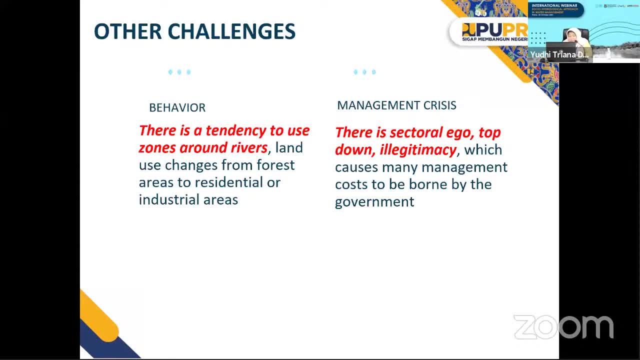 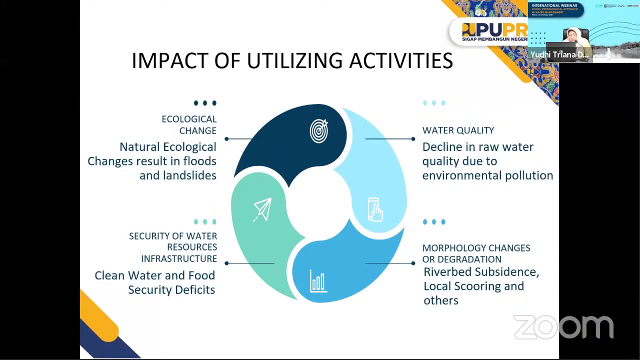 zones around rivers, Land use changes from forest areas to residential or industrial areas and there is management crisis. There is sectoral ego, top-down approach, illegitimacy, which causes many management posts to be borne by government. The impact of utilizing activities, The ecological changes. 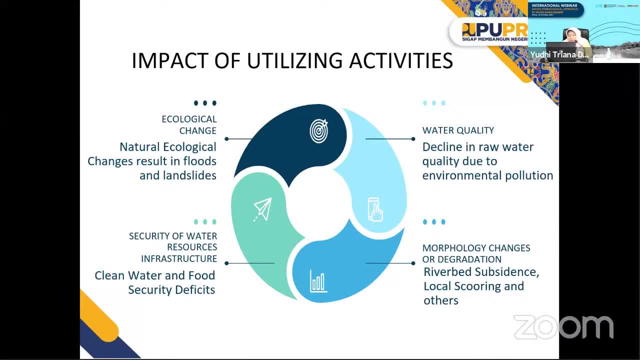 Natural ecological changes results in floods and landslides In water quality, decline in raw water quality due to environmental pollution and morphological changes or degradation, riverbed subsidence, local scoring and others, And security of water resources, infrastructure, clean water and food security deficit. 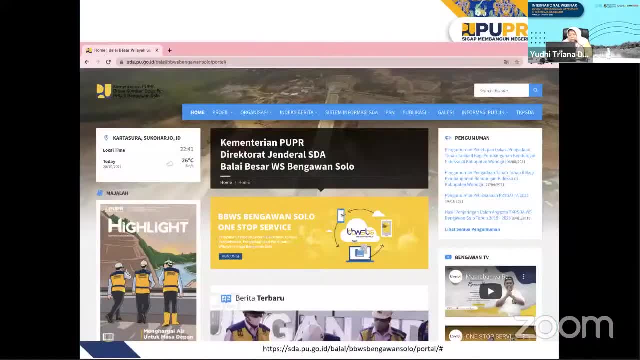 Second part, our profiles. Actually, BBWS Bengawan Solo have already existed for many years and we are really concerned in our information technology. You can access all about BBWS- Bengawan Solo activities in our website. You can access all about BBWS- Bengawan Solo activities in our website. 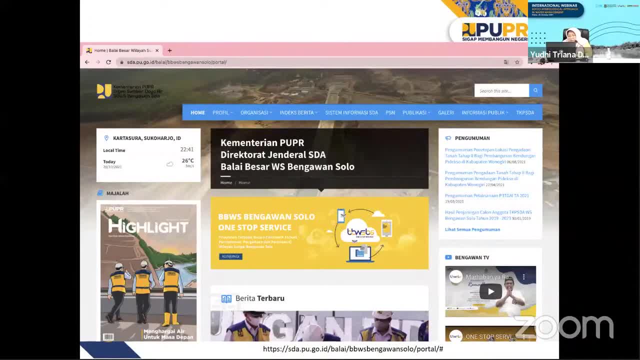 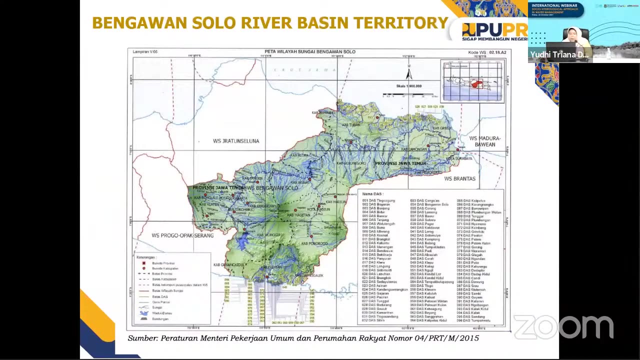 And you can share all of your opinion in here and you can give us some suggestions or many recommendations. Okay, Bengawan Solo River Basin Territory based on Minister Legitimacy Number four- The Largest Water Basin Territory in Indonesia. In 2015,, we have 96 water set spreading along the river basin. 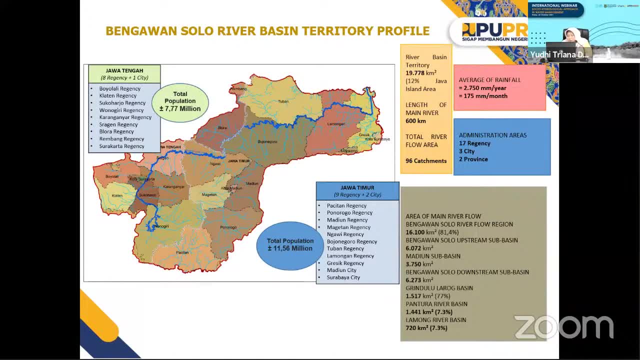 And Bengawan Solo River Basin have 19 km2.. It is about 12%. the area of Java Island of the main river is about 600 kilometers and the river basin divided into six sub-basin. First is Bengawan-Solo river flow region. second is Bengawan-Solo upstream and Madiun sub-basin. 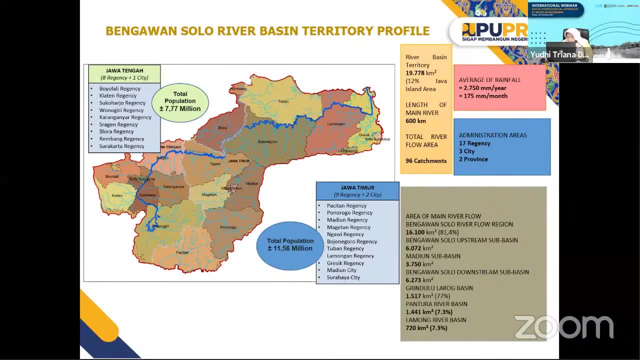 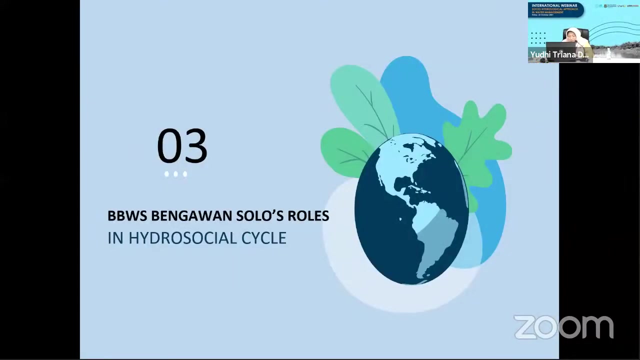 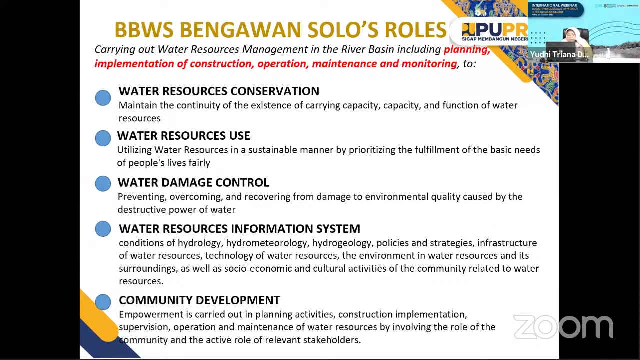 Bengawan-Solo downstream sub-basin, Grindulu-Lorok, Pantura river basin and Lamong river basin. There are two provinces over the Bengawan-Solo river basin, seven regencies and three cities. BBWS Bengawan-Solo carrying out water resources management in river basin. implementation of. 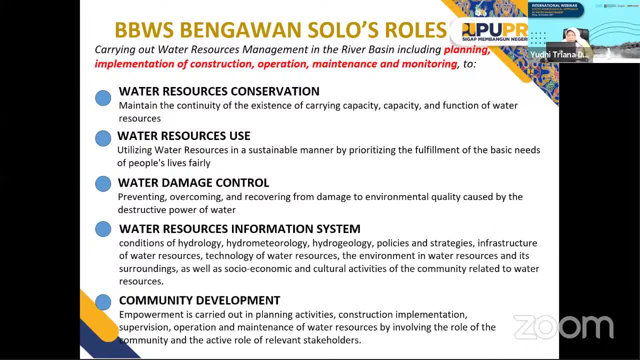 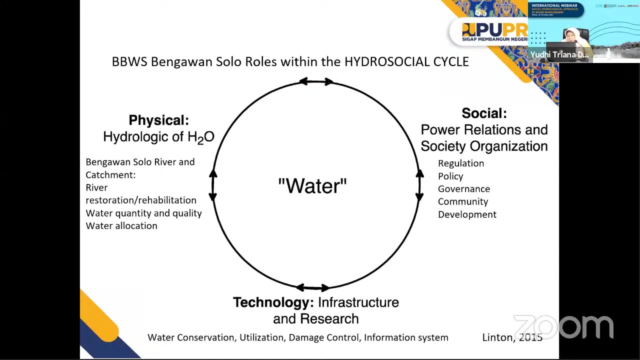 construction, operation, maintenance and monitoring. Two: first, water resources conservation. second, water resources use. third, water damage control. and fourth, water resources information system and community development. BBWS- Bengawan-Solo roles within the hydro-social cycle based on linton 2015.. There are three. 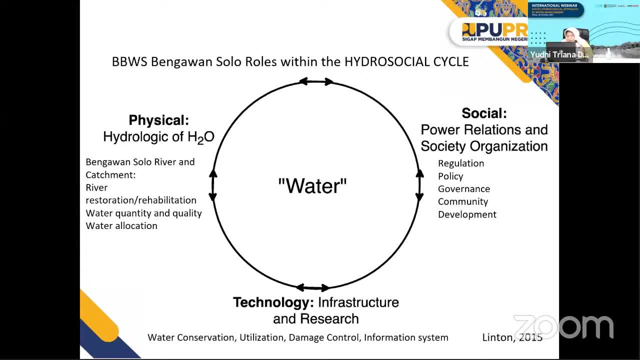 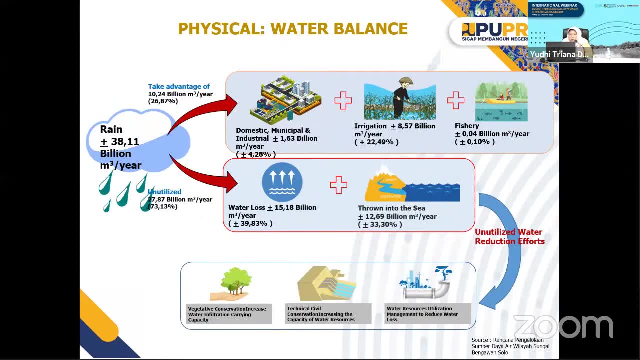 components of the hydro-social cycle based on linton 2015.. There are three components of the hydrosocial cycle. there are physical component, social component and also technology. Bengawan-Solo river basin have huge potential. Right now, there are only 26.8. 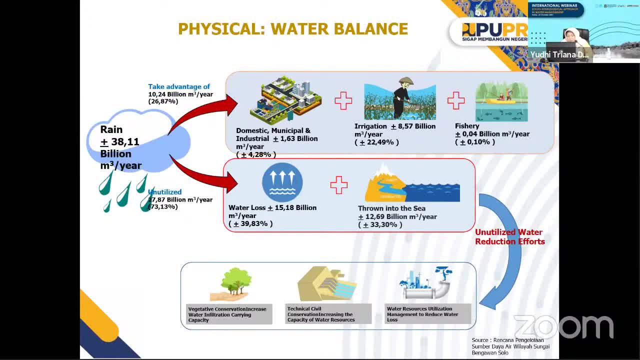 that are utilized. It is used for domestic, municipal and industrial. The portion is 4.2%, For the irrigation it is 22.49% and for fishery 0.1%, And 73.13% is unutilized. 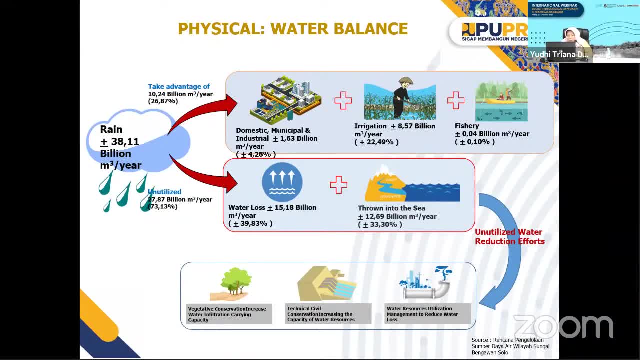 39.8% being lost and 33.3% throwing it to the sea. To reduce the unutilized water, we do some efforts, For example, vegetative conservation. Second, it's about technical civil conservation And the third is water resources utilization management to reduce water loss. 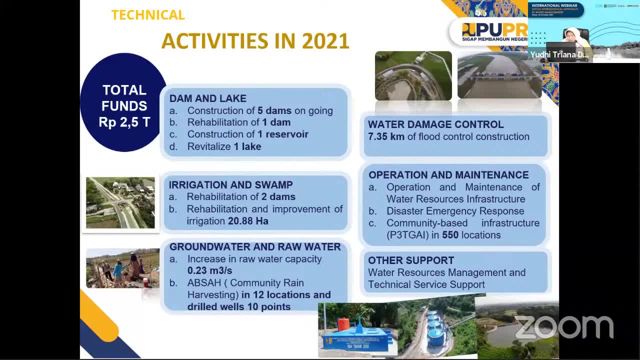 In this year- 2021, we have 2.5 trillion. It is divided into many sectors. First, it's dam and lake: The construction of five dams ongoing right now And the rehabilitation of one dam, The construction of one reservoir. 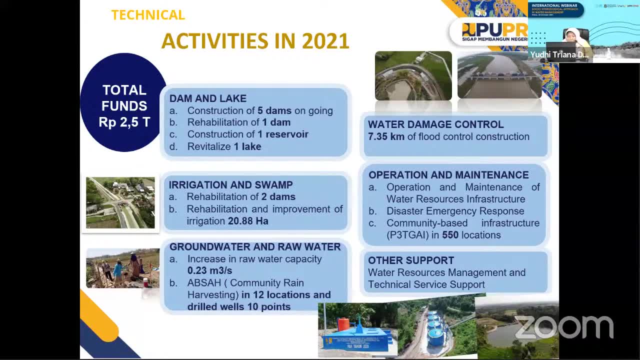 And revitalizing one lake, Irrigation and swam sectors, Rehabilitation of two dams, Rehabilitation of improvement of irrigation And in groundwater andενrawater increasing groundwatering capacity. And Apsa is a community of rain, harvesting in in 12 locations and built wells 10 points. 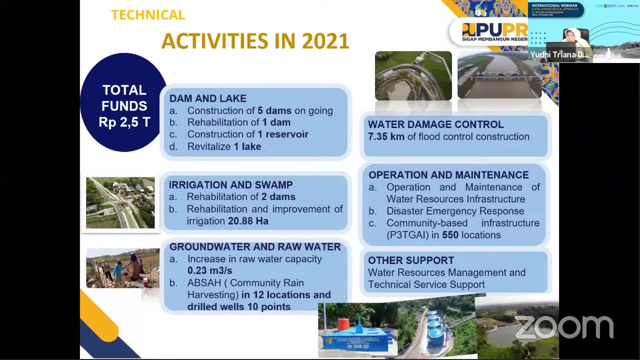 In water damage controlling- we built 7.35 of flood control construction, such as levee revetment and others. And in operation and maintenance, we also have community-based infrastructure- we call P3TKI in 550 locations and other support. 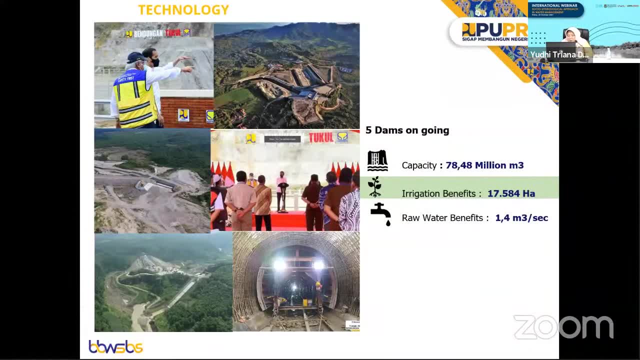 Right now there are five dams ongoing. The capacity of the total five dams is 78.48 million meter cubic And for the benefit in irrigation there are about 17.58 hectares And raw water benefits 1.4 meter cubic per second. 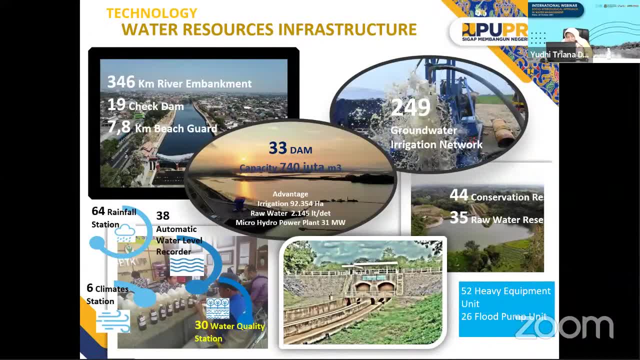 And the electricity savings in this is around 3.24 billion Generally in total. if you bike, you will Gedanken either hurt your body or you will bite. Right now, EBWS, Bengawan Solo has so many activities. There are 30 dams, 33 dams. 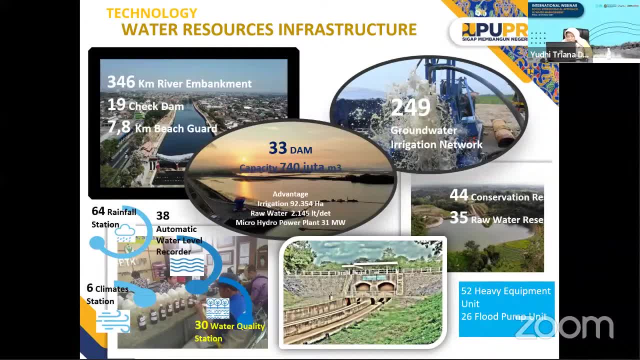 with total capacity 240 million meter cubic. We have also 346 kilometers river embankment, 19 check dams and ground cells, 7.8 kilometer beach guards infrastructure. We have also 249 groundwater irrigation network. We also have flood forecaster warning system. 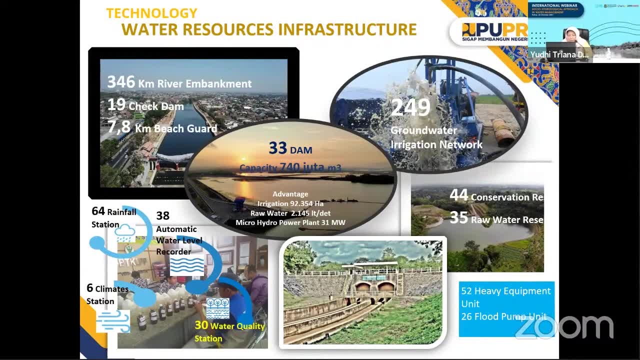 We have 64 rainfall station, 38 automatic water level recorder and 6 climate station, and we have also 30 water quality station And we also have 52 equipment- heavy equipment unit for the emergency condition when flooding happens, And we have also 26 flood pump. 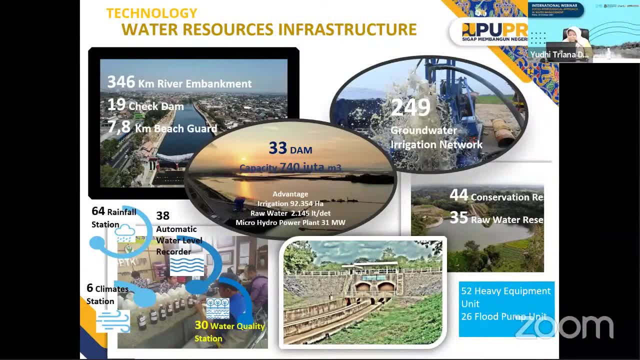 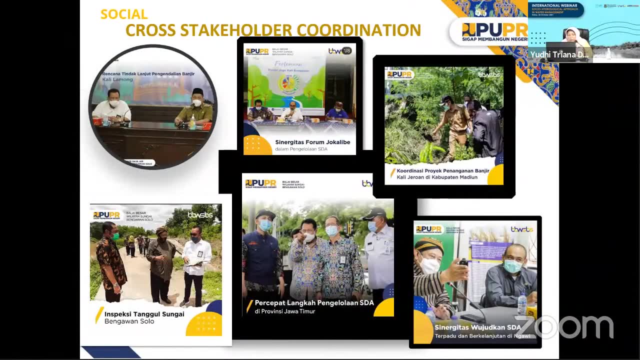 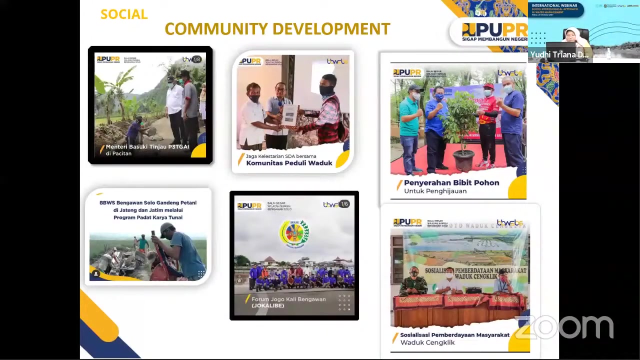 This is the documentation of our activities in social cross-stakeholder. We have so many discussions with the local leader And we always have a good relationship in making decisions. This is documentary for our community works. We have Jogokali, Bengawan Solo and we do some conservation and there are so many activities. 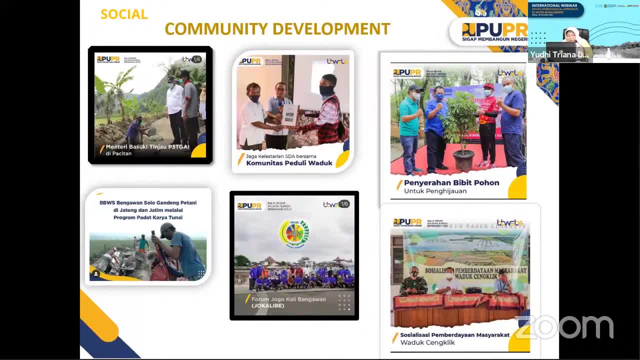 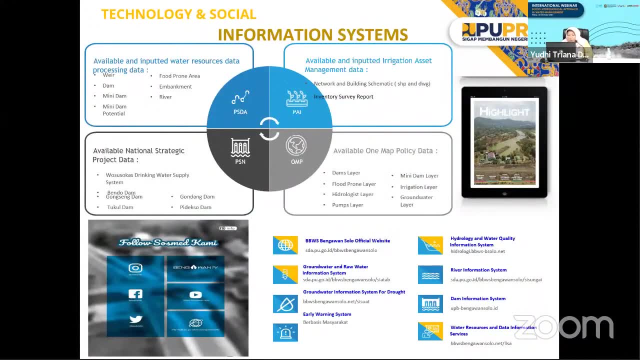 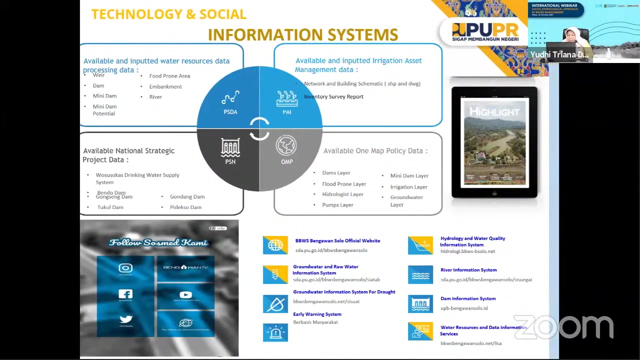 in Jawa Tengah and Jawa Timur, Central Java and East Java. And this is technology and social information. We have also many kinds of information channels. We have Bengawan TV, We have Twitter, We have Facebook, We have Instagram and everybody can access the social media. 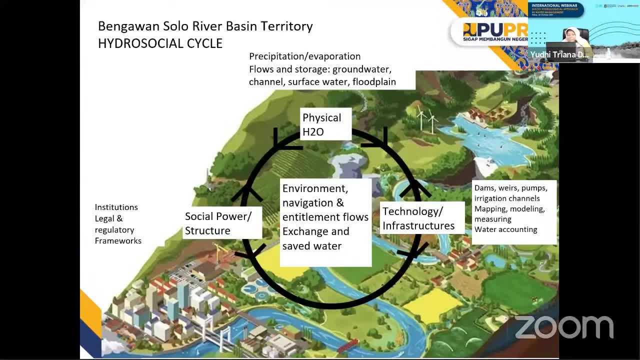 Bengawan Solo River Basin Territory Hydrosocial Cycle. This is Bengawan Solo River Basin Territory Hydrosocial Cycle. We have three parts: physical, social and also technology And BBWS Bengawan Solo. Right now we have all facilities to support this part, this component, in embracing the 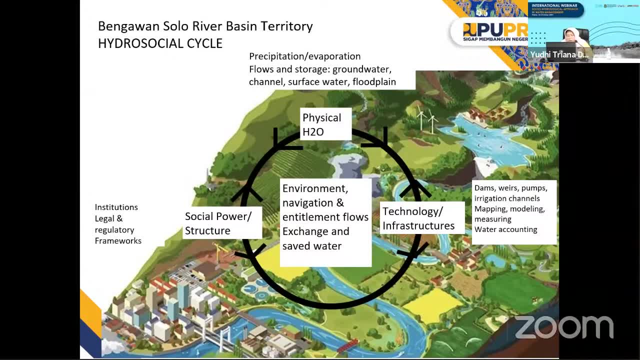 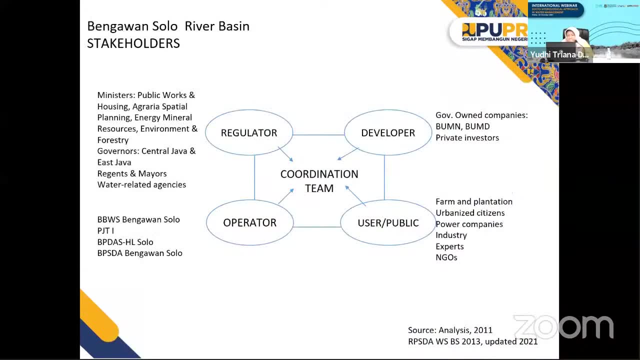 three components to gain our goal to implement the integrated water resources management. Actually, there are four stakeholders in the project. There are regulators, operators, developers and users or public BBWS. Bengawan Solo takes action as an operator And we have a coordination team. 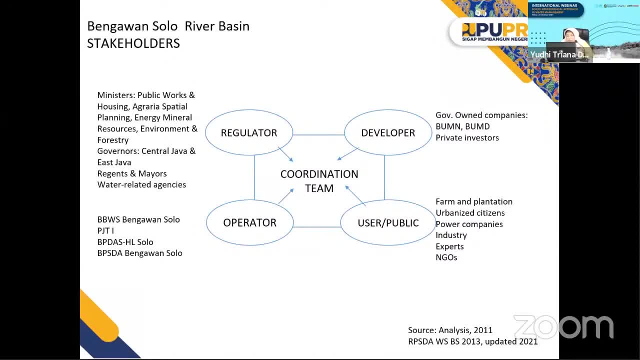 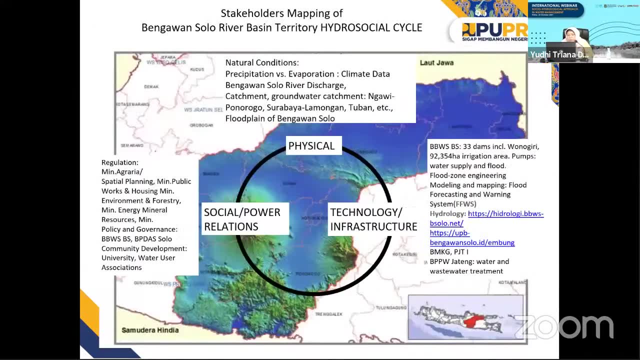 It's called TKP SDA Water Council in River Basin of Bengawan Solo River. This is stakeholder mapping of Bengawan Solo River Basin. This is stakeholder mapping of Bengawan Solo River Basin. This is stakeholder mapping of Bengawan Solo River Basin. 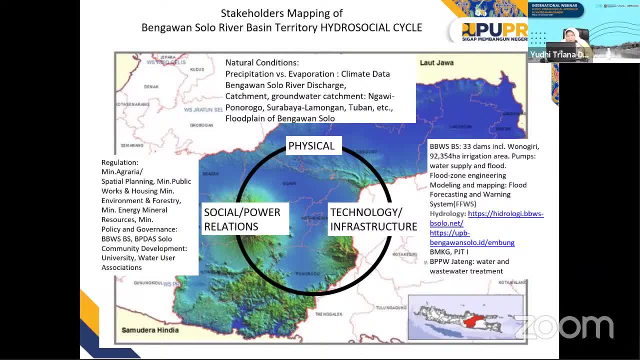 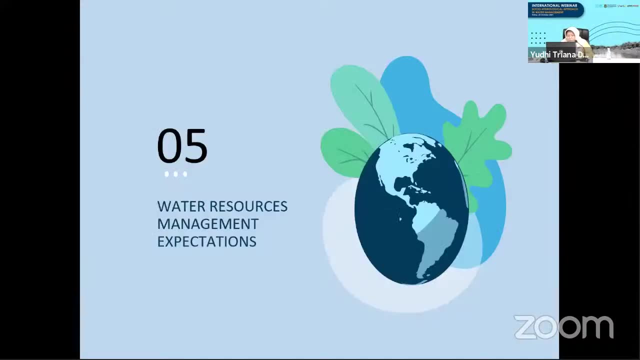 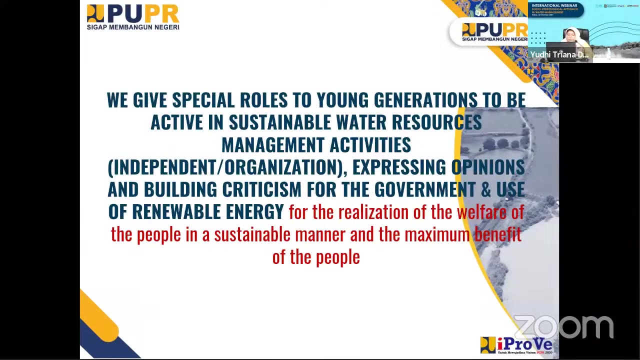 Actually, we have done all of these concepts, including the physical, social and also technology. And last, we have some expectations. We give special roles to young generations to be active in sustainable water resources management. Thank you. activities expressing opinions and building criticism for the government and use of renewable. 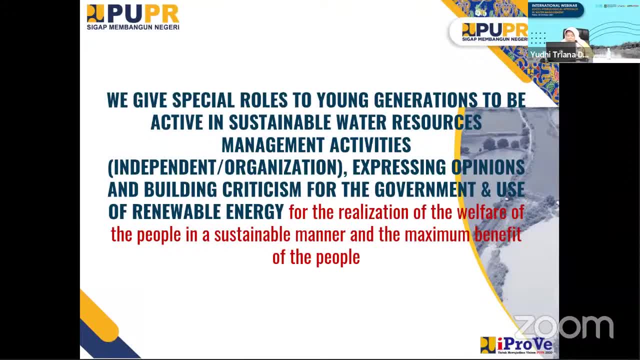 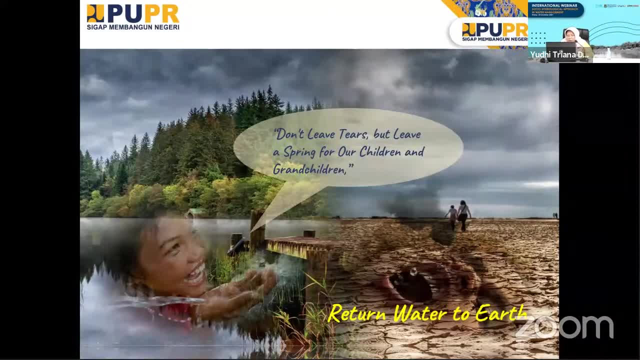 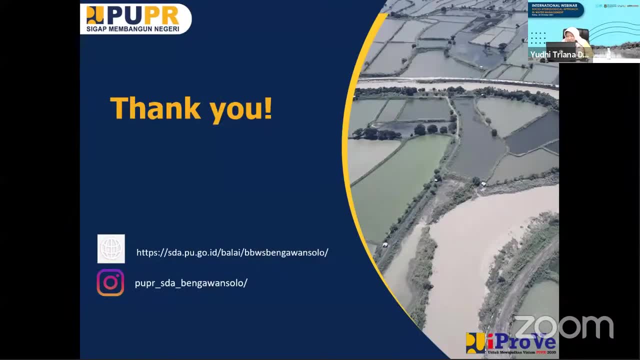 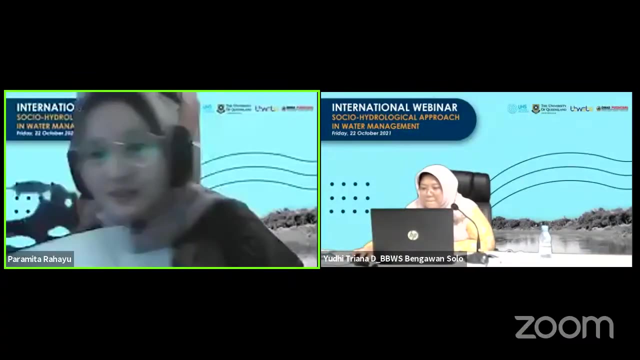 energy for the realization of the welfare of the people in a sustainable manner and the maximum benefit of the people. Don't leave tears, but leave a spring for our children and grandchildren. Thank you very much. Thank you very much, Bu Yudi. 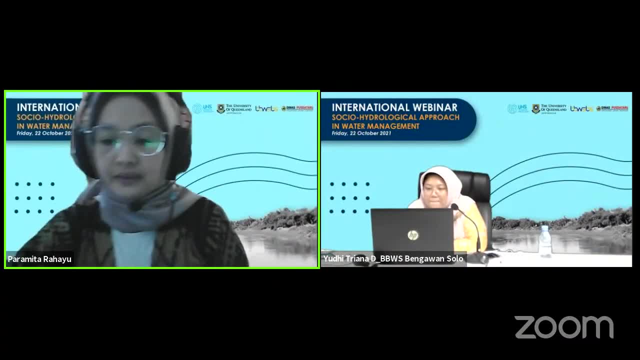 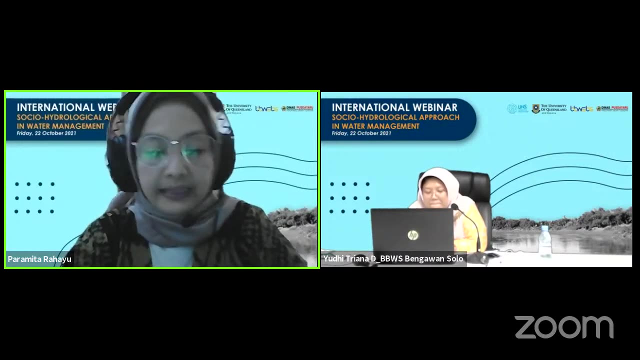 Interesting presentations about the problems of Bengawan Solo River with too much, too little, too dirty and also problem of behaviors, land conversions and management crisis. And BBWS, or Bengawan Solo River Authority, has applied technical approach, social and 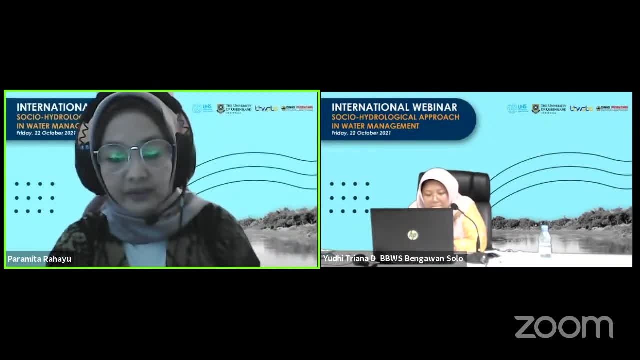 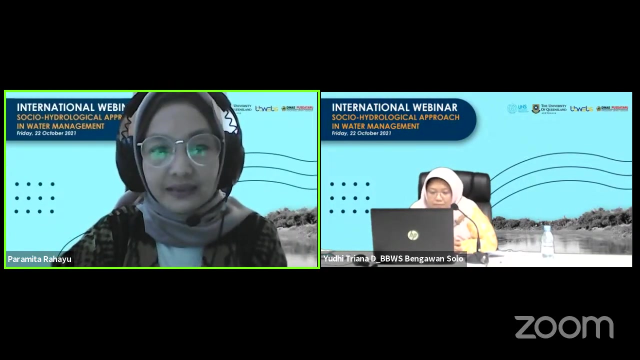 also technology and social approach, with information system to deal with the problems, with all the problems, and also the program of emphasizing the role of young generations to take part of this river management. Thank you very much, Bu Yudi. And now we go to our fourth speaker, Bapak Insinyur Eko Yunianto. 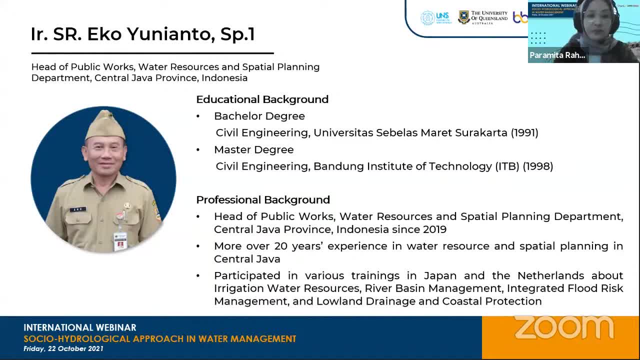 Bapak Eko Yunianto is currently Head of Public Works, Water Resources and Spatial Planning Department, Central Java Province, Indonesia. He received Bachelor's Degree from Civil Engineering Universitas Blas Maret and Master's Degree also in Civil Engineering Institute of Technology Bandung. 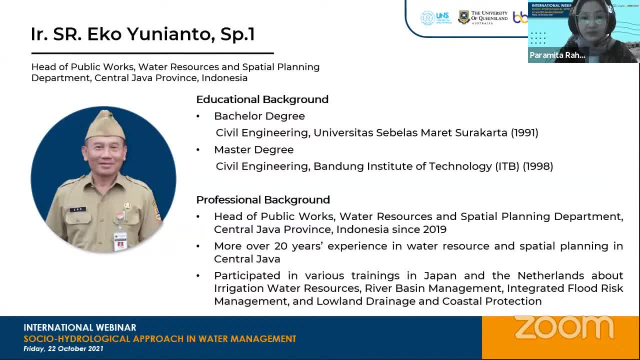 He has experienced more than 20 years in water resources and spatial planning in Central Java. He also participated in various training in Japan and the Netherlands about irrigation, water resources, river basin management, integrated flood risk management, Also low land drainage and coastal protection. 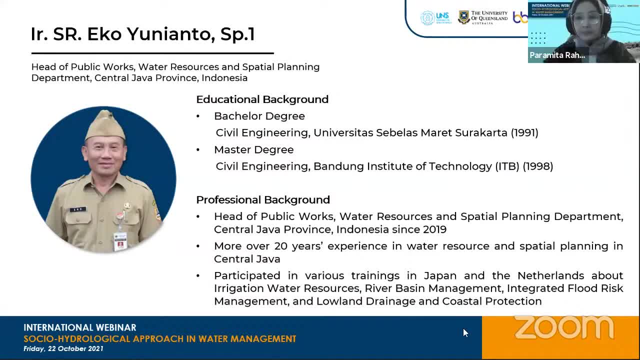 I think Pak Eko today will share his expertise in water governance with the case study of Bengawan Solo, if I'm not mistaken. Please, Pak Eko, the time is yours. Assalamu'alaikum warahmatullahi wabarakatuh. 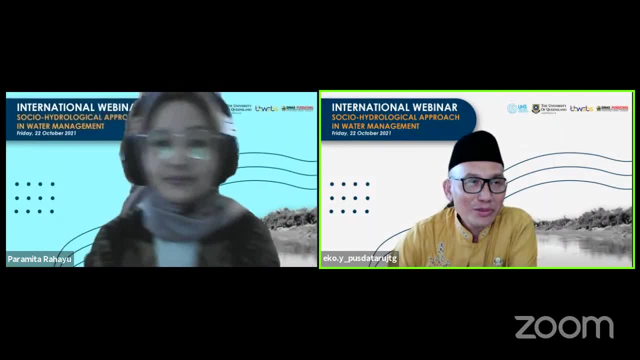 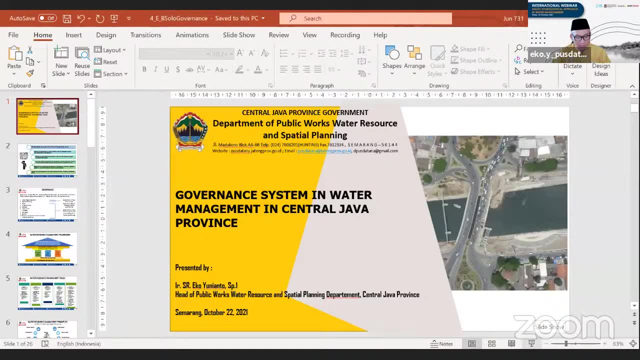 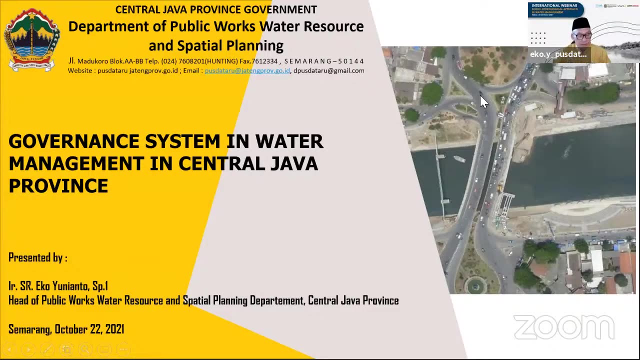 Selamat sore, Karima bin Muhammam는데. Movement in theubs and management of Panel for Peaceful Water. Thank you for the opportunity. First, I would like to send my regards to the distinguished speakers and the planning of Universitas Blas Marat that make this event possible, and all the participants. 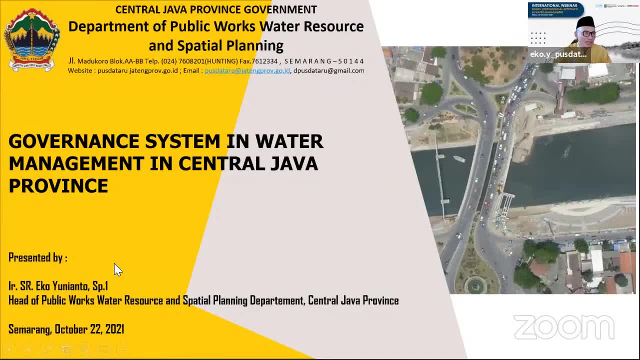 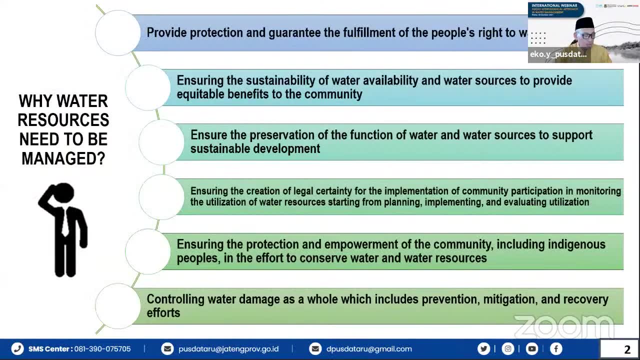 I would like to present my presentation Continuing to our topic: the government system in water resources management in Central Java. Why water resources need to be managed. I think we should be providing protection and guarantee the fulfillment of the people's right of water. 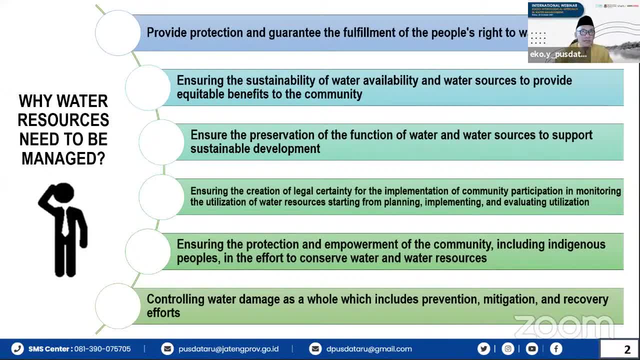 Ensuring the sustainability of water availability and the water sources to provide to the native and the community. Ensuring the presentation, The preservation of the function of water and water resources to support sustainable development. Ensuring the creation of the legal certainly for implementation of community participation in monitoring the utility of water resources, starting from planning, implementing and utilizing. 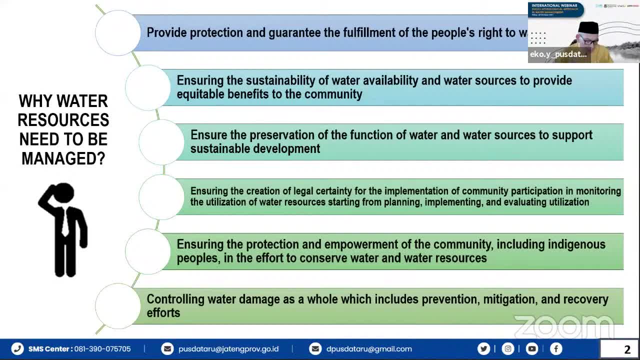 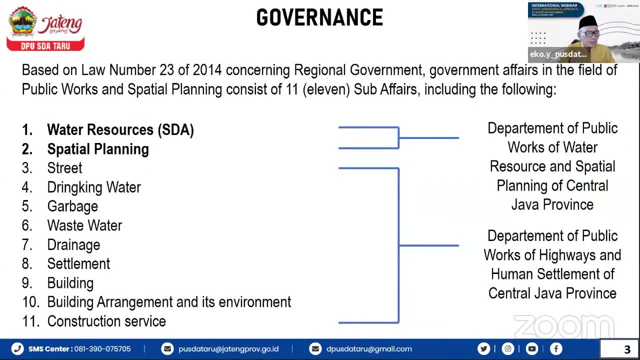 And then ensuring the protection of the environment of the community, Including water resources, Ensuring the protection of indigenous people in the effort to conserve water and water resources And the last one, controlling water demand, of which includes communication and And basically from the, because my business in my 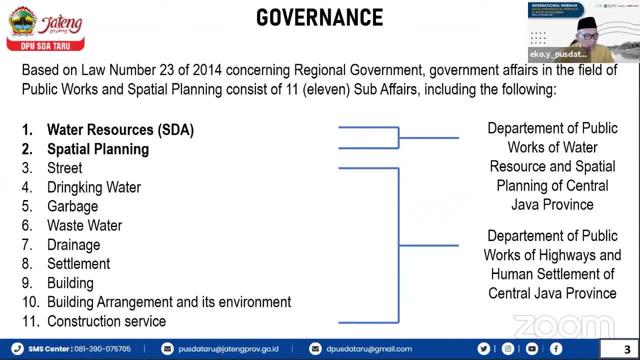 That's outlaw number 23.. 2014 concerning regional government affairs in the field Of the public work and special planning consists of 11 sub affairs, including the following: because you know that in the central Java, the fight by 2 integration: 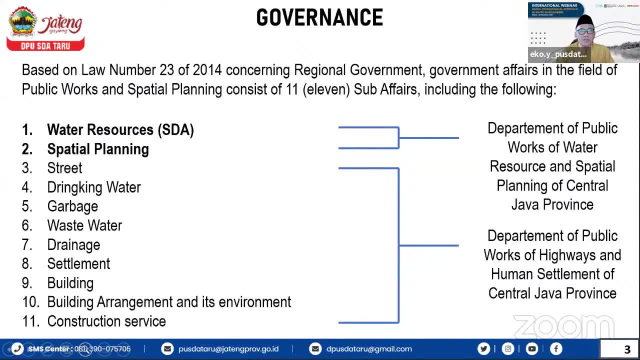 And number one and the number 2,, what research and central planning is our job? I mean in the department of public work, of water resources. And number 3, and at 11.. It's the Okay. So I want to set it like this: 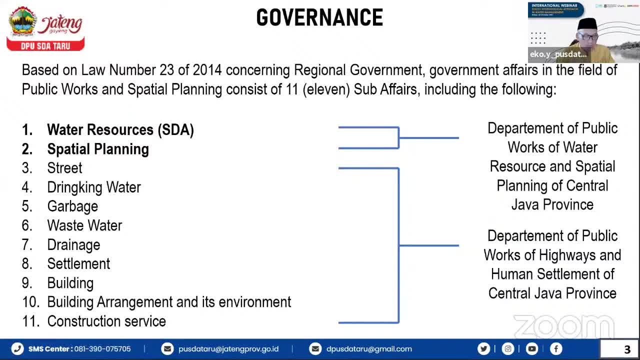 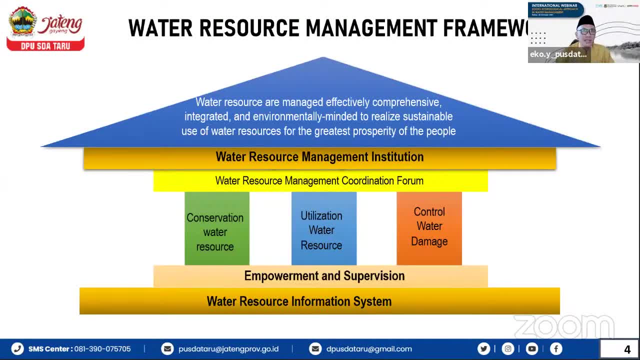 The spirit of a So pretty good Good question And then A basic of Article Passage. We got the guy 23rd. They take on the, But the resources are minutes. It could be comprehensive, Integrated And environmentally. 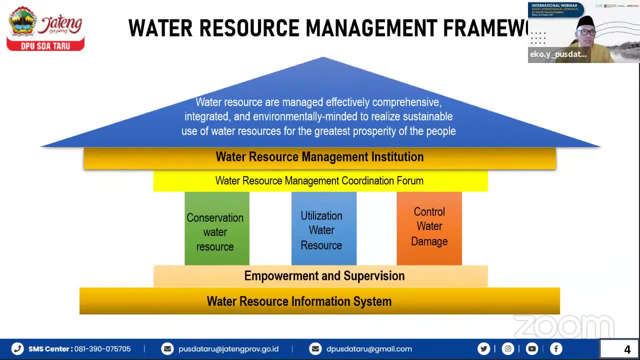 Minded to realize Sustainable use of water resources For the greatest Property of the All people In the nation. But how to What the research management to Run Wesley Should be? There are water resources management in The format. 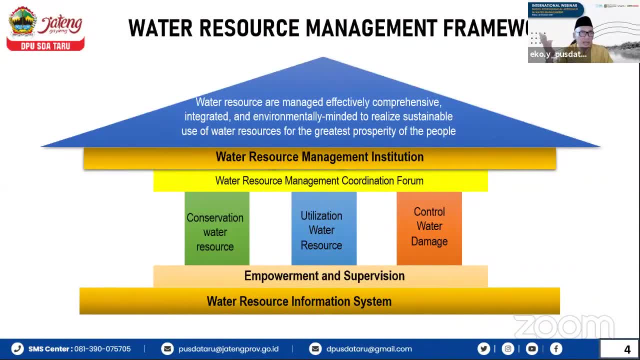 For example, On the central Government, We have the RBO Represent From Public Department Of Ministry, Like this, And then the Provincial, Like Our Institution, And From The Or. 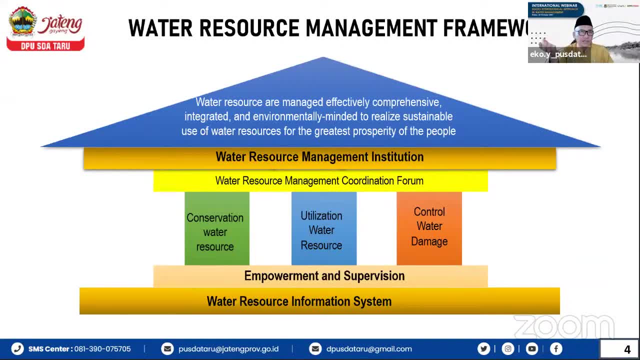 City We Have Like that And then We How to improve The A Performance Of the Water. It Should be About That By Water In The Center We Have. 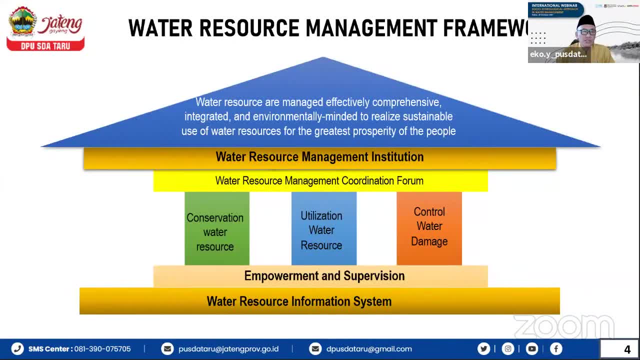 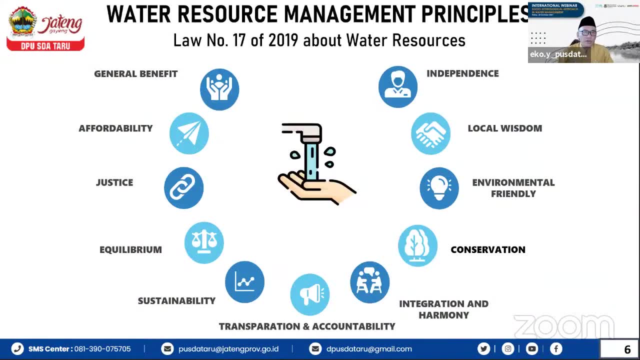 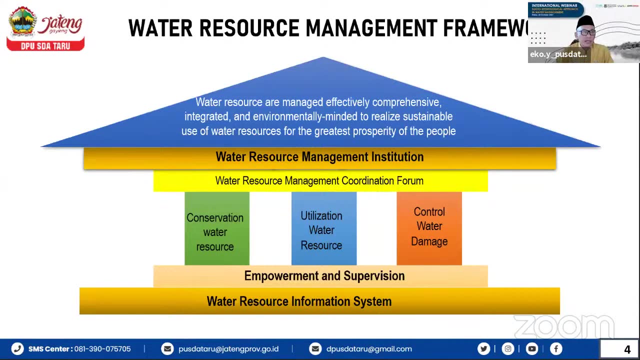 The Water Research Council, National Water Research Council, And Then Take Up In Coordination, I Think, Before People Ask, And Then We Have Commission Irrigation. 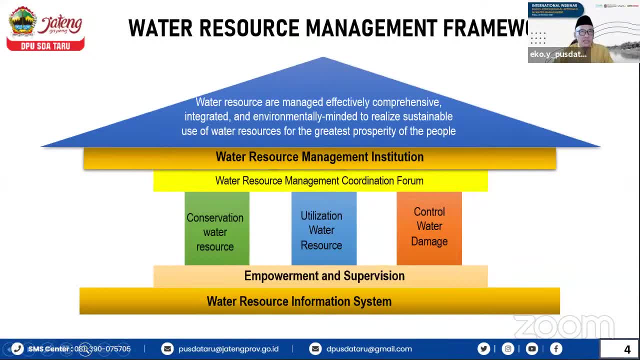 Of Water Resources, Utilities Of Water Resources And Water Water Demand That The Three Pillar Will Be Spent Exactly. We Have Two Pollution Improving. 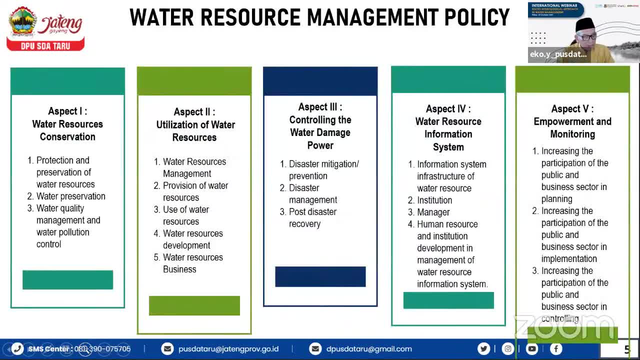 And Supervision And The Support By The Water Resources. Conservation Consists Of Protection And Preservation Of Water Resources, And The Second One Was The Presentation. 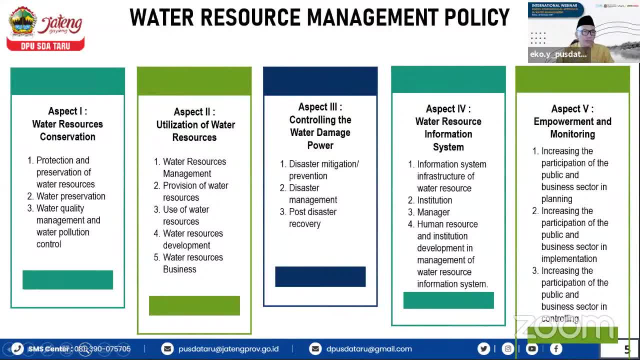 That Fun For The Quality Management And Water Pollution Control Demand Power. Because If We We Don't Able To Help The Water Resources Manage Perfectly. 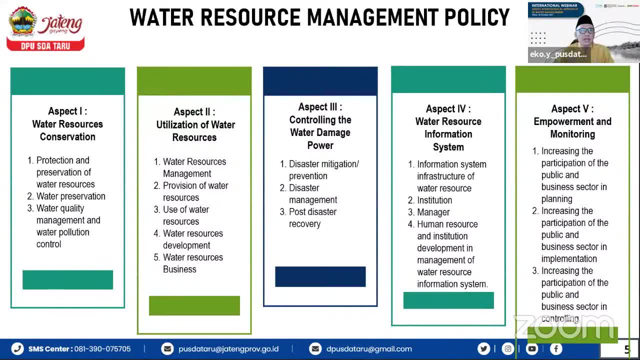 So Water Demand Will Be Happened, And Then Consider The System, Mitigation, Mitigation Presentation And Aspect Four And The Five As Water Research Information. 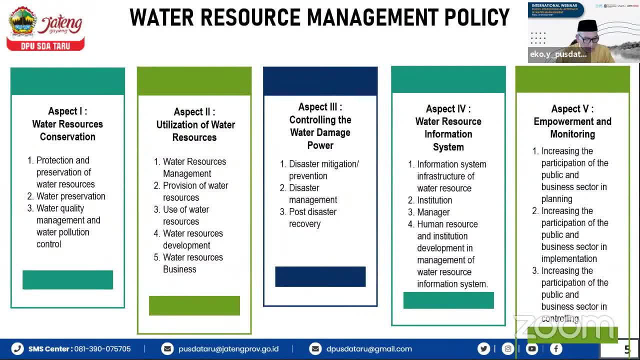 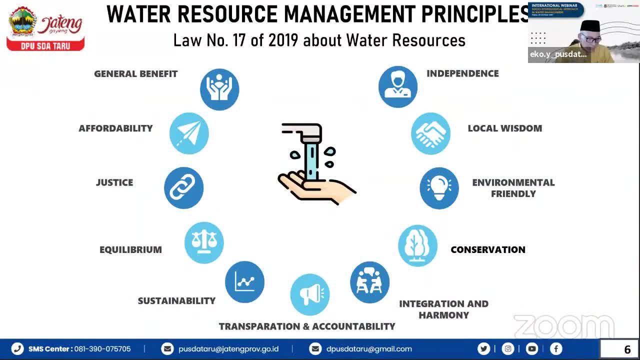 And Empowerment And Monitoring And Supervision, I Think, And Then Her Basic Form On 2019.. So About The Water Resources Next, I Think. 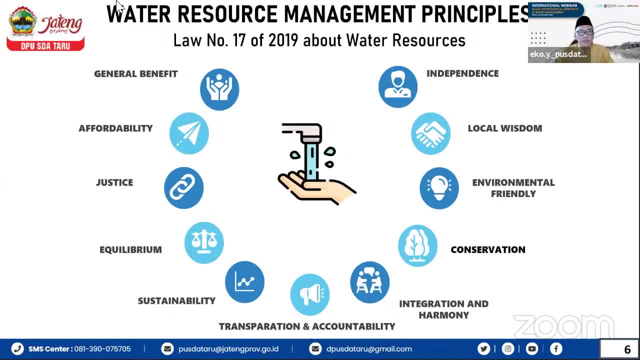 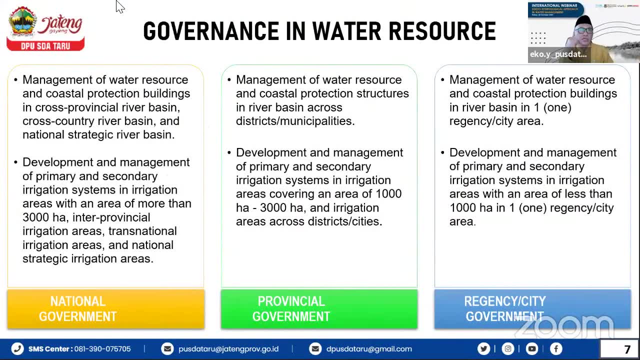 And To, To Entrust To The Fundamentals And To Another. So So, All The Fundamentals And To All, Not To You, Some To To. 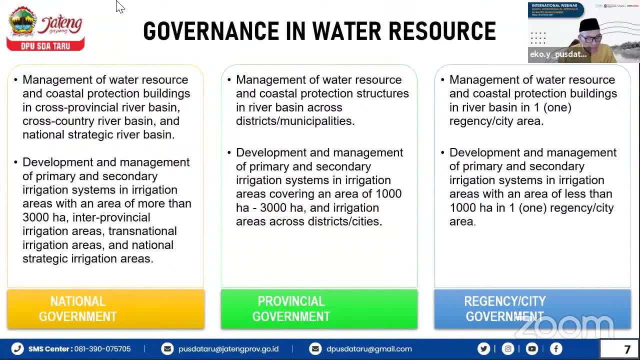 To Until Now. Now, and how the government and what the resources uh separate. uh about the description of uh responsibility from the national government and provincial government and regency or city government. but the the layer, the second layer added from the how to manage our irrigation. 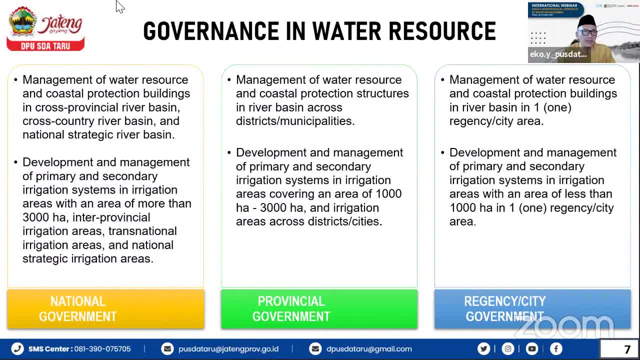 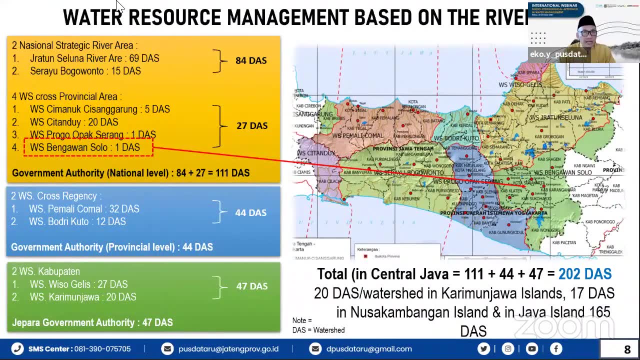 but the, the first irrigation, how to manage the river basin. i think in this, in the, our law is like this. and then, uh, in central java, we have a 10 uh, google unity of the watershed, because you need the apparatus compiling by many watersheds, because 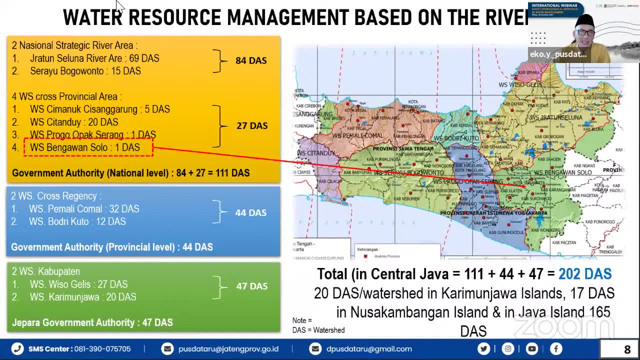 in indonesia, especially for central java, i think, because in java tengah, in central java we have 202 watersheds, we have 10 unity of watershed from the. for example, we have uh, tarimun, java island, pengawan, solo and then uh, i think we have the java tengah, general java. 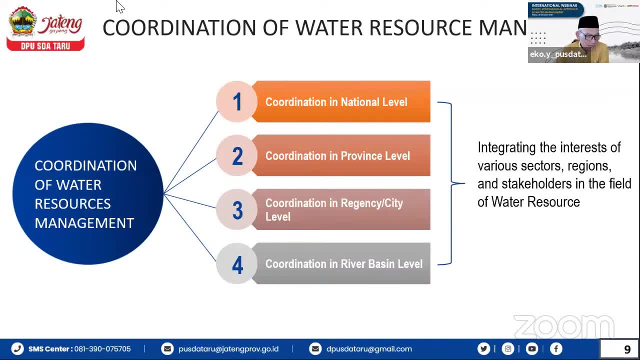 and then how to coordinate water species management in uh central java management provision in national level i think we have already talked about and then producing provincial level. we had eight take up asia coordination team for water resources. uh, basically, from the unity of the watershed we have uh sick because the tarimun java and uh resources depend on the tpu pr not to 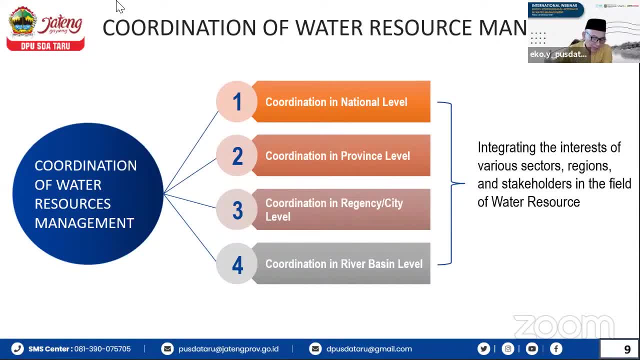 uh and coordination. regency, city level- we have gpu pr, i think uh, mostly uh- and coordination. a river basin level to integrating the interest of every sector, region and stakeholder in the field of the water resources, and then coordination from the town solo river. i think it's a. 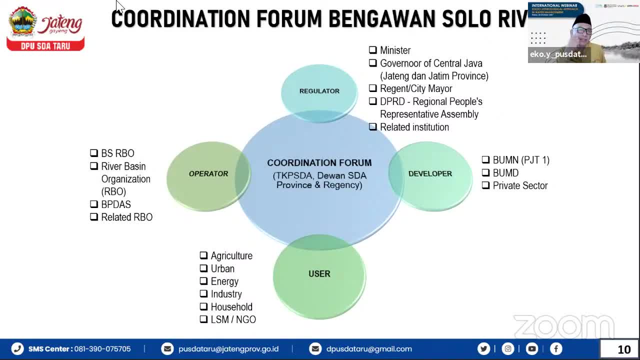 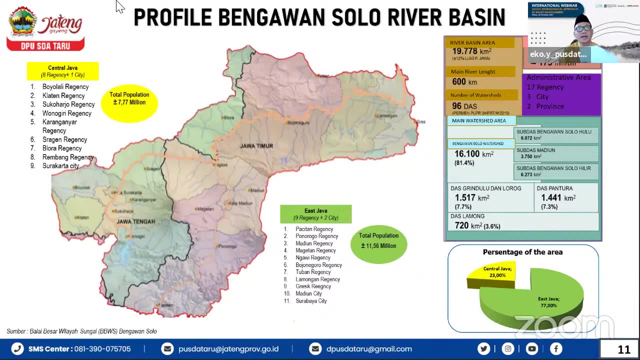 uh, the former uh speaker of uh- already excellent, i think i i want to continue that. my uh, my next sit right and then uh profile and solar reverberation is like that i think also my colleagues from uh doing and solo reverberation already explained. i think i want to also to escape. 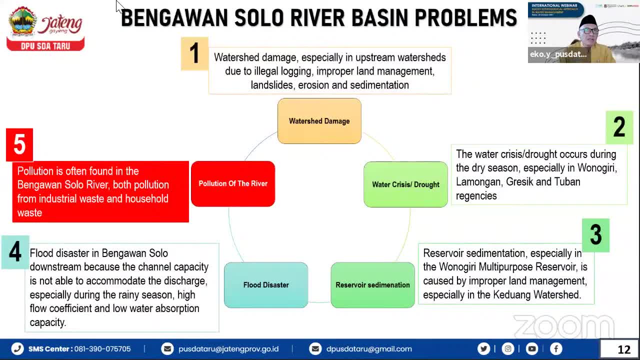 about it and then help the council. reverberation problem, i think water city mates. and then water crisis: drought because in during the dry season we have too little uh water in the uh solo reputation and the reservoirs that demand someone. then flood disaster during the rainy season. 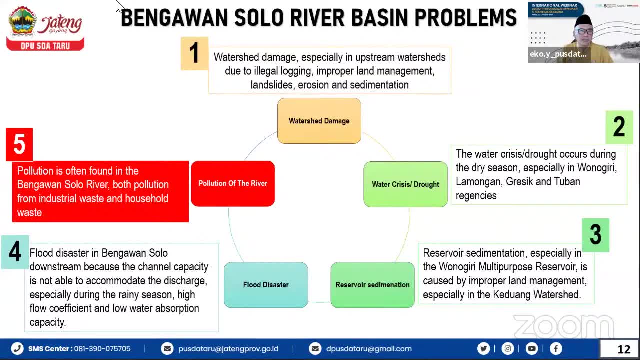 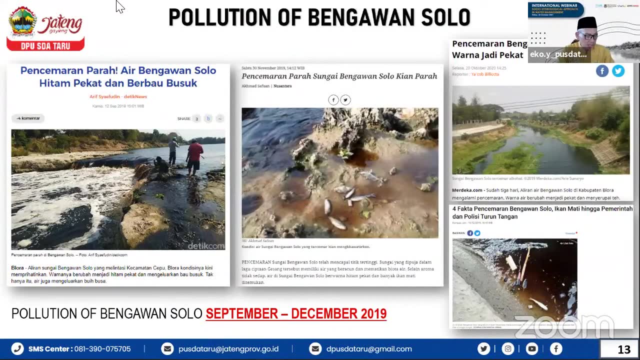 and then pollution of the river during the drainage season because of so many production of water, um pollution, especially in soloraya, i think, and then uh this overview for collection of the transolo or the the uh the morning and then uh the modi media master to to uh issue in the media. 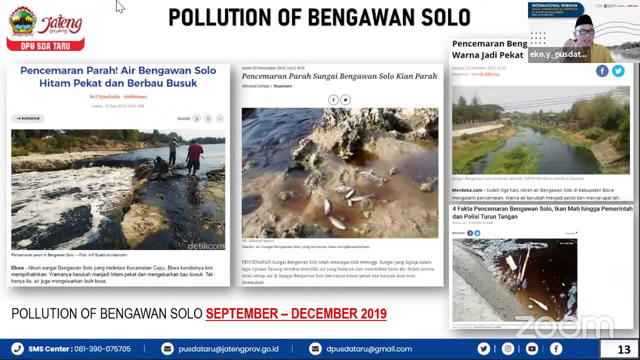 uh, especially in the up downstream in the solar, refer on the central java authority. i i mean in the segment of the uh java, central java province, especially in the uh plural uh. we can see for, like the chapter, like that, the pollution of hong kong solo record in the september, until december 2019, i think. and then next, how to. 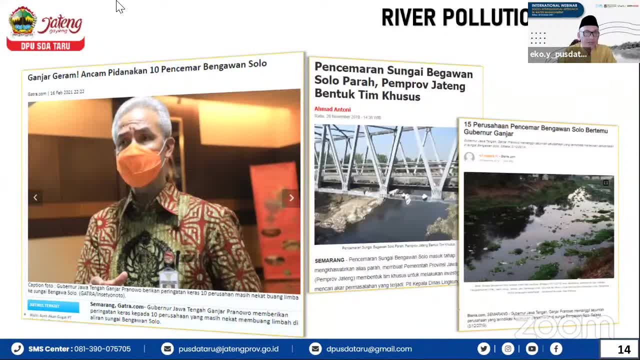 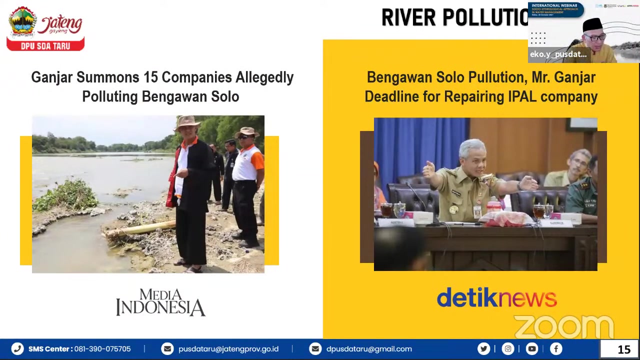 to make the action plan after revolution effort in the uh central java province. my government always gives a time extra, extra attention about this one because the river is transboundary from java tengah to east java. so my, our governor, uh to respond this uh, and then also: 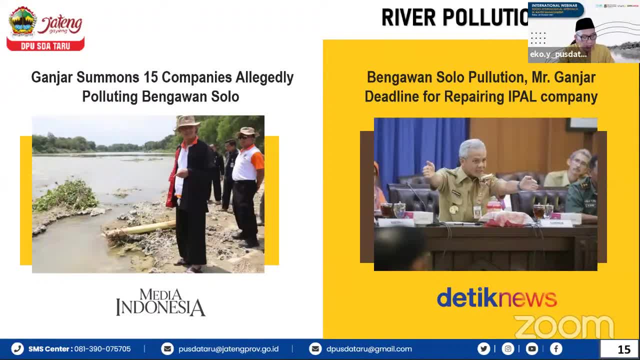 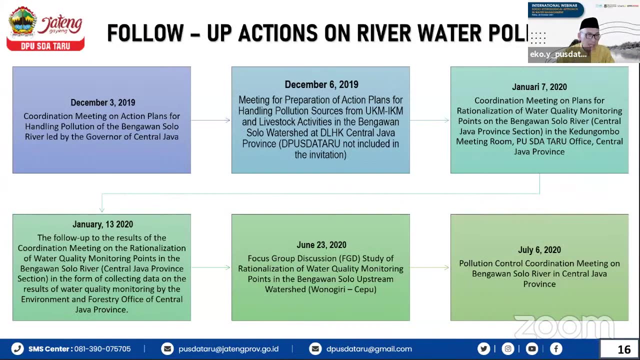 collision to master governor. deadline for firing uh ipala for the treatment company should be more, better and then follow up action and the reservoir population. i think this from the december until the july, from 90- 90- 16 until july 20, 2020. 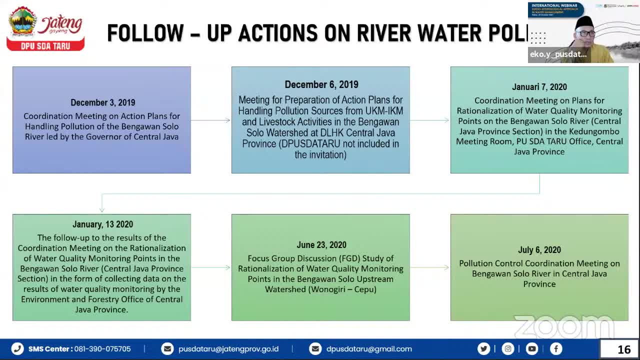 coordination meeting and etc. planning for handling population of the uh in the next step and coordination coordination meeting and plan for rationalization of water quality monitoring point in the Bukalansolo River in the Kedung Ambo meeting in our office in the Central Java. 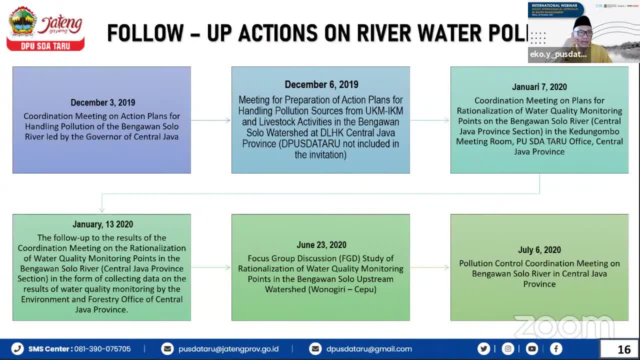 And then the following of the research of the coordination meeting of the rationalization of water quality monitoring point in the Bukalansolo River in the form of data and the result of water quality monitoring by the environmental and forest of the Central Java, And then focus discussion: study of rationalization of water quality monitoring point in the Bukalansolo. 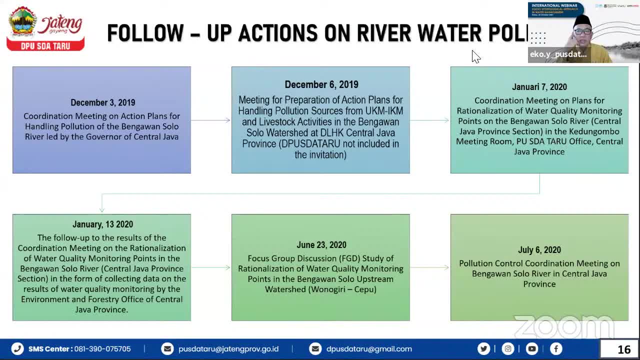 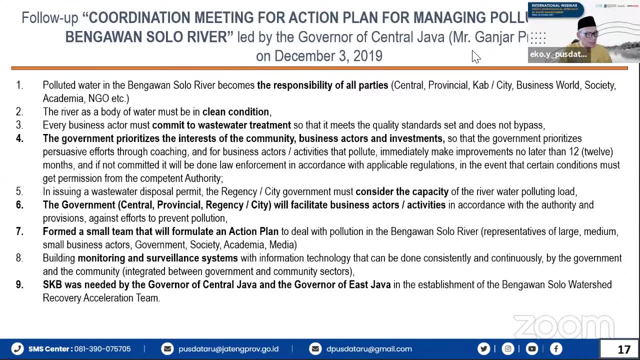 upstream watershed 103 until 4.. And then pollution control coordination meeting in the Bukalansolo River in Central Java province. And then the establishment of water quality management team and pollution control in the Bukalansolo River, etc. This is what is the water quality management team. 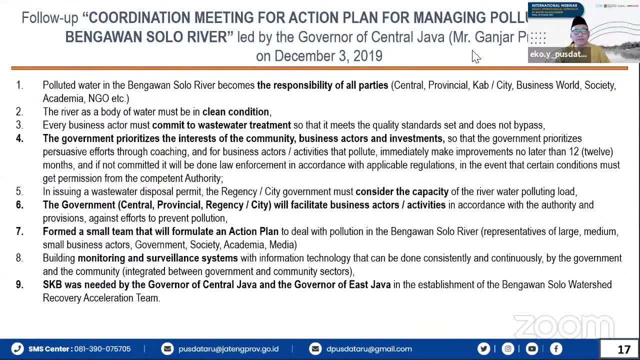 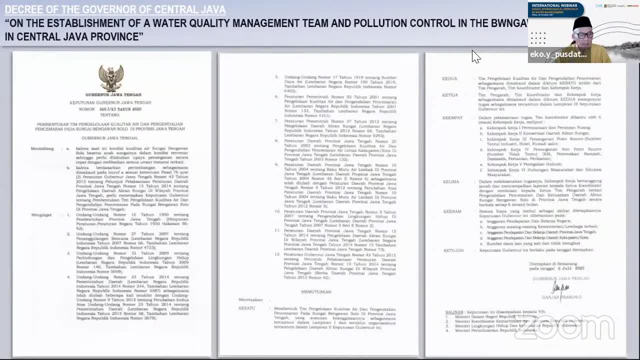 This is the water quality management team. We have a representative by Perth group- I think this one is already signed by Michael Staenberg- to build the team to establish over the quality management team And then, according on the Central Java Provincial Regulation, Peredanam Blast on 2019 about the 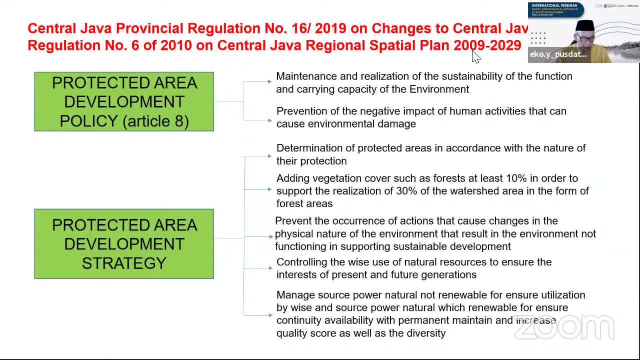 spatial planning. We have protected area development And then a discussion about the water quality management project and negative pollution development policy. Article 8, maintenance and realization of the sustainability of function and carrying capacity of the atonement and preventing of the negative impact of the human. 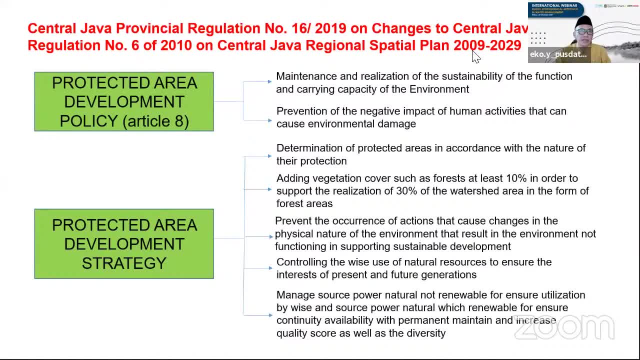 activities that cancel instrumental damage And then protected area development strategy, determine of the protected area in South Korea, with the natural of their protection. I think the situation suffer, such as for us, at least 10% to the order to somewhat the realization of still 30% of the watershed area in the 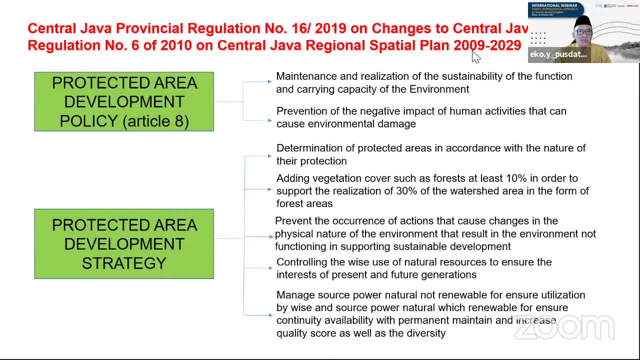 form the forest area, Prevent the occurrence of action that cause change in the physical nature of the experimental, that result in the experimental not function. Thank you, Thank you, Thank you for this materials, folks, for being here. The next part: sustainable development. 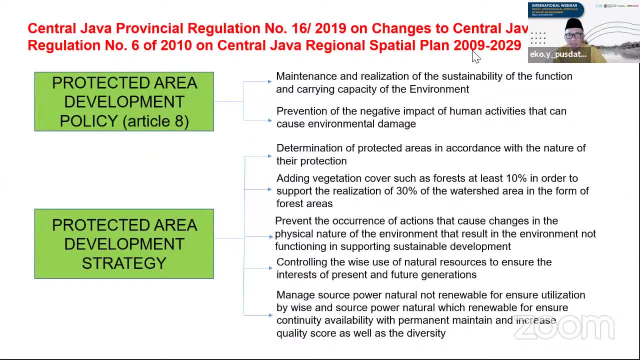 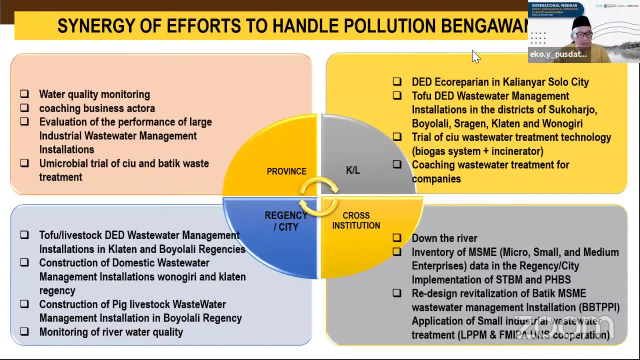 The words to ensure the rights of the person and the future generation quality. so, as well as the specificity and then synergy effort to handle pollution, begawan solo, i think this is uh collaboration, profane and department or uh chemistry and cross indonesian and regain regency city. this is like in the, our cluster detail engineering. 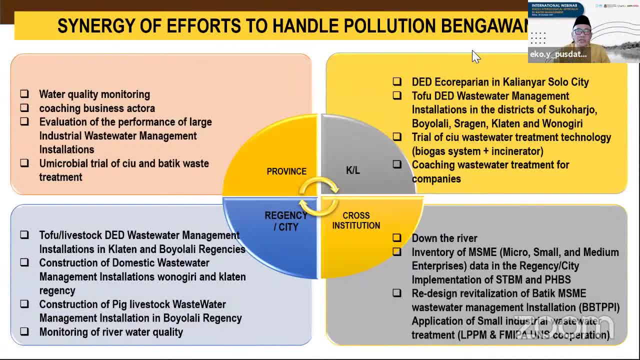 equilibrium in thalianyar, solo city and tofu management. again is the business of the uk and trial of the sea. what is called? you see, what is the traditional, what's the weather? treatment and technology, yoga system in generator and coaching water. what's the word statement for companies? 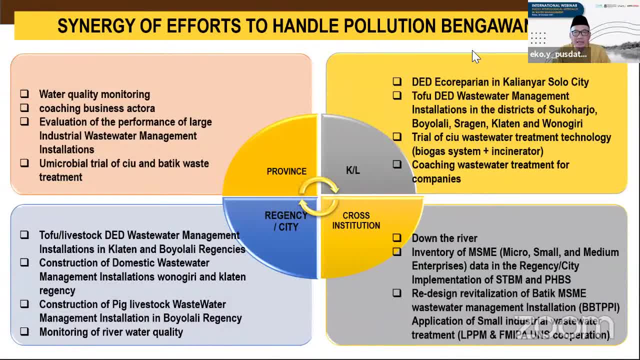 cross intuition on the right, the river, environmental, uh micro, small and medium supplies and in deep legislation, uh stbm. i think it's in the description and redesign civilization of body, because you know the solaria is a lot uh to run. it's uh so many uh body production permits, i think. and then uh coffins, what the 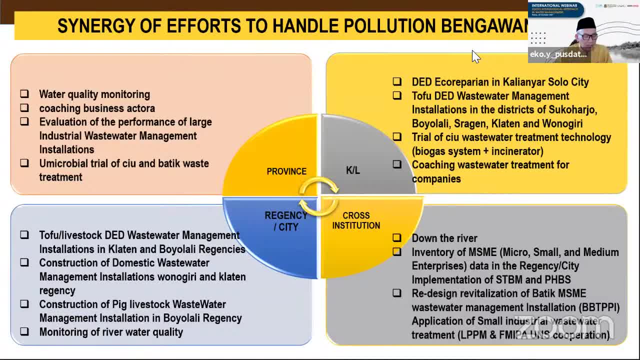 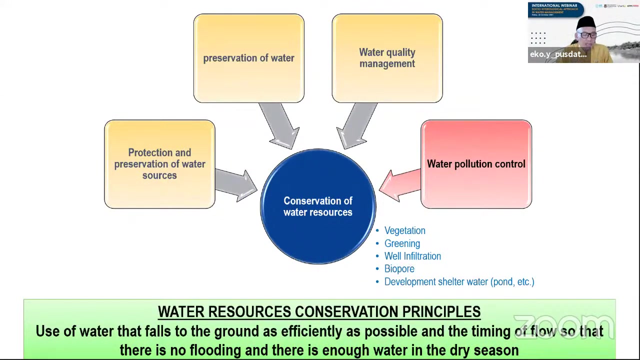 right, uh aspects on it, so i think it's in the description. in the description, what is the quality monitoring, coaching and evolution of department? of the last industry? what's the statement of the last industrial? and then the to direct you to the government in management, solar repair, uh, next month, okay, i think already. 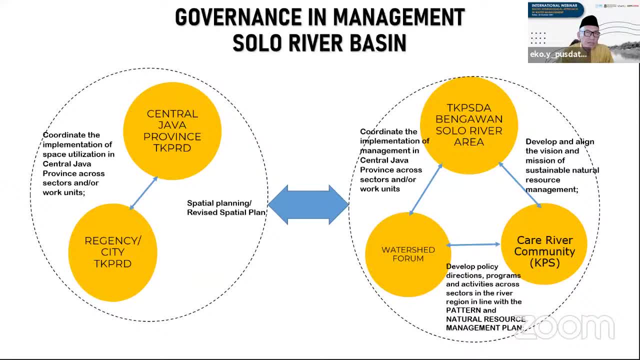 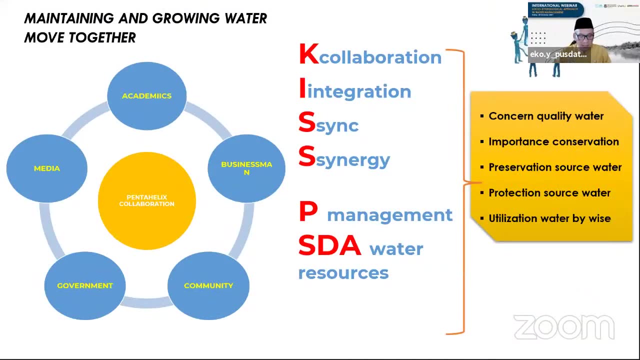 uh, also a pleasant, uh formal speaker. i want to uh the last. uh seed my, my seed minding, and the dropping water moves together. the last one was: yes, this is my point. for us, this is important thing: how to make to collaboration and integration and synchronize synergy for 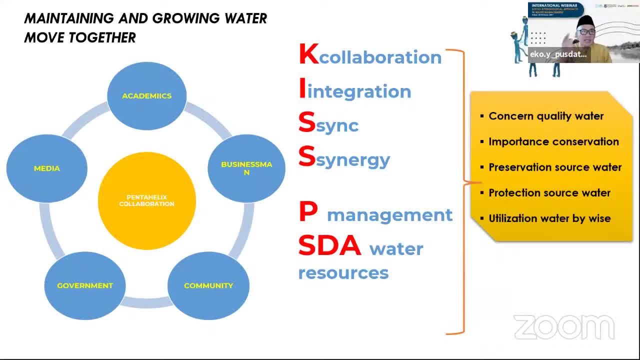 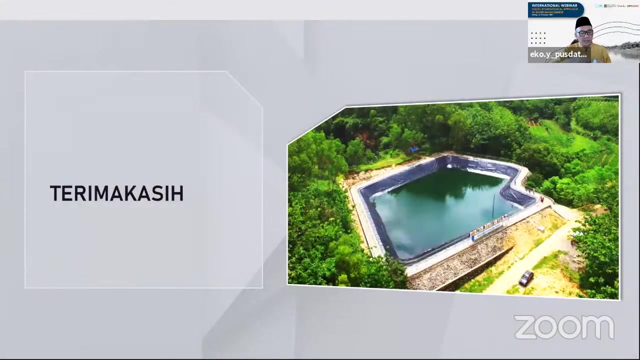 management water resources in central java and it's my point, the main and the strongly mentioned is how to uh, to endorse pentahelical collaboration between academic and business and then a community and a government from central brooklyn district and city, and how to share to the public by media. i think this is our presentation. thank you very much. 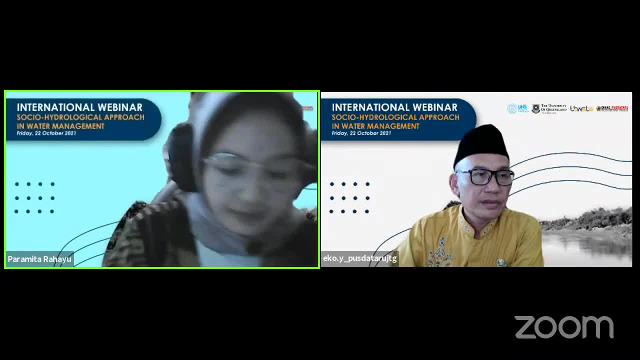 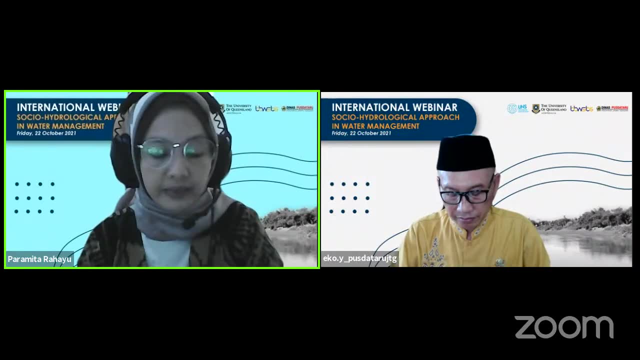 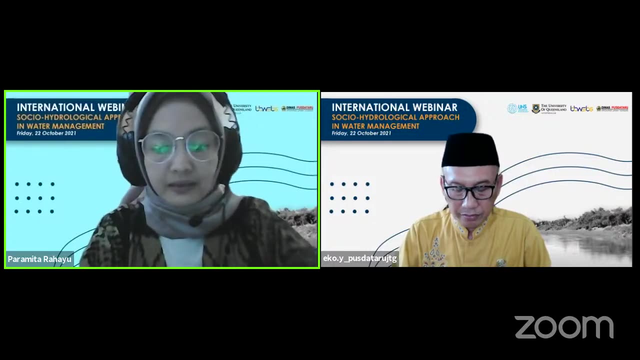 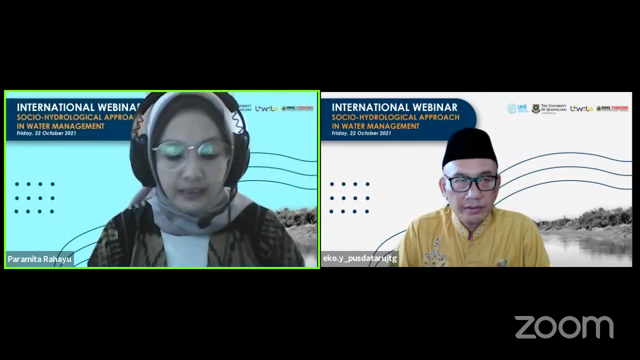 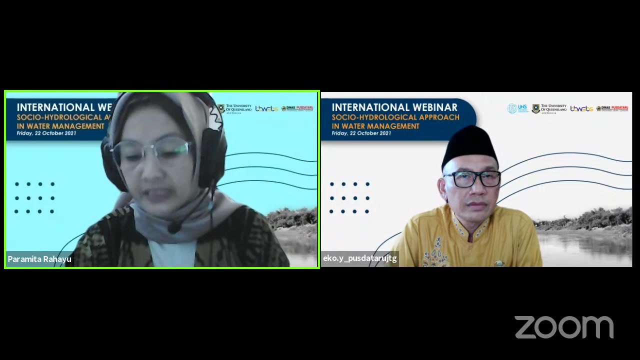 thank you very much, paiko, uh very interesting presentation about the governance of uh water resources, uh management in indonesia. that has actually five aspects: uh conservation, utilization, cultural water damage, uh water information system and also empowerment and monitoring. and, as you mentioned, uh we differentiate uh the coordination of water management in indonesia. 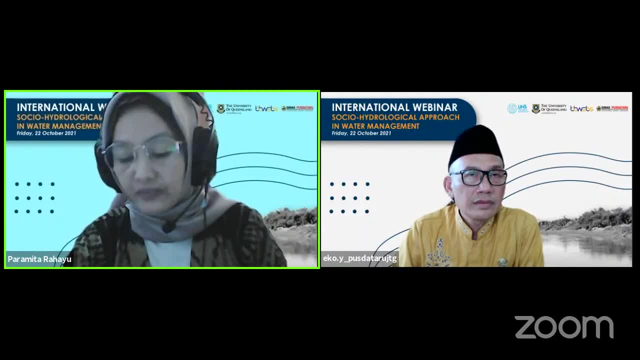 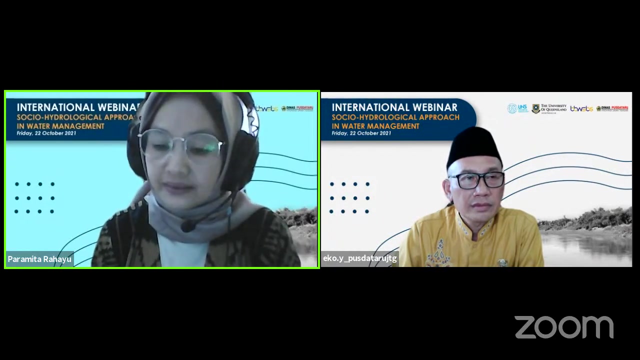 at the national level, a river basin level and then provincial and regency and city level. we also have a very complicated problems of water pollutions. in addition to water, set damage and also drought, sedimentations and also flooding problems, and in the last conclusions you mentioned that we have a pentahelix collaboration strategy for water resources management in. 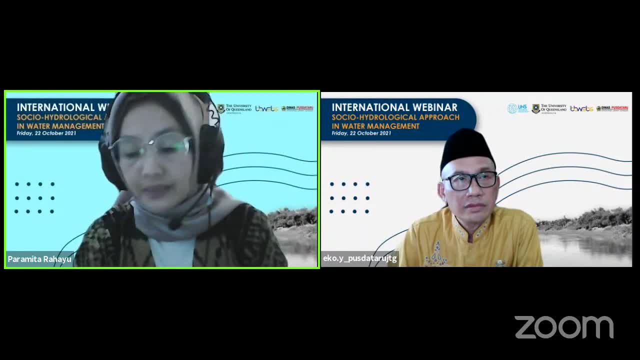 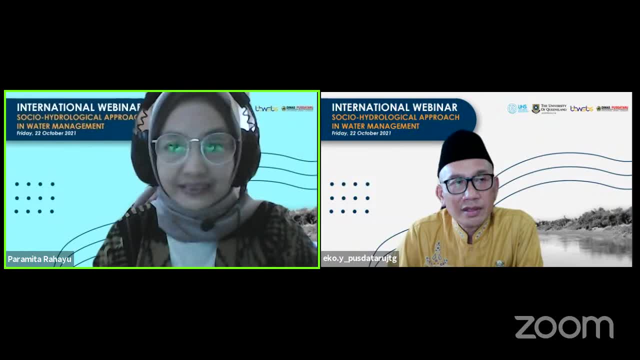 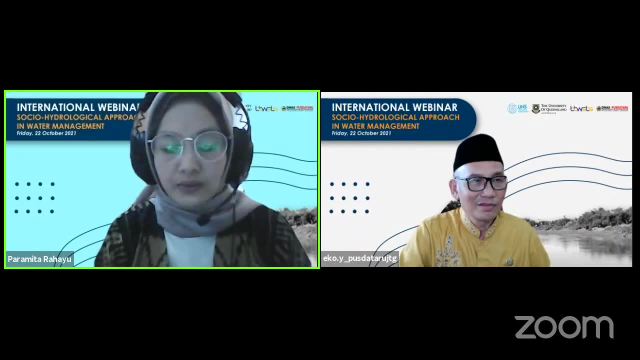 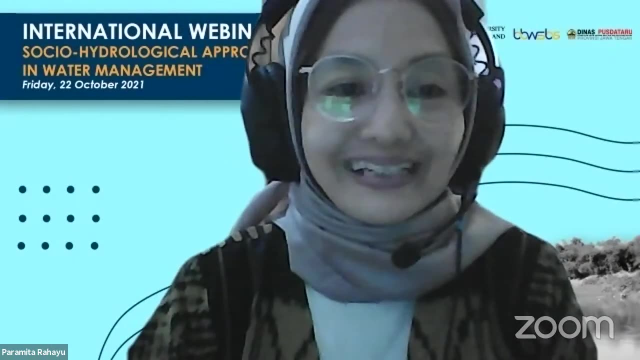 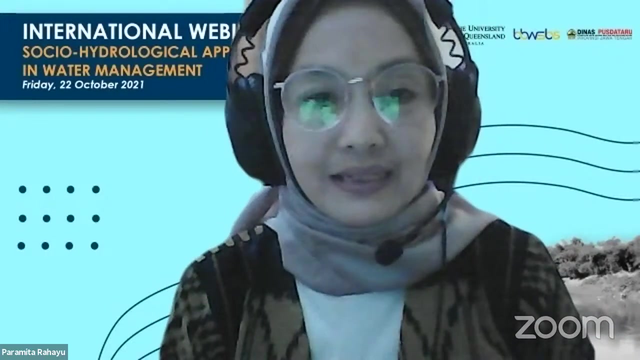 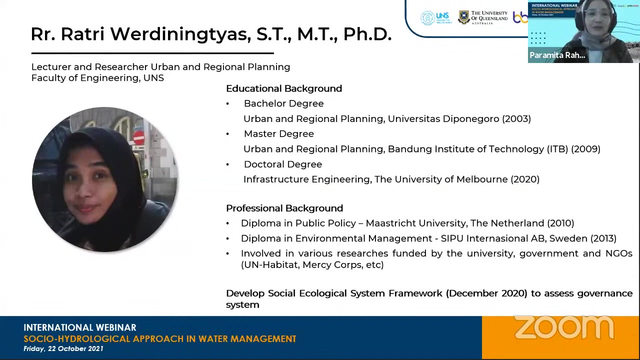 for community день and master resources. thank you, paiko, for very interesting and informative presentations. sorry i mute myself now we will go to our. Ratri is our lecturer and researcher at Urban and Regional Planning Program, Faculty of Engineering, Universitas Blas Maret. 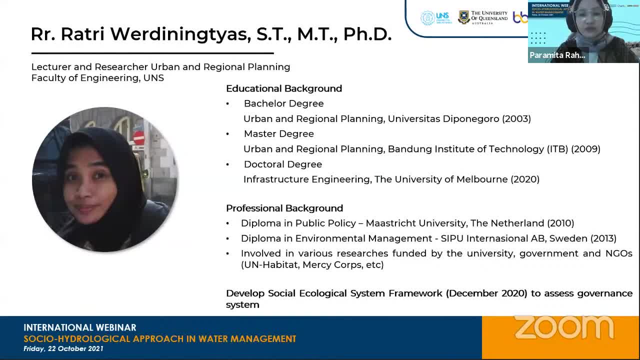 She received a bachelor's degree in Urban and Regional Planning from Universitas Diponegoro, Master's degree also in Urban and Regional Planning from Institute of Technology Bandung And her doctoral degree is in Infrastructure Engineering, the University of Melbourne. She also received a diploma in Public Policy. 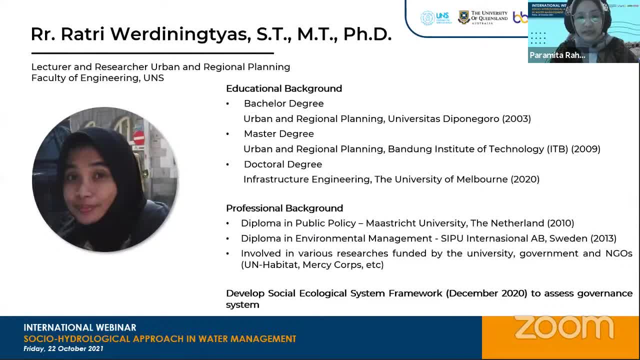 from Maastricht University, the Netherlands, Diploma in Environmental Management from SIPO International AB, Sweden, And she's involved in various research funded by the university, government and also NGO. And now she will present about the framework of social ecological system. 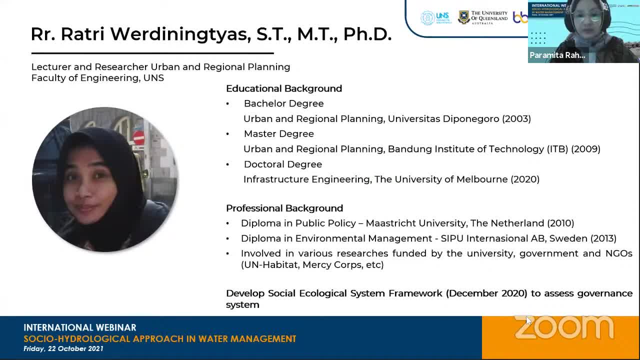 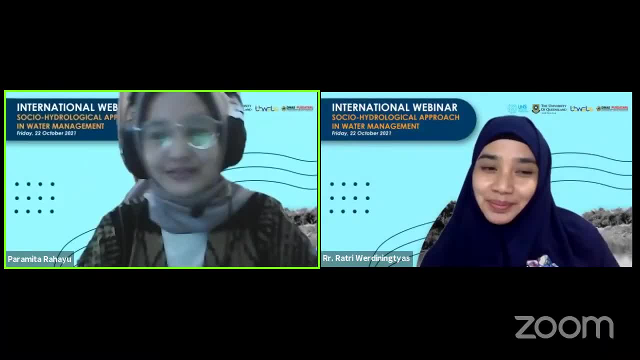 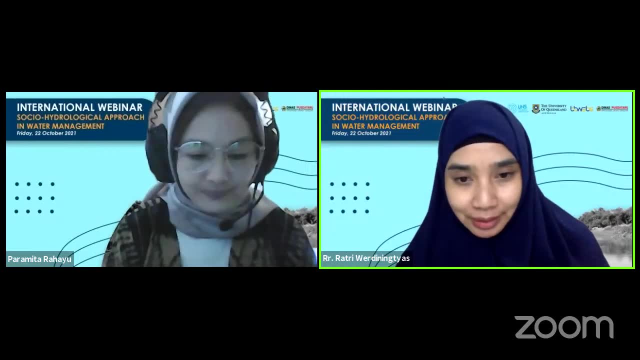 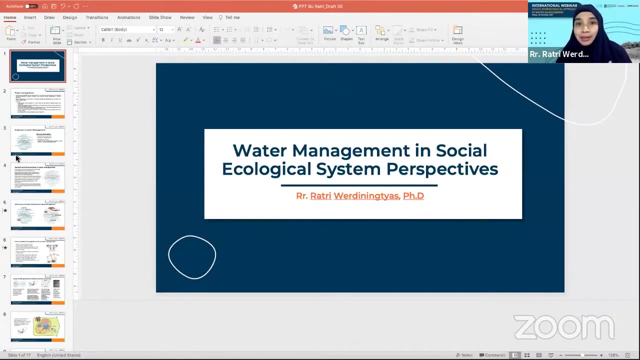 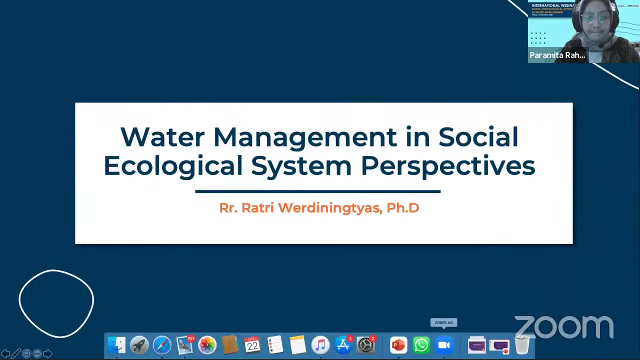 to the University of Melbourne To assess governance: Social ecological system framework to assess governance system. The time is yours, Murati. Let me share my presentation. Is that okay now? Yes, Thank you very much. Good afternoon for Indonesia and good evening for Australia. 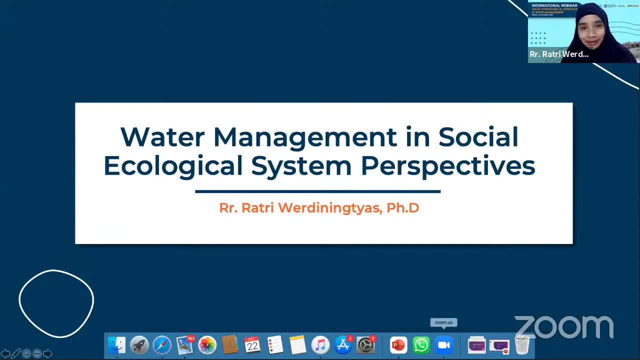 and maybe other participants from other countries I can mention. this is my pleasure to have you here. From the precious presenter we got already wonderful knowledge that stressing that Indonesia is a very important country And I think that's why I'm here today. 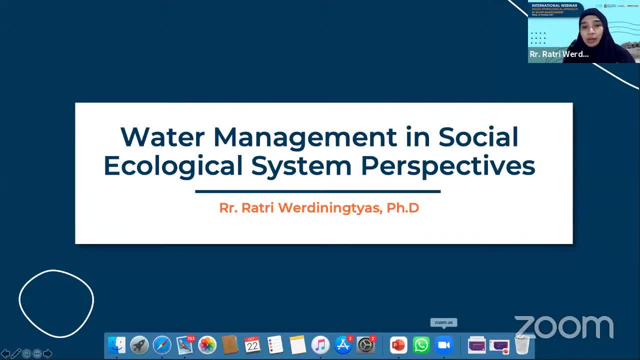 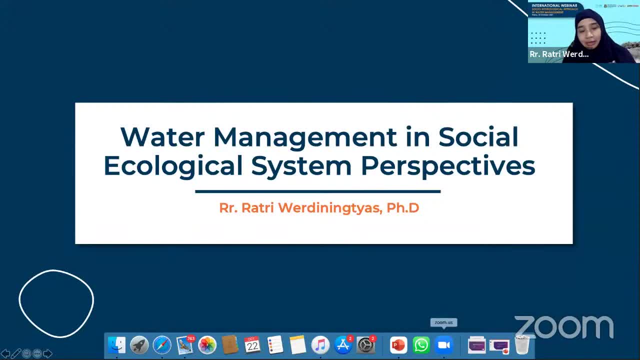 we cannot only think about technical consideration, But we also need to think up on the social section, which now nosis we also our most chance. it's not managing the water, but it's really managing the community or managing the actor behavior. 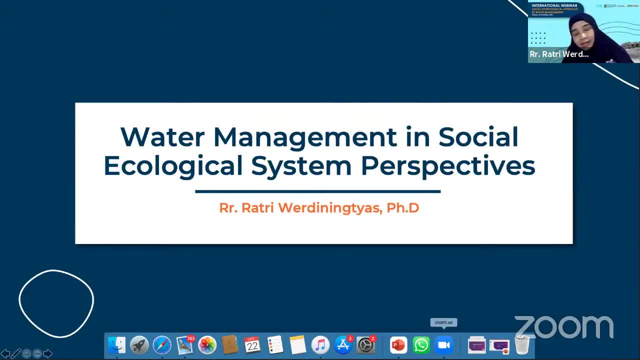 and dealing with water resource. In a country like Indonesia, water management has become a big issue. in some areas, the notion of availability is asymmetric with accessibility. Water scarcity, when comparing the resource to demand, is more relative than absolute. So for the closing presentation I want to bring another perspective, but also stressing about the importance of a social system when we are dealing with a 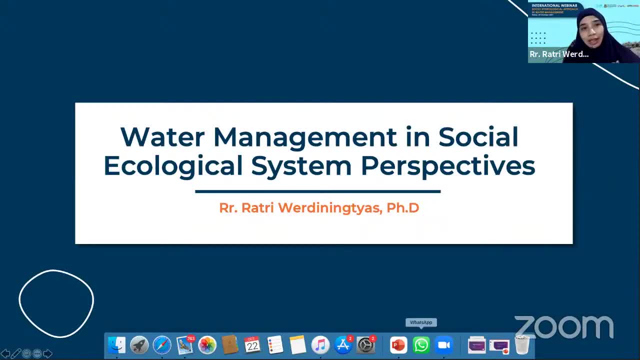 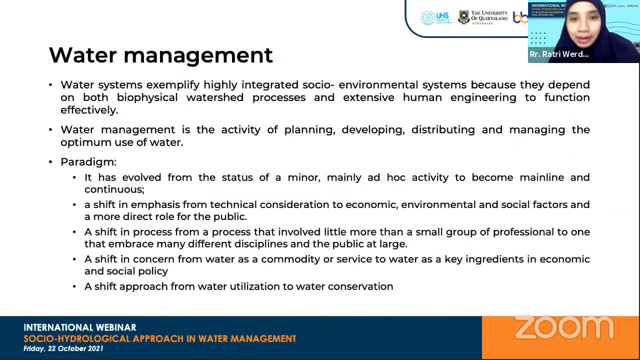 biophysical system, in this case, a water resource. My presentation is water management in a socio-ecological system perspective. As we know, water systems exemplify high integrated socio-ecological systems because they depend on both the watershed process but also how humans deal with their lives and manage the water. 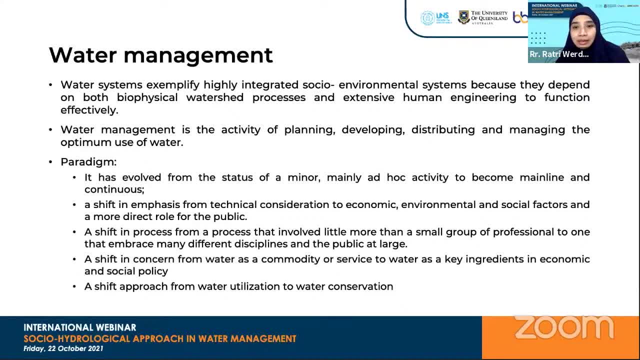 In the Anthropocene era like now, where nature doesn't have again its capacity to receive negative impact of human intervention. So we really need to be very careful in water management: how we plan, develop, distribute and manage the water to gain optimum use without treating future generation. 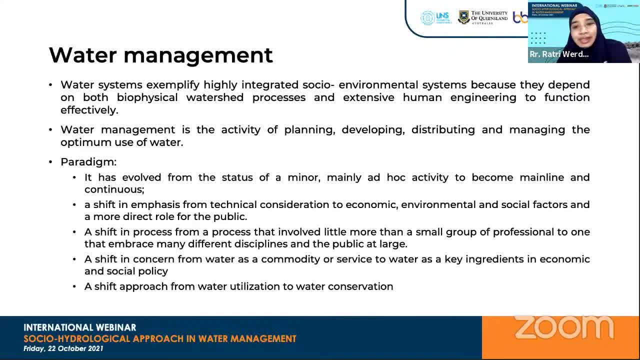 So if we can fast back to the last few decades, there is have some dramatic change in concept in water management. Water management has evolved from the status of minor, mainly ad hoc activity to become mainland or continuous process. So it's not only building a dam and expand the water infrastructure and that's the end. 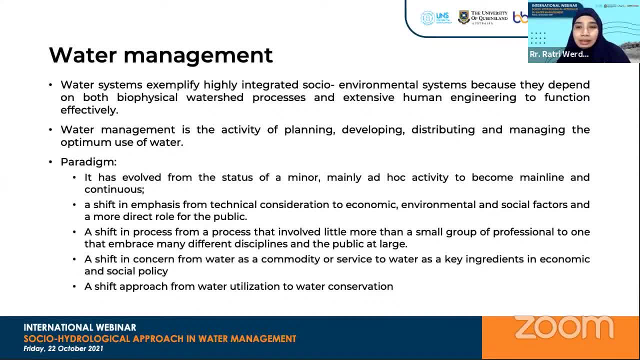 But we need to make sure that it will work and can benefit the public as it's targeted. So here we cannot only think technical stuff, but we need to consider also economic, environmental and social factor And also as much as we can improve the water. 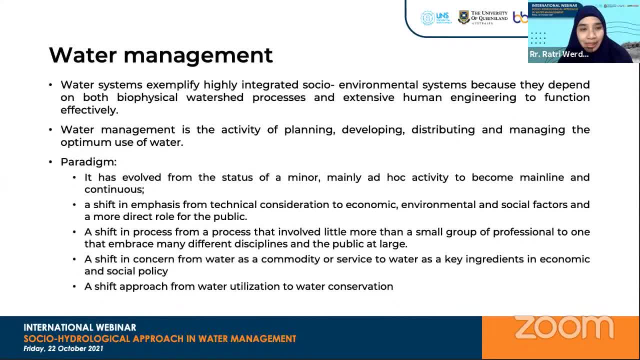 As we can improve the public so that it can be succeed As a consequence in term of actor. we also learn from previous presenter that nowadays in water management we don't only need engineer to take all the technical stuff, but we need to embrace many different discipline and the public in the same time. 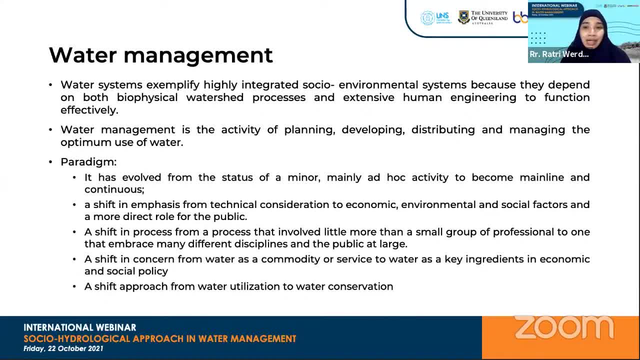 While the amount of water is fixed and we have increasing demand and pressure from growing population and also economic activity. So nowadays we cannot think water again as a commodity, but it's a key ingredient in our economic and social policy. And also we can see today there is also shifting. 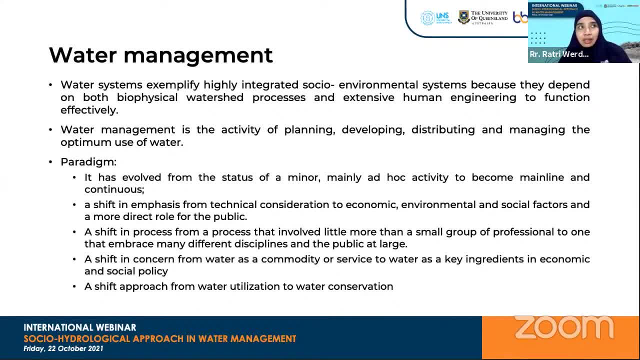 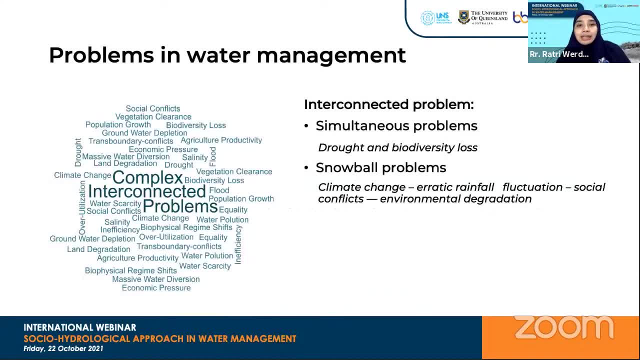 People are starting to think the importance of to do water conservation instead of think only water supply and its utilization As a highly social ecosystem. Talking about water In water management is really attribute to a single problem, But it's related to many problem which is connected to each other. 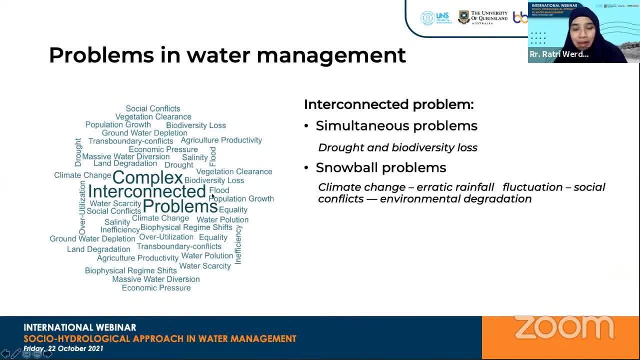 Also, like already explained from the previous presenter, For example, in the term of water, seed blood drop is- have relation with our catchment condition. We can just not blame that it's become a climate change. It's caused by climate change, something like that. 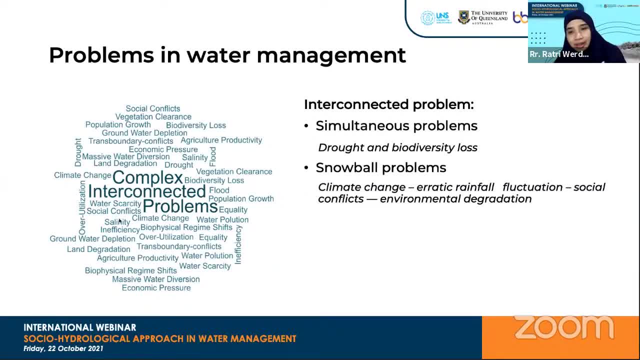 So when we are talking about water management, We are actually talking about how manage complex, interconnected problem that can occur in the same time. I call it simultaneous problem. For example, here, when we experience drought, there will be, of course, biodiversity loss. 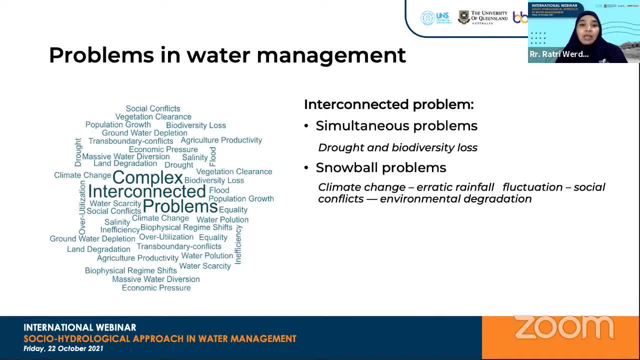 And as there is no enough water for the environmental flow or problem that create downstream problem and on the whole of the system, I call this snowball problem. For example, here is the climate change. It creates erratic rain population And because of that it's people water security. 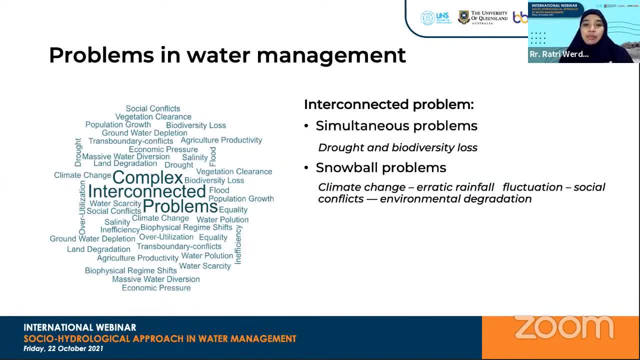 When people feel insecure about water, people tends to do action to save the interest, Which then led to the social conflict and also environmental degradation And that, at the end, destroy a whole system and make us further from what we are dream of about sustainable water resource system. 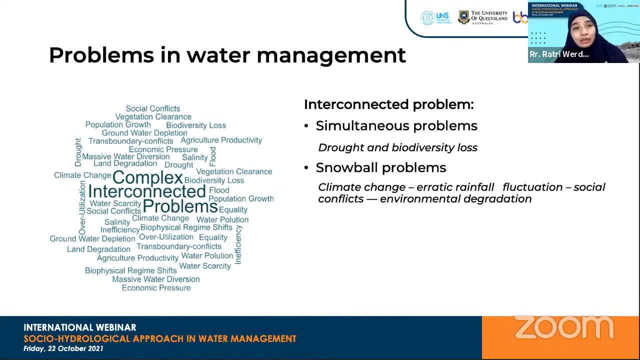 So you know. So in water management we try not only to cope with many existing problem which are correlated to each other, But it's also to minimize negative impact that could happen in the future because our incapacity to solve the current problem. 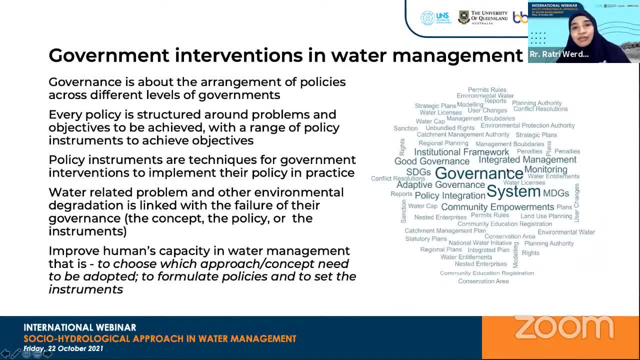 Talking about government intervention. Actually, we can say that it's ranging from the concept to policy instrument. Let's see. The first actually is about the arrangement of the policy across different level of government And where every policy is always formulated based on problem and objective, with a range of policy instrument. 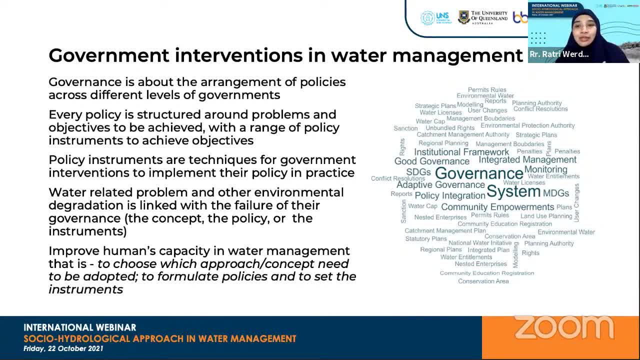 And the policy instrument itself are the technique of the government to implement the policy to practice. So watching and even experiencing how government in adapting and surviving from various problem related to the water. We also familiar with hundred approach, Like already, maybe also some speaker also explain approach of government to try to do like we can see in the figure here from the concept. 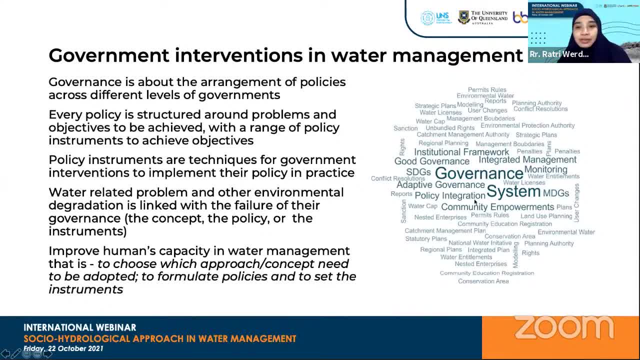 Like they want to adapt into IWERM, record-based engagement management, Try to empower the community and also adaptive government and so on. And also they also try to implement many policy instruments like plan permit, user test and rules. So and I will agree that here that water related problem and social and other information relation happen is linked with the failure of this approach we choose. 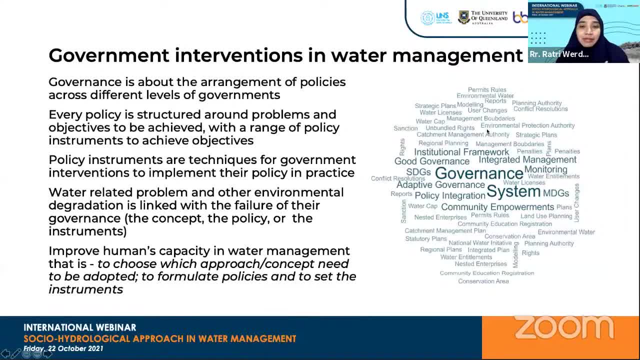 So the only thing that the way we to cope with this problem is by improving our capacity in water management, That is, the capacity of us to choose which approach or concept need to be adopted, How to formulate the policy and how to set the instrument. 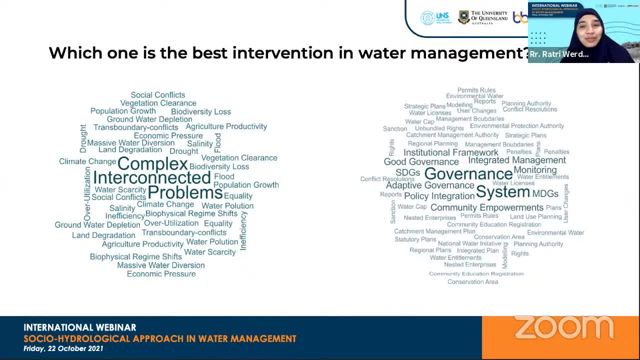 As so many participants here is coming from many government agency, If you are asked to drive a land from which government intervention you will choose to solve a problem is in the left side. We will understand that there will be a big possibility of various land direction. 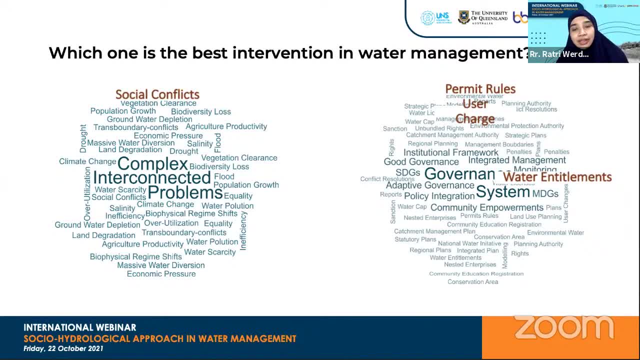 For example, to manage social conflict in water distribution. Some people will think license permit user charge is the best solution to make sure everyone get what they afford. But some other will say we cannot take the charge or make difficult to people to access water, because water is human right. 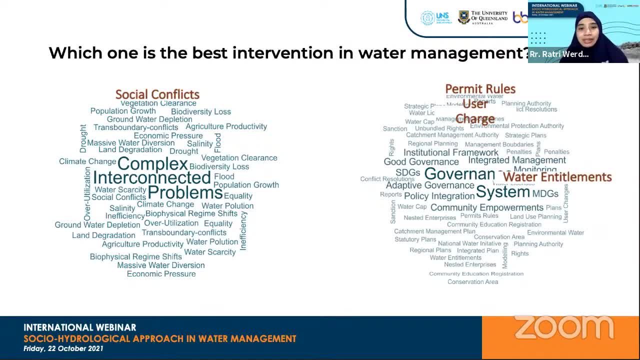 So we need to. we cannot take a charge for this. So here the government will choose how they will deal and manage water based on their perspective, knowledge, capacity and, of course, the context, specific condition of their own region. This is also happen to other problem related to water. 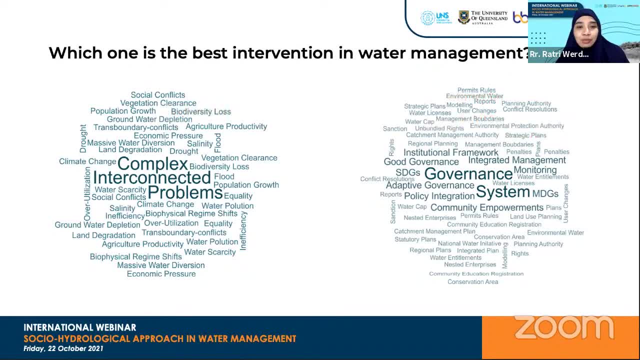 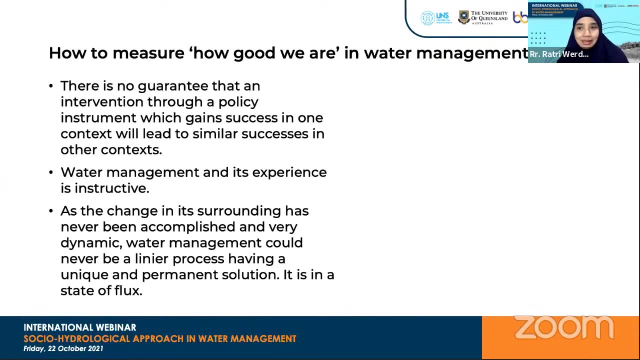 There will be more than one alternative for people to choose. So so there is no. so actually, there is no general prescription how water needs to be conducted as condition which water management is, a place, very context. It's context specific within the region. 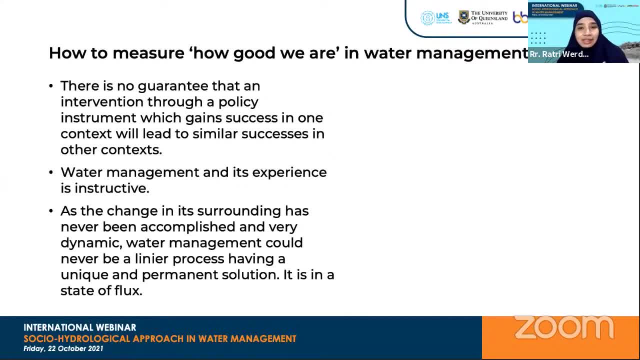 In a number of cases change in government intervention has resulted in considerably negative impact instead of promotion of the social condition as it's targeted. So we actually cannot just duplicate other government intervention for solution, because there is no guarantee that intervention through a policies instrument which can success in other country or other region will lead similar success to also. 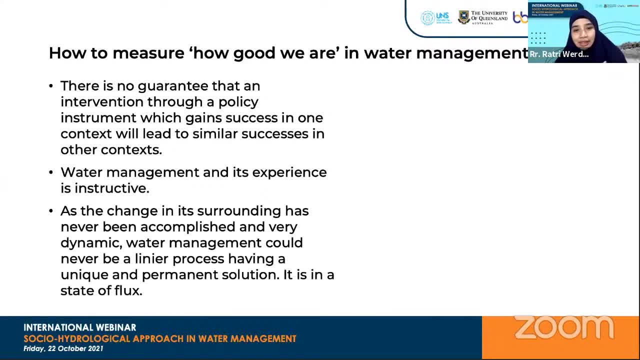 to our region In deciding which intervention actually water management is. human learning process. we learn from our experience and improve ourselves to deal with water. So water management and etc. is instructive and it's not a linear process because with permanent solution, because the change is of surrounding is very dynamic. 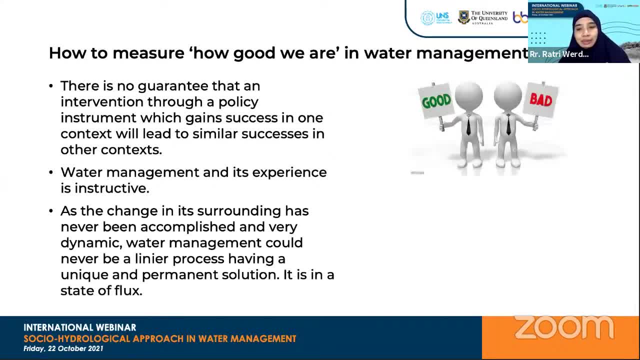 So to improve water management, So to improve water management, To improve our capacity to be better, we need to understand how good and bad our interventions are. now. Are we good enough? Or actually we don't know that we are good or bad? 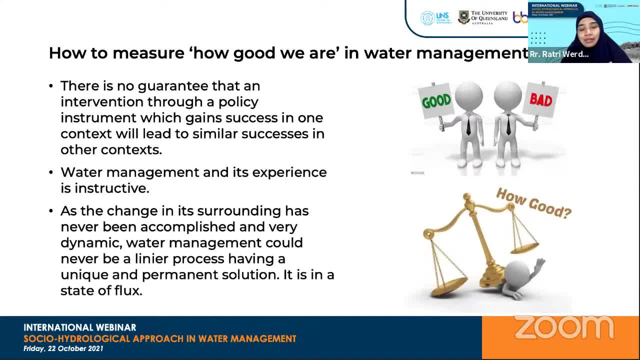 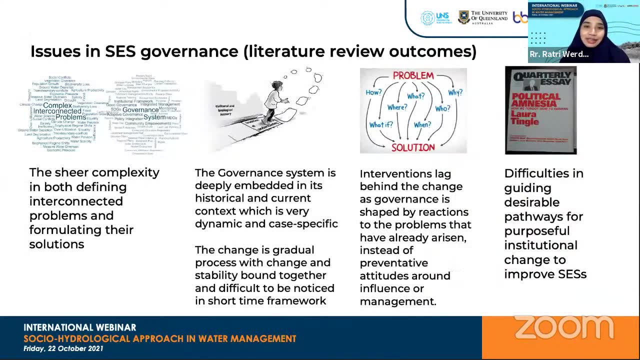 So the challenging problem here is how to understand that, where we are, we are good or we are bad. 35 minutes remaining, Oh my god. So we just over said that we are in grid 5 or something like that. Sorry, I said that. 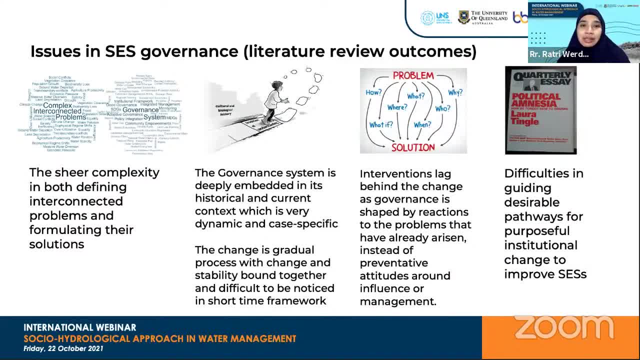 So there is in the literature. there is a common global issue in the social ecosystem government. It's also in the water resource government that I explained interconnected and also the government system is a slow mode when stability and change wants to be together. 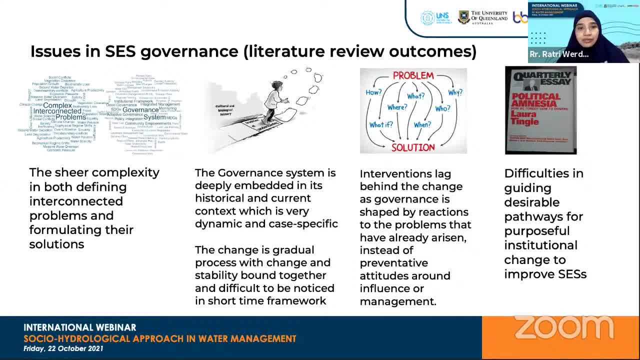 and it's very difficult to understand in short-term work And also the intervention given by the government usually is lagged behind and political amnesia that it's very rare that a government makes learn from the history. they are the tendency of the government to concentrate on the existing problem instead of learning how the problem. 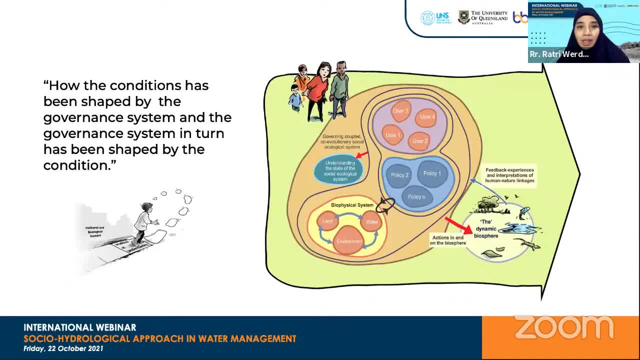 occurs because of the precious action. So the main problem here is: we don't know, understand. we don't understand how the condition has to be signed by the government And how the government system in turn has been saved by the condition in the practice. 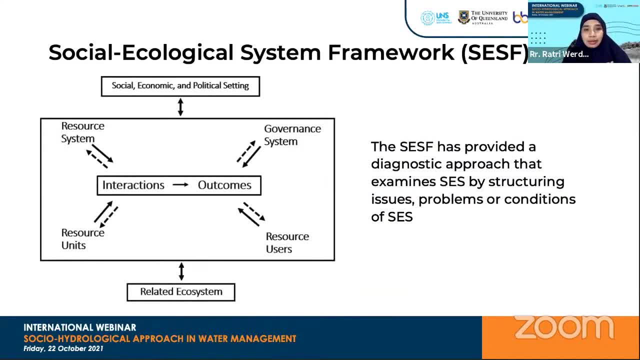 And that is a very big problem. And the framework of socio-ecological system, framework in the last three decades, have been motivated to understand that. So, proposed by Ostrom, the framework is very useful framework to elaborate our condition in managing socio-ecological system. 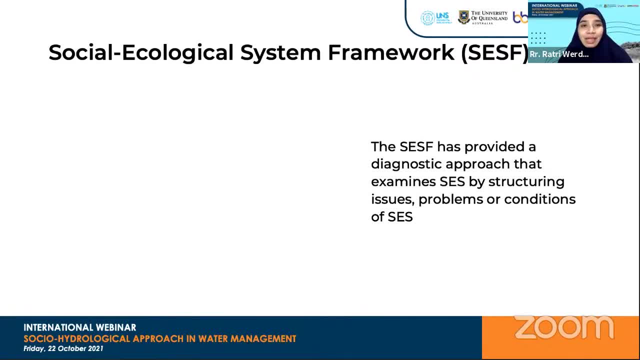 Maybe because of the time, I need to skip it. I'm sorry. Actually, the framework is very powerful and already used by many scholars across the world. to this cricket: instrumental issue: identify problem and risk. conclusion of what the socio-ecological system condition. 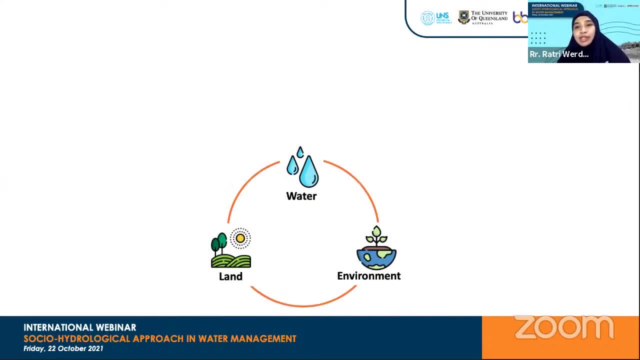 When we talk about the socio-ecological system, for example, we want to elaborate the condition of our Western system. Actually, we will not think about it. We will not think about it. We will not think about one resource. We also not think about one resource user. 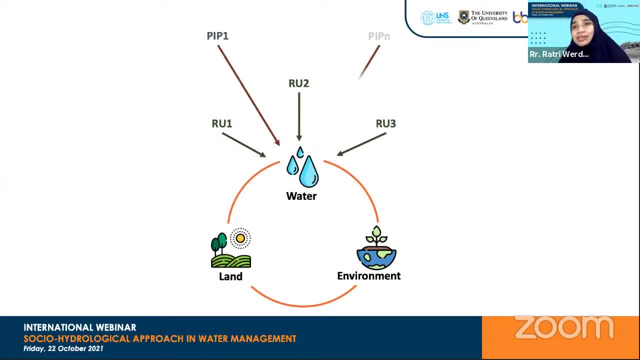 There are many resource users. We are not thinking about one public authority who is responsible to water, So water government actually try to manage how the interaction between resource among the resource user and also how authority with resource user and also among the authorities itself. 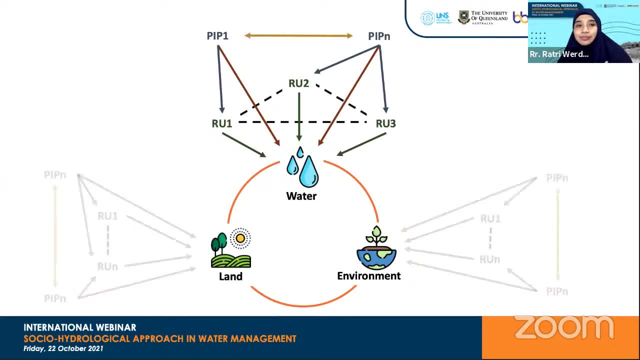 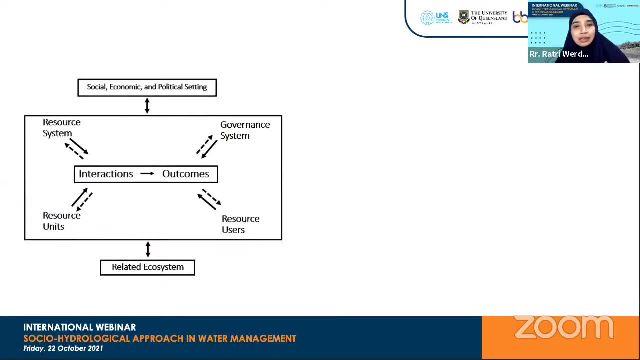 So it also happened to other countries. So I think it's a very important point. So here in the Ostrom framework the government system is treated by a certain variable. here outside The framework doesn't consider the rule of government in directing the interaction hundreds. 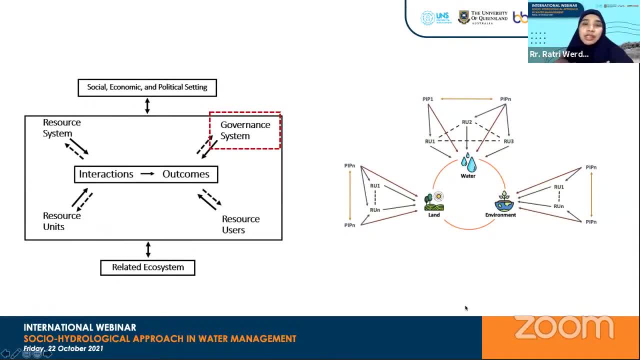 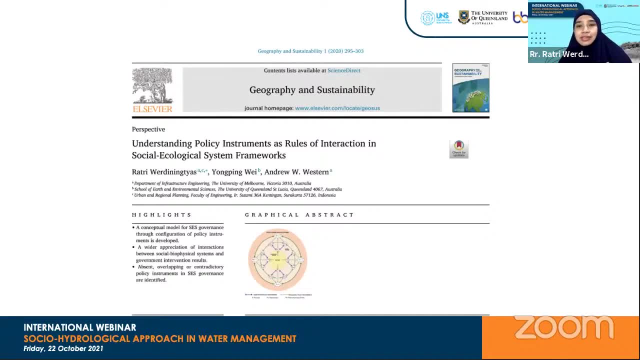 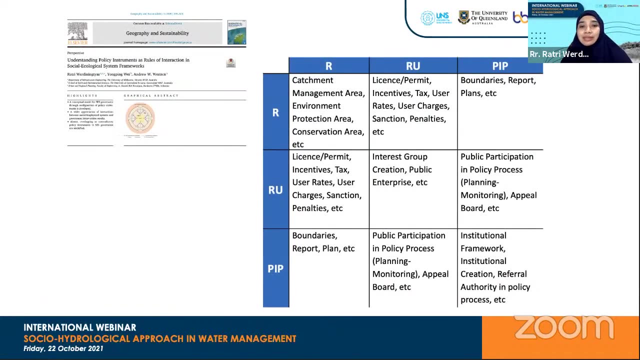 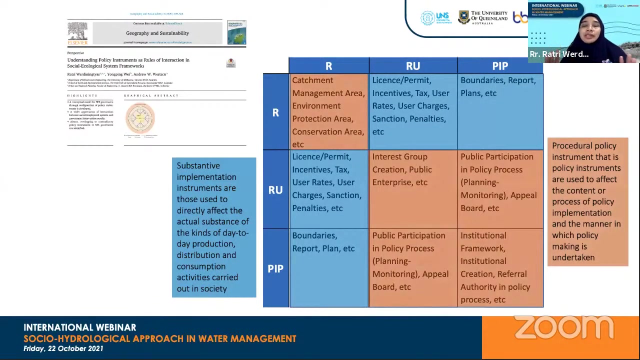 of interactions that can happen because the dynamic interaction between a socio-ecological component. So here we put a government system and energy system by put policy instrument. policy instrument that is two kind policy instrument, that is, substantive policy instrument and procedural policies instrument, and both of this policy instrument actually try to manage the interaction. 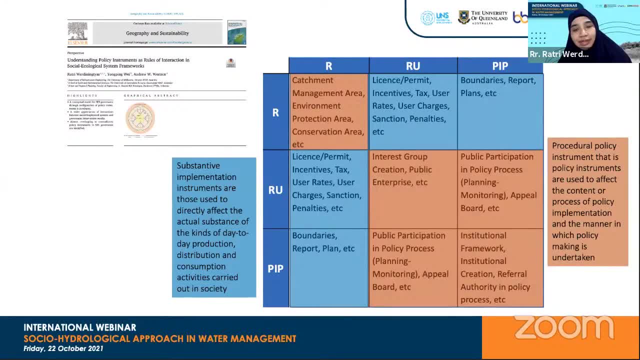 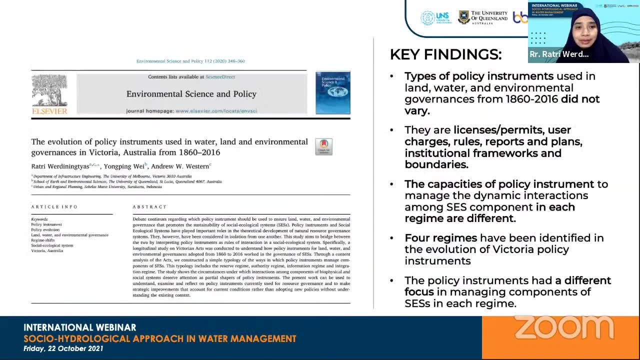 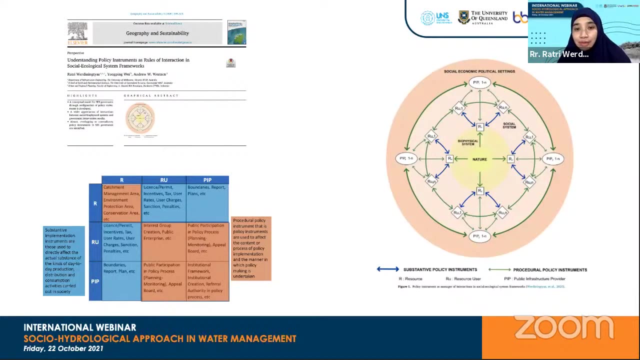 between resource, resource teaser and public infrastructure provider. So we propose four tier systems. We try to propose a four tier framework that is, try to make a general about the interaction, about component of socio-ecological system actually is managed or regulated by policy instrument. 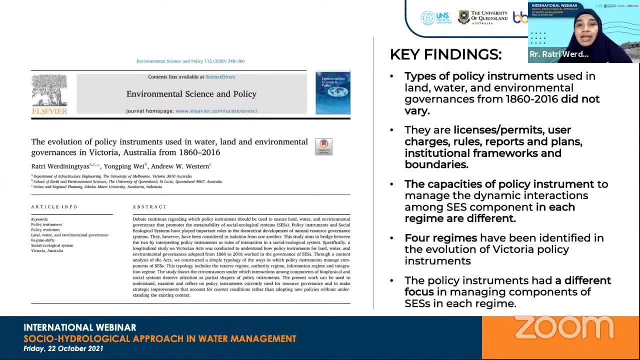 We have applied that framework to four tier systems. We have analyzed the policy instrument used in Victoria government from 1860 until 2016.. And we found that actually the policy instrument used by Victoria government is not vary from the 18th century until 19th century, but they change in their capacity to manage the interaction. 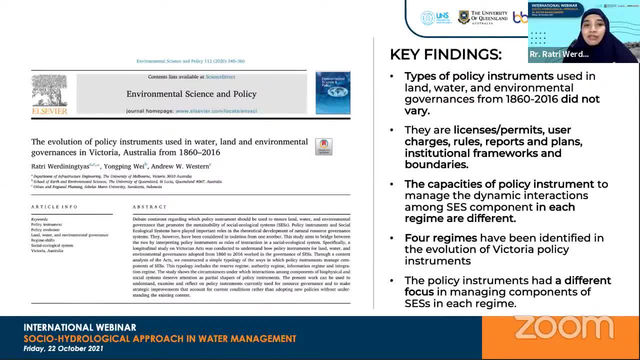 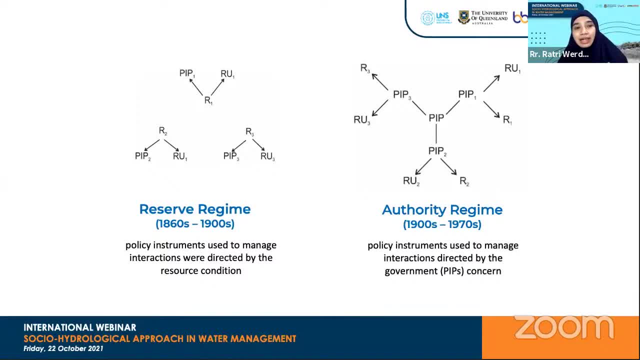 of component of socio-ecological system And there is a four regime. We can identify that first is reserve regime from 1860 until 1900, that at the time policy instrument used to manage interaction was directed by the resource condition. The second one, in the authority regime, is policy instrument used to manage interaction. 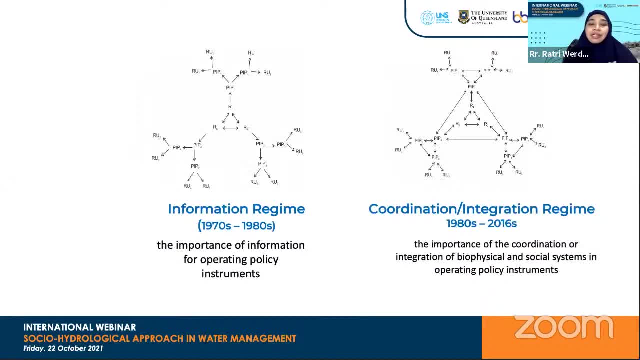 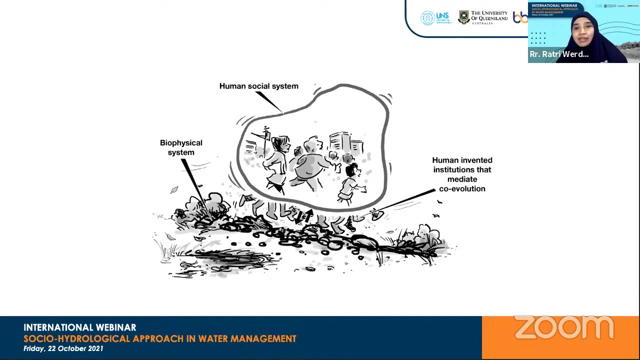 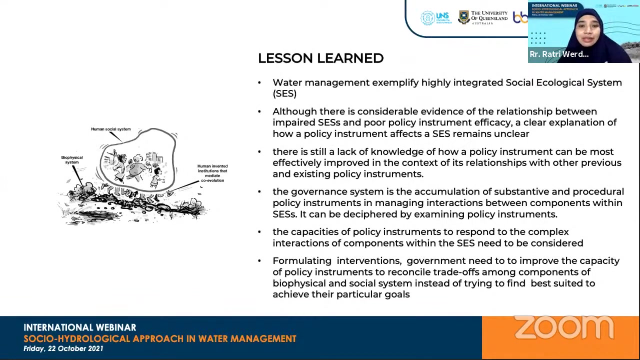 directed by the government concern. And the third one is by information, by physical information and the latest one from Victoria, the important of the policy instrument 示 the fantasies. So the first idea, so by mind, can be 1994: we integrate physical, working or social systems. 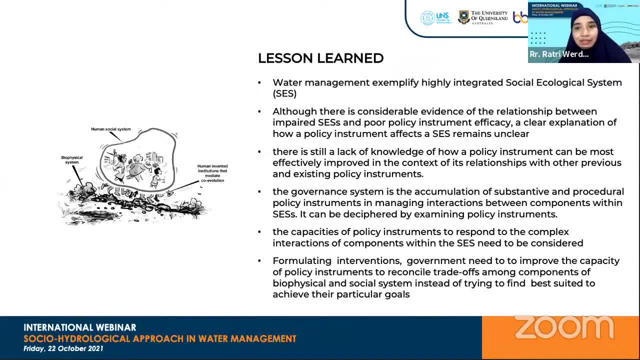 very challenging work. from the framework i have explained before we can see actually the government system is the accumulation of substantive or procedural policy instrument in managing interaction between component uh social, ecological system. so understanding the government system can be dispaired by explaining the implementation of the policy instrument, examining the policy. 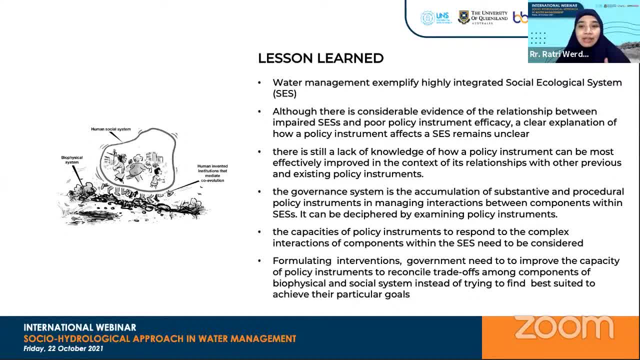 instrument is mean we need to understand the capacity of our policy instrument to respond the complex interaction among components within a social ecological system. by doing that, by understanding that it will be helpful for the government to formulate intervention in water management because actually for improving government need to improve the 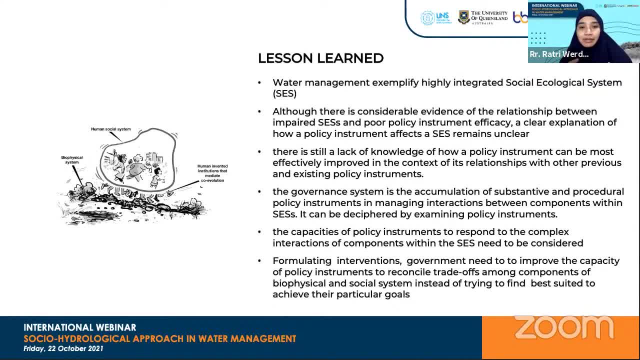 capacity of the policy instrument to reconcile the threat among the component biophysical and social system. instead of trying to find the best, uh uh, try a famous policy instrument that is a sucker in other countries than adopted to achieve their particular goal. I think that I can explain for today's presentation. 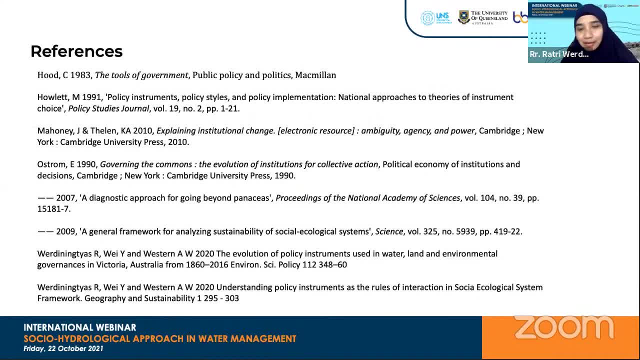 Thank you very much. Time I give back to Miss Mita. Mita, Yeah, Buratri, thank you very much for very interesting presentations. We didn't pass the time limit A little bit, So we discussed about complex interconnected problems, right? 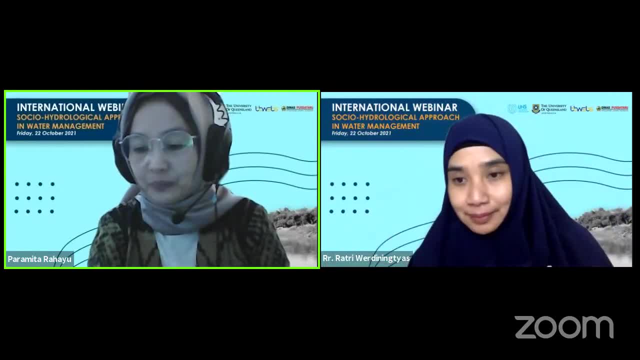 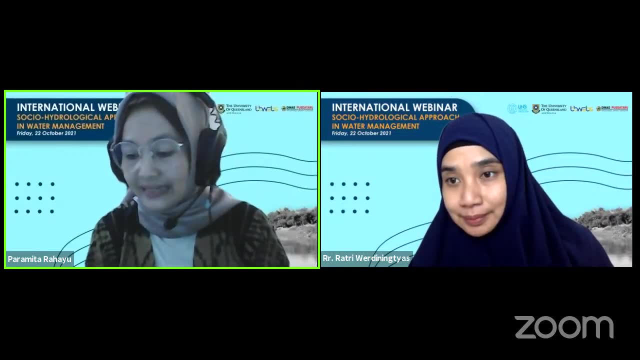 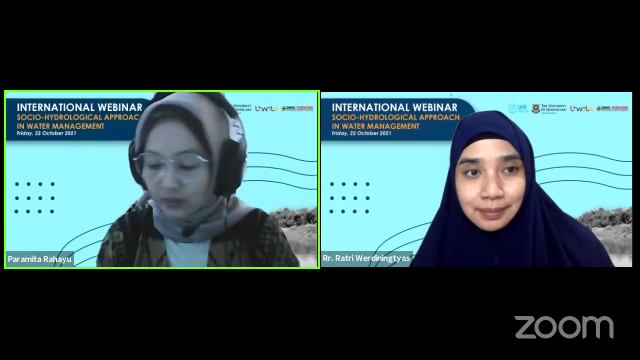 So water management is about complex interconnected problems and the governance system. to understand how good we are, So we have to understand the policy instrument applied over time in the refurbishment area So we could apply the best policy instrument for certain refurbishment with its program. 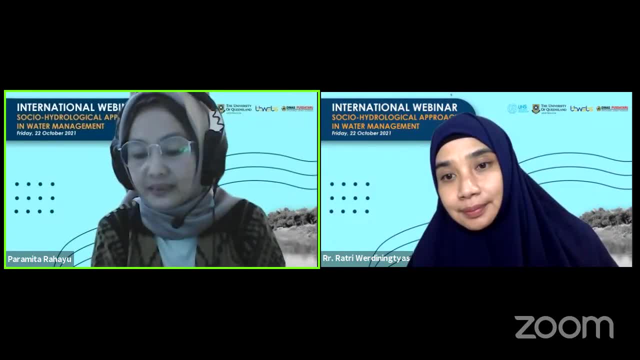 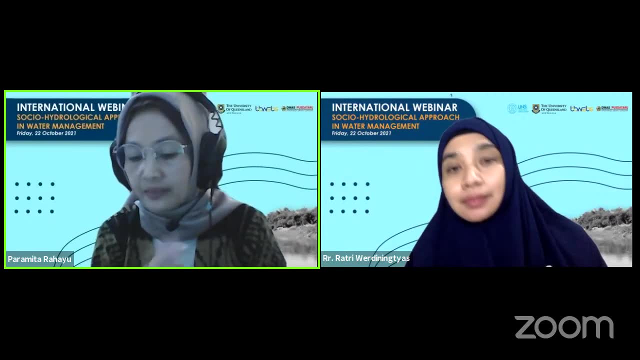 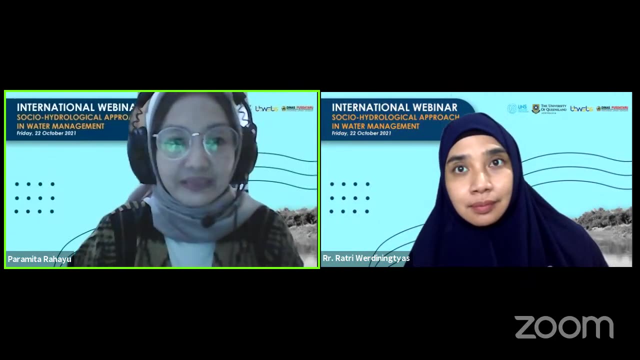 So we have to put attention about the complex interconnected problems, the governance system, how good we are And through the understanding policy instrument over time we can understand what are best to apply to the certain refurbishment problems or water management problems. Thank you very much, Buratri. 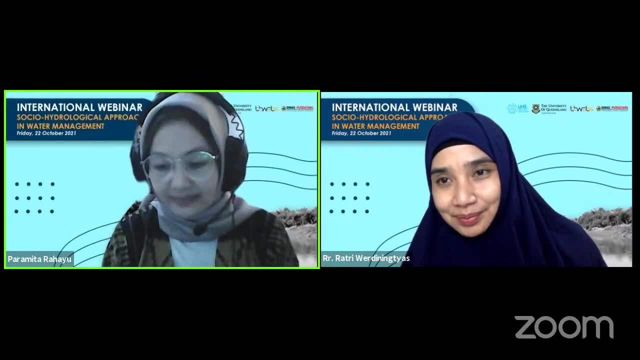 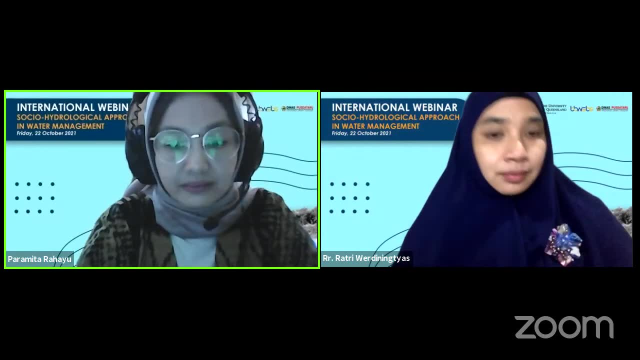 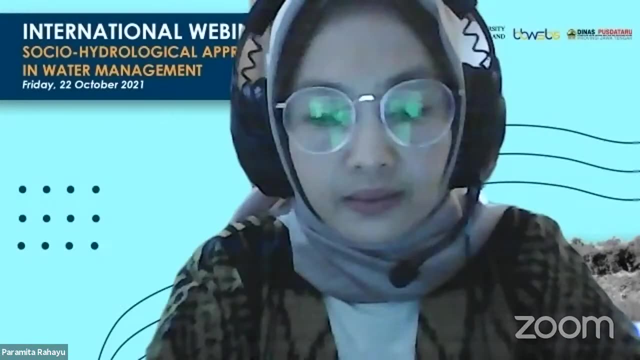 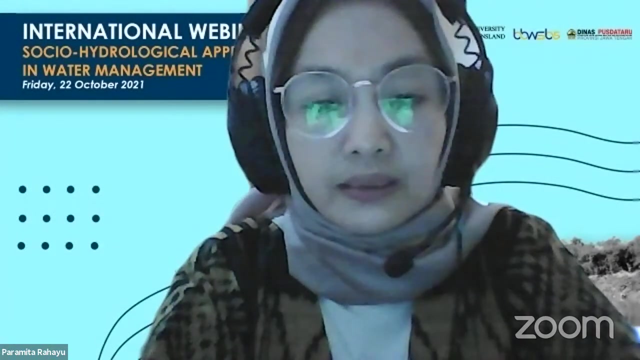 Now I think that's the last presenter. Then we will go to Q&A session, I think, And let me Let me see the several questions that we received here through the G4.. The first question is addressed to Dr Frederick Bookert. 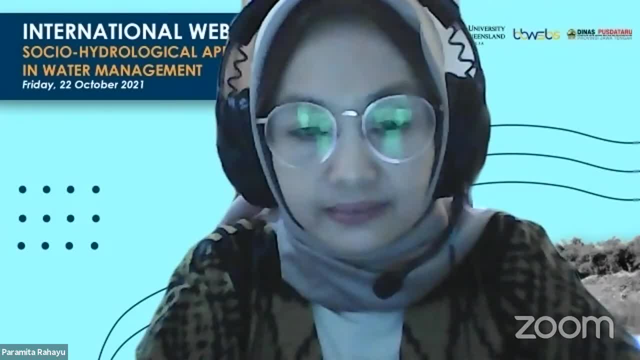 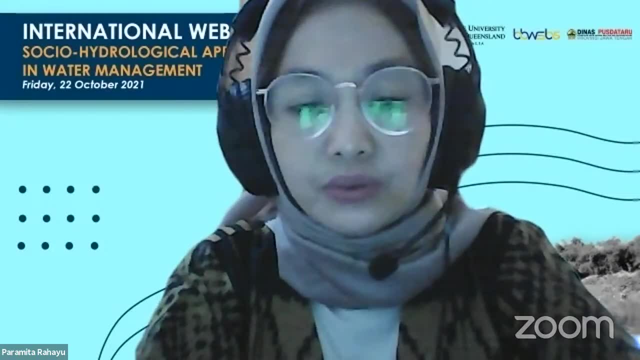 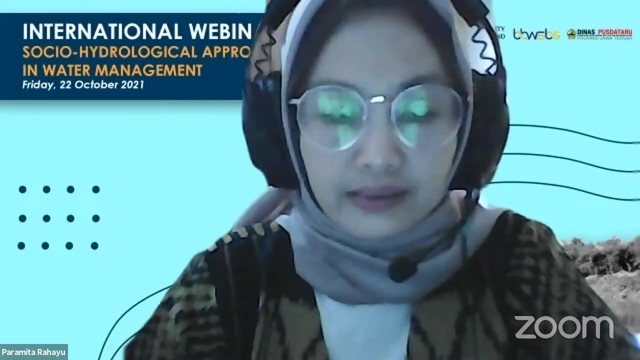 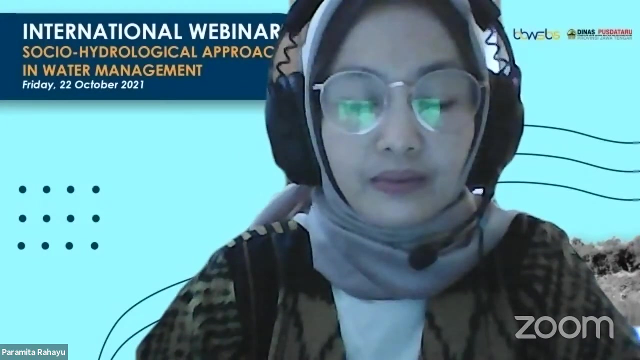 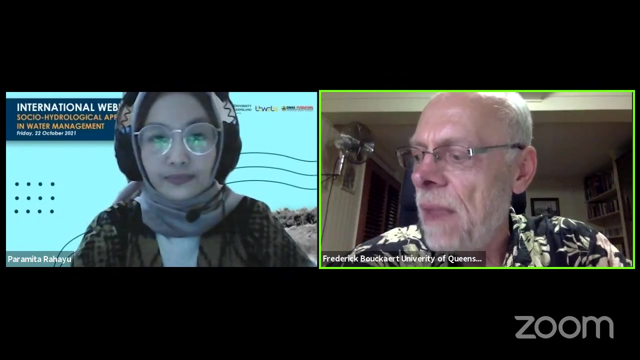 It's about in what extent the role of community can be defined to improve the social institutional capacity. Please, Dr Bookert, you can answer the question. Thank you for that question. It's an important question, I think, because the role of community, I think, is very important in two respects. 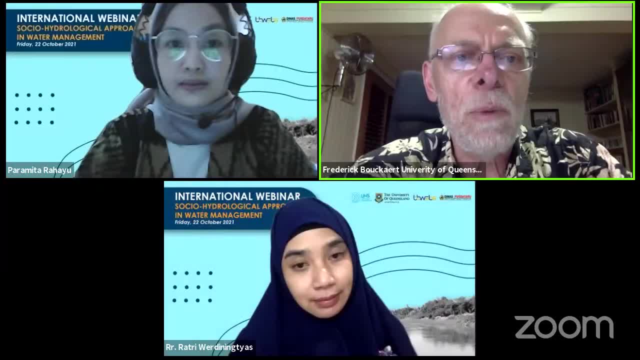 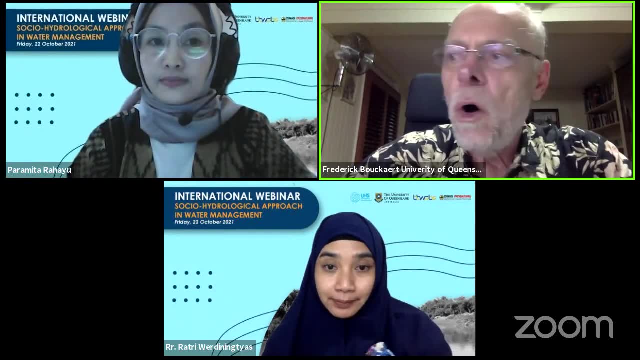 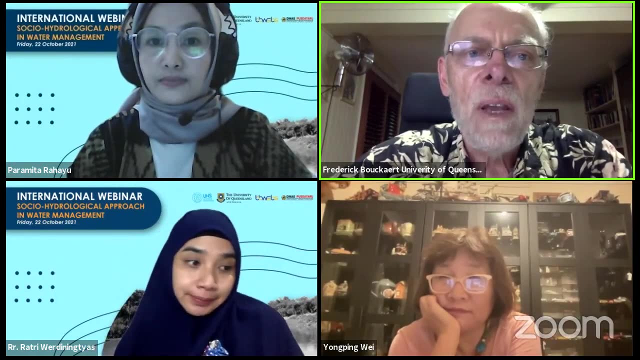 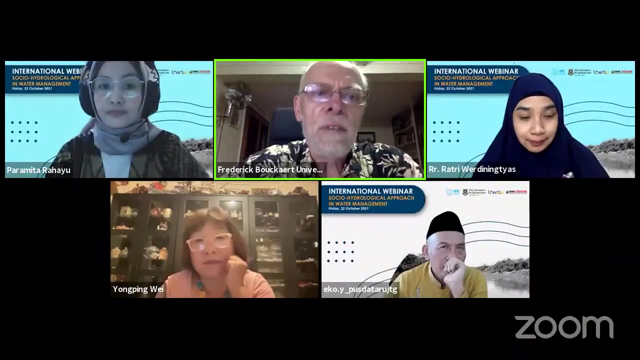 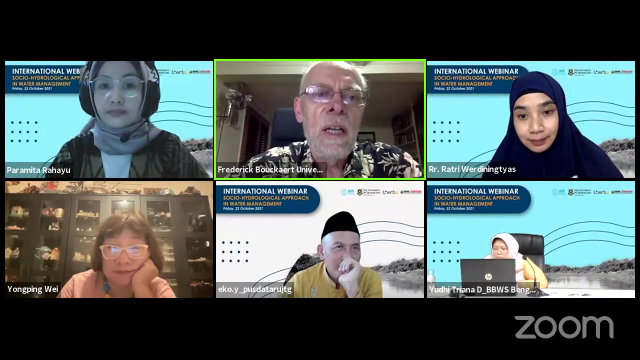 One is that, in a general sense, that the community needs to be able to agree On how the policy is being developed and how a basin plan is being developed and implemented in general, in a general sense, But the community that lives in the river basin, in particular, I think they need to also have a voice in this whole planning process in the sense that they are also affected by some of those decisions. 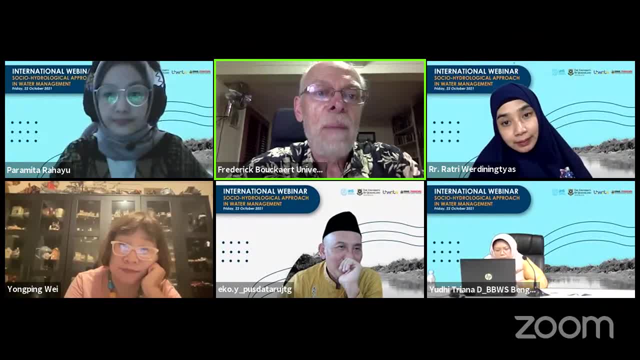 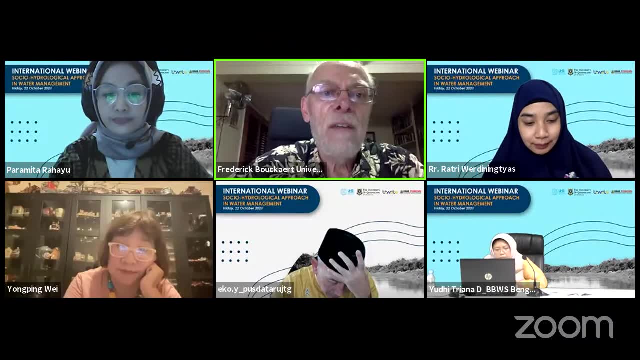 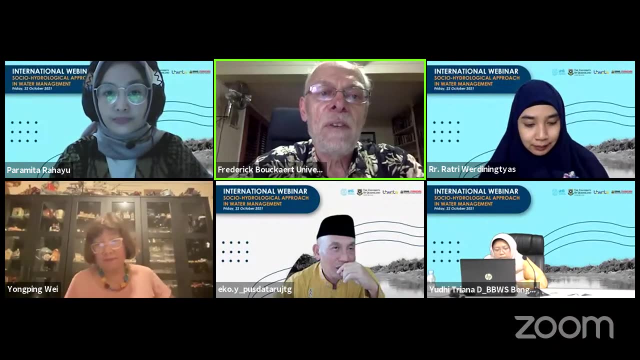 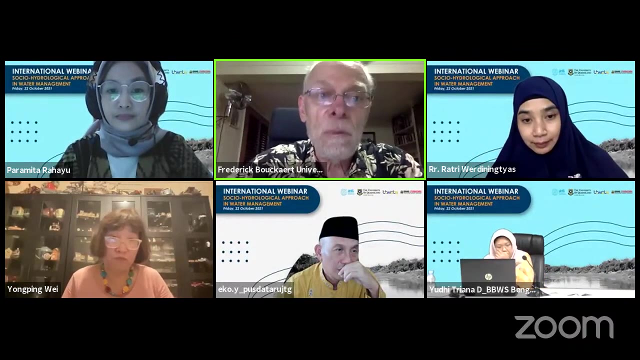 They are water users. They basically. if suddenly there is a decision made to build a dam, for example, to have more water storage, it might mean that some people get displaced from where they are living. It might mean that they might not be displaced but their homes might be in danger because they are situated downstream of a dam. 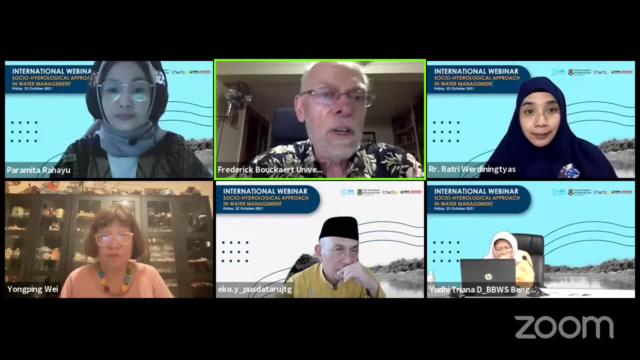 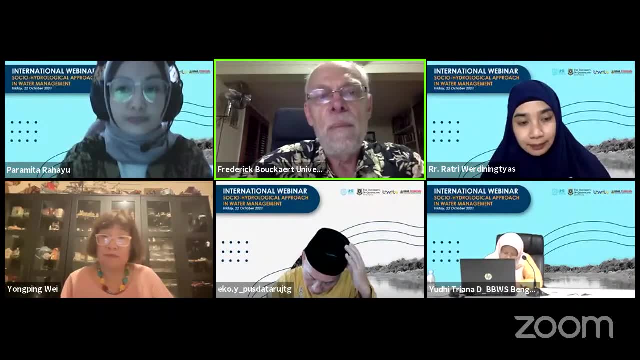 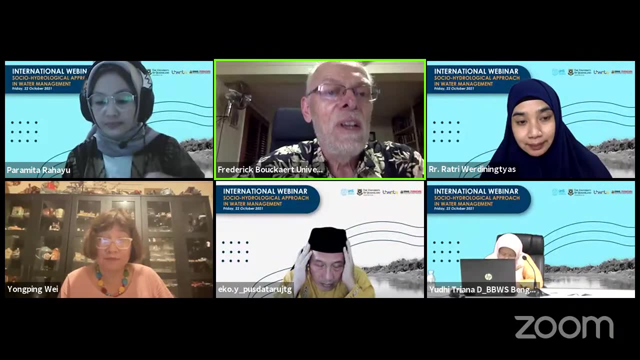 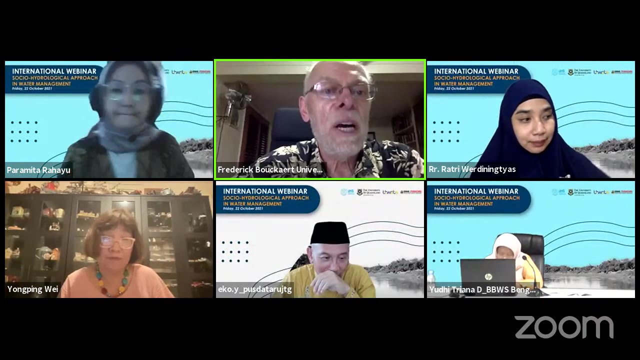 So it's important to listen to all the voices of the community. Thank you, And in fact, the members of a community living in a basin was one of my categories in my analysis, So I think they need to be consulted and their voice needs to be taken into account in the planning process. 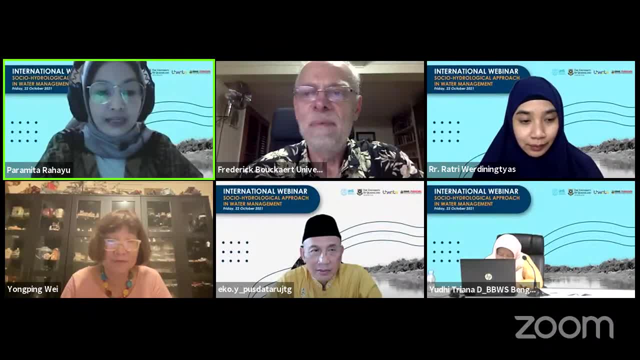 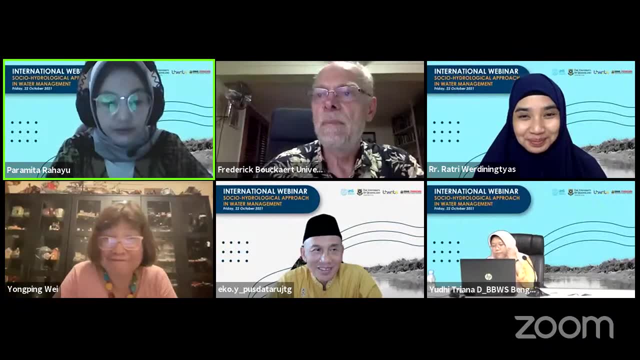 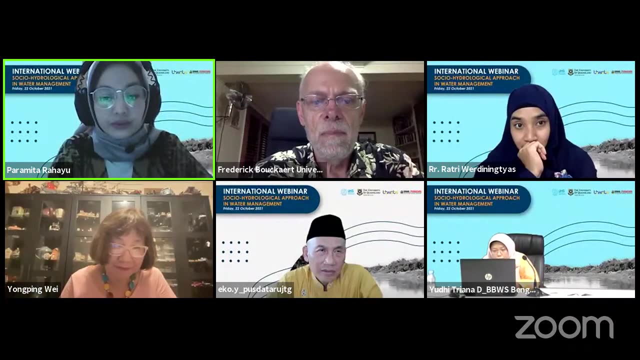 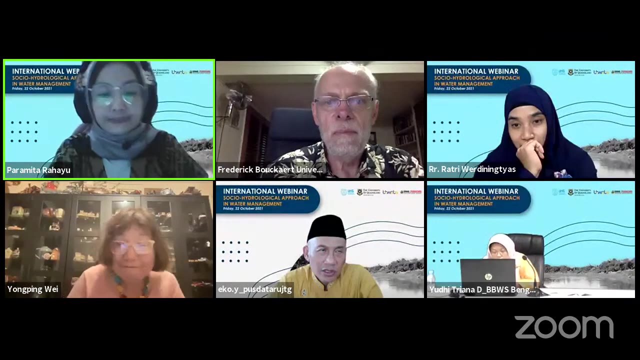 Thank you very much, Dr Bookert. And the second question. And the second question is for Professor Yongping Wei. Since social is such an intangible substance, what is your idea to measure the social aspect to be engaged with water resources management? 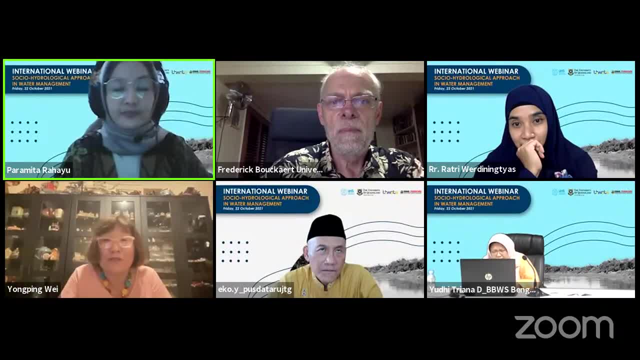 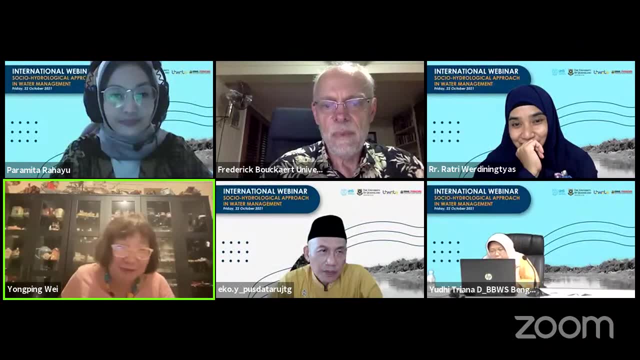 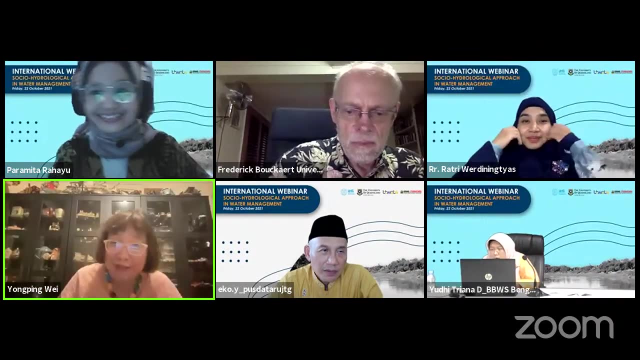 Thank you. That's really really important question. It's really really challenging question to address. You know what means social Engagement is social, Technology is social, Policy is social And our value is social. Our opinion is social. 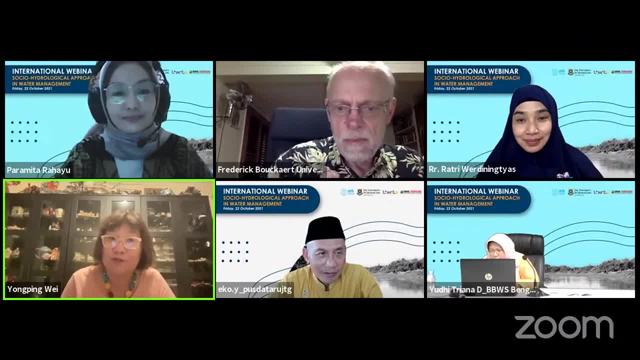 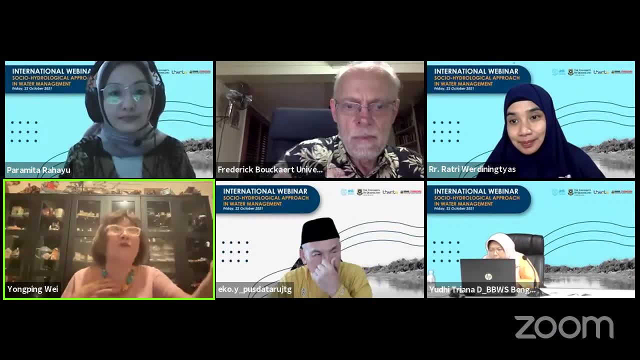 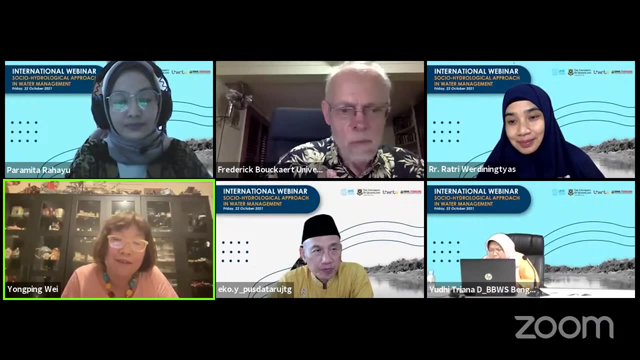 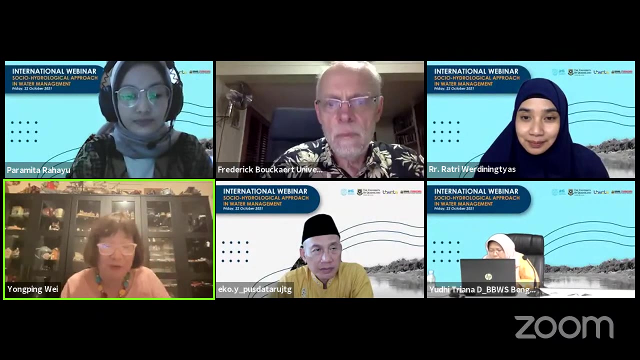 So in the last 100 years, social science takes very quantitative research to tell what's your opinion, You're good or bad, How good you are, like Rachi said, But I think in this transformation generation, we're living in the digital learning era. 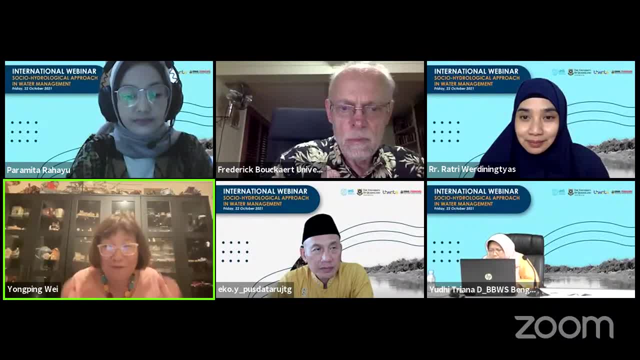 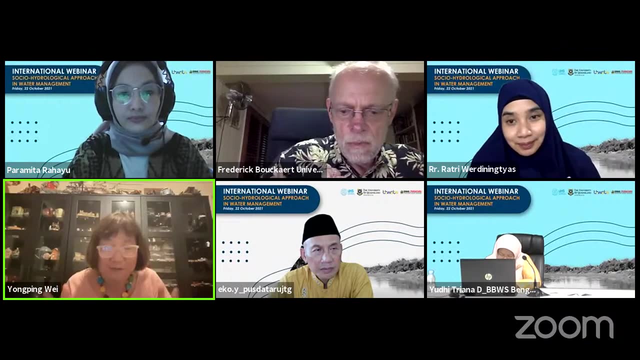 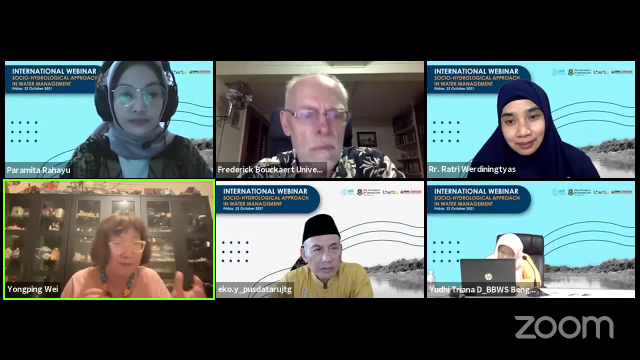 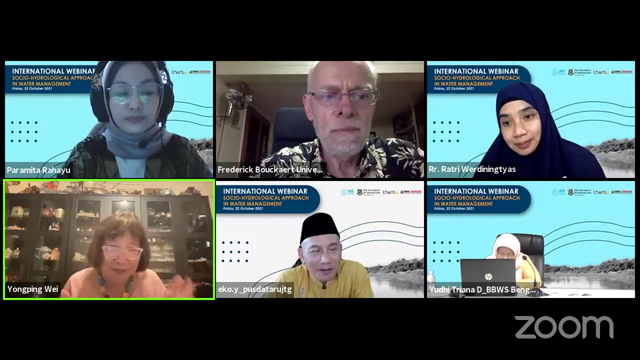 We need to digitize quantity for all our social aspects: Policy, technology, opinion and engagement. So that's what I have done, My group has done last 10 years, And we try to quantify all social aspects, Enable them to be integrated in the traditional biophysical model which has been developed by our quantitative for our social scientists, hydrologists or other modelings. 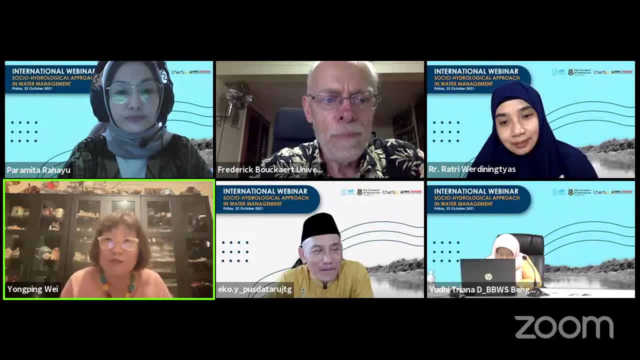 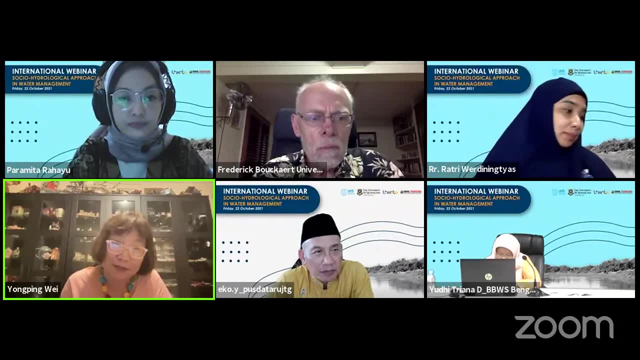 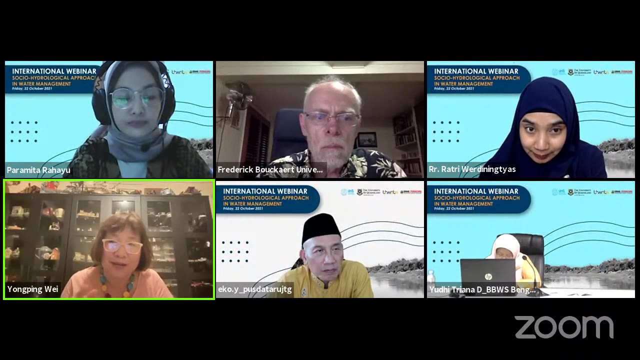 So the ways we do, We do integrate social science, We do integrate social science, social science methodology and the text mining approach to integrate a quantitative approach and a qualitative approach, to make the quantitative contents to be expressed in the quantitative, quantitative way, to enable the traditional social aspects or variables to be quantified. 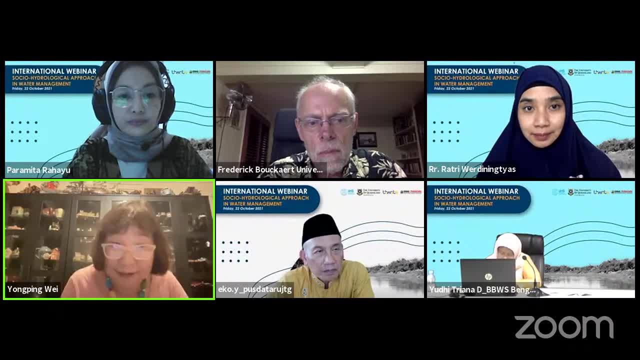 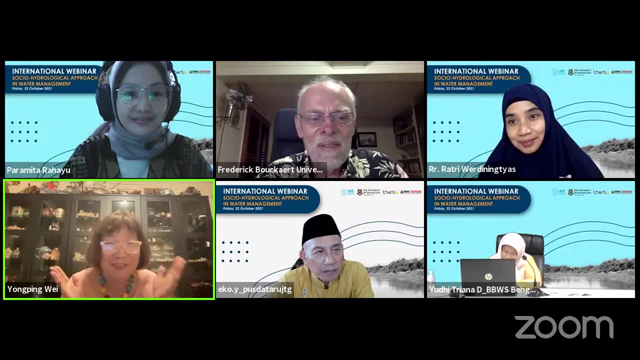 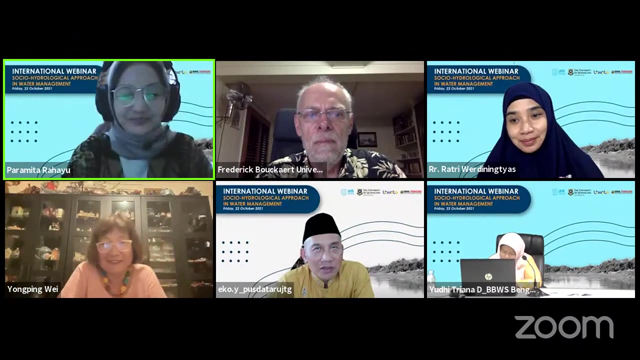 to integrate it in the process-based understanding. thank you, probably too much, but well, welcome any. any time you have any questions, you have my email, then talk to me. i'm very excited to explain how social aspects can be quantified, thank you. thank you very much, uh, our third question is for. 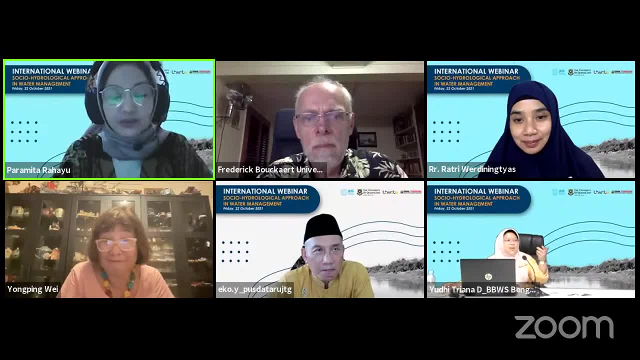 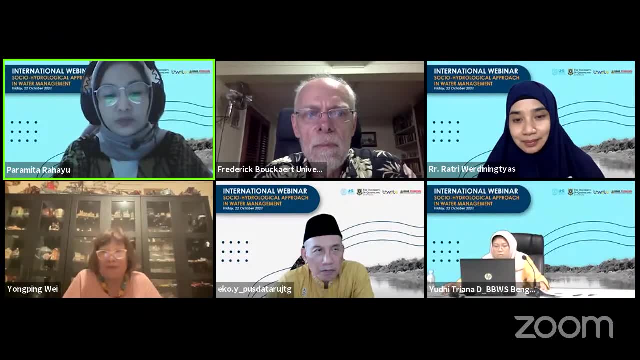 Bu Yudi uh in water management concepts. in order to do good water management, we should at least know about input and output in water cycle. but in Bengawan solo we are lacking in those items. we don't have comprehensive data about the input and output in water cycles. 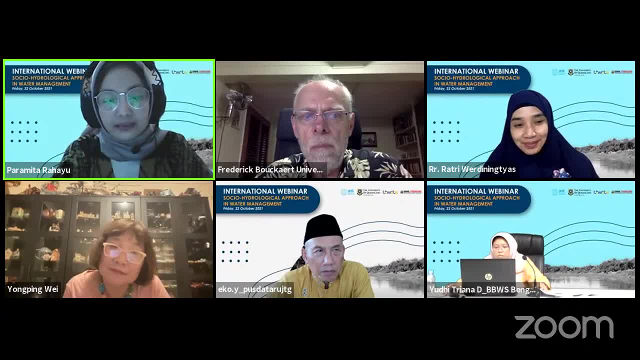 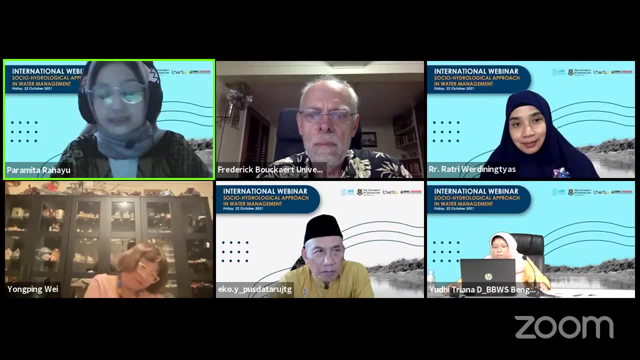 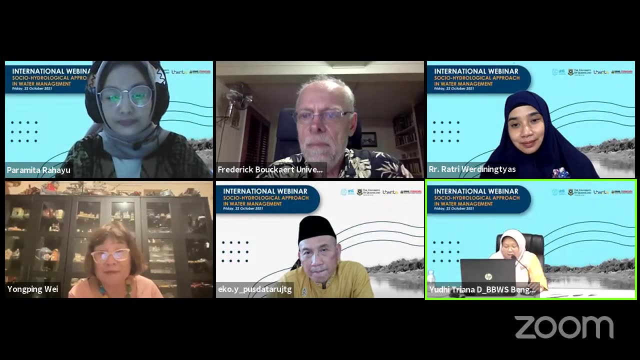 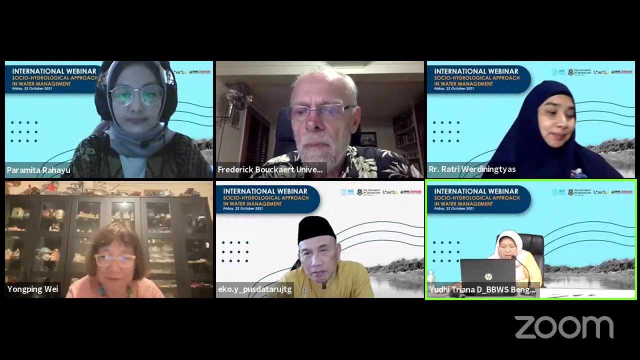 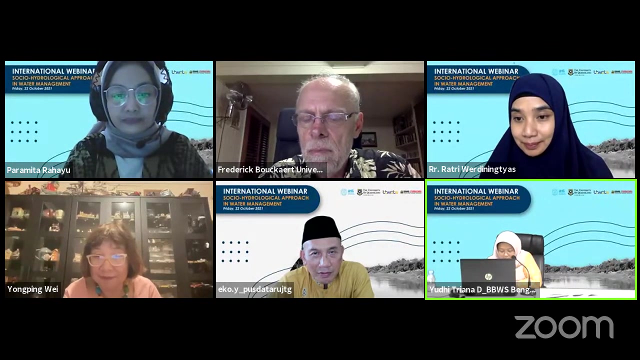 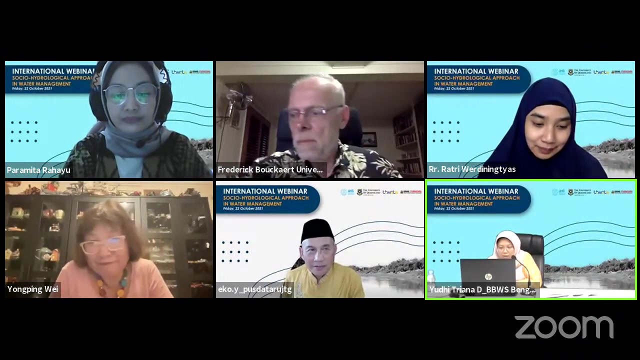 water cycle. what i would like to know is that, in that conditions, what we should, what we should do to improve water management. okay, thank you very much for the question. we try to answer uh about the input and the output, especially for uh our discussion today. we want to highlight it also about the social. maybe, uh, this social aspect, like what we discussed. 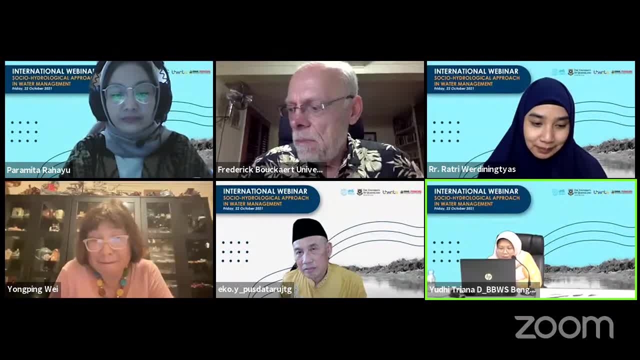 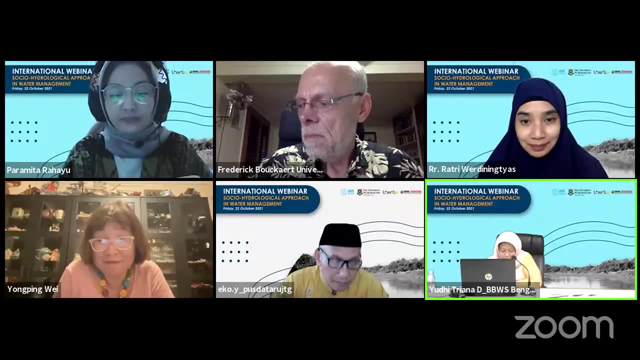 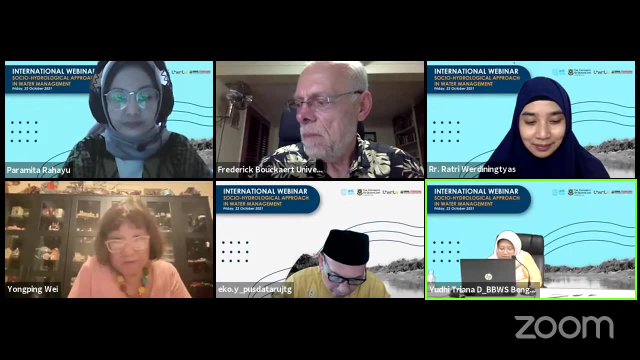 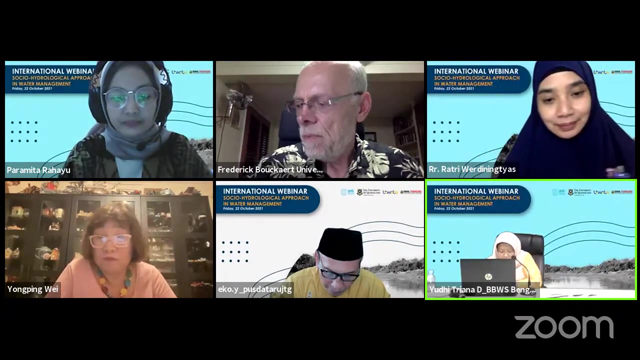 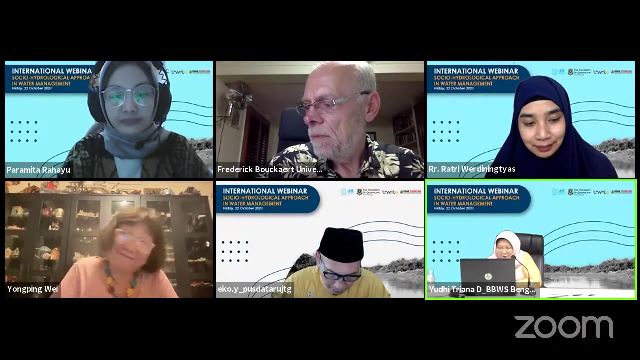 with professor young ping and uh, dr poker. uh, right now we have water councils that embracing all the voices from stakeholders from many regencies spreading along the pengawan solo, but we are not yet quantified the social acts aspect like: uh what, professor young pingway? maybe this is our homework, ibu paramita and 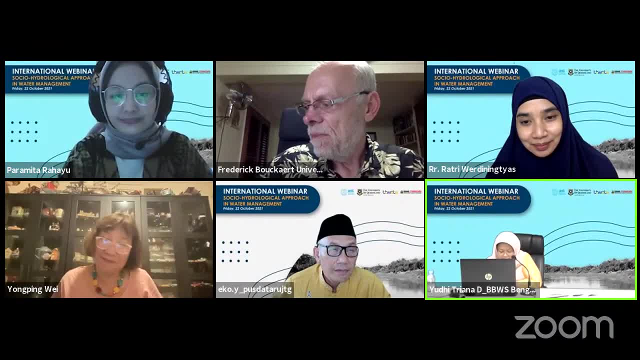 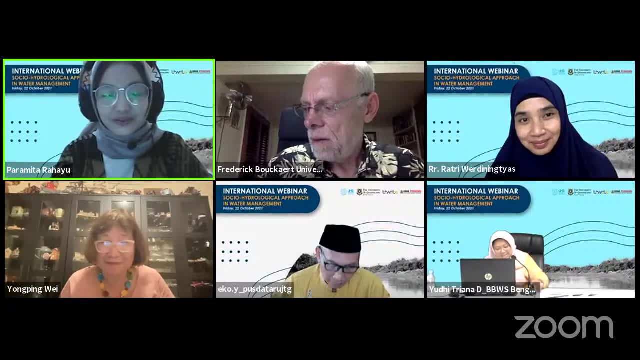 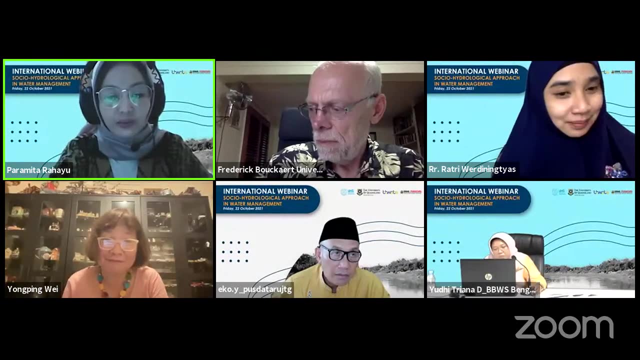 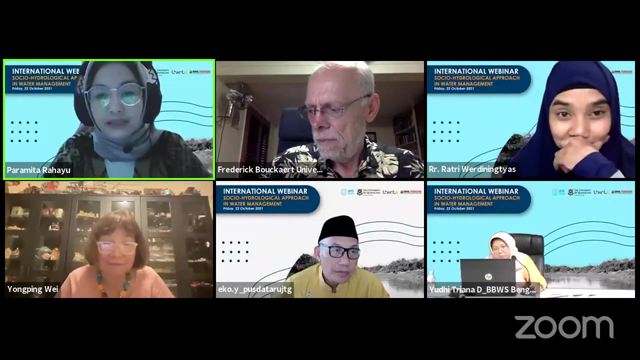 for next time have to be more concerned about this uh social aspect. i think that's our answer. yeah, thank you, and uh more questions will be for uh. another question will be for paeko: how to synchronize the management of bengawan solar river by pusdataru and bbws in overcoming 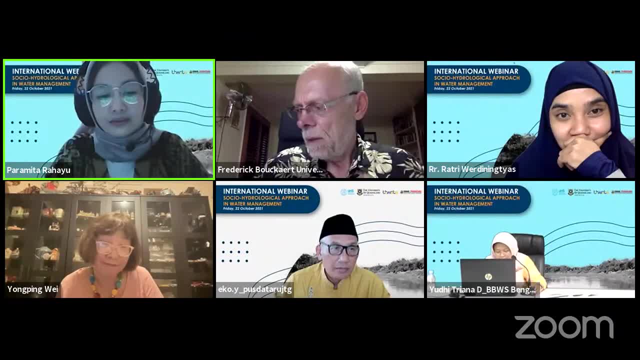 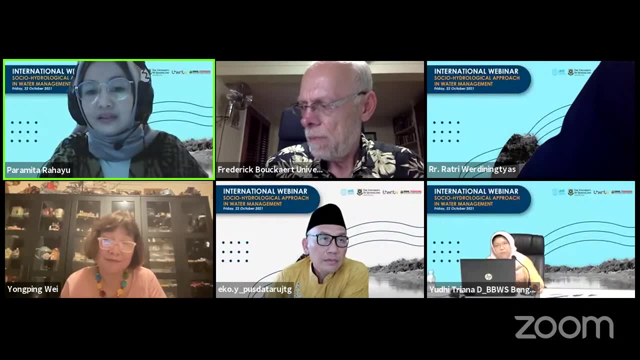 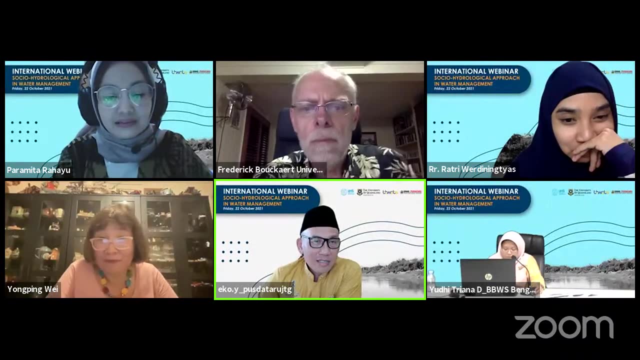 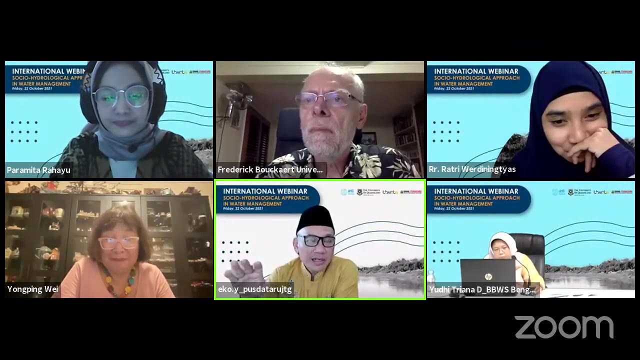 settlements on the river area that often interfere with the run, smooth running of the river. okay, thank you, uh. i will try to answer, but maybe it is not the answer. you know, because uh bengalan, solo uh river basin is the authority from the central government, so 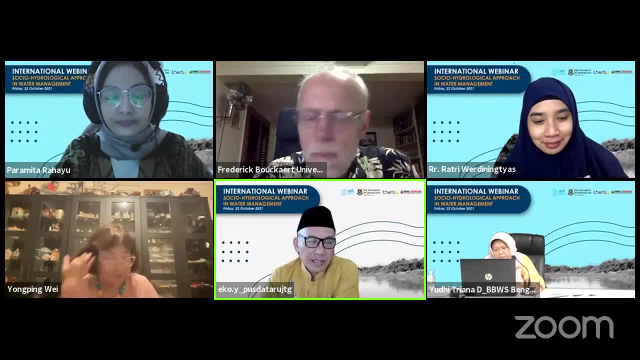 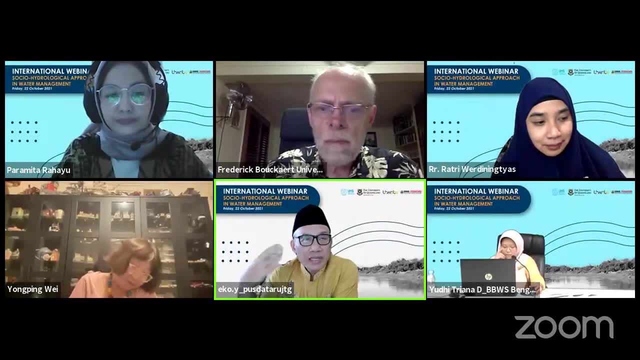 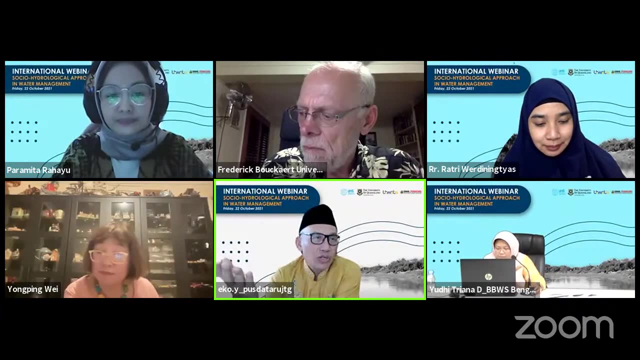 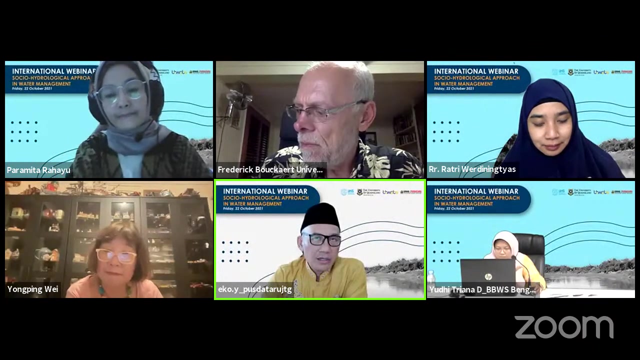 if the local government and then uh, district or city government have activity about the water resources management should be coordination, and then we have to permission from the authority. so what we have to do, in line with what the bbs will turn in the next, i think the key point is like: 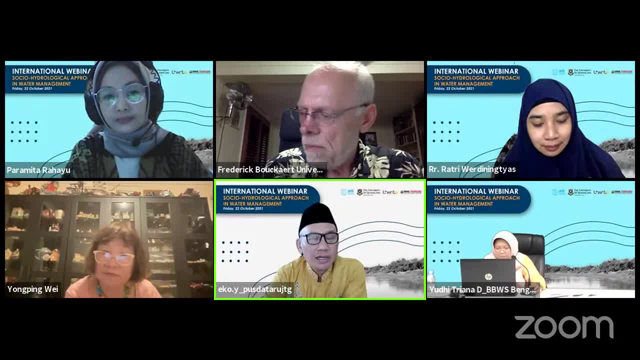 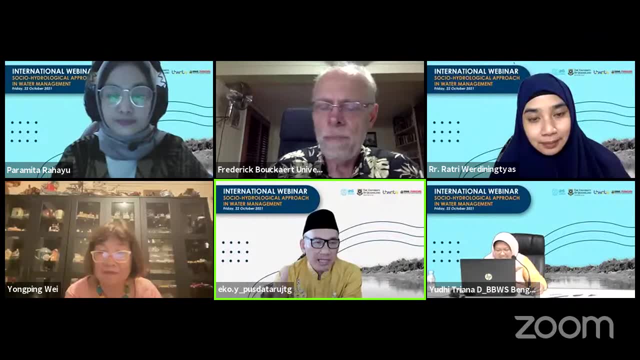 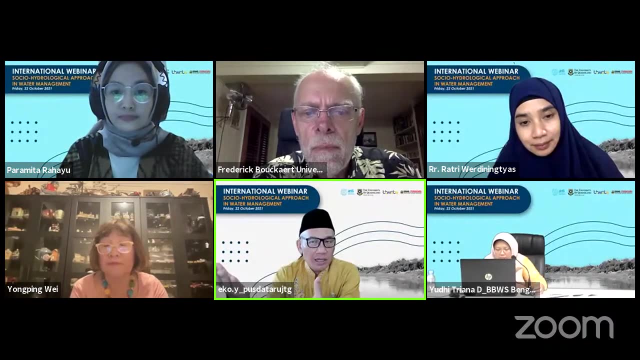 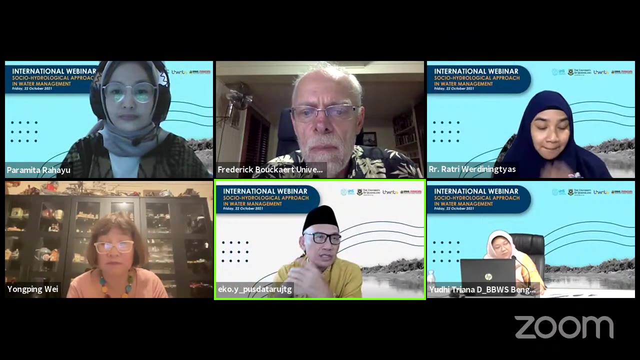 that. so, especially for water resources in uh uh solar river, i think it's this one, except we have uh the mechanism for the muslim bank. like that. this is uh should be done, but the uh about the water resource management we have to in line with the uh uh bbs, because one of the 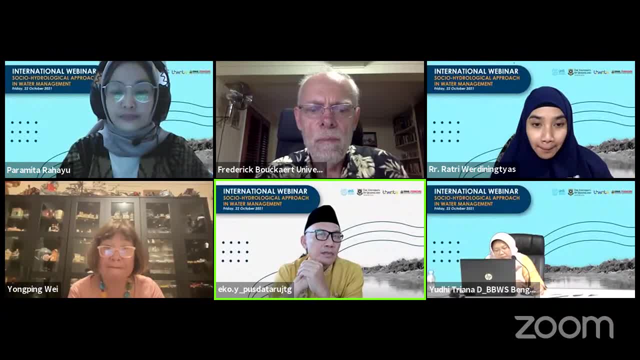 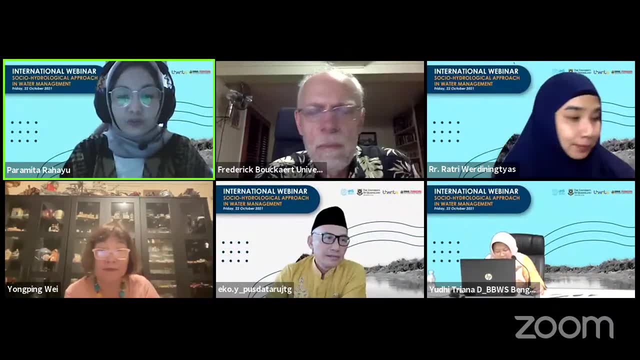 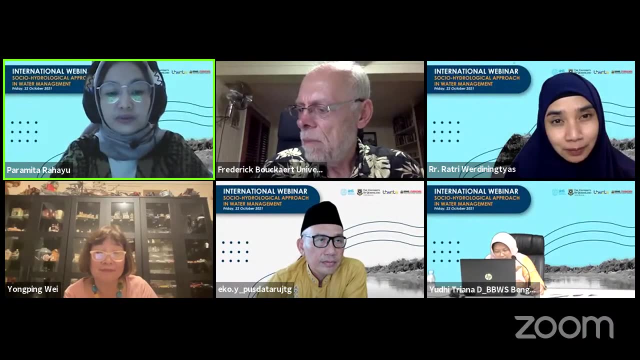 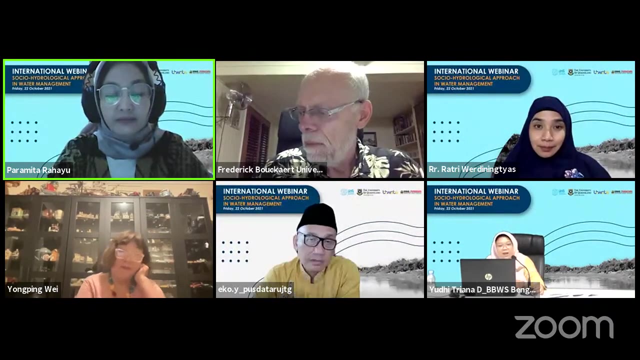 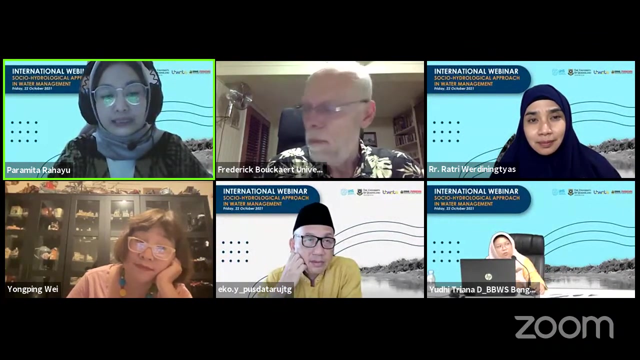 authorities in the uh general, uh uh government. i think this is this one. okay, thank you, paiko, and for buratri uh. there are many water related problems in indonesia, such as floods, growth, lack of adequate water storage and so on, and they cause stress to water availability and sustainability and cause problems to water quality. 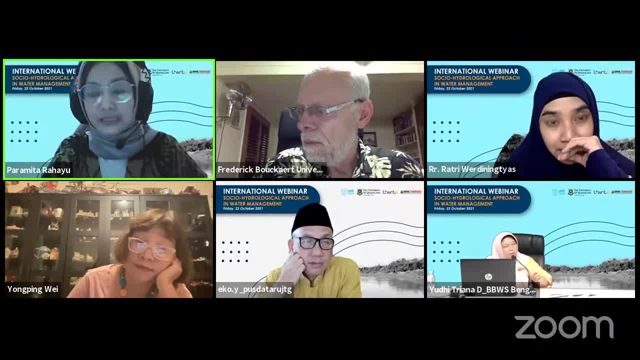 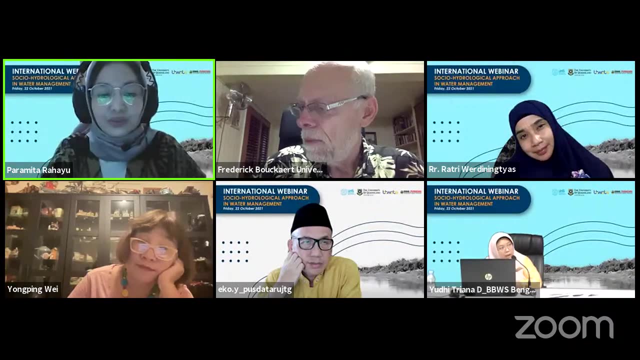 and those problems are mainly caused by human activities. the question is how to manage the issues of water problems caused by human themselves. what kind of policies or punishments can make individuals not pollute rivers or build houses on riverbanks, and how to take effective steps to invite all levels of society to manage water to be more efficient? because of the 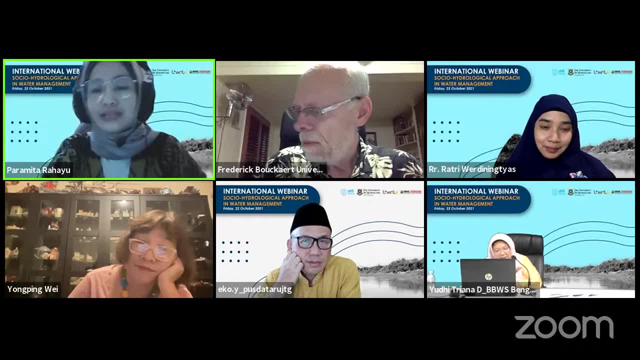 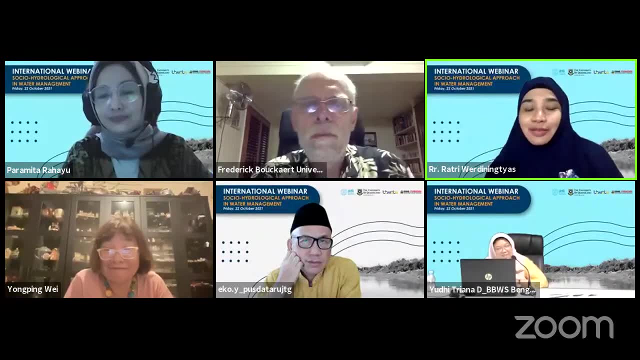 clean water has started to become scars of climate change. yeah, felice buratri, okay, uh, as uh, what i learned from victoria, i just shortcut uh from island victoria for the first. uh, they didn't integrate so like in the first regime, actually, when they manage the water. 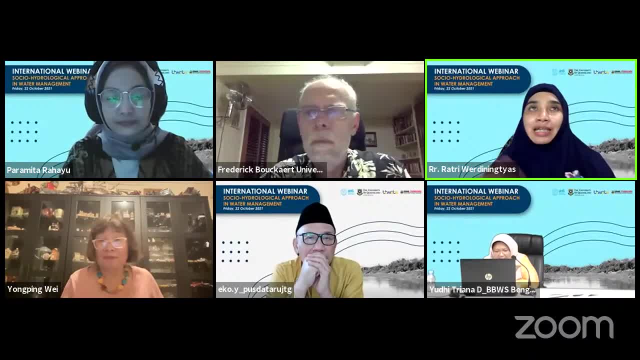 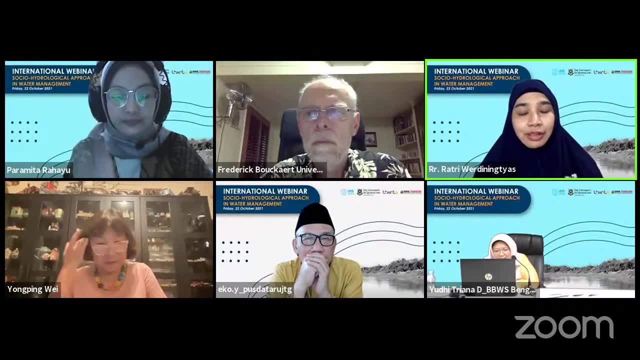 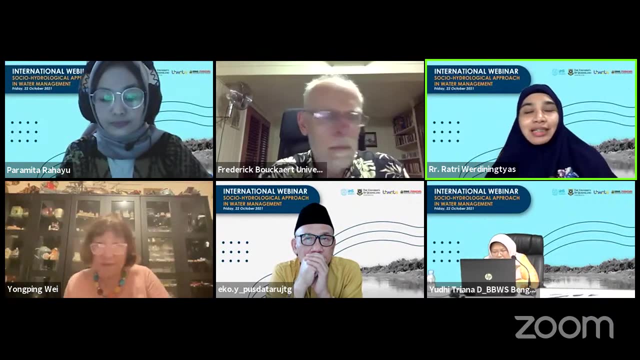 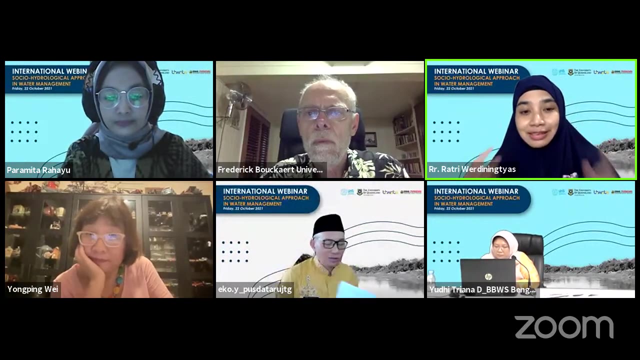 the consideration is also the water accessibility license or every rule uh is granted actually, or it will be granted if the there is a water availability. and the second one is like maybe a little bit from like our government line, our government now like uh, the government concern is become a drive, drive the policy instrument, for example. 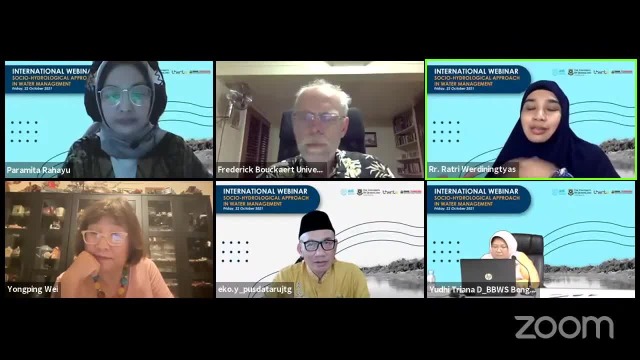 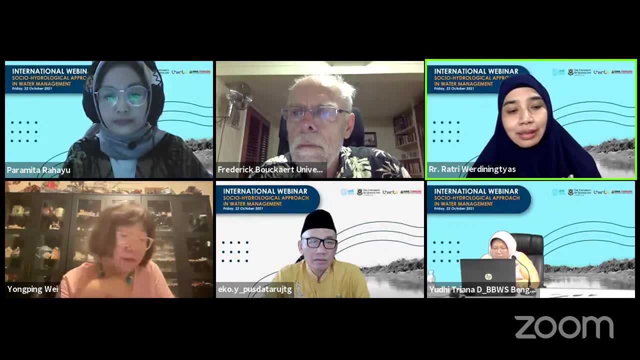 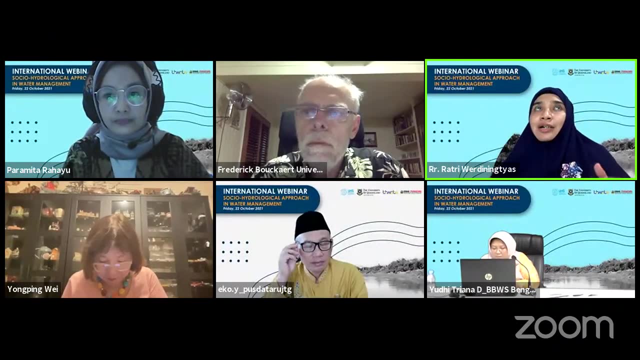 like what government wants, so the policy instrument or the intervention is directed to support the government concern, something like that. but the good, the best thing at the third region actually is also trying. we are trying is actually: uh, we need to base our decision make, decision making based on our understanding about the biophysical system. so, for example, we 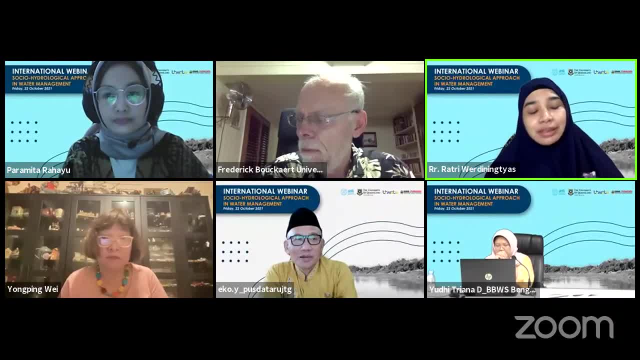 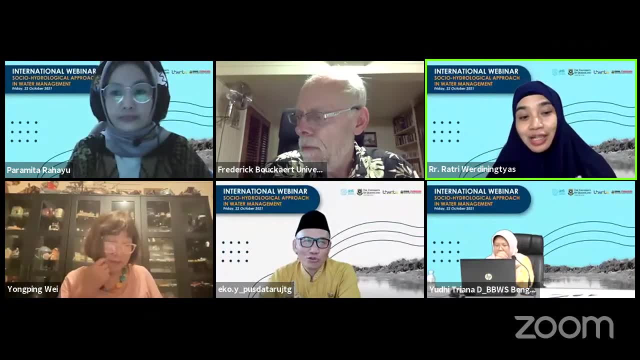 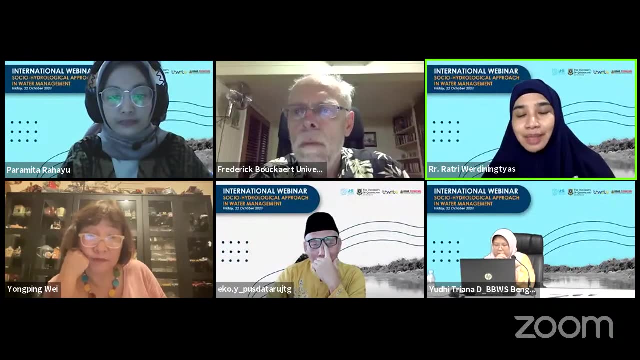 cannot just give a client without understanding how much water actually we have. even we do say we don't have that, that integrated data. so we, how we know that uh, our, our, our intervention, or when we give a grant or a license, it will not uh harm the, uh, the environment. 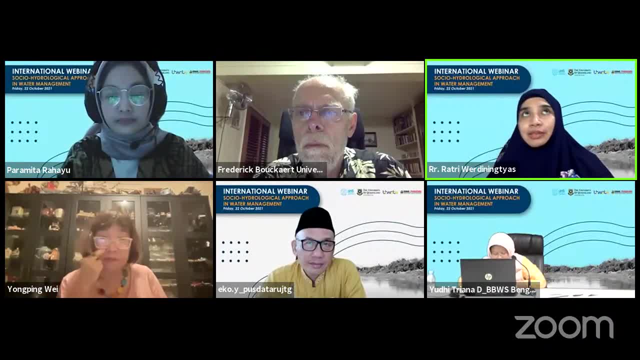 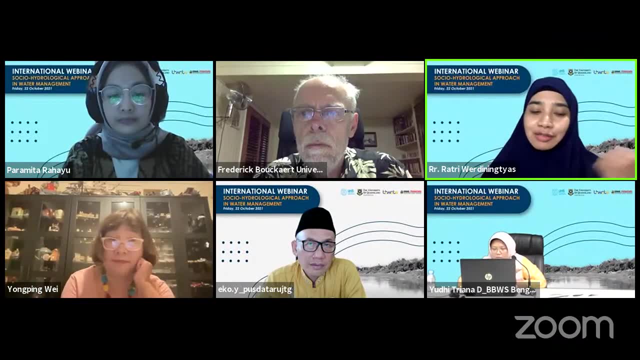 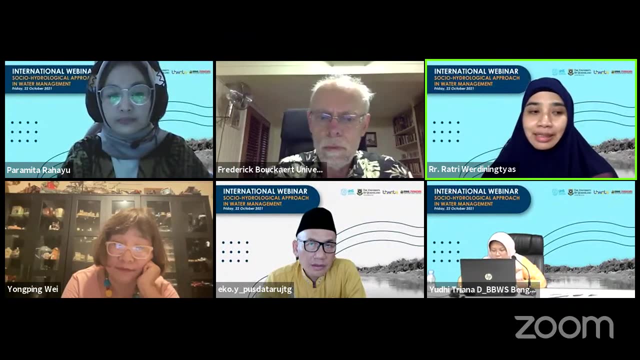 something like that and let's just form the factorial regime, exterior regime. actually they try to coordinate all the action. all the action here. uh, like you say, there is water pollution, uh problem with the flood drop and every, and in indonesia also there are many government agency like try to cope with, uh try to put with, that incremental problem, but actually they are not. 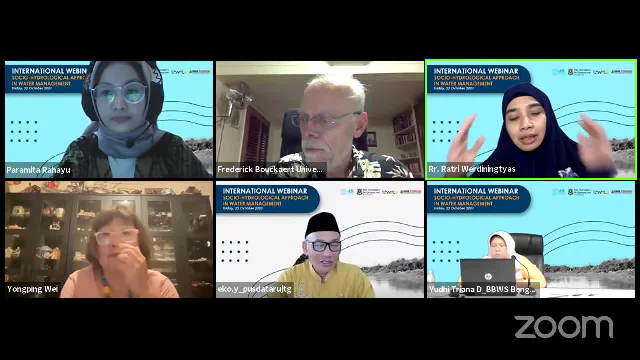 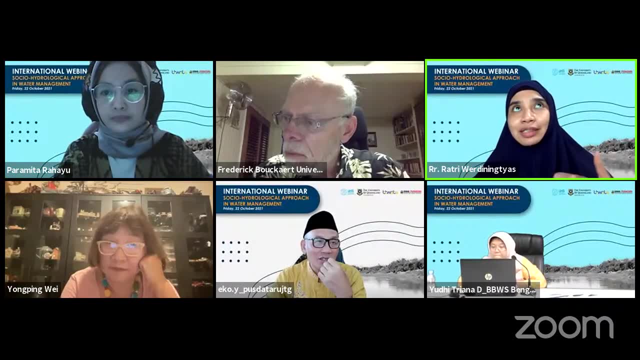 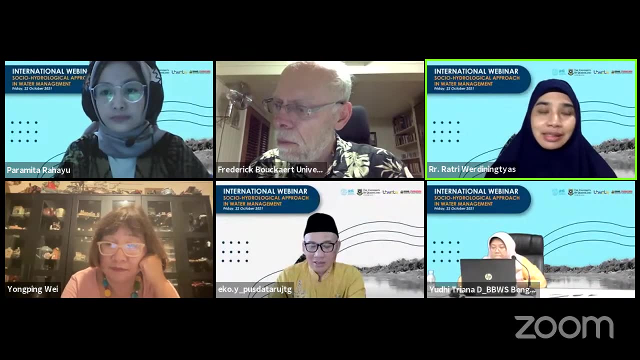 incremental. like i said before, they are interconnected but sometimes the government see they are incremental so they don't try to interconnect uh their decision maker decision making and not supported by integrated uh data, so that's make the decision. is uh incremental, then it make uh like in the third. 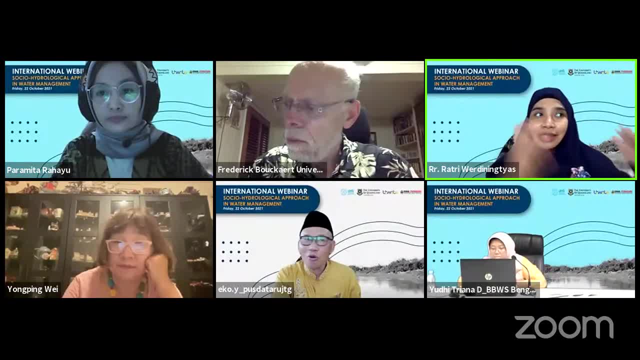 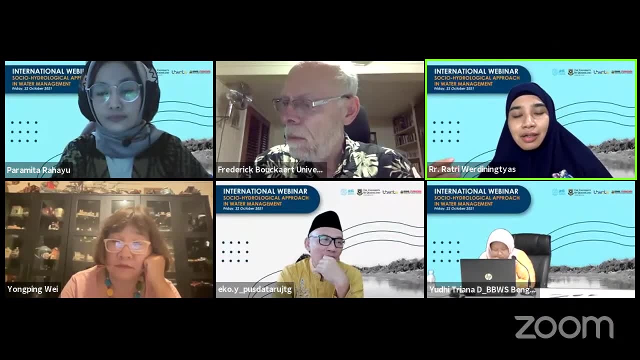 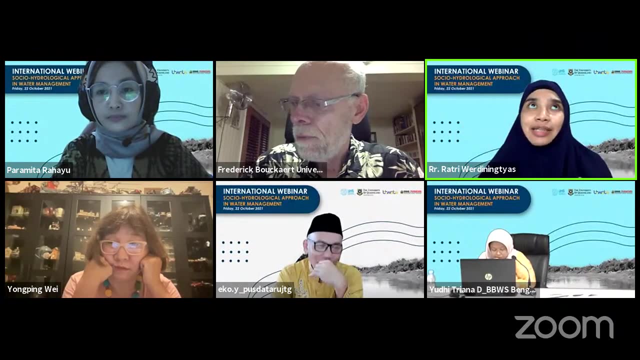 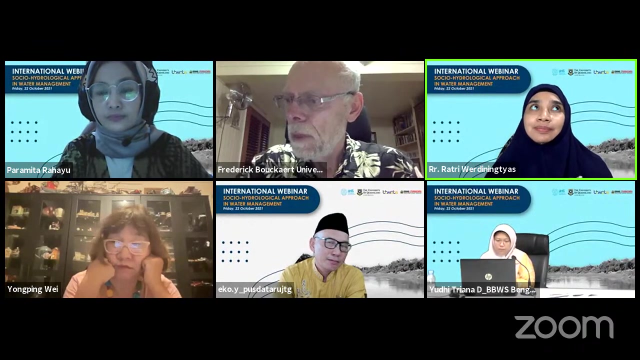 uh regime of the victoria. like, yeah, they're based on their biophysical condition, but they are still inconsistent between authority. uh of uh among authority, because they have different perspective, they have different interests. uh, they have different background. for example, like uh, now in indonesia there are many. uh. what is that mushroom about groundwater exploitation? 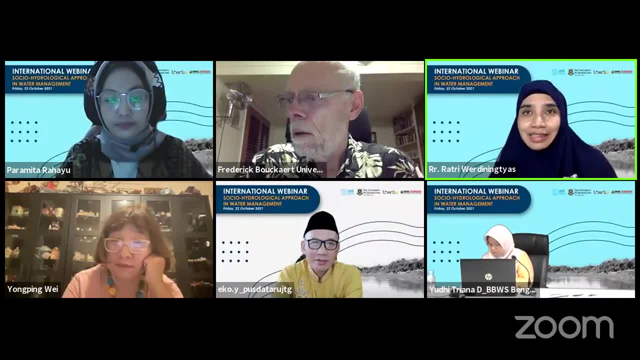 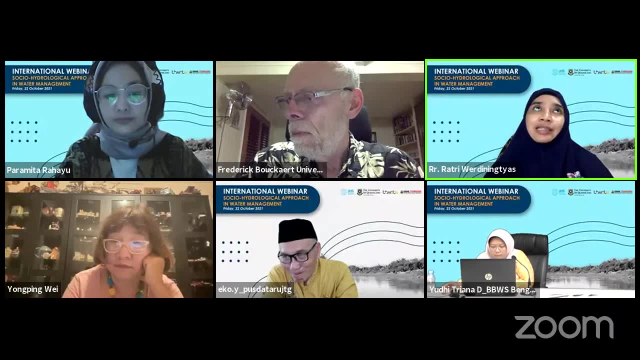 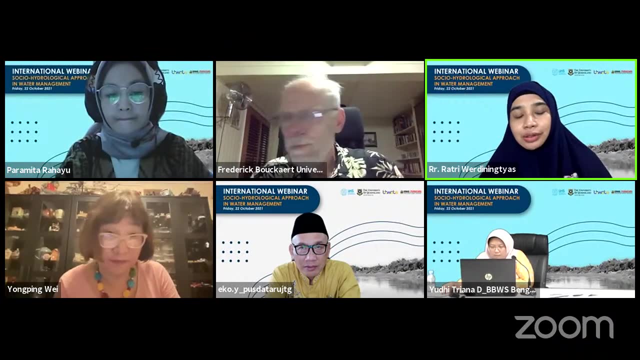 and actually the for environmental agency. they said no, it harmed the environmental. but if the- i'm sorry to say that agriculture i can see say that i need to. uh like i have target about homemade spaghetti i need to produce, so i will give a help for the farmer to build the groundwater or 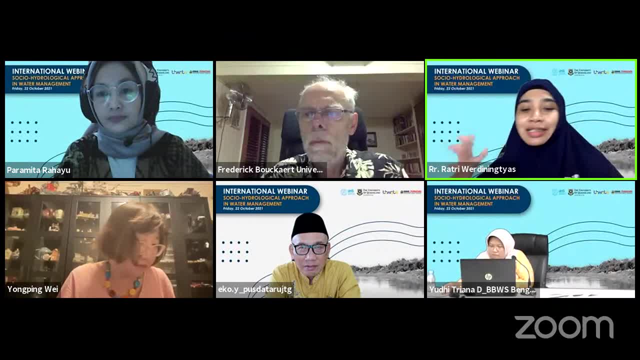 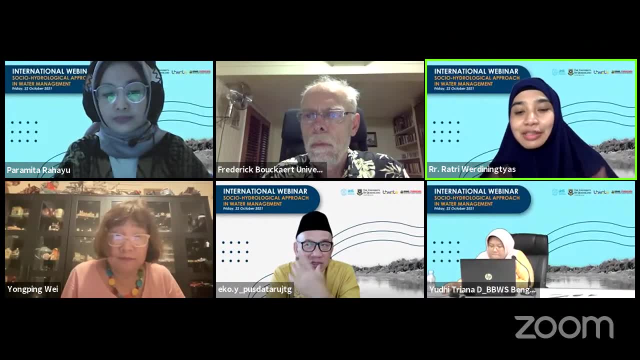 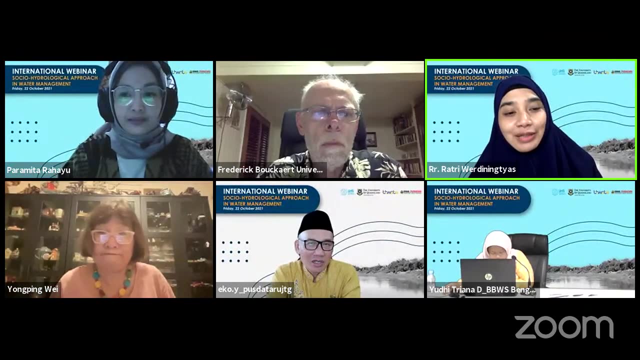 uh, try to dig a wheel, for example. so there is in in synchronized uh decision because, uh, there is no one decision making process and we don't have actually integrated data. that's maybe my answer. hopefully it's answered the question. i don't know who's the end. 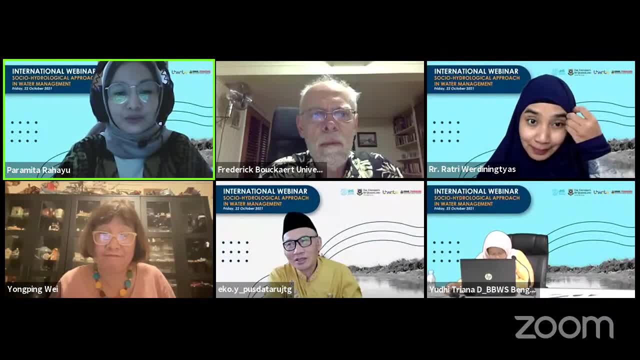 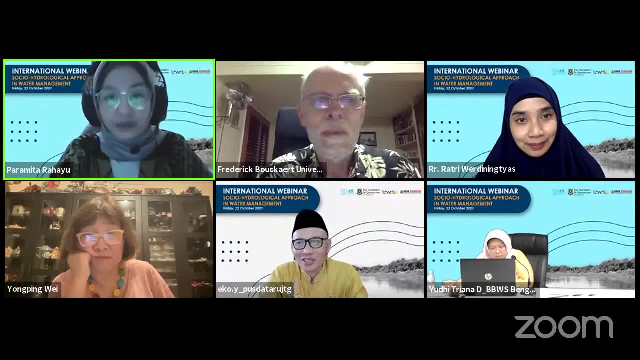 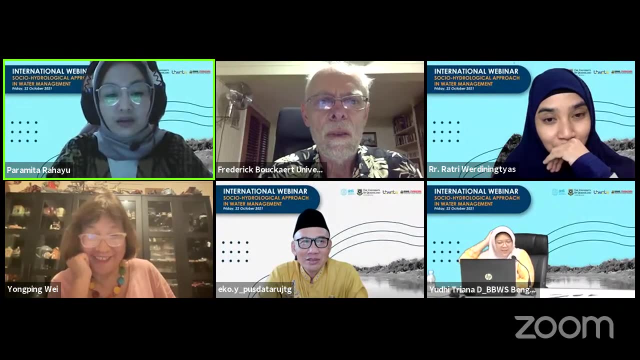 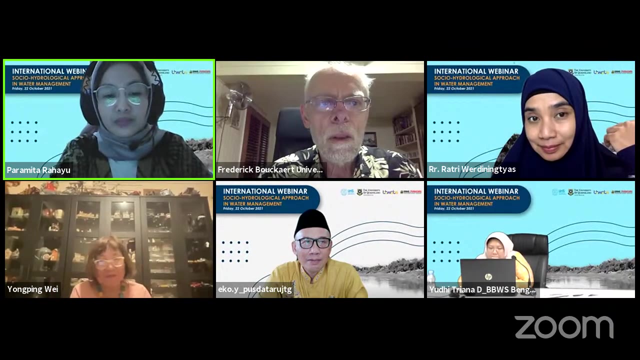 thank you very much, muratri. and we back to uh to dr boker. uh, another question for you is that: is your framework uh applicable to every places or river basins, because, or is it for certain types of rivers only, or because in indonesia there are some types of? 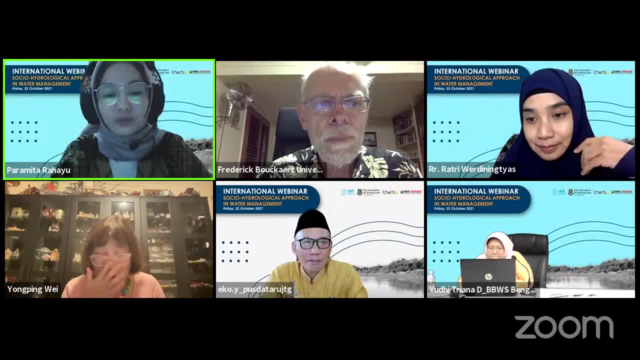 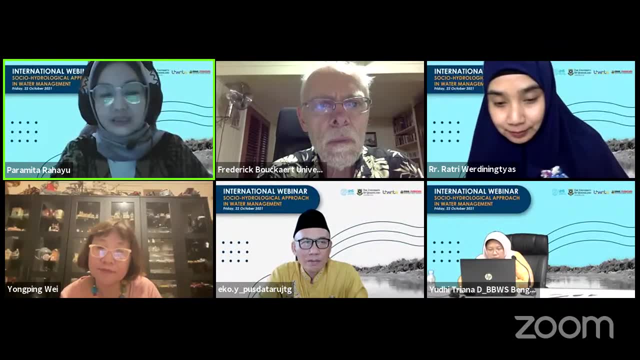 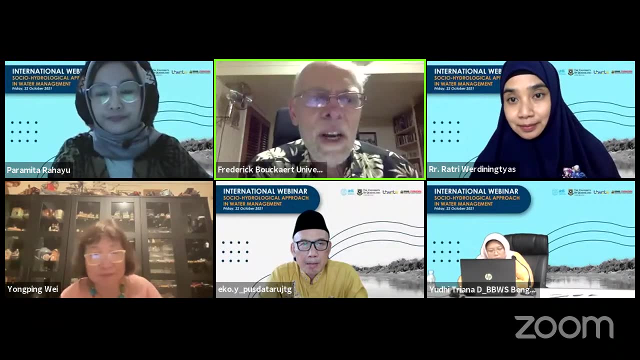 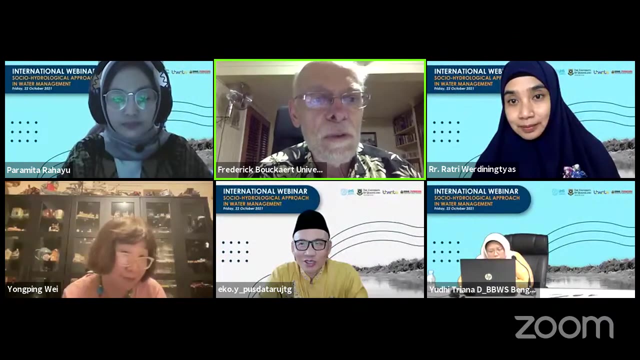 rivers? uh, some rivers have multi-functions, not only for water flow or source water sources, but also for tourism, social, economic and agriculture. is it applicable to every types of river basin? yes, thank you for that question, um i i deliberately designed the framework to be applicable across many different types of river basins. that's also allowed me to do the comparison between. 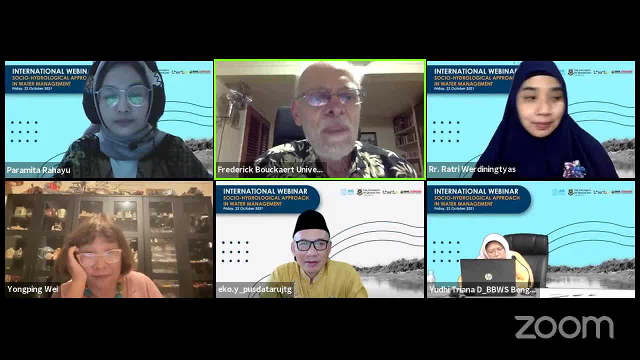 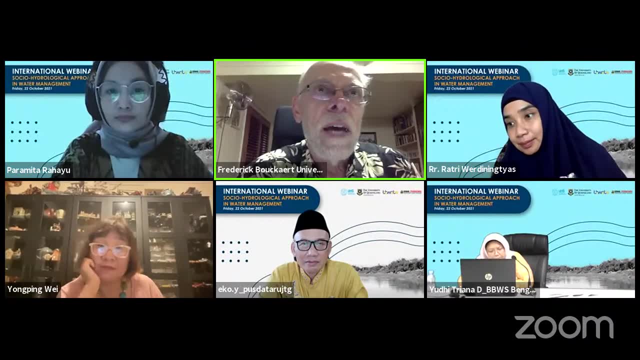 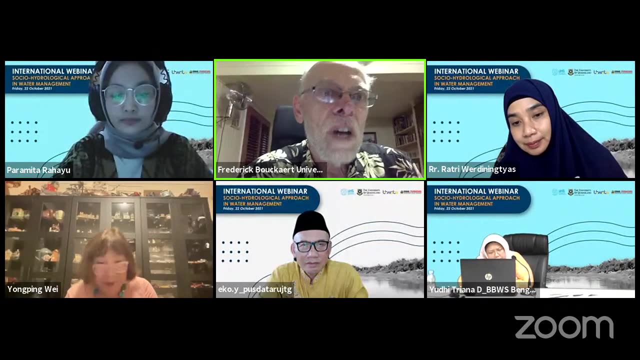 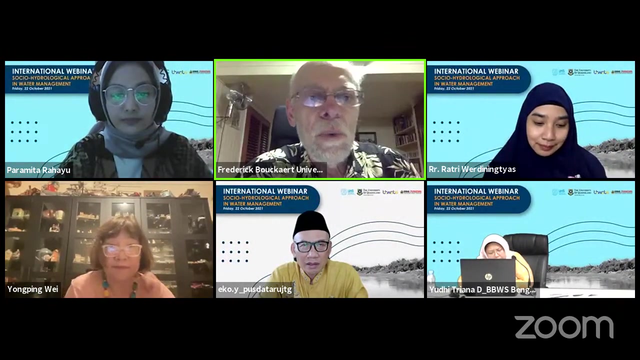 river basins in four different continents and in different situations. it is definitely applicable also in indonesia. the eight indicators of my framework basically allow you to um assign different attributes for each indicator. so if, for example, there is uh water flows or river flows, you can under under that indicator, you can put in um uses of tourism. you 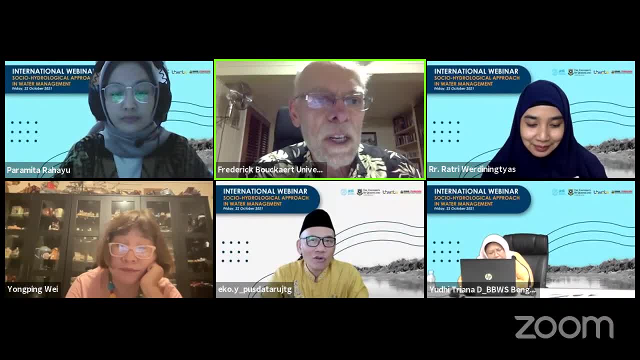 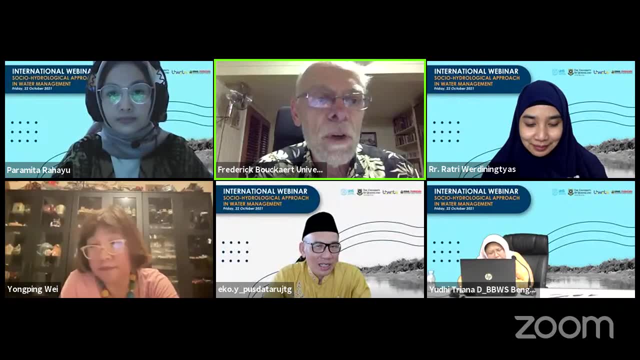 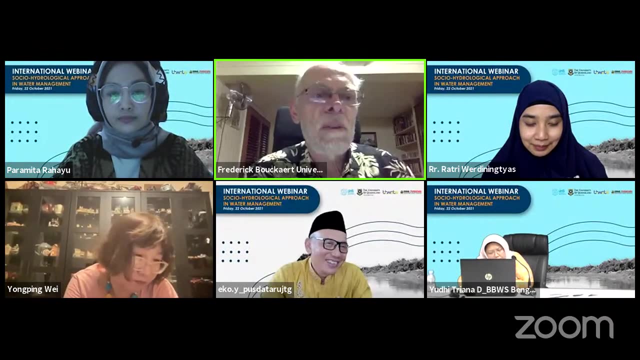 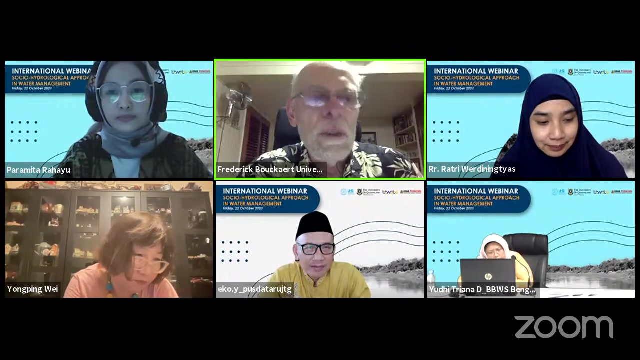 can put in uses of hydropower all sorts of different things that are relevant and applicable to that river basin, and so the river base, the framework, can be designed to actually assess the river basin, with its typical characteristics, its river flows and its conditions um and and its um social institutional capacity conditions as well. so, yes, the answer is it. 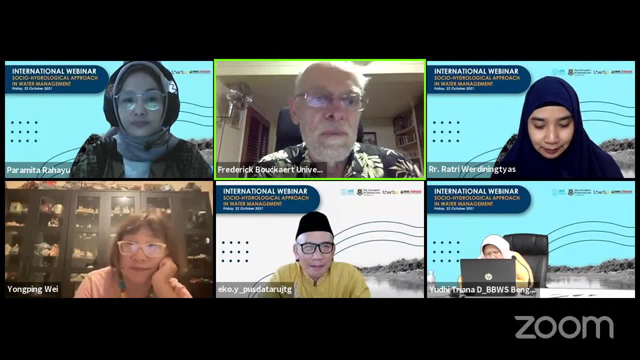 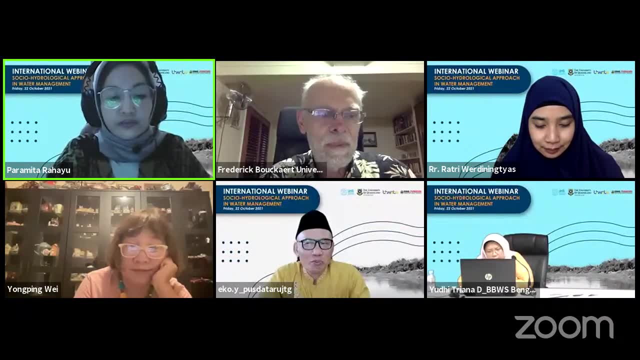 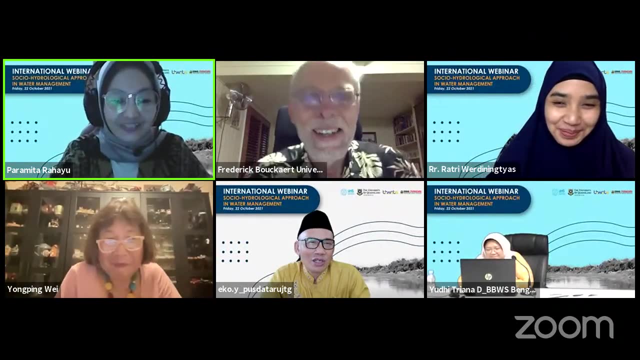 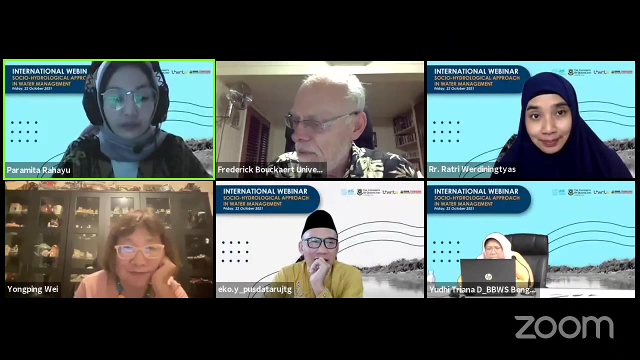 can be used um for any river basin. thank you, dr booker. is applicable to any river basin. yeah, another question, more question for professor yong ping wei. yes, in the research about the resilience of socio-hydrological system in chitarum river basin is in west java province, indonesia, conducted by our institutions. 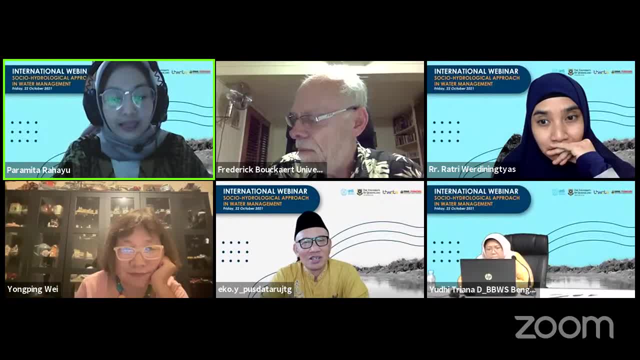 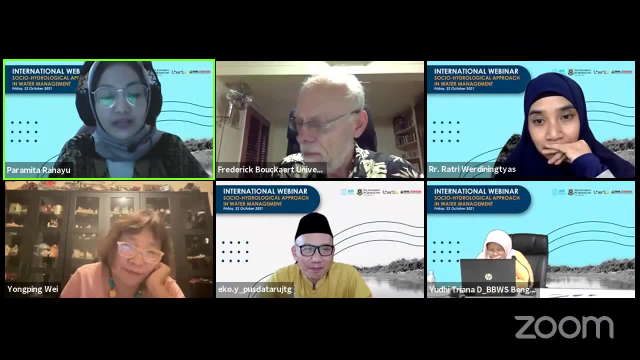 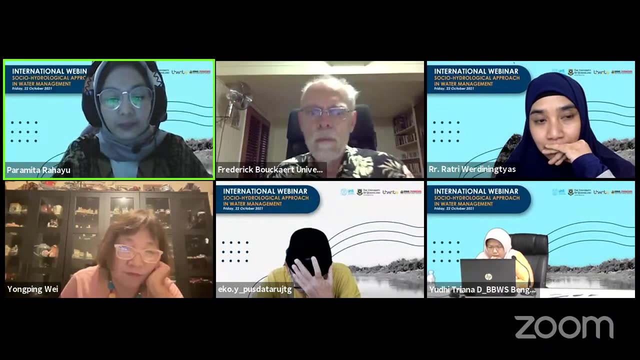 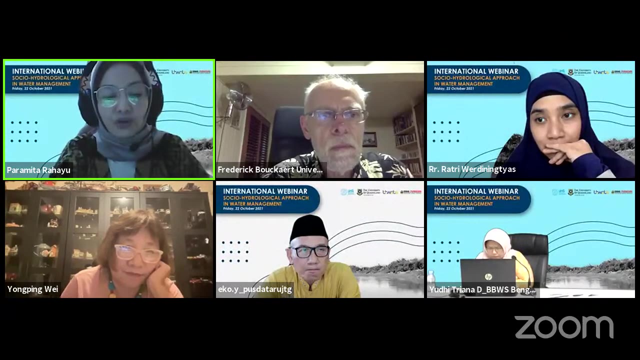 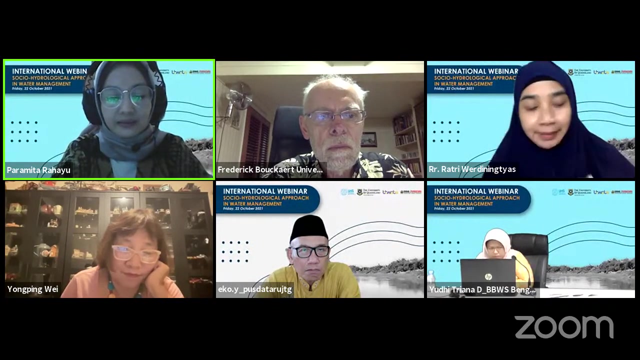 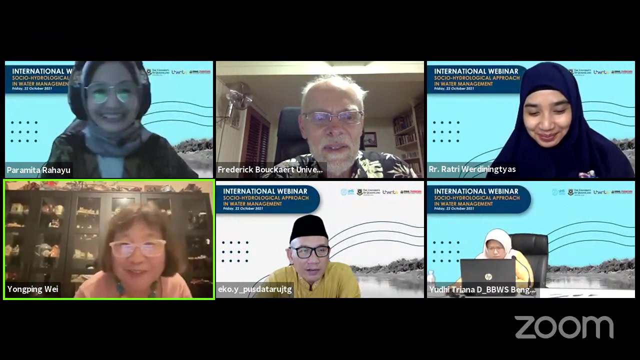 we used social capital in at the society level, value, beliefs, norms and pro-environmental behavior at individual level to measure the human resources adaptive capacity index. do you have any opinion regarding the use of this method, society level and individual level? that's my expertise. feel excited anyway. so so, uh, because a social capital, you know opinion. 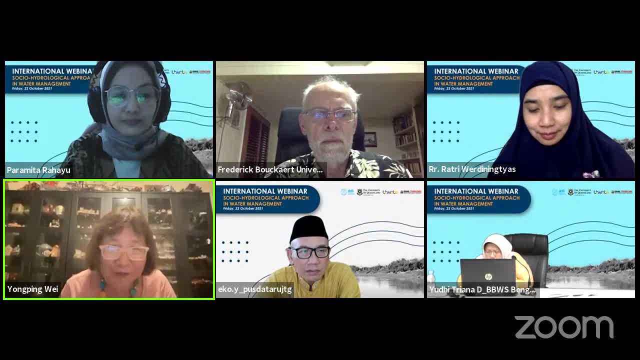 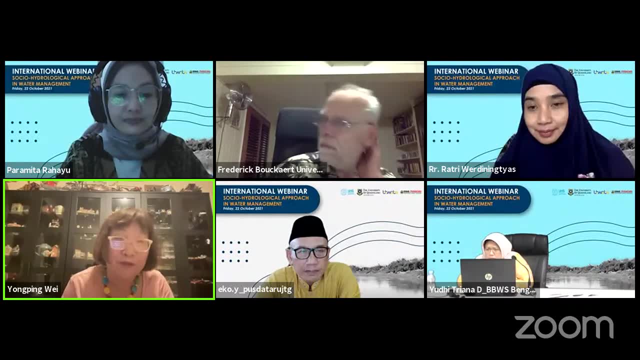 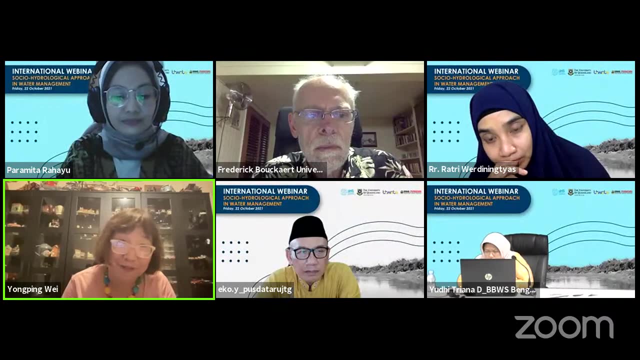 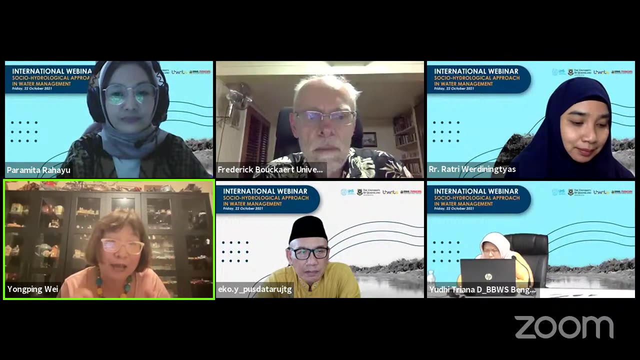 opinion value. that's a social capital. so certainly that has to be quantified, otherwise you never can measure resilience of your social ecological system. the first and second statement is: if you want to quantify the social capital, have many ways. in society level you have some ways in the group level, group behavior, some of the ways, and individual level. 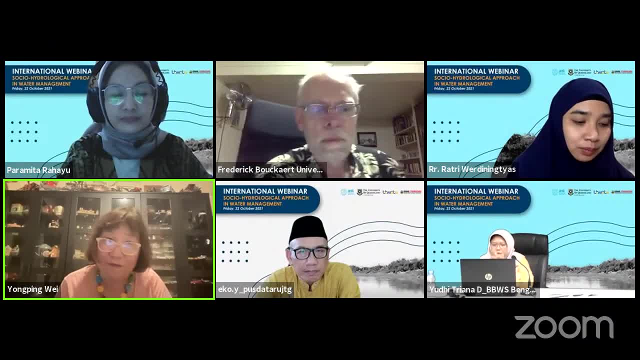 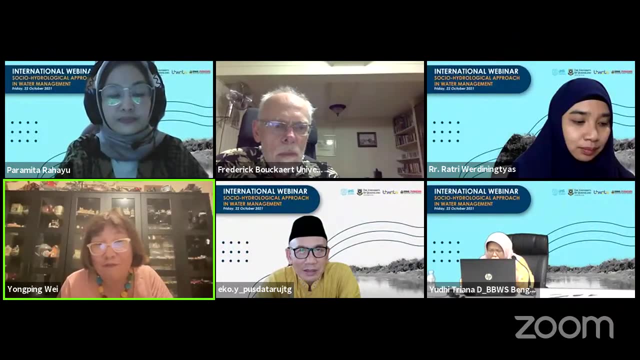 have some ways and in terms of different data source you have different ways. if you got something from your questionnaire, that's different method. if you're some from from media, you know newspaper as other ways. if you're something from the census, you put the census in the shopping market, you put the 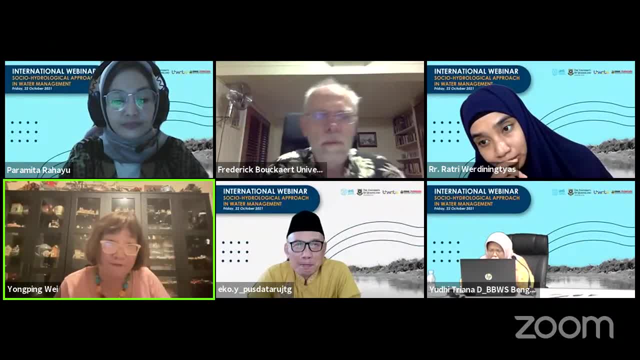 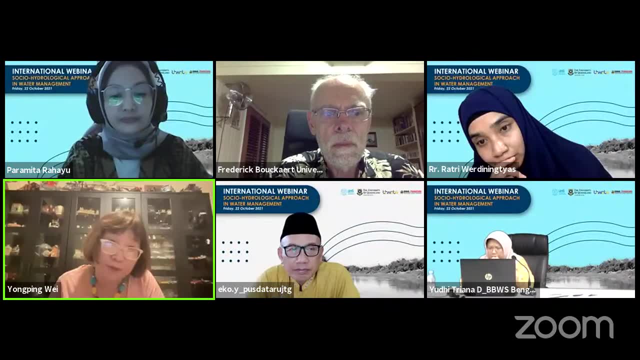 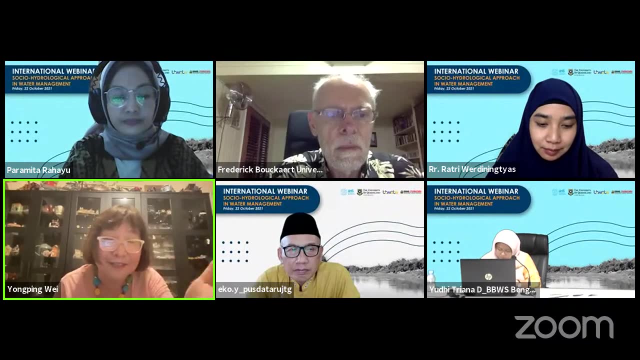 census. in some ways there's a different ways. so certainly we have different ways to quantify social capital and we have ways to integrate that to the water balance model- fantastic one of our guests, the lectures put the putting your catchment, the water balance model. there's fantastic we. 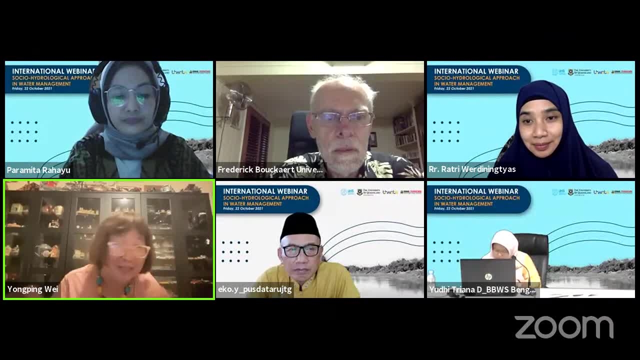 that's my daily work, so we have many ways to do that, but unfortunately, since there is part of the women's contraptionился in the open sea, as you can imagine, we have an Hateio model. there's two ways. fantastic for me and i will share with you later, because it is not just one way. the appropri updated the. process, but i will touch on here if i should bring a consumption of specific values to that brush in the totally two ways we put the phase relation. a lot of it is форс uqa's examples. they practice for the width overall ability diet. just wants to know that. you know what's all about. i was having some. 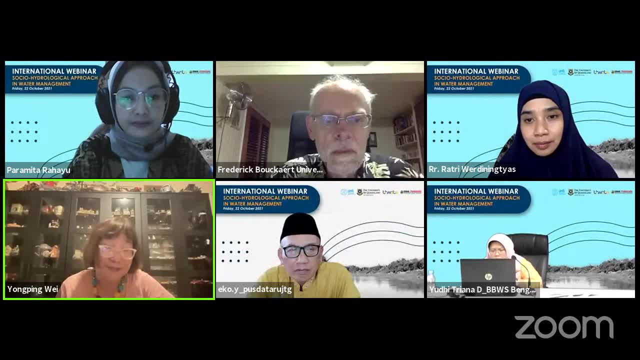 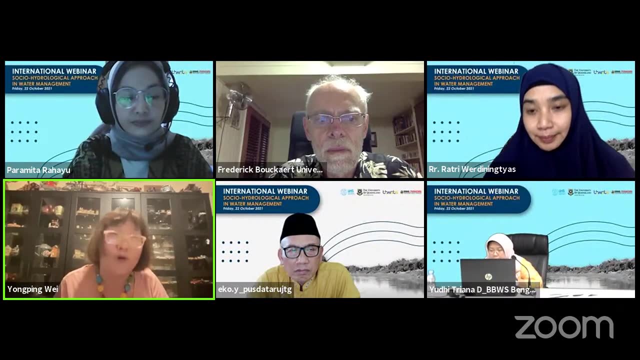 I can tell you details for different methods, different data sources and the different levels, but very happy and open to any questions and we will set up another room session. I can tell ways I do or I can send a reference our group already published to this question. 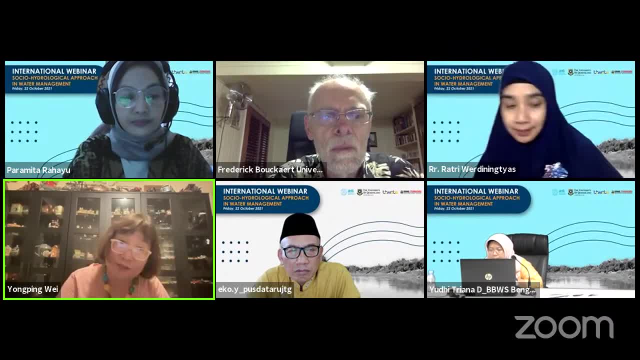 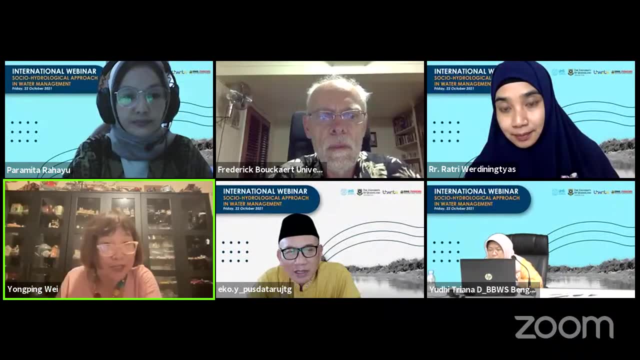 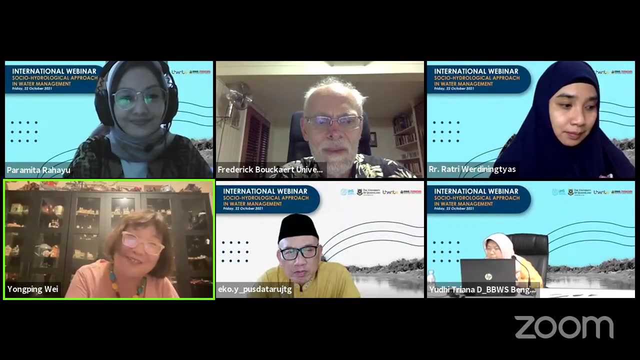 Certainly it depends on which is your data source and which level- society level, group level and individual level- and which kind of ways you do So. certainly answer is yes, but I couldn't tell you very detailed what I have done. 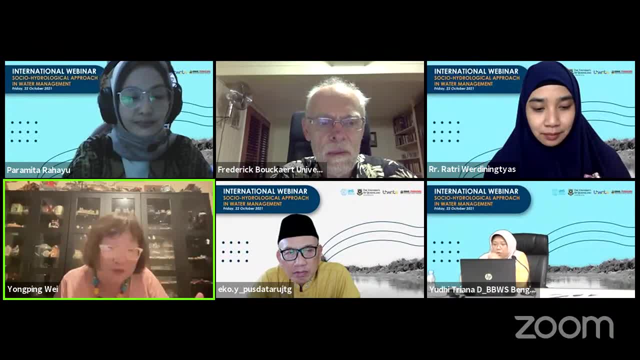 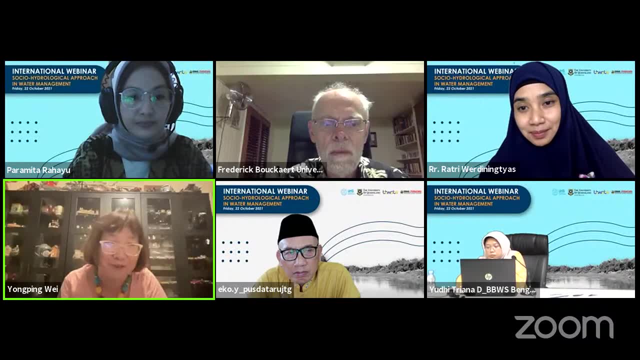 But I show you some examples that our group, our students, have done. One slide is one PhD student, four years work. So I just show what I showed you before. but we have many, many other ways to do. Certainly, I'm more than happy to share what we have done. 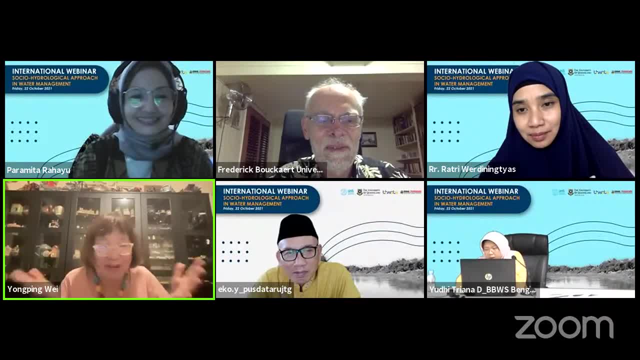 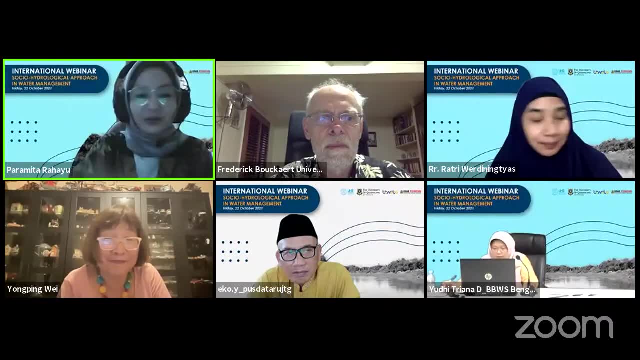 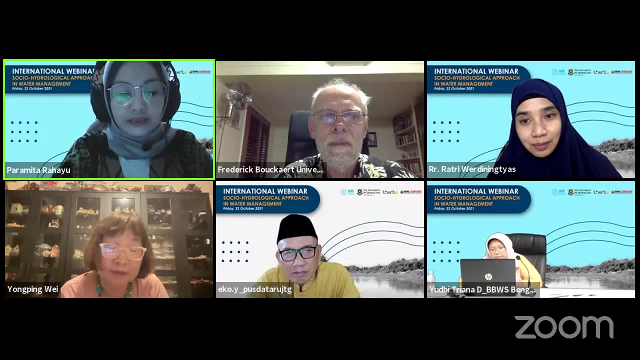 Sorry, I couldn't give you the one simple answer, but I can show, send you our publications. yeah, Thank you, Professor Yongping, And we have more questions for you and also Dr Buchardt. The question is from Bambang Widianto. 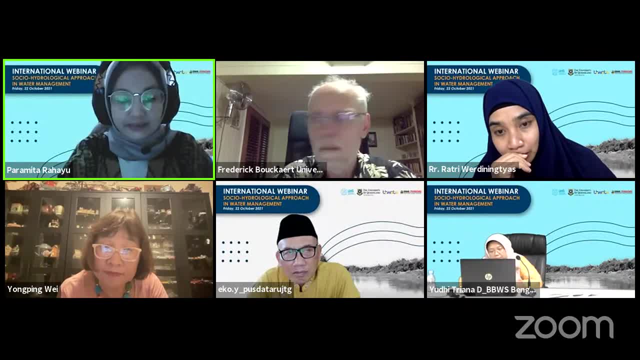 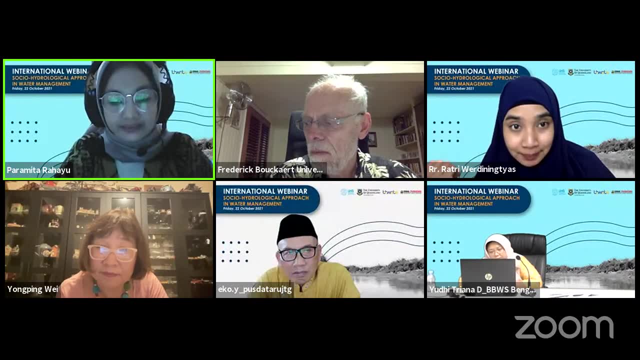 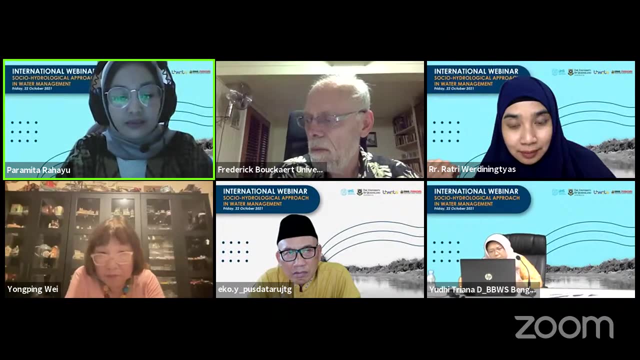 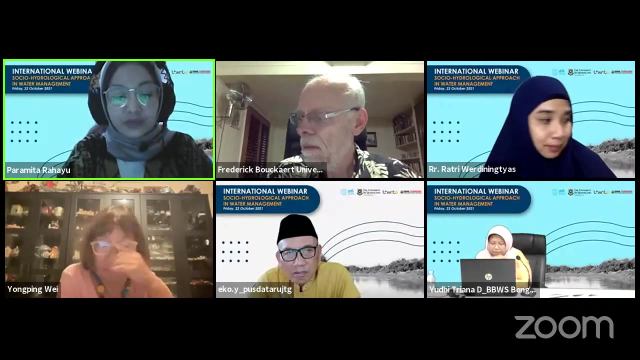 Could you tell us, or share the experiences, an example of collaboration between river management institutions and residences in a rural and urban area in Australia or other places? The river management office tends to be hierarchical, while some communities from the riverbanks are individual and some are egalitarian. 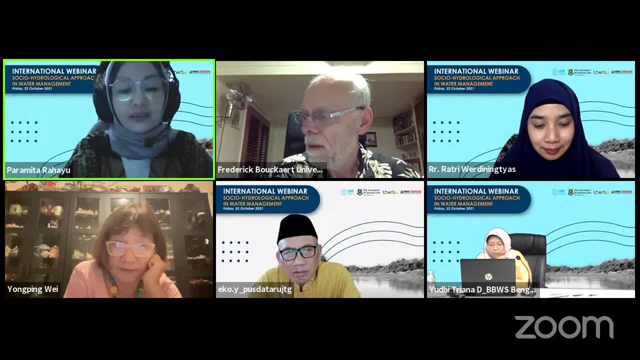 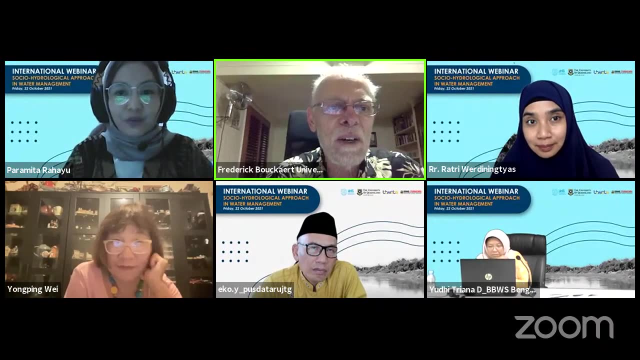 So how to build collaborations and what the example of your case. Thank you, Is this a question for both of us or is it for me? Yes, for both of you. All right, Yongping, do you want to start, or? 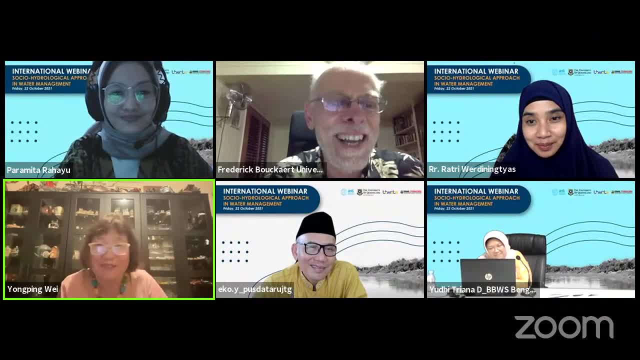 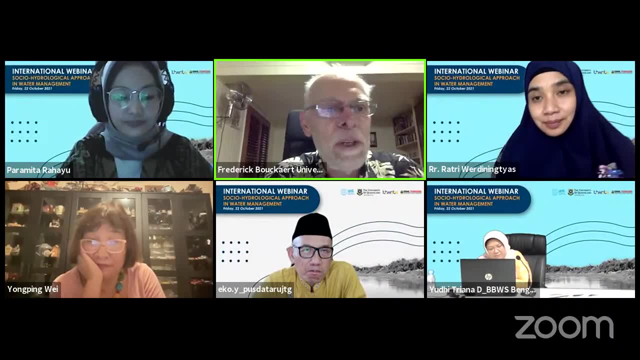 Yeah, you can start. I was thinking its not. Anyway, you start first, Please. Okay, I think I have to talk from my experience working in the Murray Darling Basin in Australia, because I have a long career in working with them. 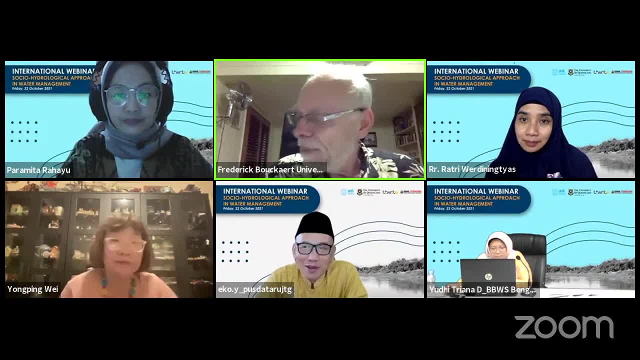 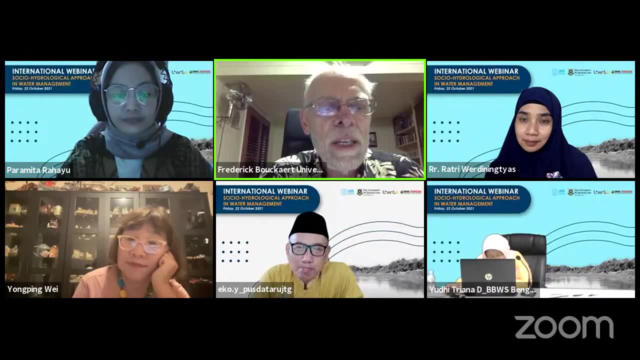 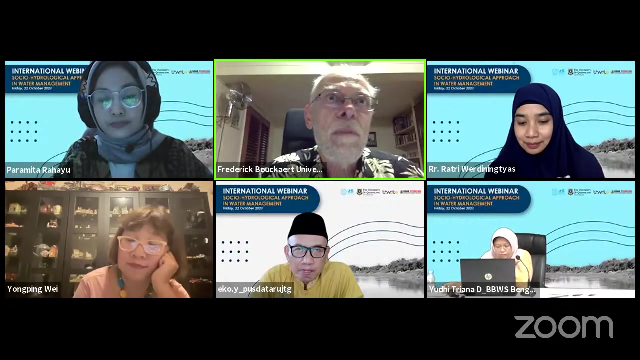 Before I I did my PhD. Basically, I think there has always been a bit of a tension between top-down and bottom-up collaboration between different organisations. In Australia we had a period where there was a lot of bottom-up information from catchment management authorities. They 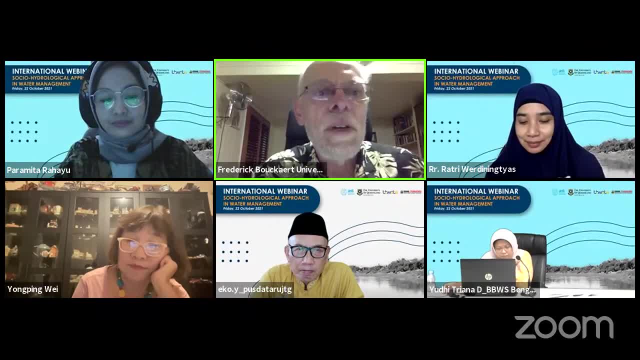 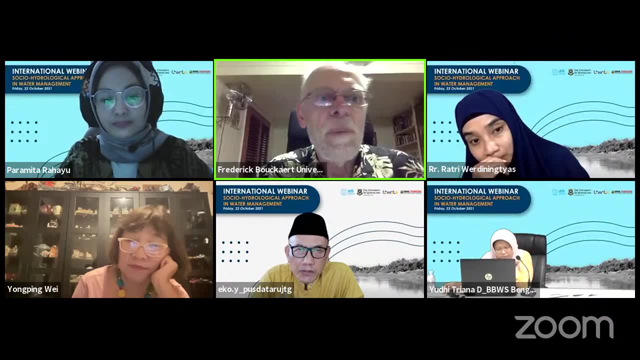 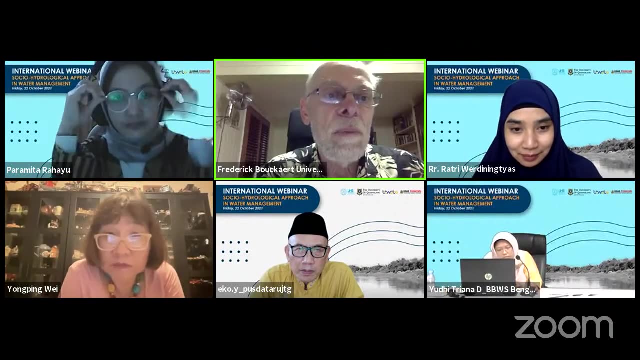 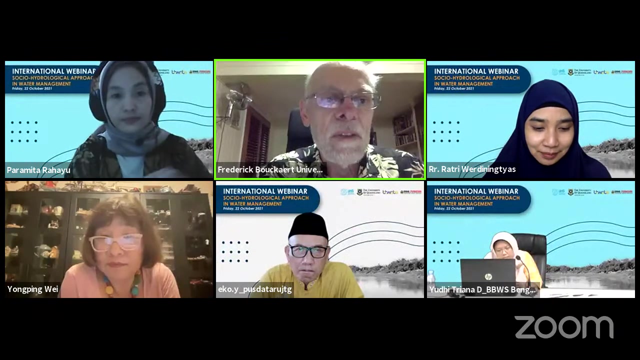 were basically at a very small-scale level, tackling the problems of localised people, of localised farmers, of small rural communities At that moment. they were basically looking at providing more sustainable collaboration for land and water management. It was funded by the federal government, not so much by the states. 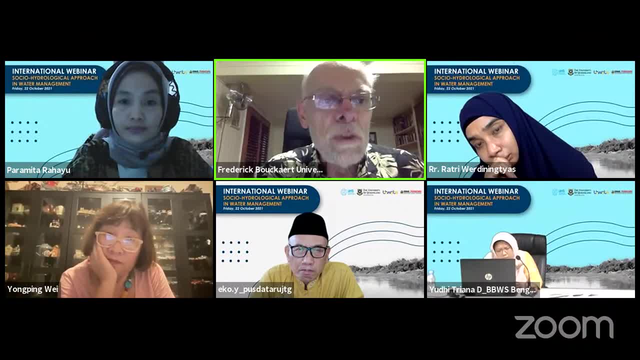 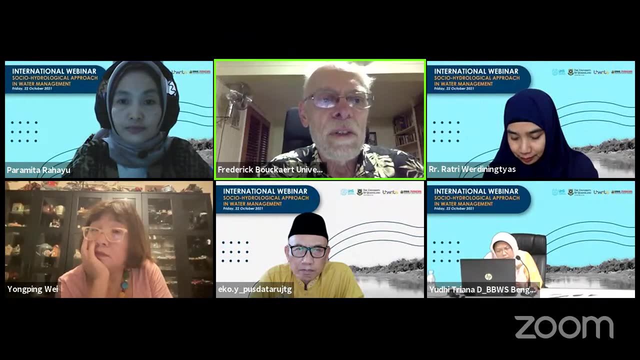 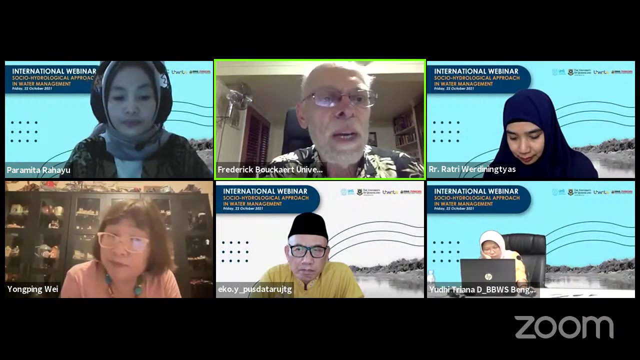 That worked quite well, but then the focus narrowed specifically onto water and not so much land management, sustainable land management. When the Basin Plan came into effect, these catchment management authorities were no longer consulted by the federal government, which is very unfortunate. When they did a top-down approach for the Basin Plan, they realised 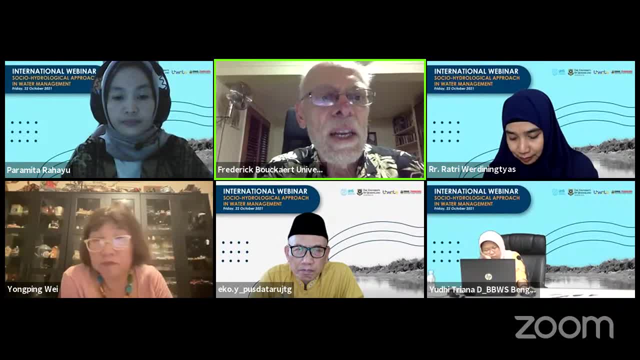 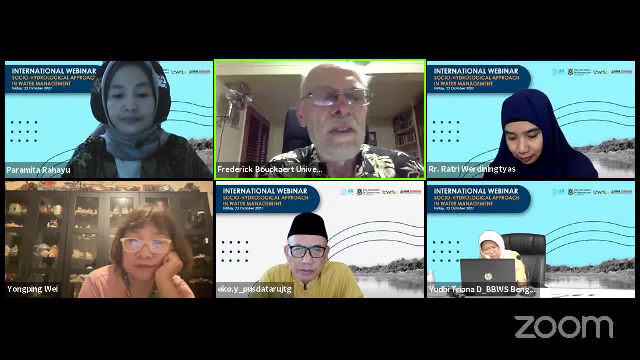 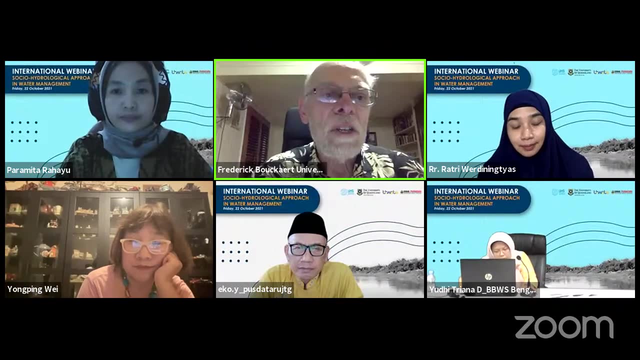 that you need collaboration from the localised people. You need collaboration from the localised community, an organisation that is watching over from the local levels as well. and some of the stakeholders were protesting against the Basin Plan, saying it didn't consult with us, it didn't take into account our needs, and so on. Then, suddenly, they had to start. 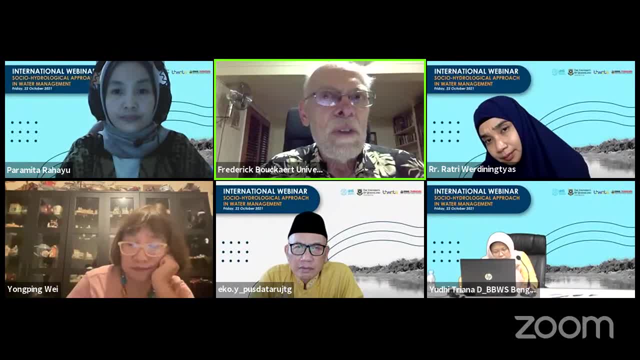 consulting a lot with stakeholders, They didn't go back to the catchment management authorities. They went to talk to the people who were protesting a lot and not necessarily the other ones. I think this relates to the performance of our alert bodies To the people: signs up there—who are saying: 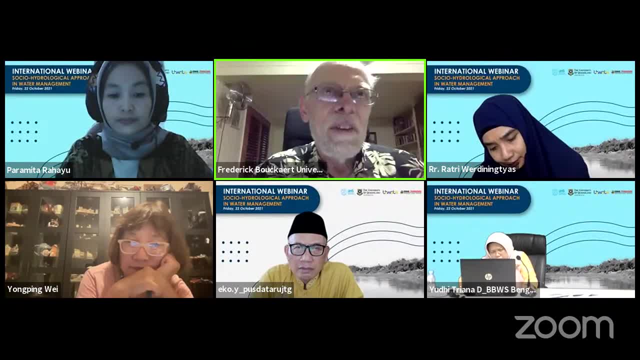 and not necessarily the other ones. So I think the planning and coordination of stakeholder engagement in the Murray-Darling Basin has been a little bit ad hoc and not very effective. always, especially since the basin plan has been implemented- They have been trying to be more systematic about it. 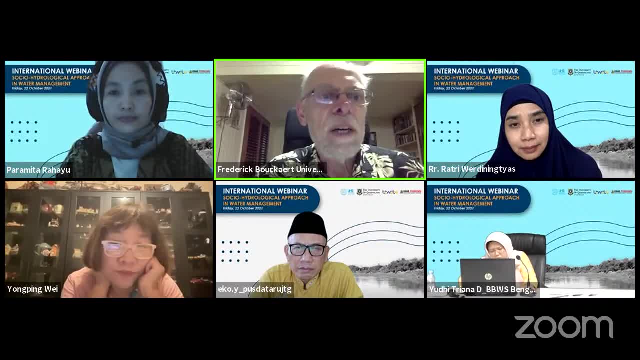 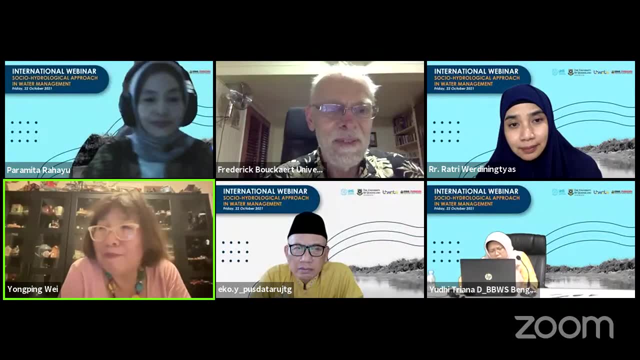 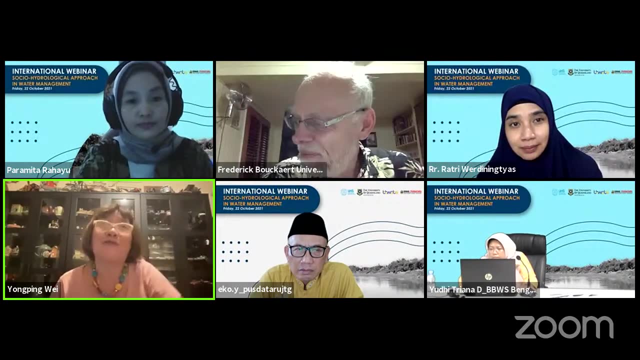 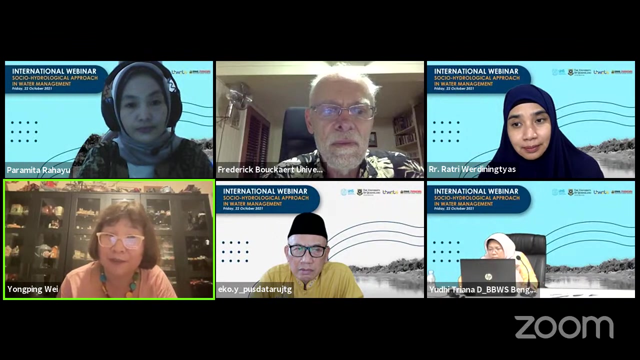 but I think they're still ignoring a large part of the local communities. Right So my experience and the perspective. now I don't have experience from the federal government to state government or catchment authority, So I'd like to share my experience at the river basin scale, the catchment scale. 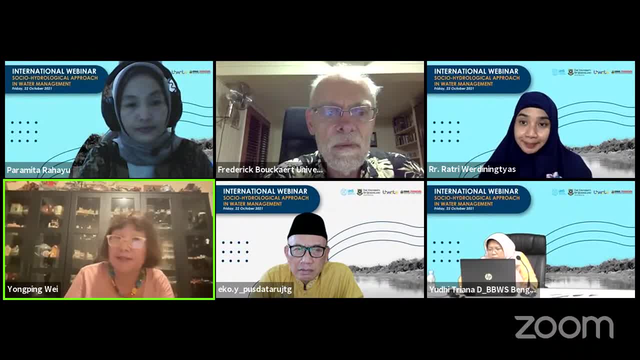 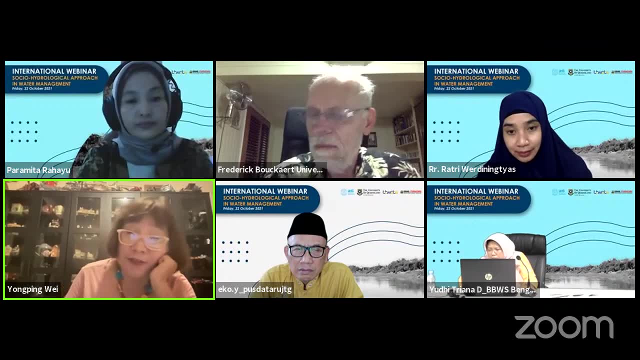 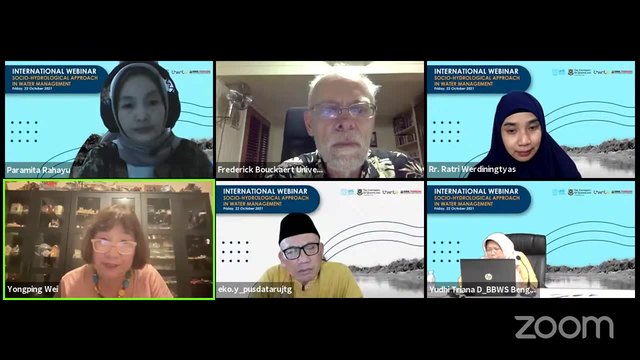 I think the most important for the collaboration between different stakeholders- upstream, middle, downstream- is I think it's a social learning process. Social learning or not just sharing process is very important from the planning, implementation, policy, implementation, monitoring, evaluation. 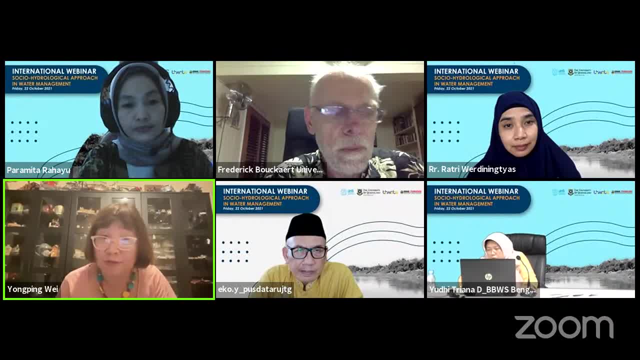 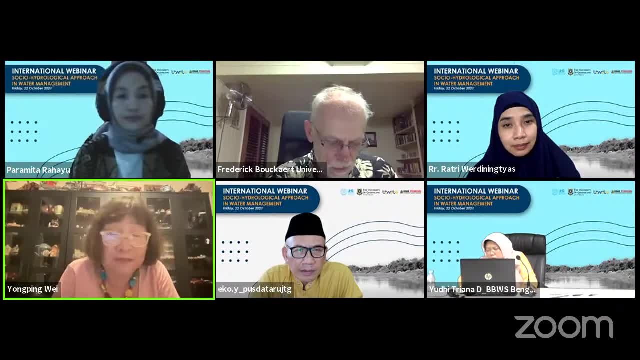 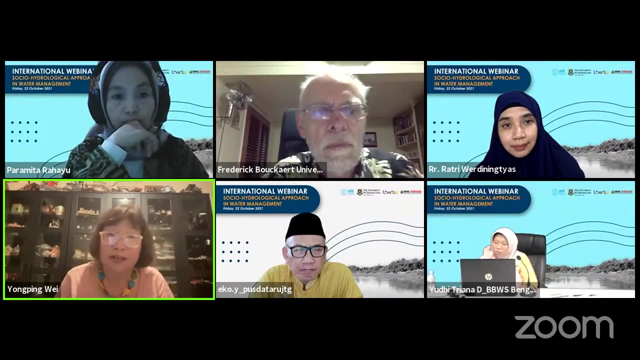 So the social learning process is really important. So one of the best examples in Australia we already done very good is the catchment Goldberg catchment authority- Sorry, The catchment authority. Later I can share you some experience they have done Is they use social learning as a tool. 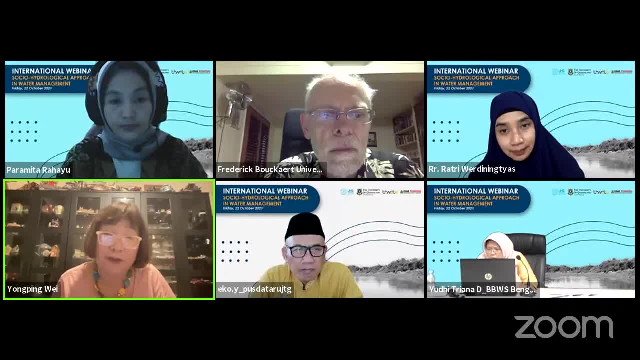 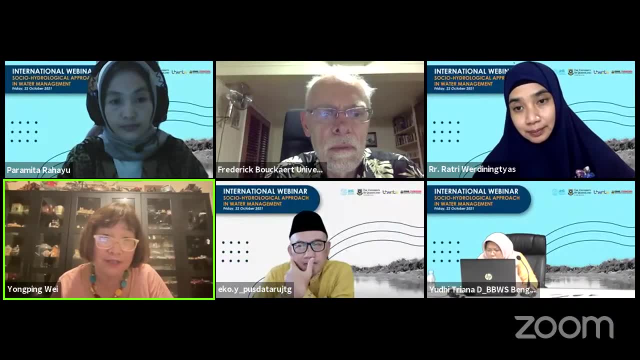 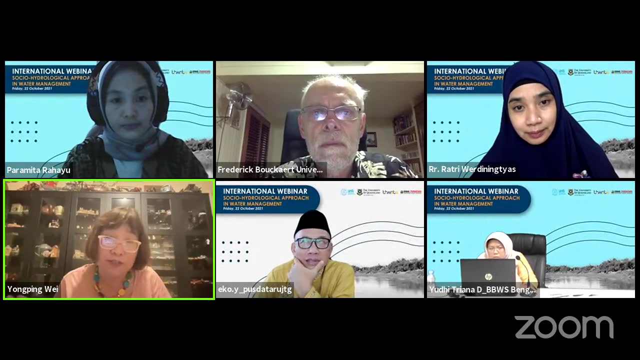 from the beginning of the planning onto evaluation, the whole the planning, all the practice. So social learning is a very important tool for catchment authority to use to engage all state holders in different step of the what we call like consultation of the water resource management. 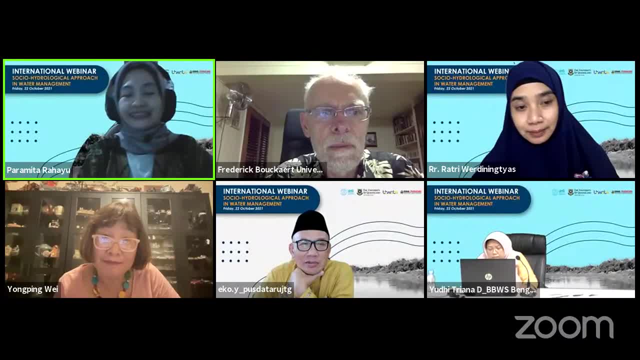 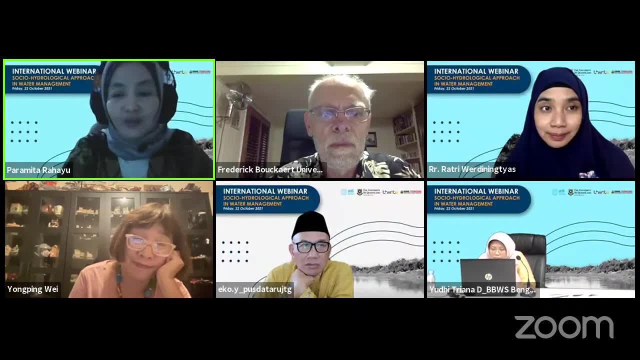 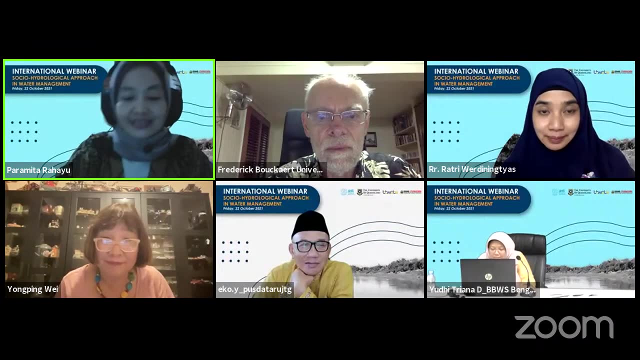 Okay, Thank you, Professor Yampi, And that is the last question for our Q&A session And I would like to thank all the distinguished speakers for all the presentations and all the answers and the discussions, And I think I will close this session. 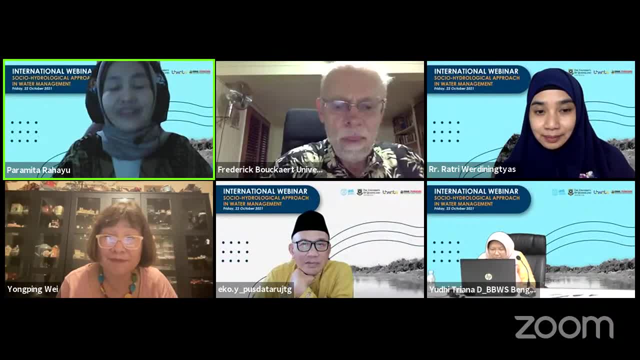 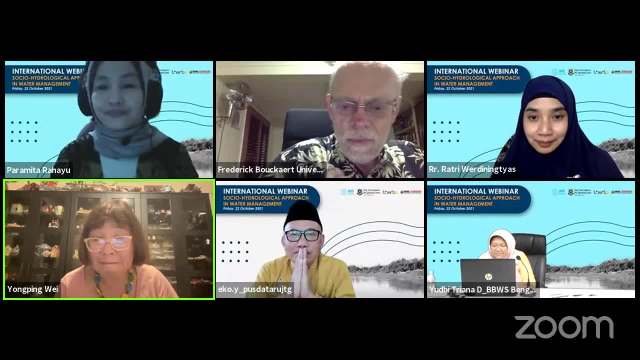 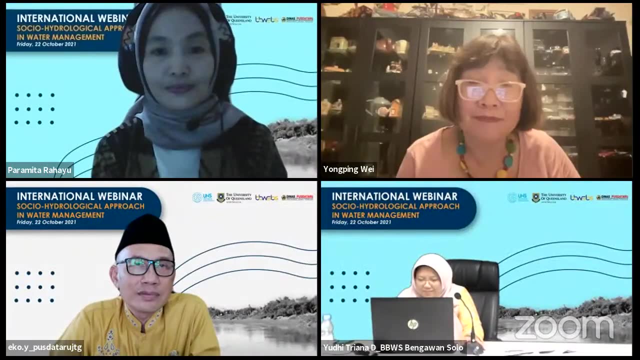 and back to moderator Bu Lintang Subinat. Thank you very much for all of you. Thank you, Yeah. thank you very much, Dr Paramita, for moderating this session very well. That was such a fruitful discussion. 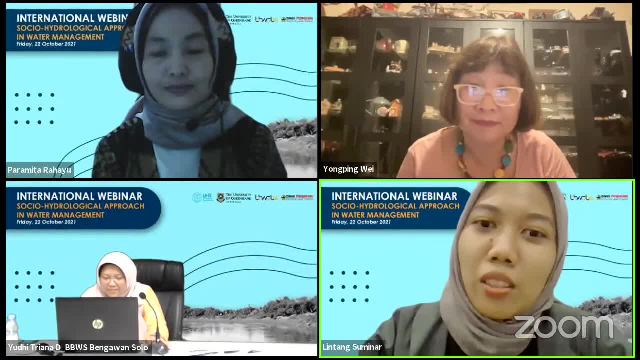 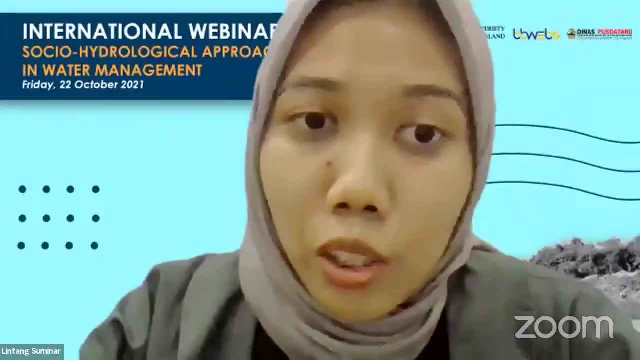 And I also would like to thank all the speakers here for delivering the materials of the presentations that are very insightful for all the participants And thank you. Thank you for the participants who already submitted the questions. We apologize that we cannot accommodate all the questions here. 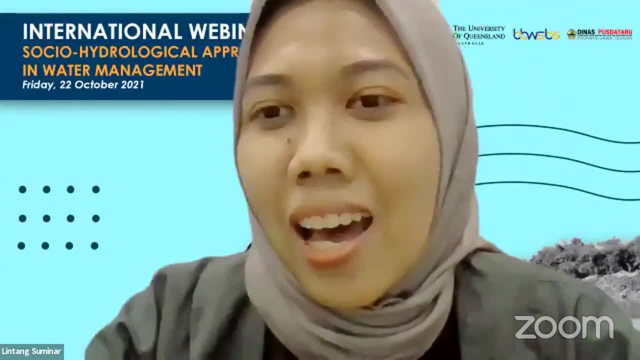 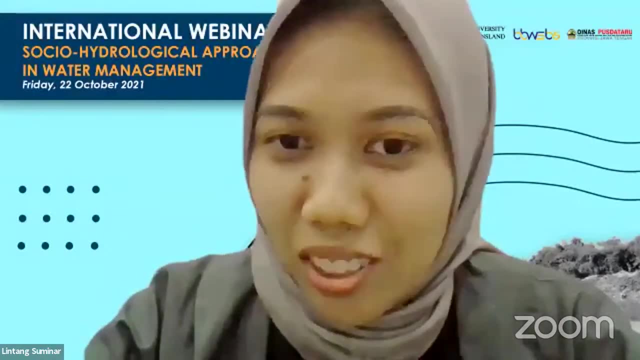 but we try our best to send the response to you by email as soon as possible. So before we work up to this event, let's do the photo session first. So all the participants, please kindly turn your camera on. Thank you, Thank you. 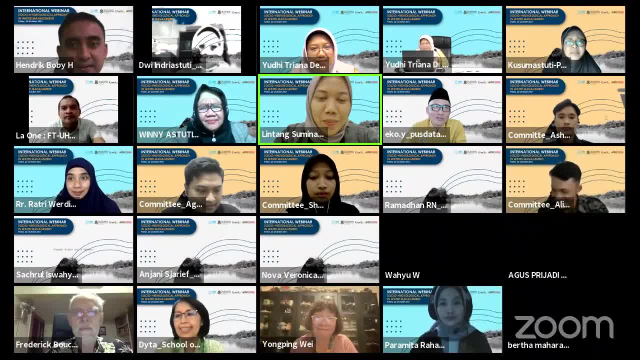 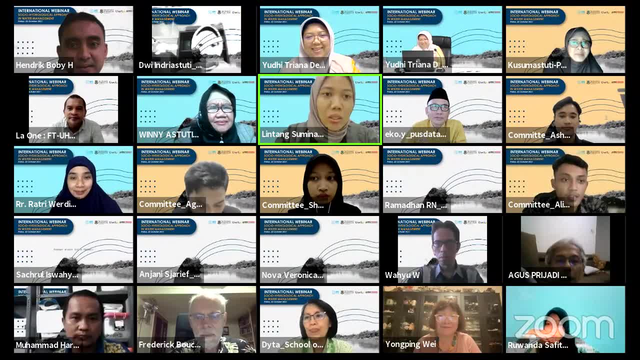 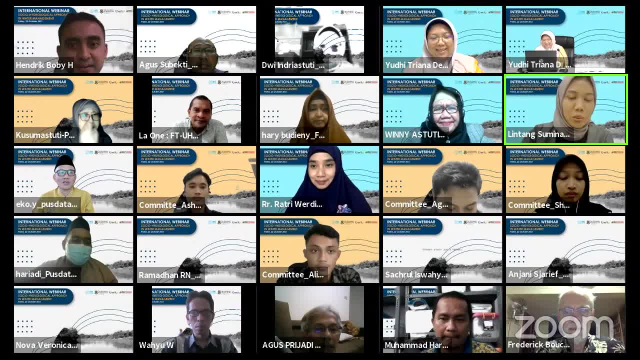 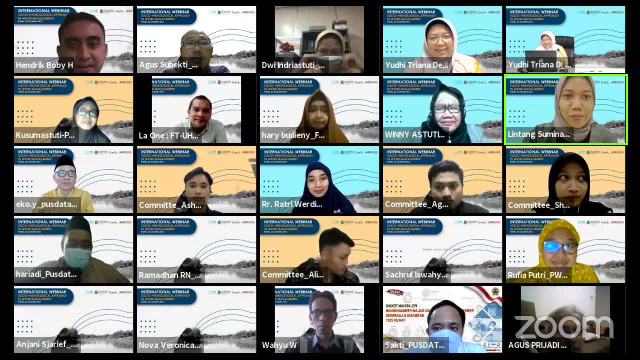 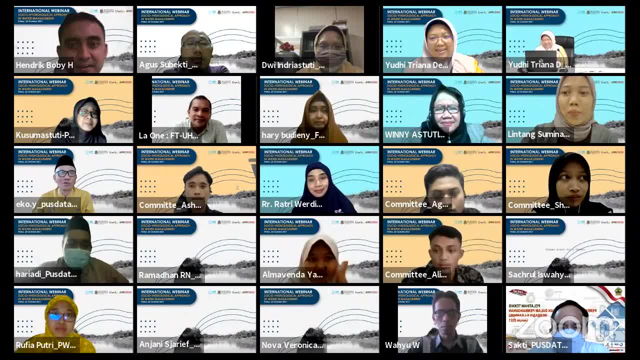 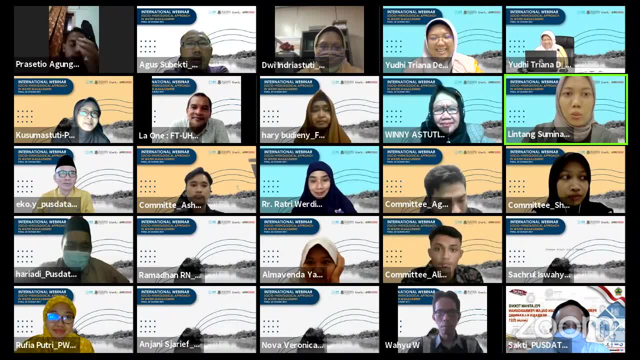 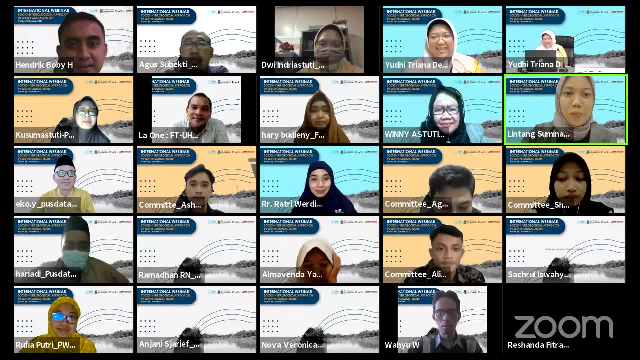 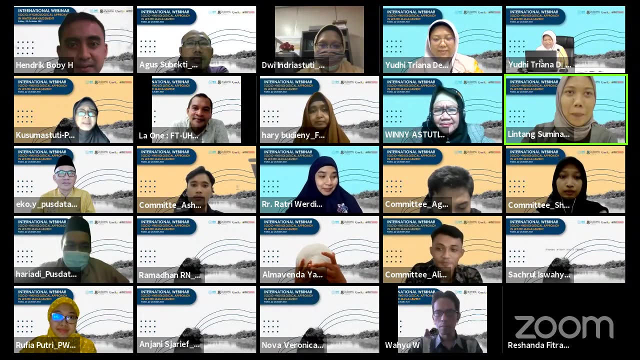 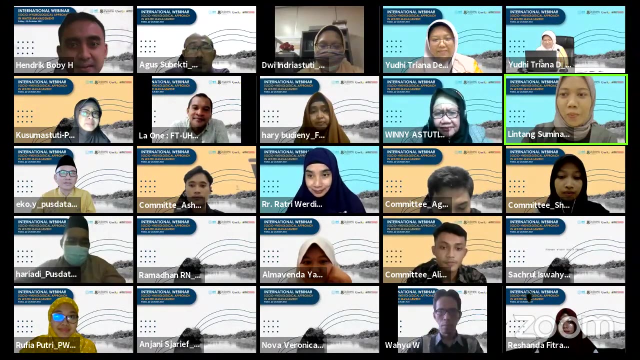 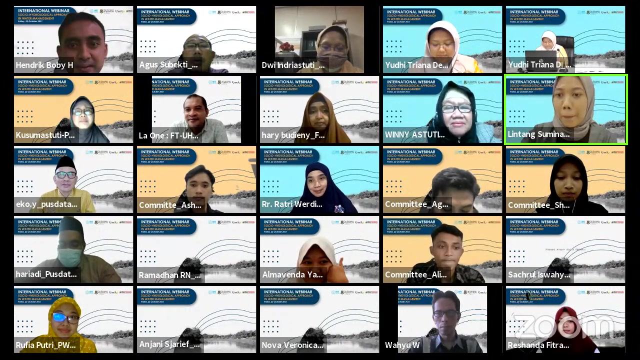 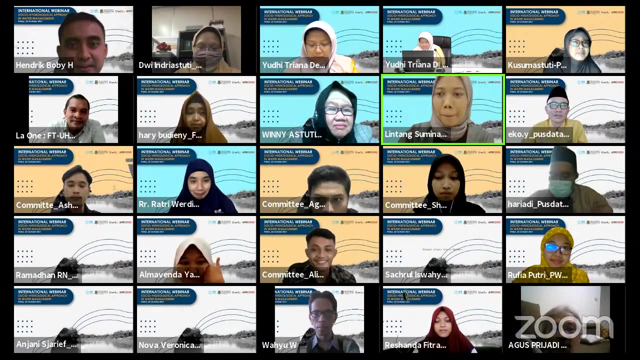 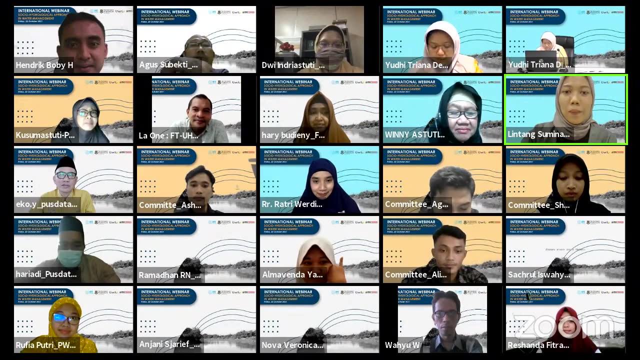 page one: one, two, three. Come back here. Page two: one, two, three. Page three: one, two, three. Page four: one, two, three. Page five: one, two, three. Page six: one, two, three. 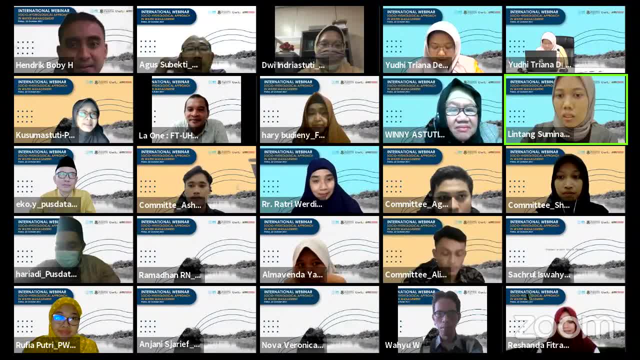 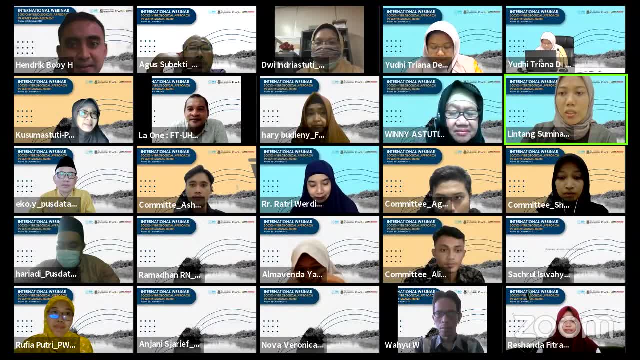 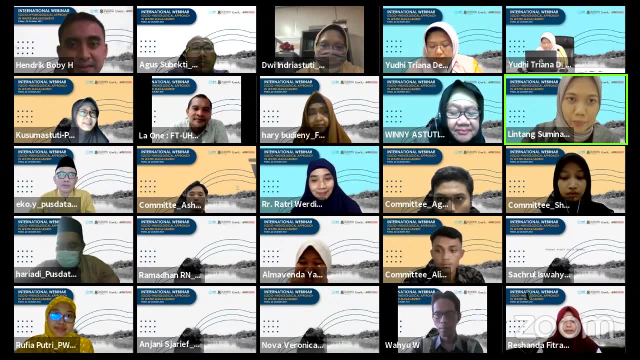 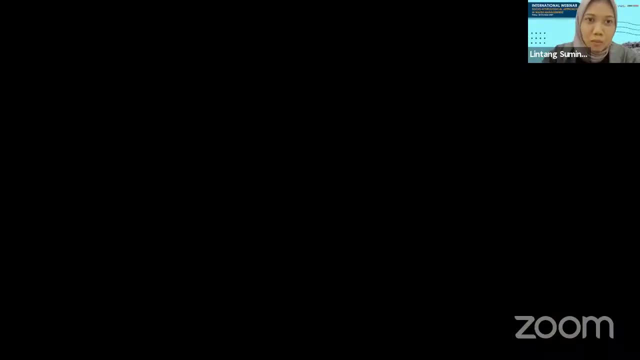 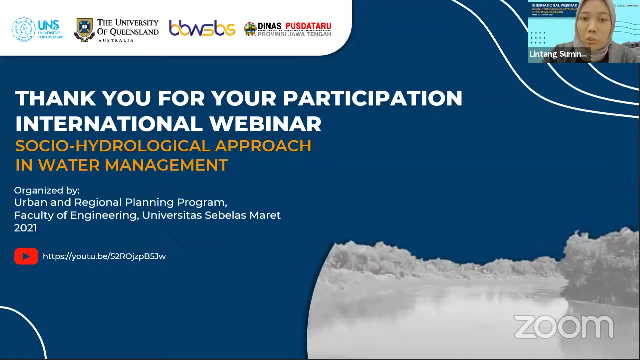 Page seven: one, two, three And the last page: one, two, three And the last page: one two, three. Well, thank you all And yeah, I'm sorry if it takes too long. Okay, and once again I would like to remind: 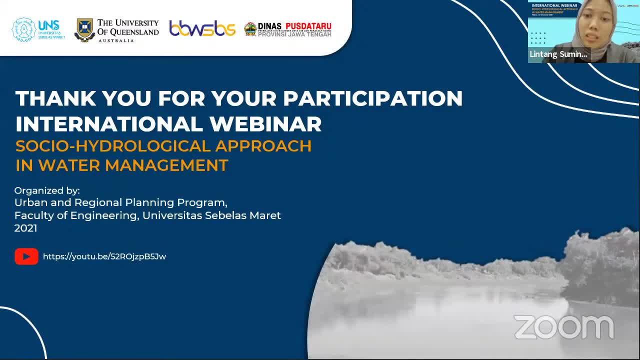 to all the participants to fill the attendance form in the link that is already shared by the committee. The committee will send your certificates and also the materials of today's webinar based upon your attendance record, And, for those who are not yet registered, please do make sure you have the details. 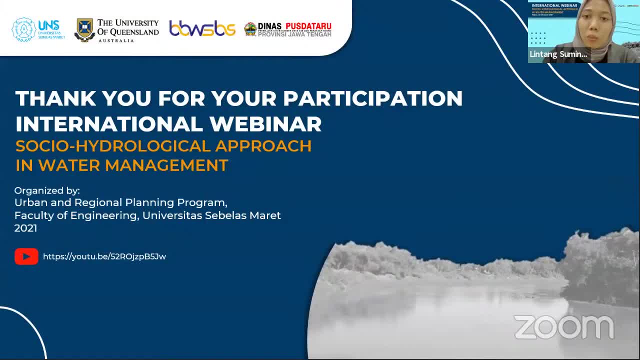 of your attendance record sent in within the first week after this event through email for all the participants in this Zoom meeting and also the participants in YouTube live streaming. I would also like to thank once again to all the speakers here: Professor Yongping Hui, Dr Frederick Bukert. 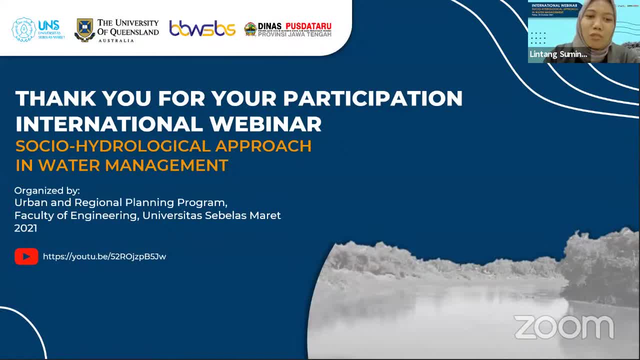 Bapak Eko Yunianto, Ibu Yudi Triana Dewi, and also Dr Atri Werdimin Thias and also Dr Paramita Isawar, Mujerator. today. On behalf of the team, I would also like to thank everyone here in the room. 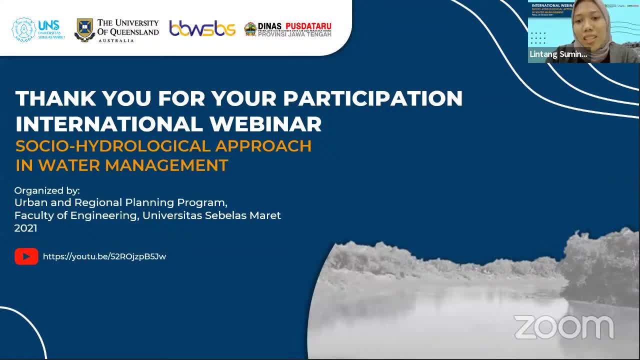 i'd like to thank you all for joining and participating in this webinar. socio-hydrological approach in water management. i'm tindang suminar signing off. stay safe and stay healthy, and see you again in the next event. wasalamualaikum, warahmatullahi wabarakatuh. 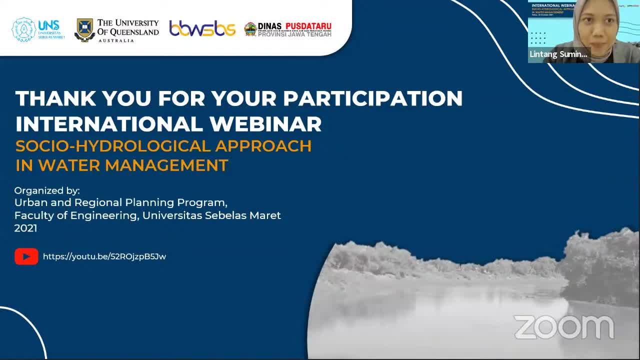 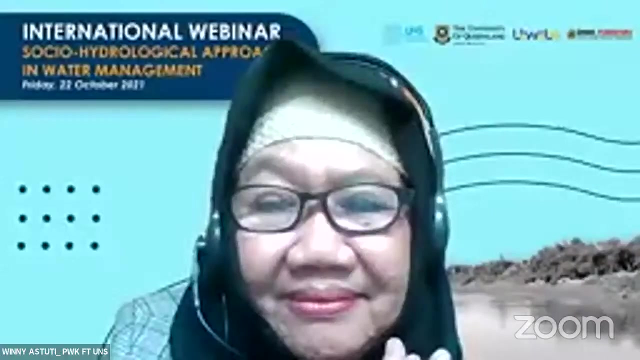 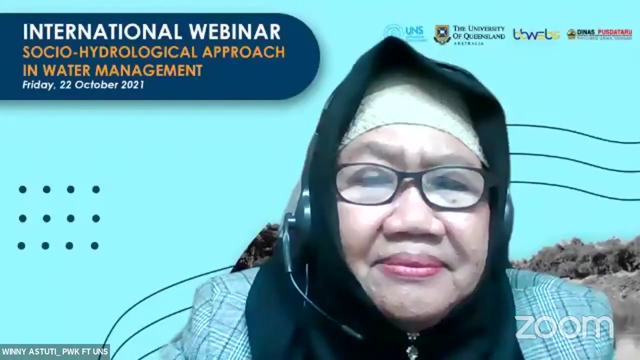 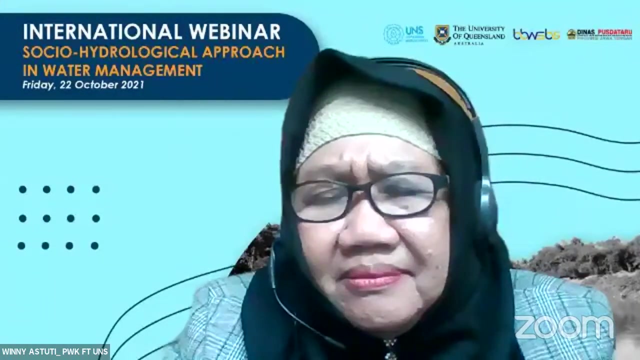 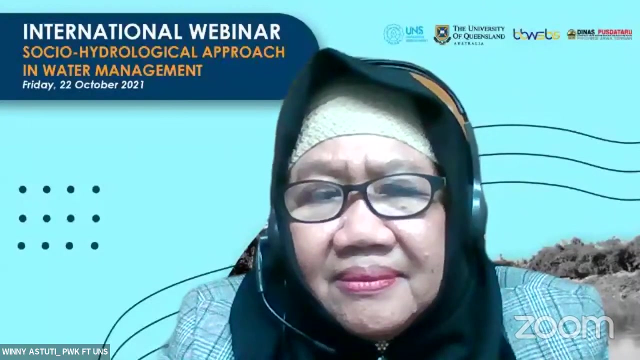 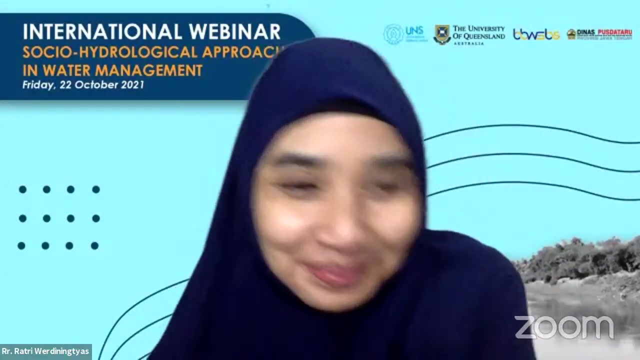 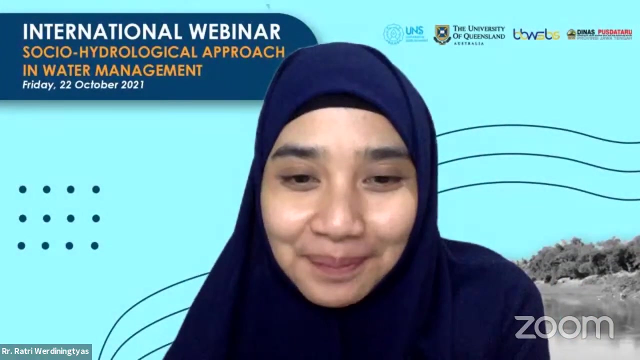 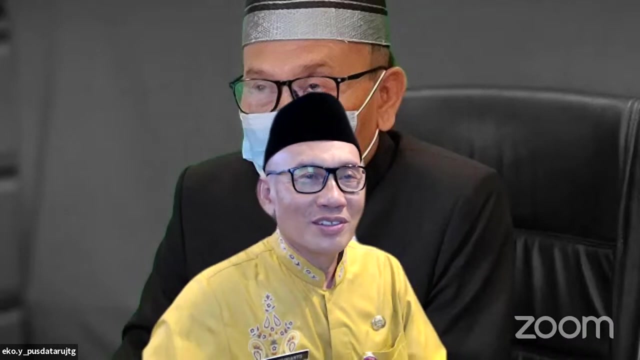 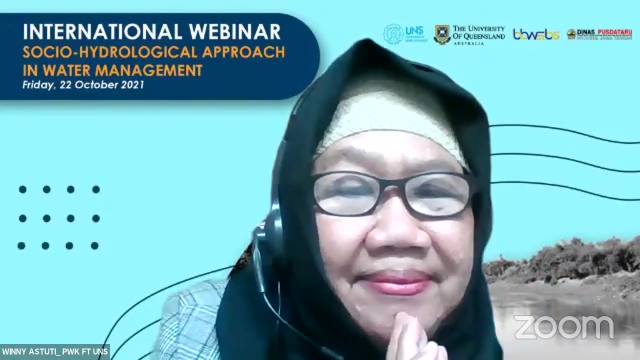 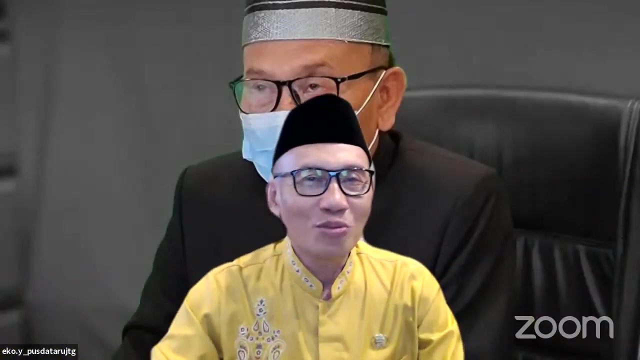 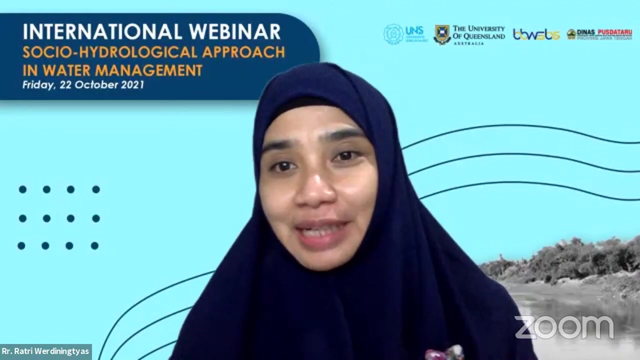 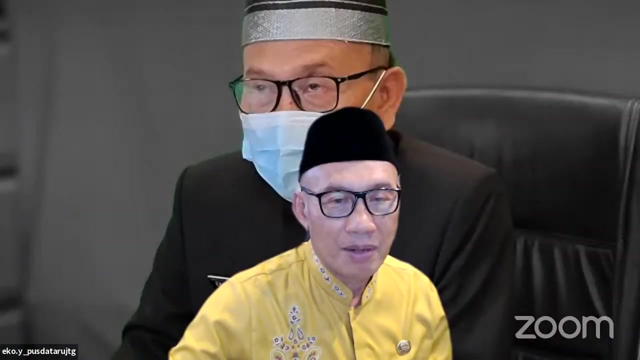 thank you, professor yomping, thank you, thank you, thank you all, thank you, yes, close. i think we can uh close the stop the recording. thank you very much. foreign, foreign, foreign, foreign, foreign, bye foreign. So do you know about this, Habibah? A new case, right, Sir? 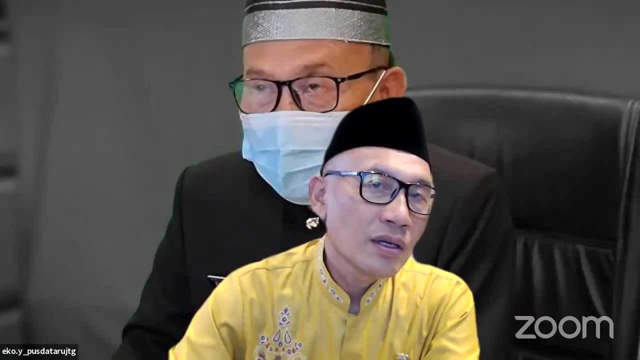 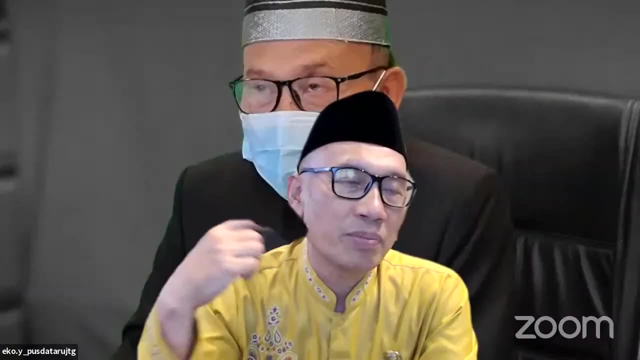 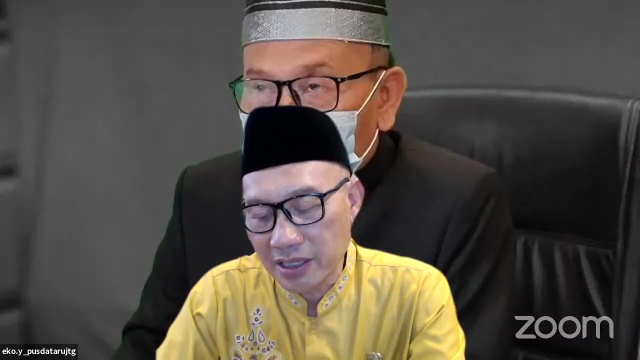 Is it Jakarta? Yes, in Jakarta, In Semarang Ma'am. Yes, our installation is in the field of space arrangement. Oh, that's right In the section. the section is for the use of space. Oh, that's great. 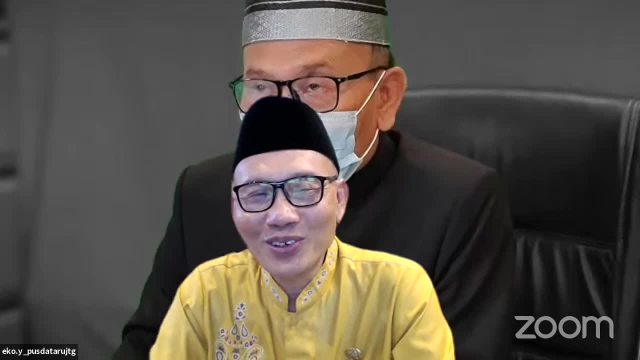 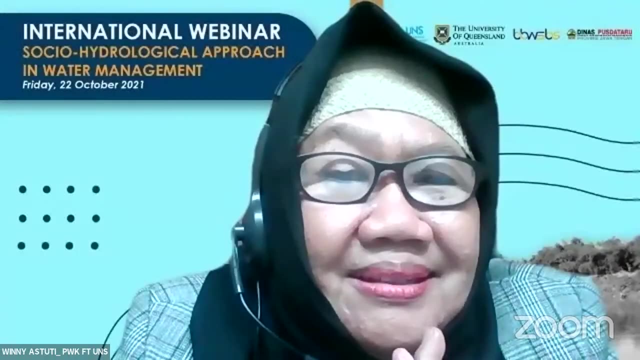 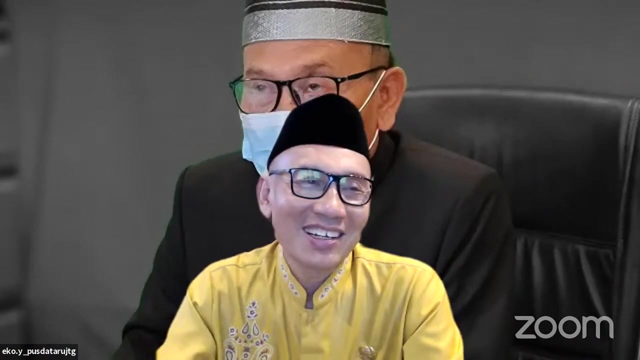 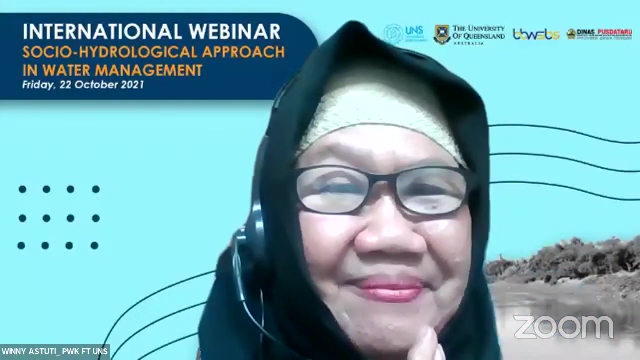 I hope it will develop. I'm still on vacation. You're still on vacation? Yes, I'm still on vacation. Yes, I'm still on vacation, And later the students can come. Oh, yes, Maybe after the practice or work. 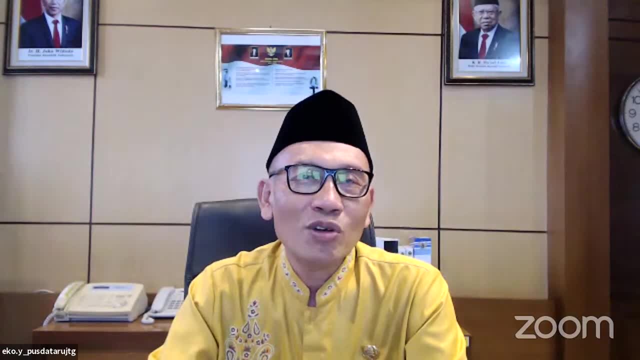 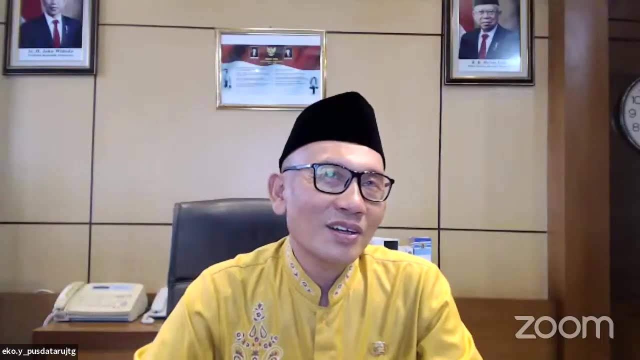 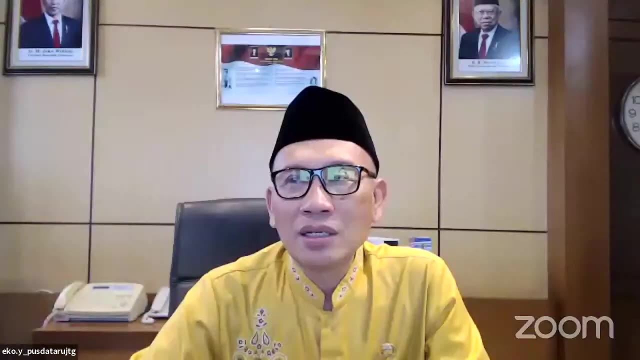 In the province of Central Java. the PU is from all the WNAs. Oh, that's right sir. Yes, sir, Is this already put? sir Menawi, Mr Sakranagara, Yes, sir, What's the name of the PU, sir? 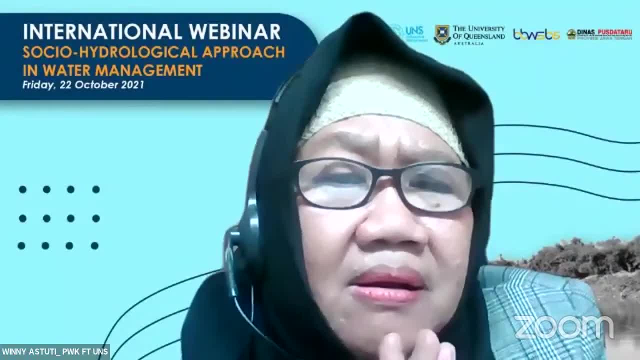 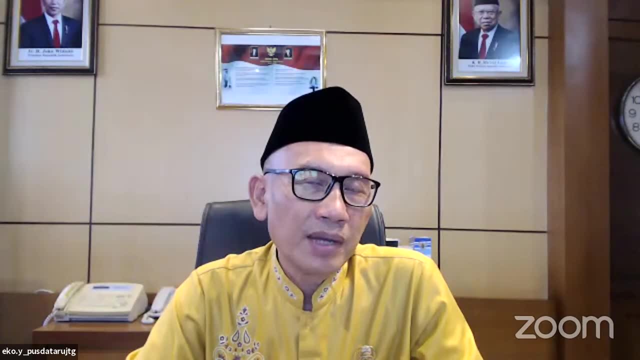 It's called Cipta Karya, Cipta Karya sir. Cipta Karya is Mr Arief sir, But the unit of our class is 82.. Mr Arief Priyuka. Oh, Mr Arief. 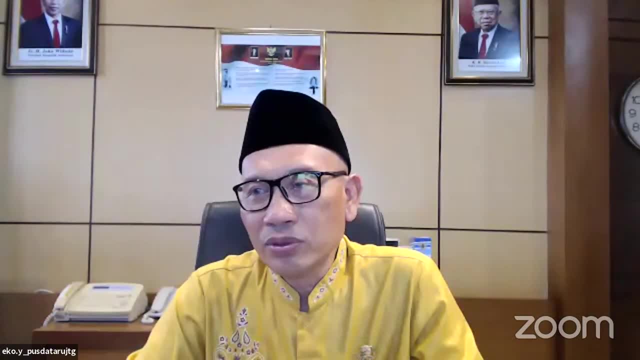 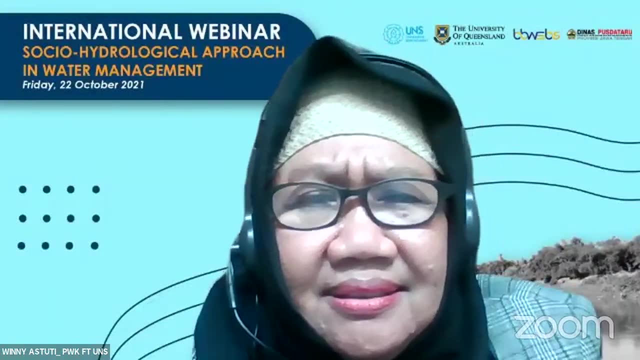 And the one in the city is from the architect. sir, Who is it, sir, The official secretary? Oh, the one in Solo, sir The secretary is from. The architect is also Mr Arief, sir From Delanggu. 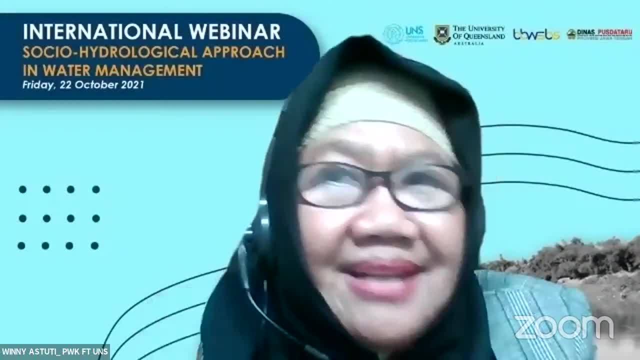 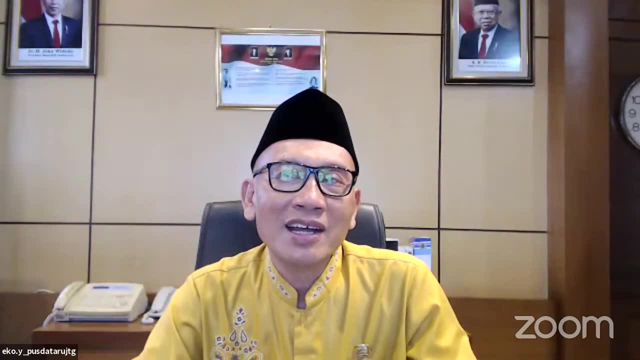 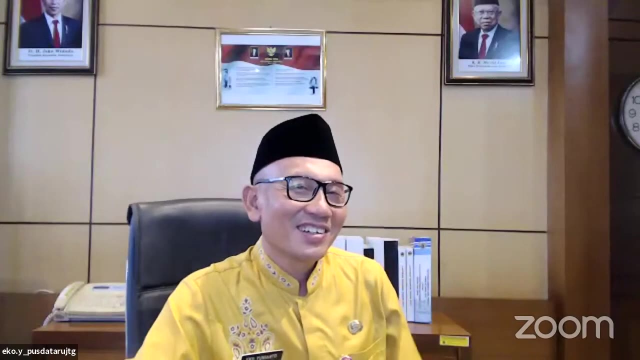 Oh sir, Mr Arief has also been invited. Every Wednesday there is a routine ceremony. This is a ritual ceremony, sir. Yes, sir, Oh sir, We have also been invited, but not yet. That's exciting too. 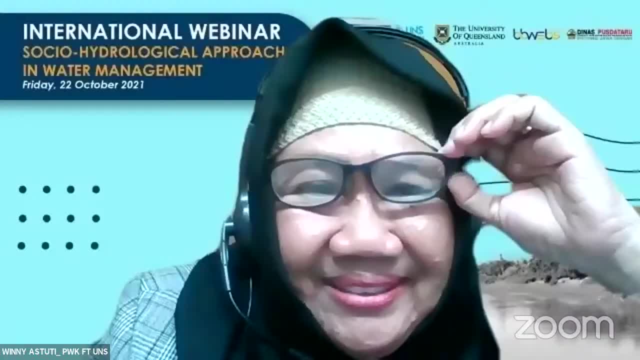 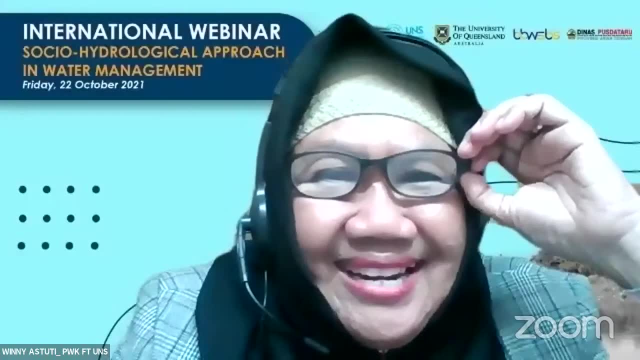 A lot. Yes, sir, We haven't been invited for a long time. We haven't been invited to campus for a long time. Yes sir, Campus. Yes sir, The rules of the village. Yes sir, Yes sir. 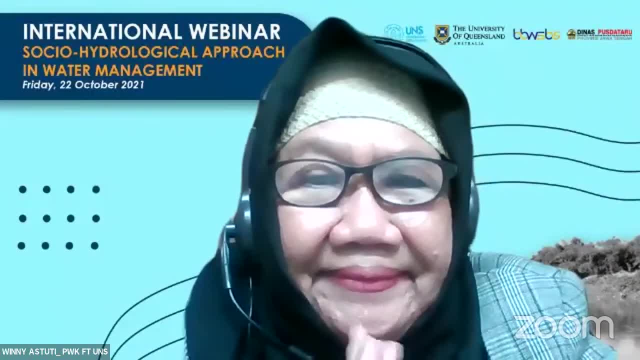 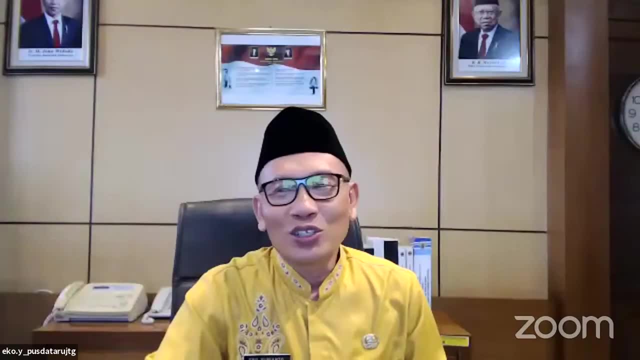 Of course, Of course, Yes, sir, Please, please, Please sir, Thank you. Okay, thank you, Sir, I'll bother you again, sir. Yes, sir, I'm happy There are people who are ready. 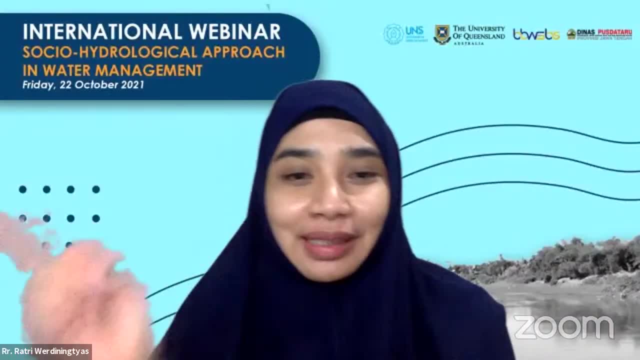 There are people who are not ready. Yes, I'll turn around, sir, Change sir, Yes, sir, yes, sir, yes, Yes, sir, Yes, yes, sir, Yes, yes, yes, sir, You're a little skinny ma'am.